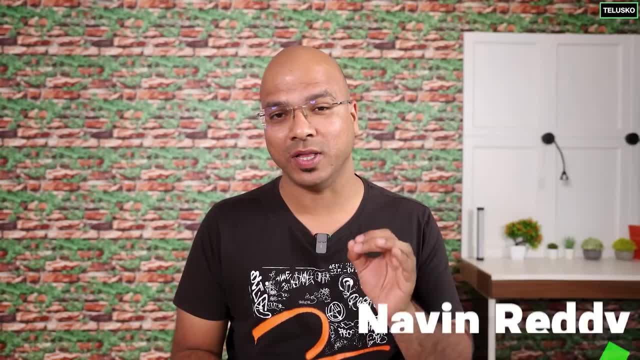 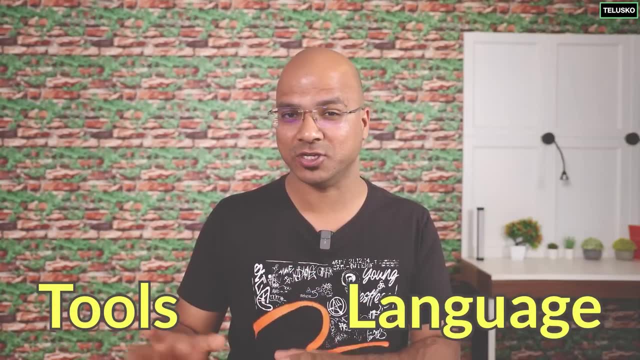 Welcome back aliens. My name is Navin Reddy and in this course we are going to learn about Git. Now, when you build an application, apart from learning the language and the tools to build the application, there are other things which you have to learn about, and one of it is Git. So that means 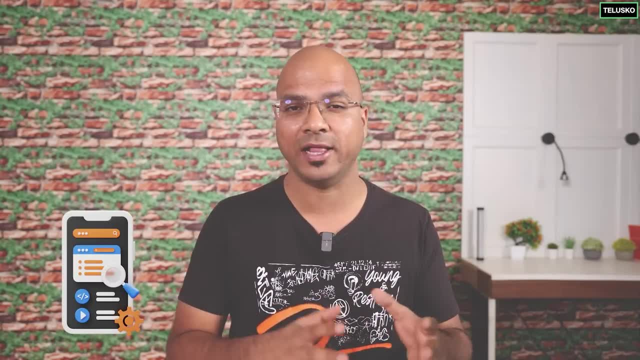 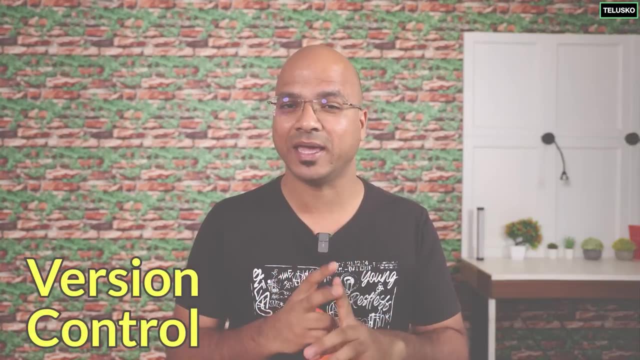 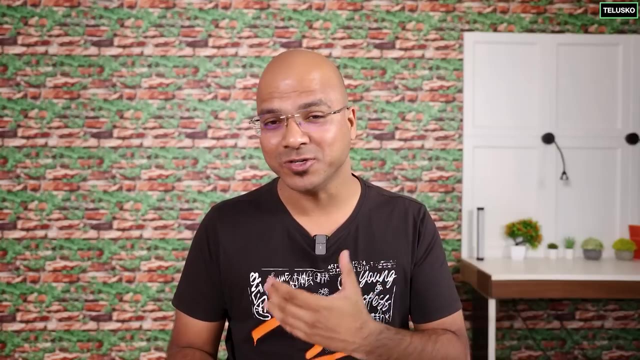 irrespective of what kind of application you are building- it can be mobile web enterprise. you will be using this tool for two reasons: One for the version control and second for the collaboration. And then this tool is actually easy. it's just that the concept might be new and most of the 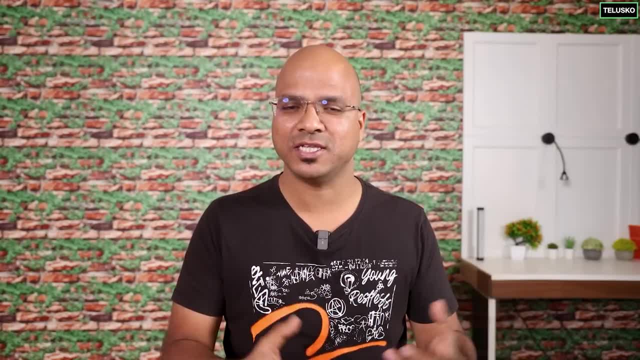 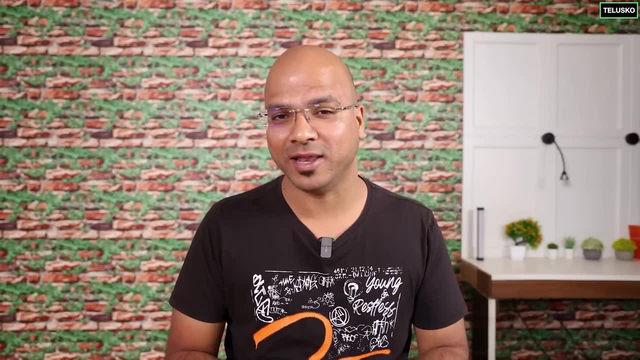 thing which we do is through commands, And of course, you can do most of these things with the help of GUI, because most of the IDEs provide you with this tool, But then, when you work with the command line, you have more power to change stuff. So in this course, we are going to learn different. 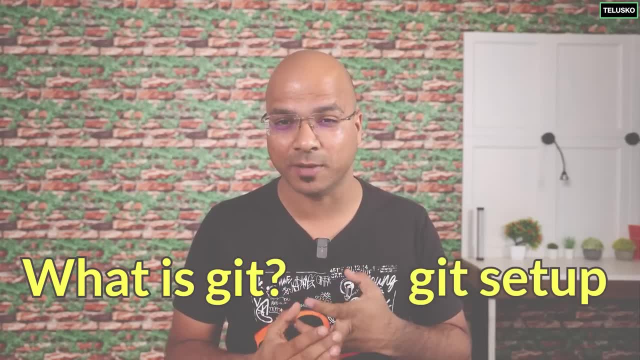 things. First of all, we'll understand what is Git, how do we do the setup, how do you create your own repository, how do you create account on GitHub, how to installize the project, commit the project and how to build your own Git application. So let's get started. 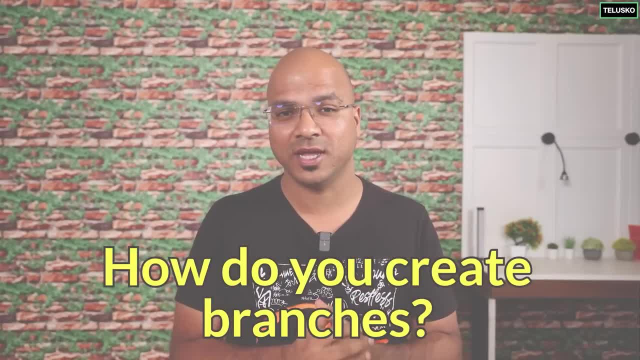 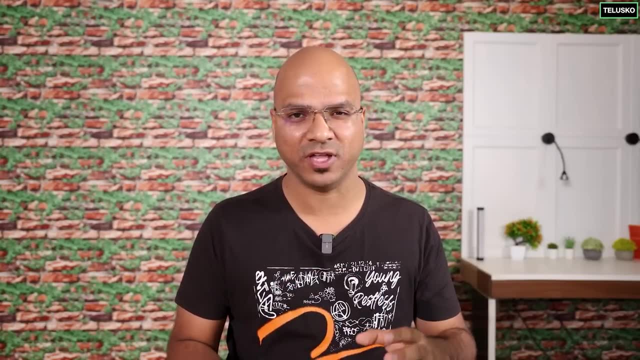 And how do you push your code on the GitHub repository, how do you create branches, and we'll be doing that practically, So you will enjoy this course. and don't worry, the course is designed for the beginners. Even if you have no idea what Git is, we will take care of it. So I 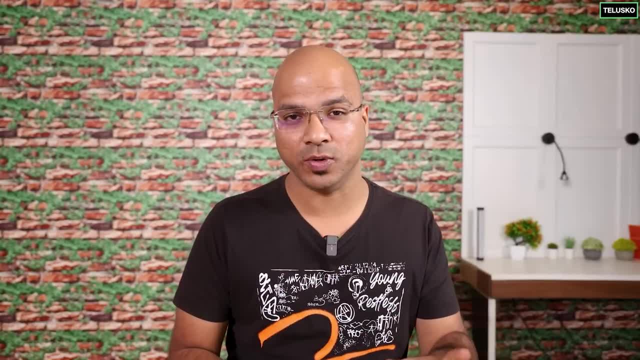 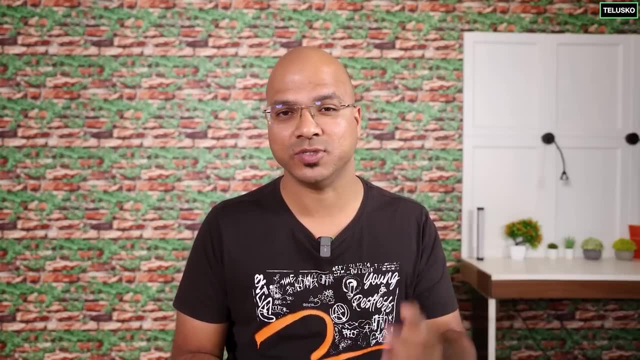 hope you will enjoy this course and also make sure don't just watch the video, practice the thing by yourself. So whatever I'm doing parallelly, you can do it on your machine and let me know how it feels or if you have any issues in the comment section. Git is a distributed version control. 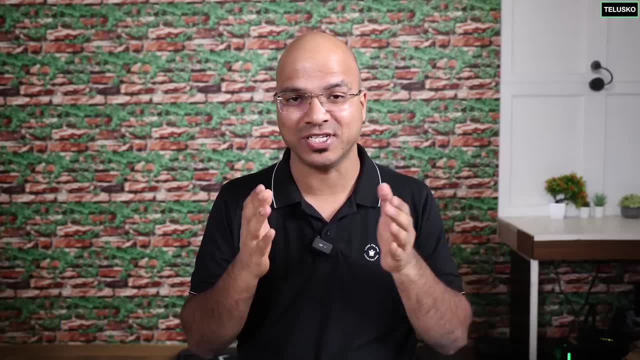 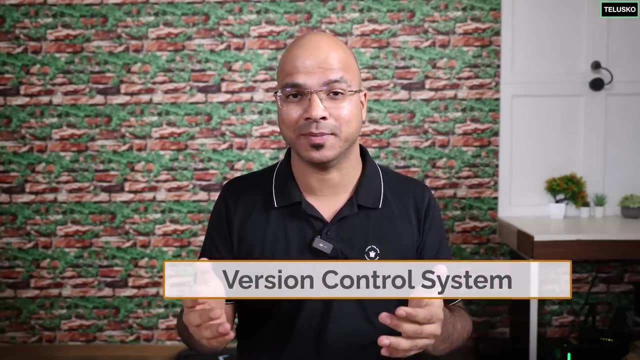 system. Git is a distributed version control system. Now the problem is, if you want to understand Git, you have to first understand what do you mean by version control, And then we can discuss about version control system, then we can discuss about why it is called distributed, and then Git will make much more sense. 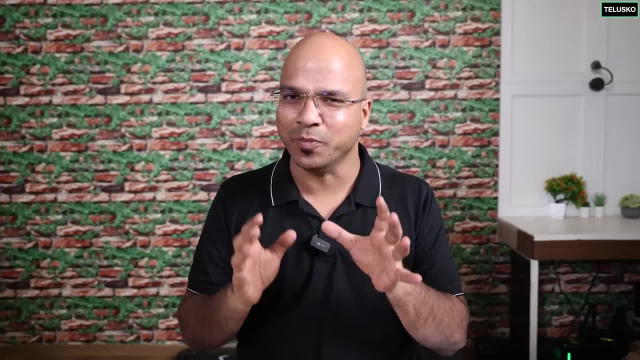 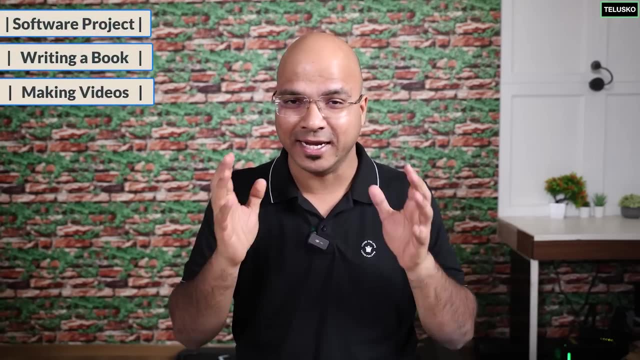 So let's talk about version control. See, the thing is, when you make a project, of course it can be any project. It can be a software project, or it can be writing a book or making videos. It's all about a project. And when you make a project, the way you work is you. 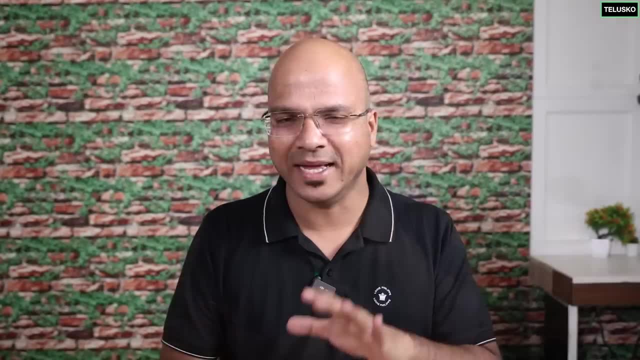 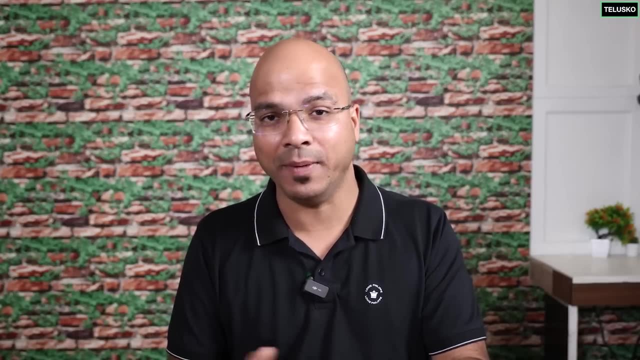 create different versions of it. So if you don't want to say version, let's say you make multiple updates. So when I start writing a book I will write something and then I will edit the same file. Or maybe I want to go back to my previous file. So let's say, if I'm writing chapter one, 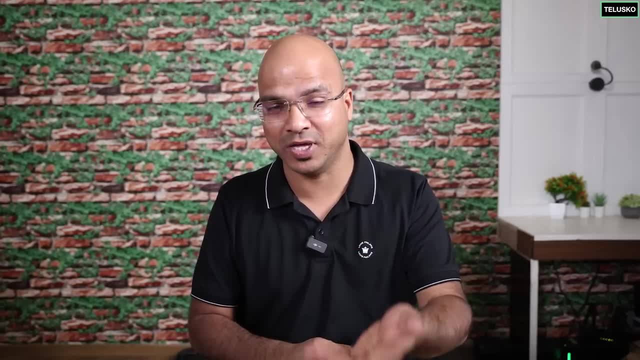 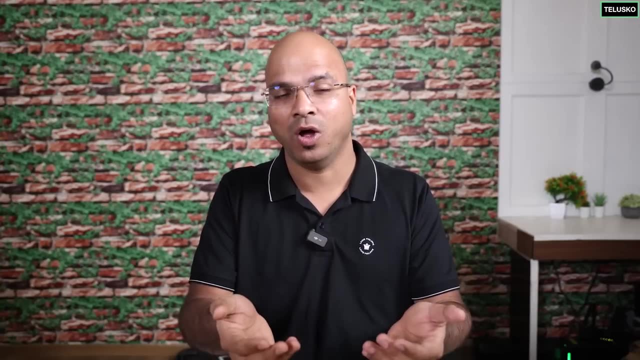 I will complete that chapter one and then I will go for chapter two, chapter three. Now, at every chapter end I will just try to save it, And then, on chapter two, I will try to save a file. On chapter three, I want to save a file, Or maybe while writing this: 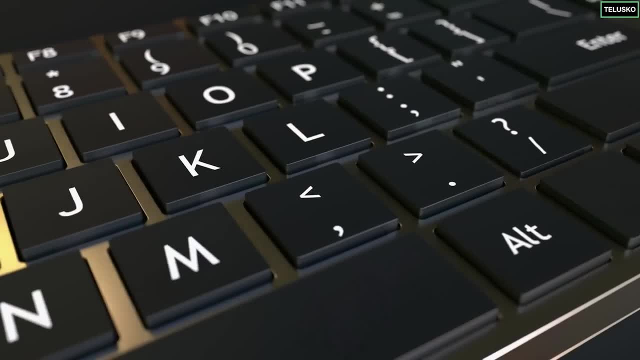 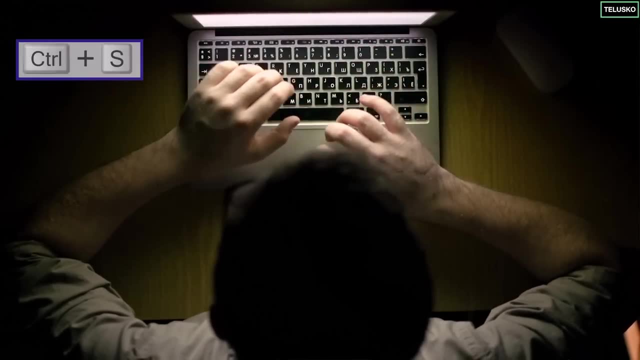 I will do the save right- And saving is very important right- Otherwise, if your laptop crashes, you will lose all data. So, as a writer, we normally say: control S, not once, multiple times, just to be on the safe side. The important part here is we want to. 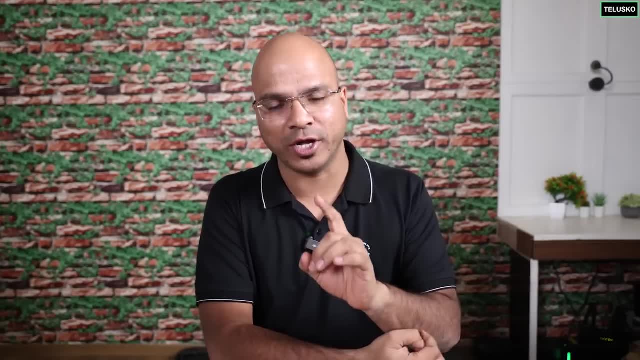 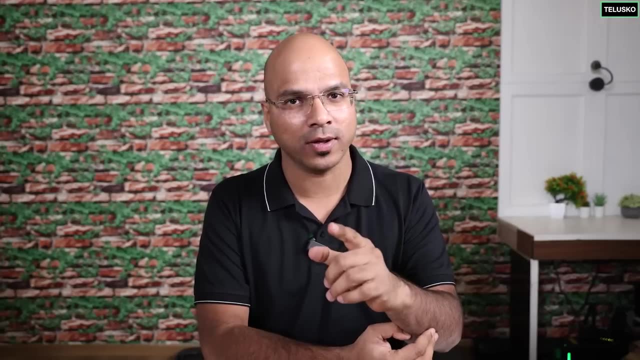 make the copies of it. Now, there are multiple ways of doing that. What you can do is you can save the same file. The thing is, if you save the same file, you will lose the previous file, right? Or what you can do is you can create a new file, So every. 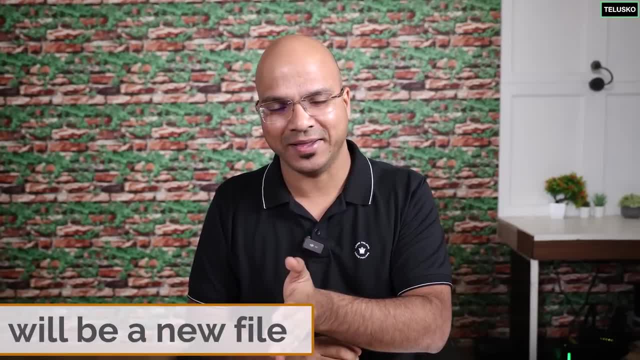 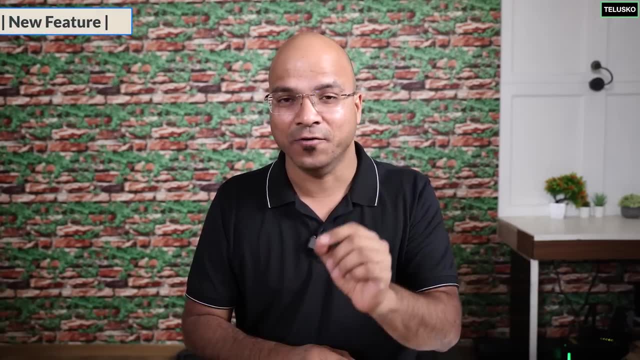 new update will be a new file And, as a software developer, we used to do that in my college days. I remember when we used to create a project. every time we add a new feature, we used to create a new folder And let me know if you have done this, or maybe you can just give a smile if you have done. 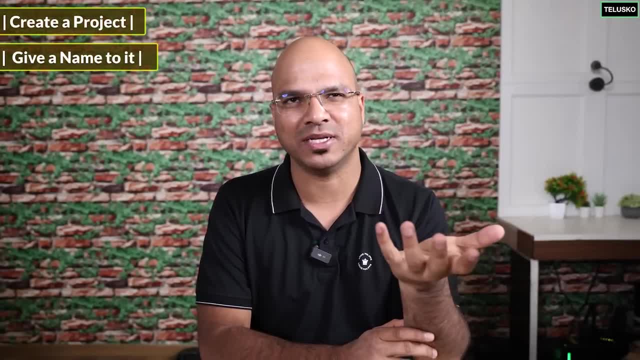 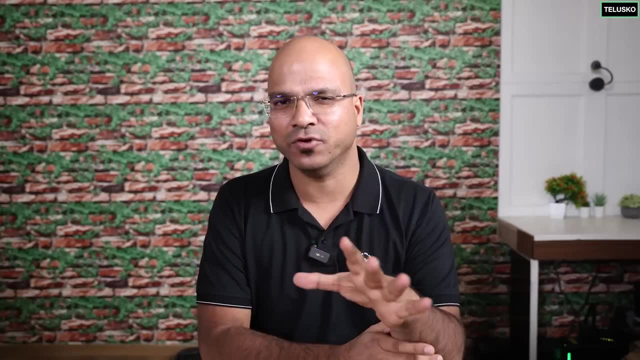 this: We create a project and then we give a name to it. Let's say the project is for a quiz application, So you will say quiz app. And then, if you think this is now we have added few features, we can say quiz app one, quiz app two, quiz app three, quiz app four. So we can say quiz app one. 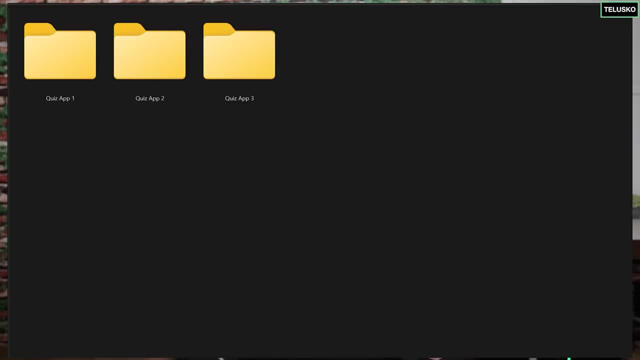 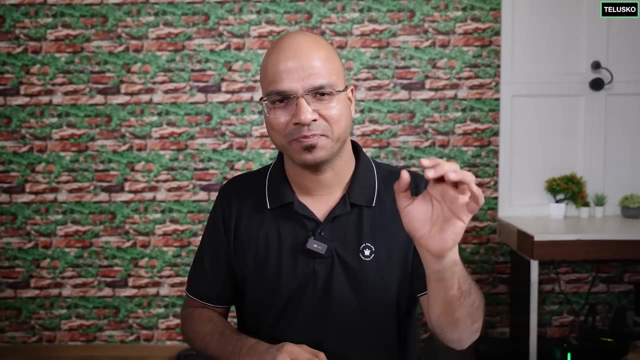 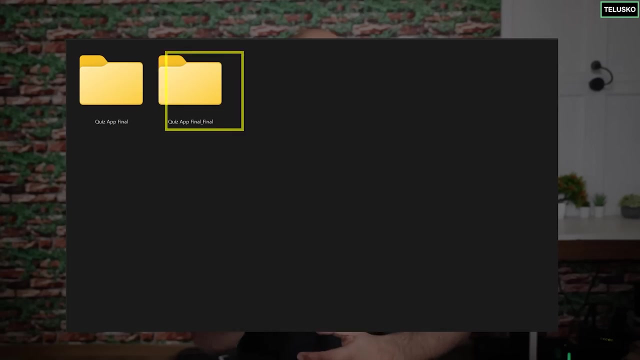 quiz app two. quiz app three: Of course it will have a new updates, new features in that particular new folder right. And then, the moment you feel that project is complete, you say quiz app final. then you say quiz app final, final because maybe you want to make some final changes. 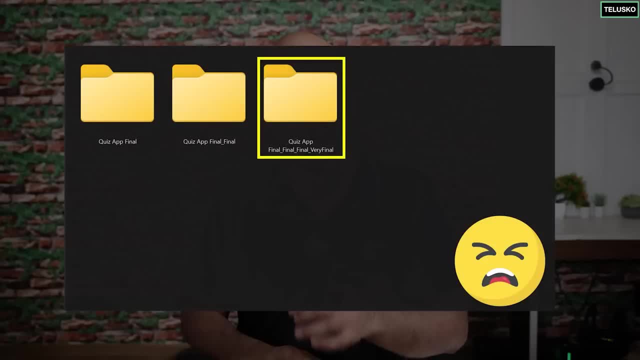 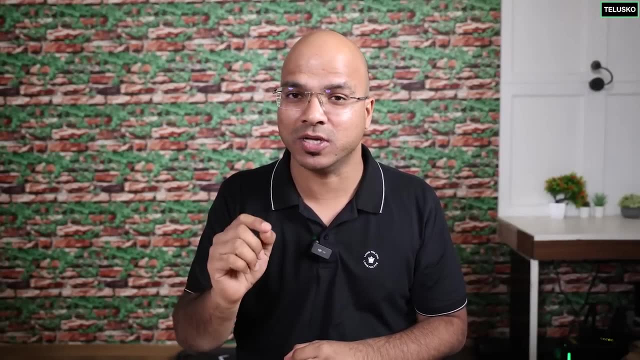 And then you realize, oh, there's a bug. Then you say: quiz app: final, final, final, very final. Okay, So this is the type of folder we used to create. The thing is, why do we do this? It's because 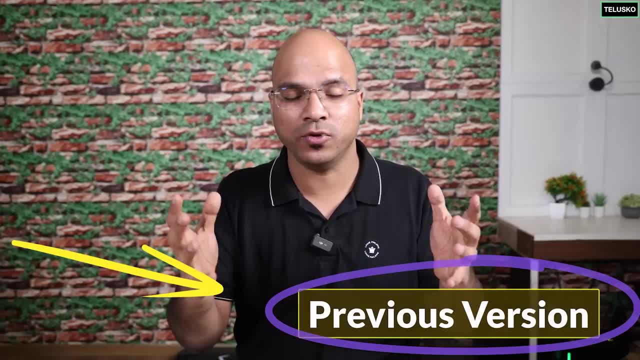 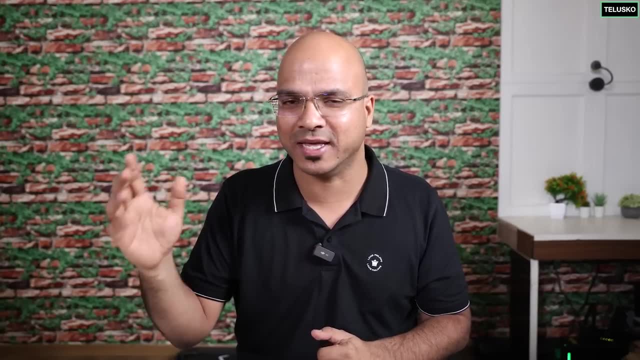 what if you want to go back to the previous version? What if you have created a project and then it's working and now you added new features and then you thought it is working, but it's not. there are some bugs. You may want to go back to the previous version, right Now having that version. 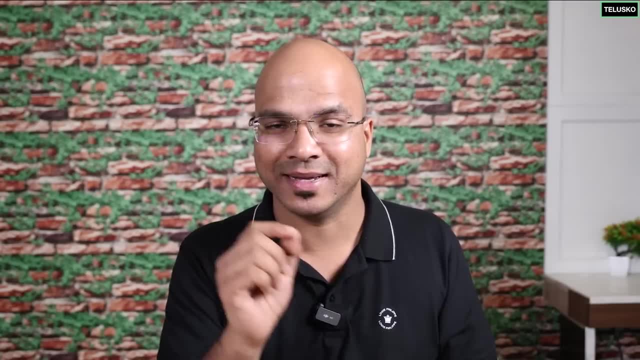 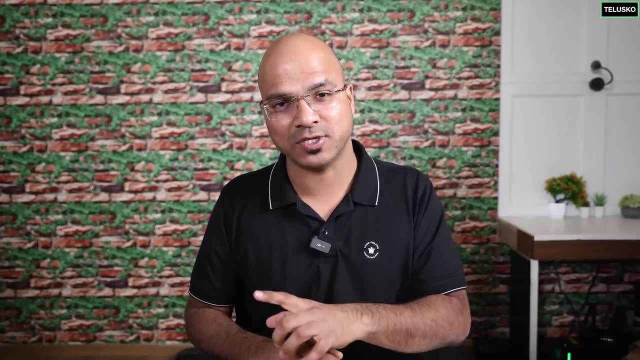 called or having that power of going back to any version. that is called version control, And to achieve this we need to use some software, some system, and that system is called a version control system. So we need to use some software to achieve this, And to achieve this, we need to use some. 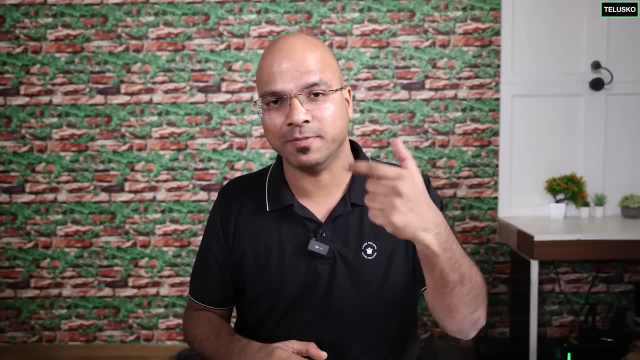 software to achieve this. And to achieve this, we need to use some software to achieve this. So, example, if you are building a project, you will be saving that file multiple times and then you will not replace the older project. The older project will be there, right? So let's say you have a software. 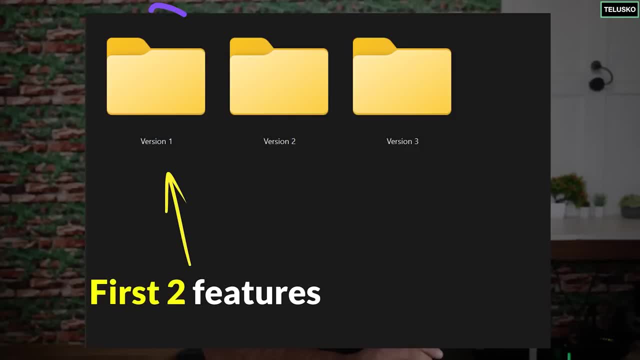 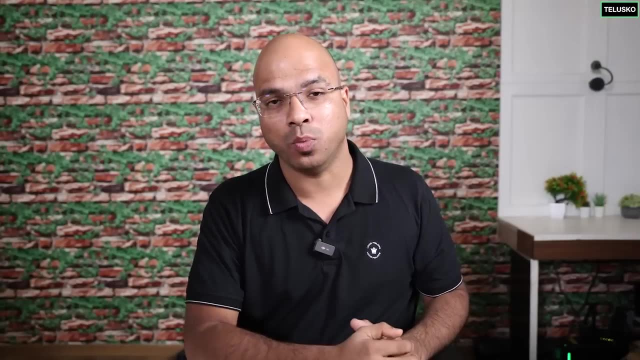 with X number of features. So you got the first two feature in the first version, Then you got the third feature on the second version And at any given point you can go back to the previous version. Also, what if you are not alone in the project? You have multiple people working in the 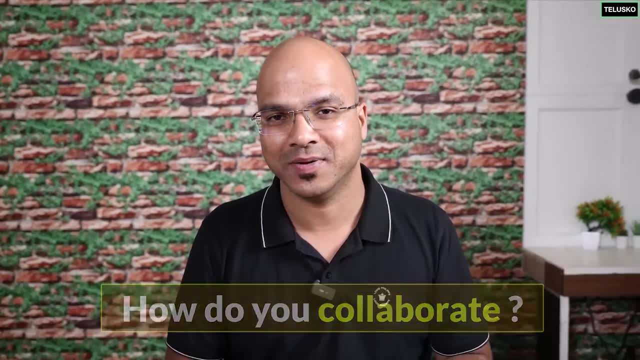 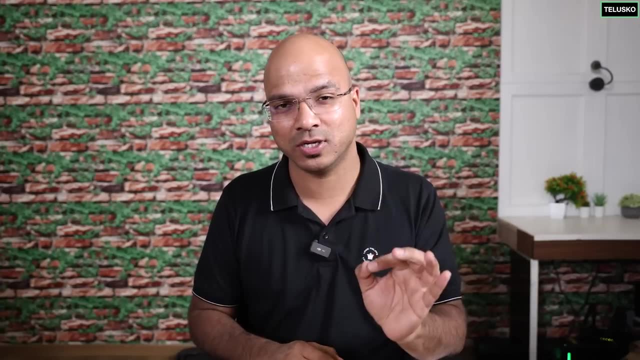 same project. How do you collaborate? That's also important, right? So you will get those features with the help of version control And, as I mentioned before, you need a system, So we call it as a version control system. Now, when you talk about version control system, we can categorize. 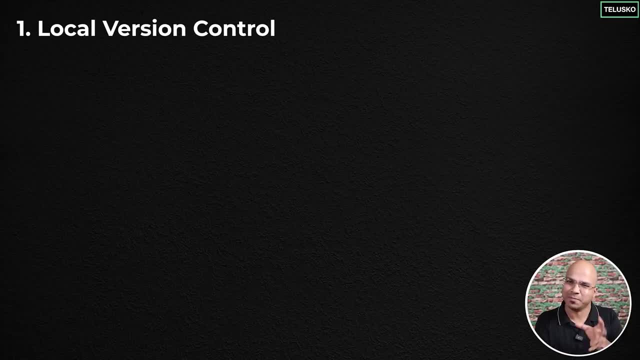 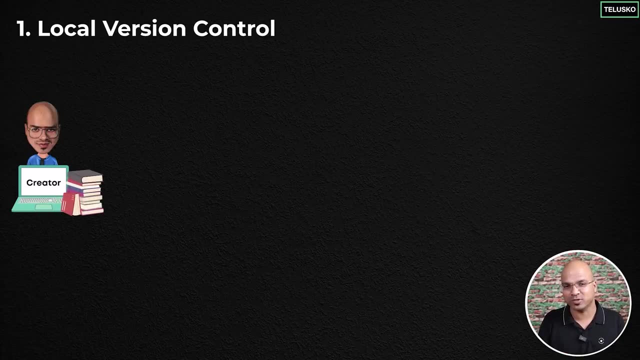 into three parts here. The first one is a local version control, which simply means that, as a developer or as a creator, if I write software or if I write a book, if I write something and if I want to save in my own machine with different versions, of course that is local copy right. 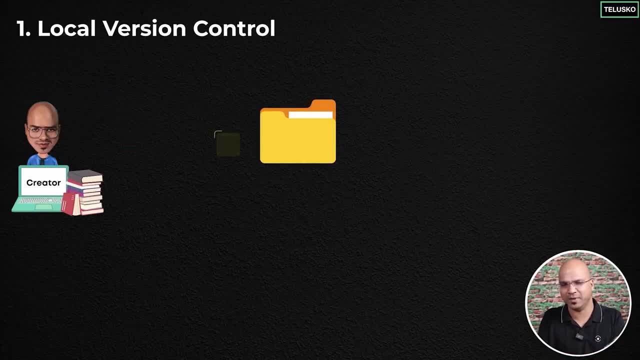 And in my own particular machine I'm creating different versions of it, Maybe having a folder inside a folder. Then I can create a folder inside a folder, And then I can create a folder inside a folder, And then I can create a folder inside a folder, And then I can create a folder inside a folder. 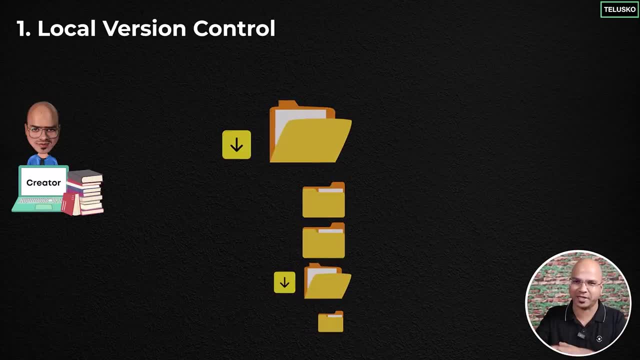 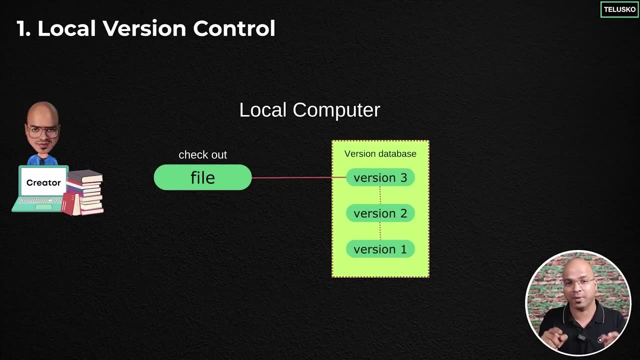 Then having different folders of it, Or maybe I can just create a database where I will save all these files Again. that's my choice, or that depends upon the version control system. But the thing is everything is happening on my machine. The problem here is what, if I want to? 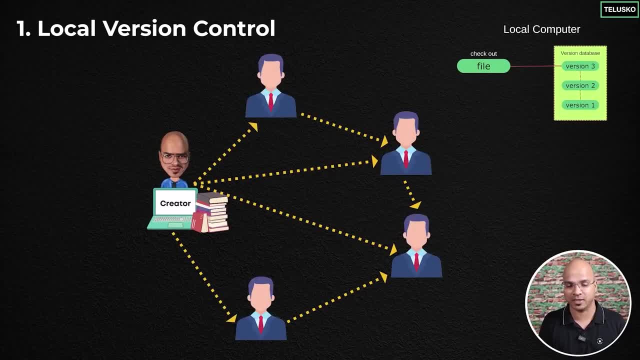 collaborate with other people. I have, let's say, five people in the team and they all want to work on the same project. How will we do that? And also, what if I'm relying on my machine and then one day my machine says, okay, I'm done, I'm not going to start again? How will you get your? 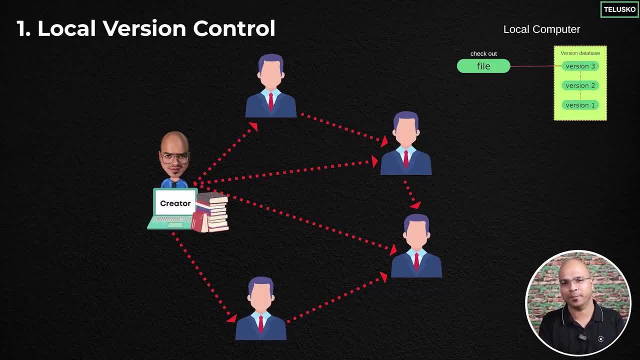 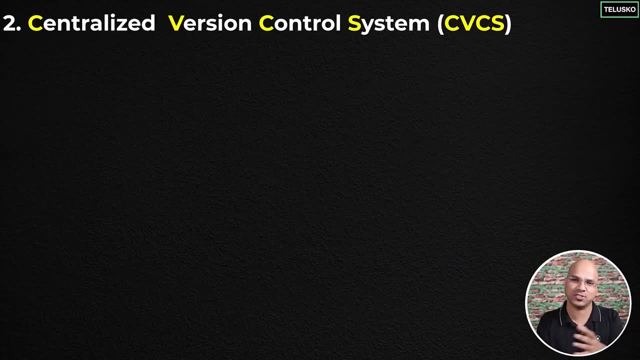 projects, And that's where you can't simply rely on local copy. And that's where we have one more option, which is called CVCS. So VCS is version control system. CVCS is your centralized version control system. Now, in this case, what you do is, let's say, you have five people in the network, or 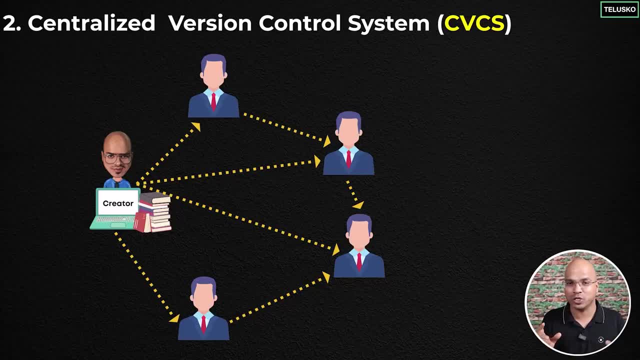 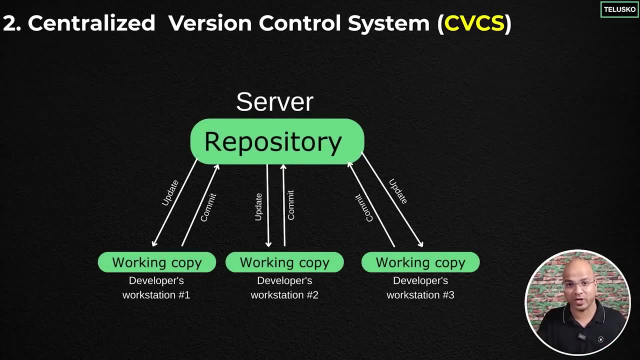 five people want to work on the same project. So what you will do is you will use a central repository, not the local one, but a remote one. So all these machines which you are working on in different locations in the world, you will be having a local copy, And that's where you can. 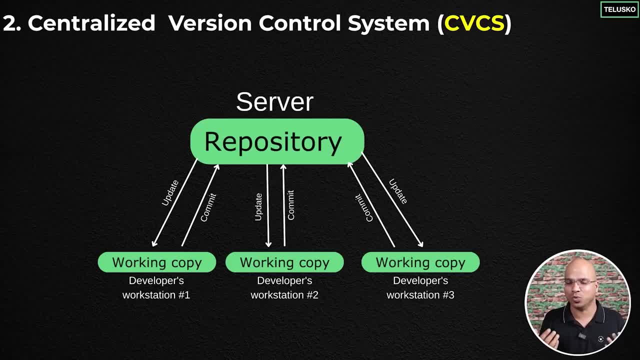 use a centralized version control system. Now, at this point, every time you want to make a change, you have to get the copy from the centralized system, make the changes in your machine and then you have to save it on the centralized version control system, which is CVCS. 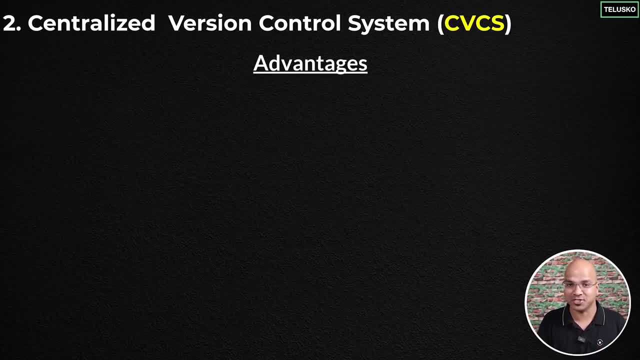 Now the problem with this is okay. first of all, let's talk about the advantage. The advantage is, if you are working in a file of a group, everyone has access to it, So they will know what you're working on. So let's say you have done something, and then when you say: save Now, basically, 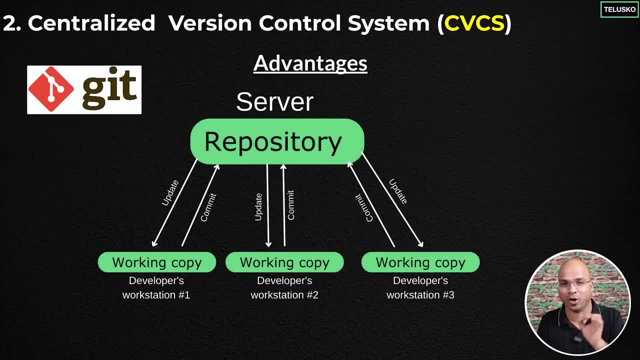 since we're talking about Git, let's use the word which we use in Git, called commit. So let's say: when you commit something to the centralized server now, at this point, the other people will have a recent code. They know what you're doing, right? But also 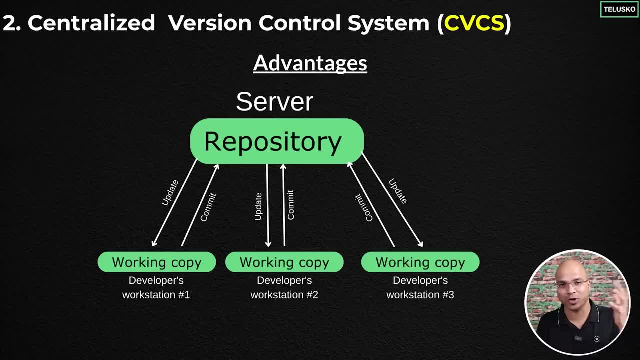 there's a problem. The problem is: everything is stored on a central system, right? What if the central server says: I'm done, I'm not going to start again. your data is gone now, right? So that's the problem with the centralized version control system. Now that's where we have to look. 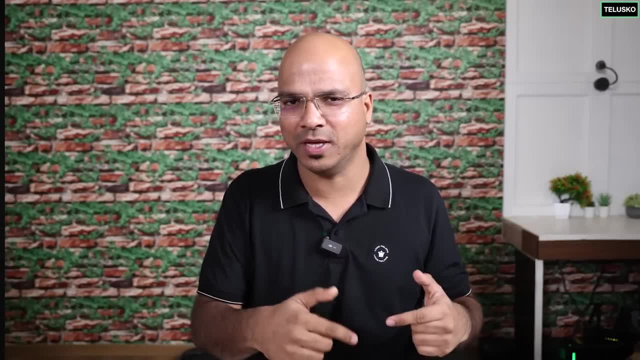 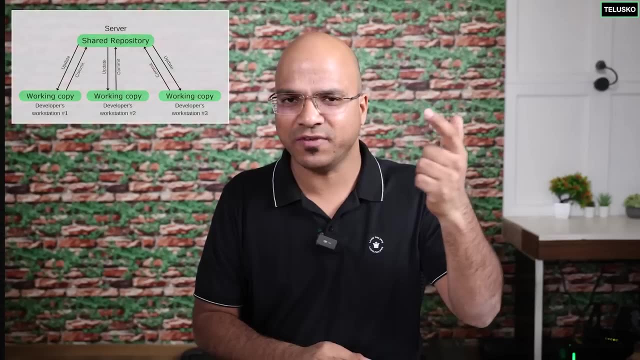 for an alternative where you should be able to have a copy on your machine as well, and not just you should have the history as well, because in the centralized version, even if your server goes down, at least you have a local copy of the current version. Yes, you have it, but we don't. 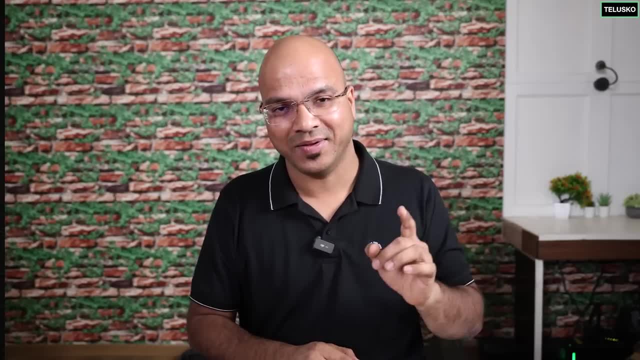 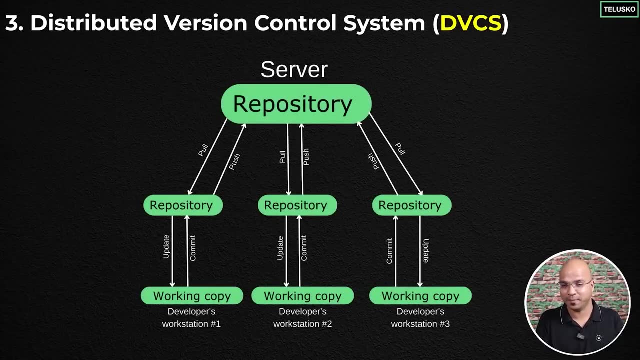 want just current version. What we want is the history, right, And that's where you can use something called a distributed version control system, where you will have a local copy but not just the current version. You will have the entire commit history. So let's say you have created. 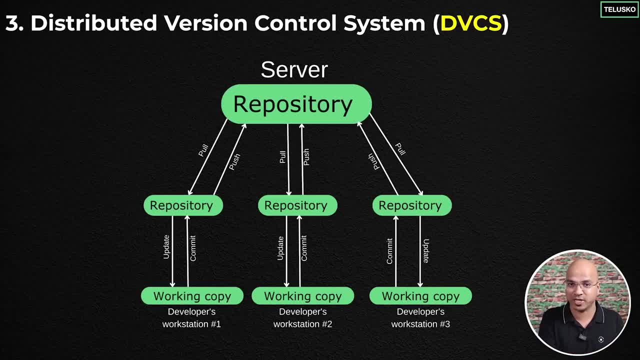 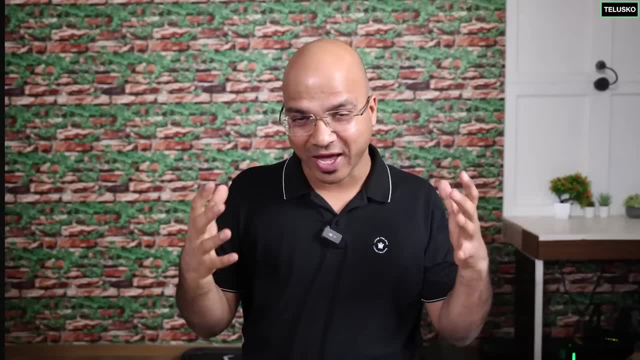 version 1, version 2, version 3,. everything will be present in your local machine as well, and you can collaborate with the other developers or with your colleagues. basically, So we have done with the first step of what is Git by understanding something called version control system. Now 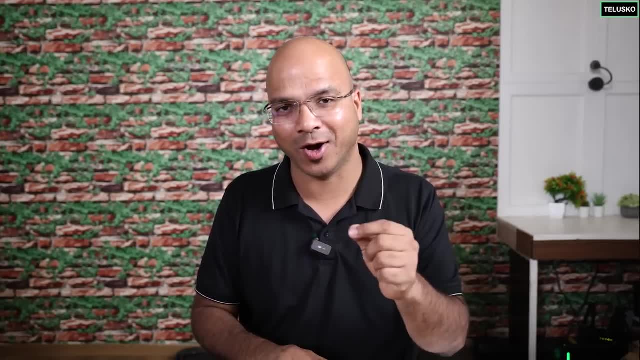 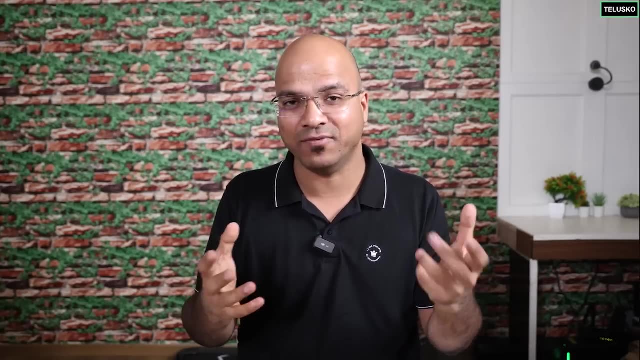 the more theoretical concept you know, it will be easier for you to work on the Git software, right? So basically, Git is a distributed, which means you will have a local copy. Of course you can have a remote copy as well. There are a lot of options available. Example: let's say if you want to work on your remote repositories, So you will have a copy there. plus you will have a copy on your local machine as well. So let's say, someday if you want to work in a long flight and you don't have internet access, you can still work on your project because you have everything. 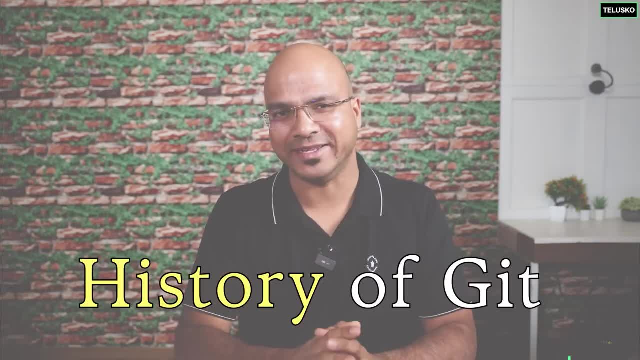 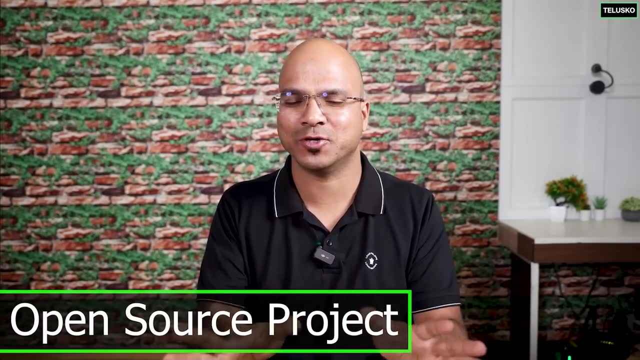 in your own machine. So let's understand the history of Git Now. it is interesting. That's why we have this special video for it. The thing is, if we talk about any open source project, So what happens in open source project is we have multiple people working on the same project. but you will say 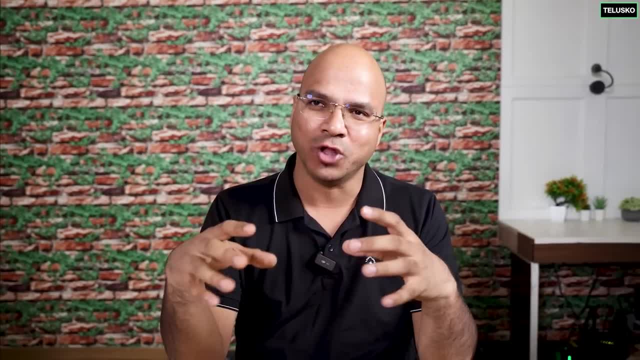 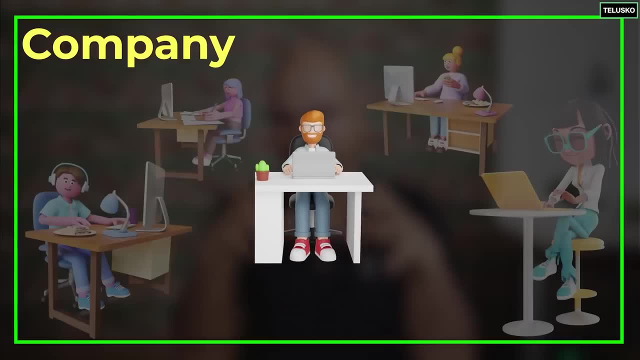 hey, that also happens with the normal projects, right? The thing is, in normal projects we have limited set of people. Let's say, if you are working for a company and you are building a project, you have, let's say, a set of people in a team. They will be working on it. 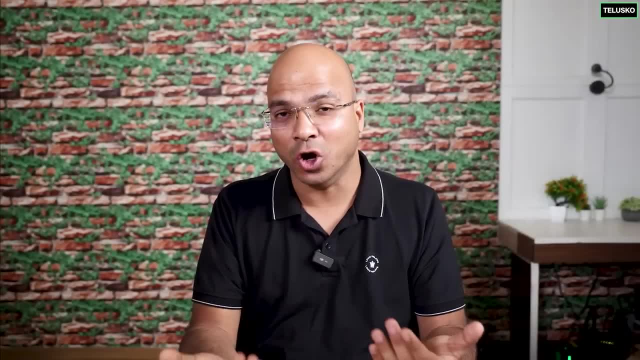 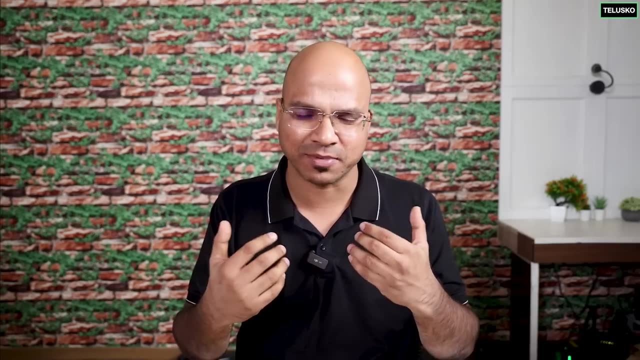 and then you trust everyone because they are a part of a project. In the open source project, anyone can contribute. Let's say, one day I decided to be a part of one open source project. Of course it will take some time for me to understand the project and then, if I feel, 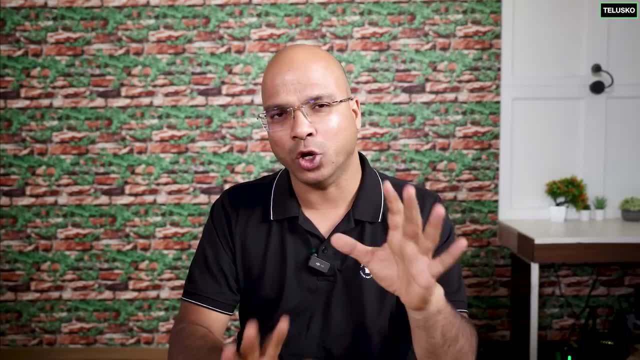 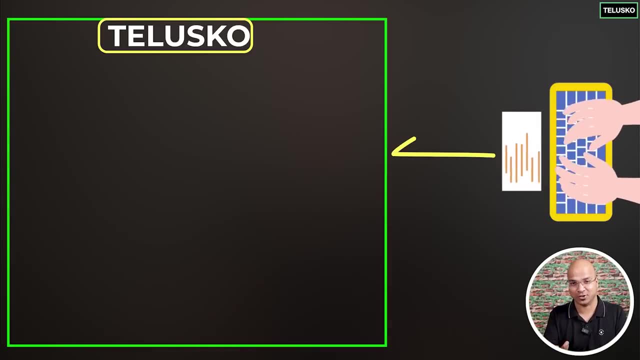 hey, you know everything is good in this particular project. So let's say it's any OS. Let's say we have this own Telisco OS and then one day I want to contribute to that particular OS, I want to add a new feature of, let's say, a Bluetooth connectivity, Just for an example. 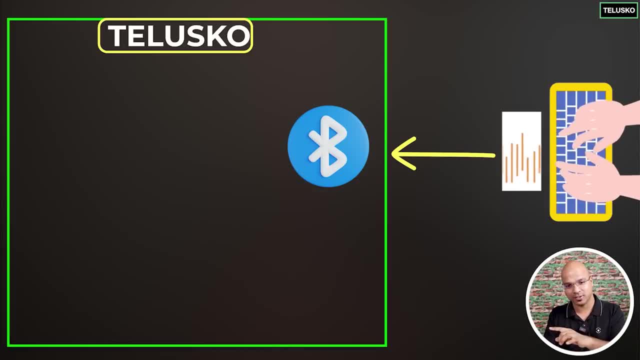 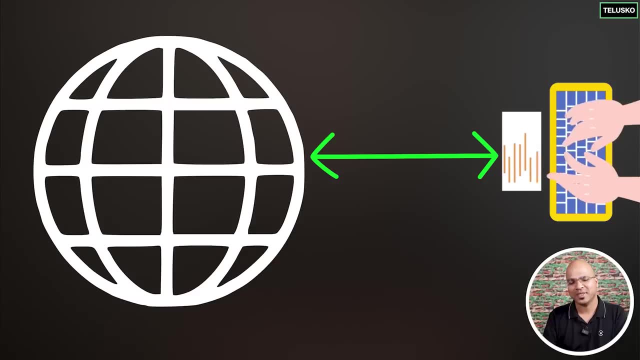 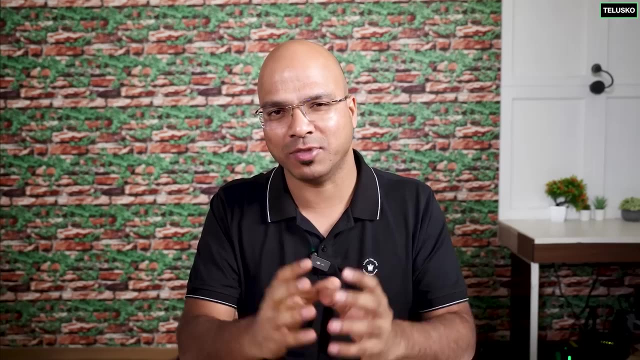 I can write my own module and add that in the OS in my machine. But if I want the entire world to use it, I have to send them the new code. right, But then how this thing will work, How multiple people in the world can contribute to one project. In the earlier days we used to do something. 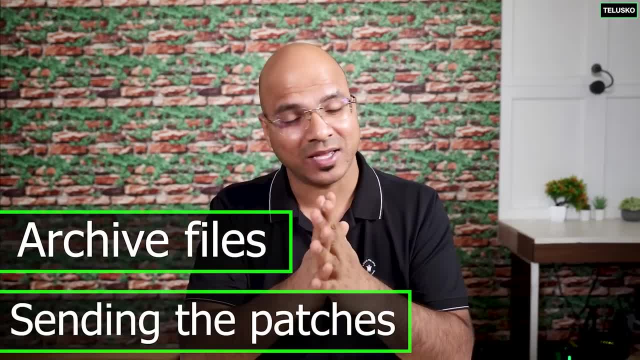 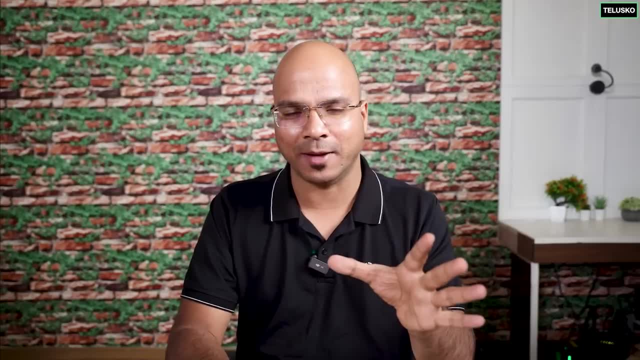 called archive files or sending the batches right Now. the same thing happened with Linux as well. Now, if you know Linux kernel- very famous one. the founder is Linus Torvald and he is very particular about how Linux should work. what are the features we should have Now? initial days were 1991 to 2002.. 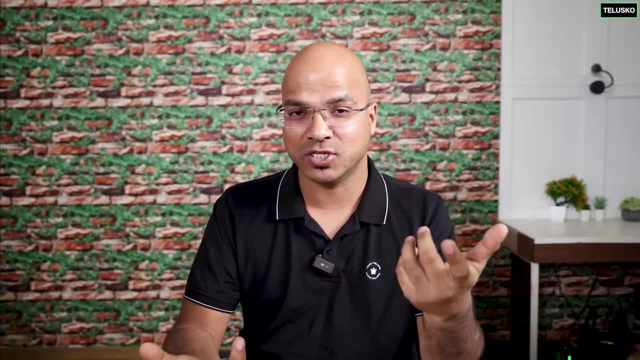 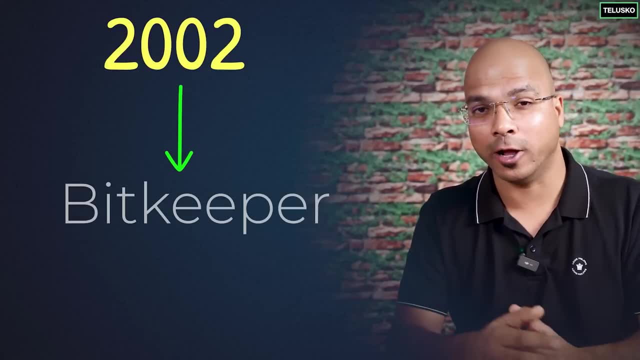 It was more about: if you want to provide the features, you can send patches or you can use archive files. But then, in 2002, they started using some proprietary tool called BitKeeper. Now BitKeeper, I think, was free at that point, and then they started using 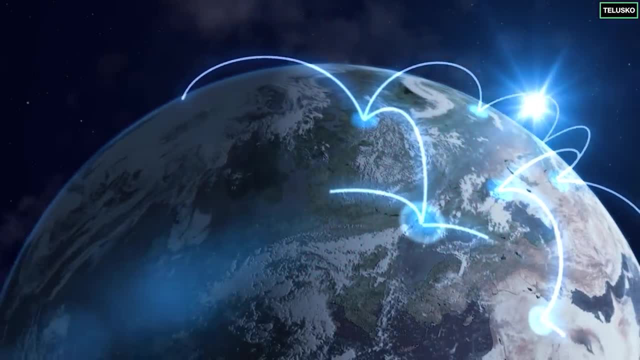 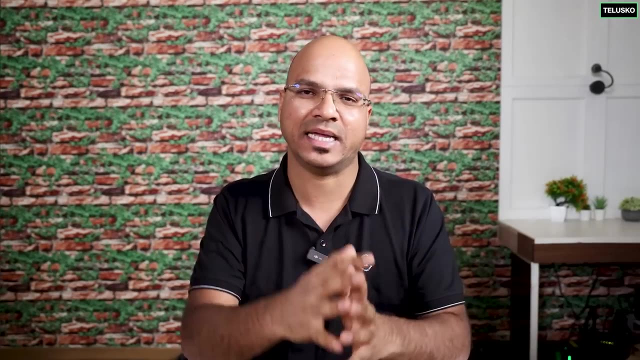 BitKeeper so that they can get the contribution from the world easily. now They don't have to go through a manual process of doing that, So they can simply use BitKeeper and they can send their code, and then they can do the merging as well. Now the problem is at one point. 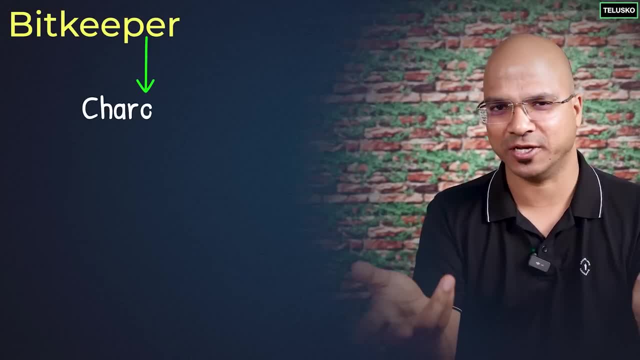 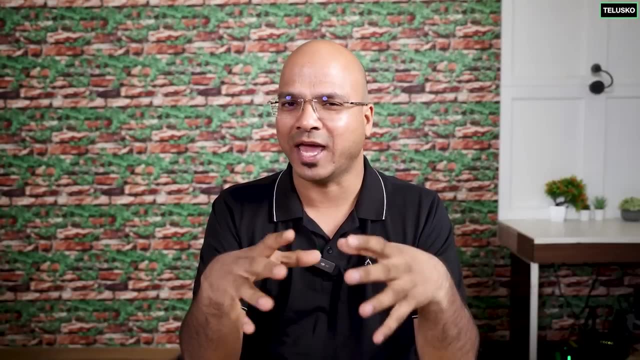 the policy of BitKeeper changed and they started charging. Now the Linux community was doing it for free, and then the entire world was using Linux for free, So they thought it's a good time now to move away from BitKeeper, and that's where Git was. 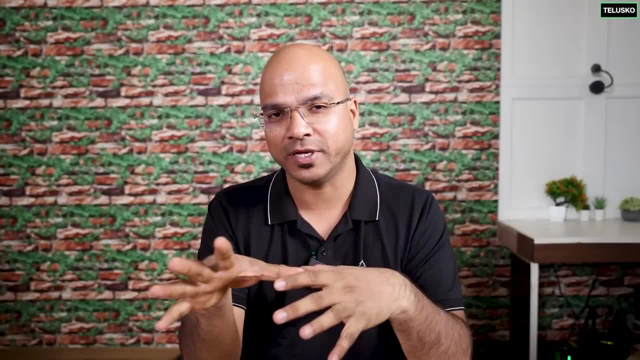 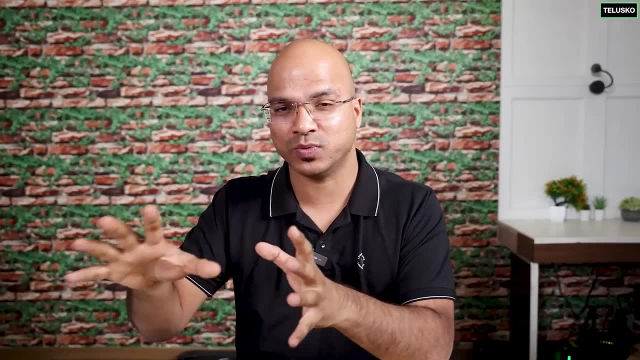 formed. Of course, they tried to make it very different from BitKeeper. So BitKeeper was working a different way and Git worked in a different way. Again, what is that different way that we understand once we start the actual implementation? But that's how, in 2005,, Git started. It's not like. 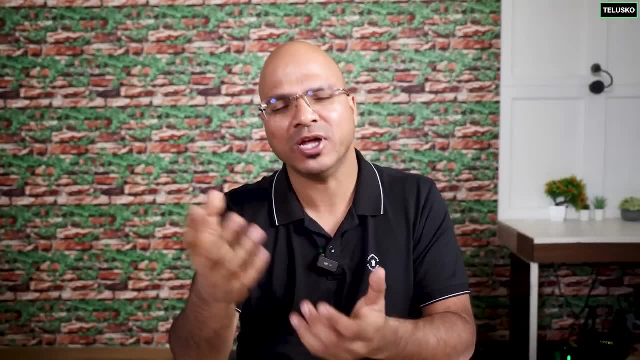 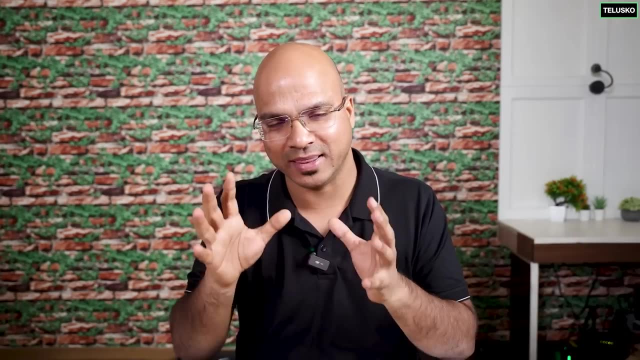 someone thought, hey, let's do this version control system. No, they were using something else. It's just that, because of some issue between the BitKeeper and the community, they moved away from it and they started using Git, As I mentioned before. 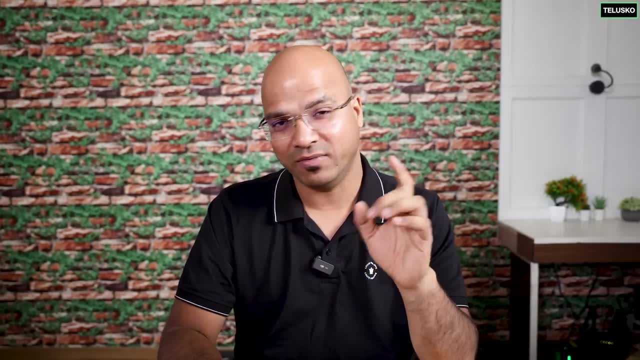 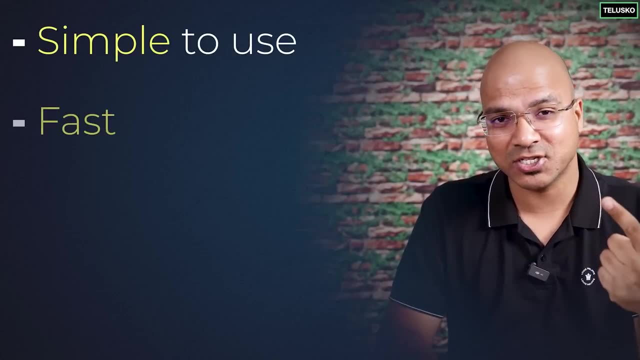 Git is different from all different version control systems, right Even different from BitKeeper, And since it is different, it has given some amazing features. It is very simple to use, It is fast. It also allows you something called branching, Again once we move towards the 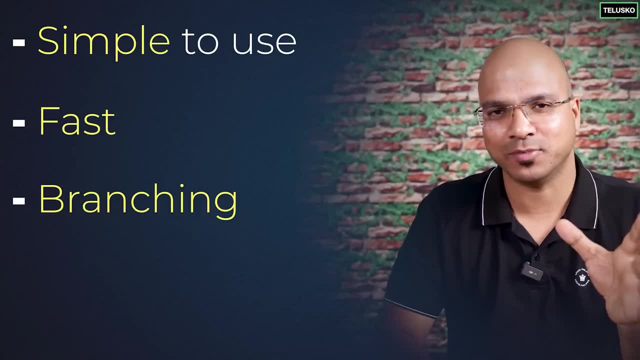 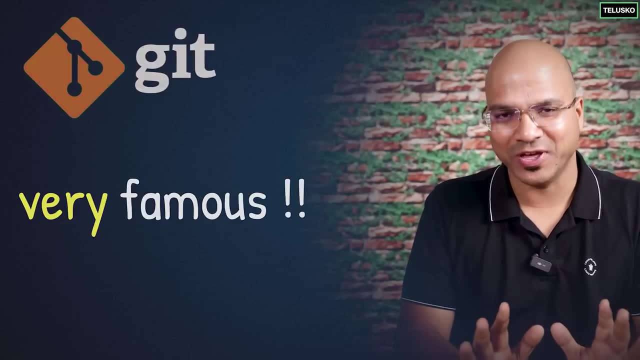 advanced part of Git, we'll understand what branching means And it's a fun concept to learn and also to implement. And it is fully distributed, which makes Git very famous. And I know we have done enough build up. And the question is: how do we use Git? We want to 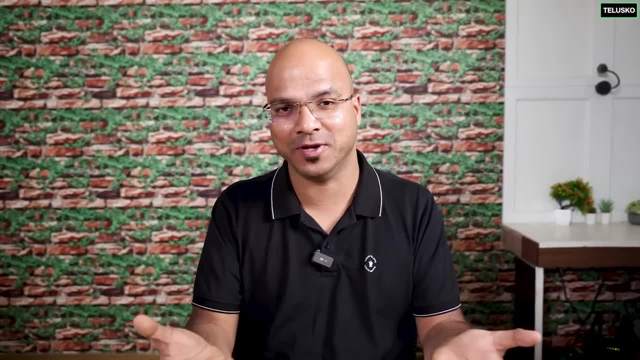 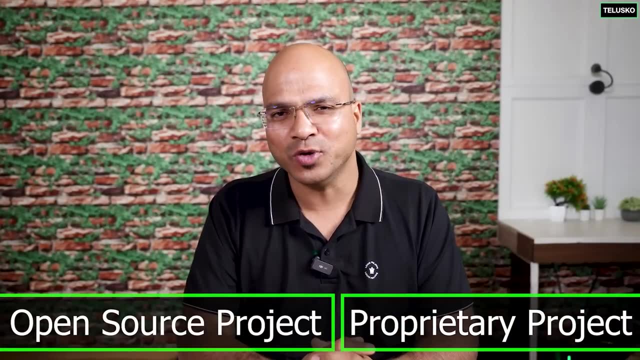 collaborate and we want to work with Git so that we can collaborate with different people and we can build a project. It doesn't matter if it's a proprietary project, you're working in a company or open source. How do we use it? And that we'll understand in the upcoming videos. 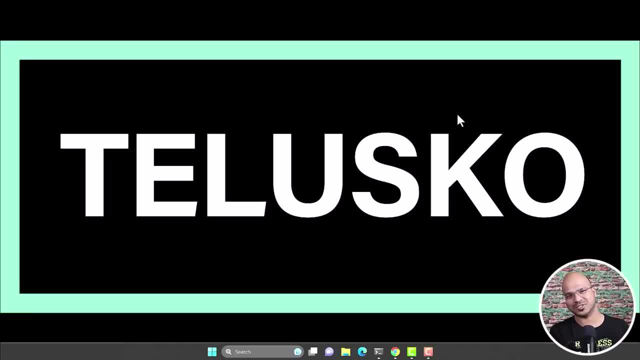 Now it's time to install Git. Of course we want to work with those commands And, as I mentioned before, if you want to master Git or if you want to use the features of Git, command line or basically, commands are the way to go. Now, how do you know that in your machine you have Git Now? 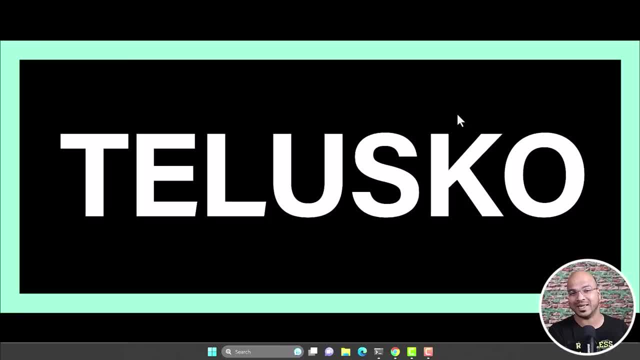 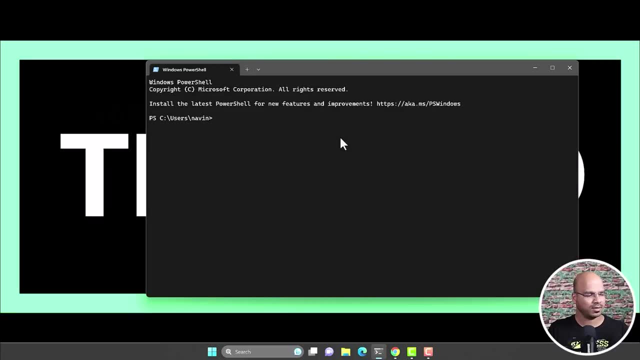 if you are using Mac. basically, in Mac, if you have installed Xcode, you will get Git by default. But if you are using Windows, you will not get that. So how do we verify? So it's very easy: You just have to use the command prompt. So I will open my command prompt here and PowerShell. 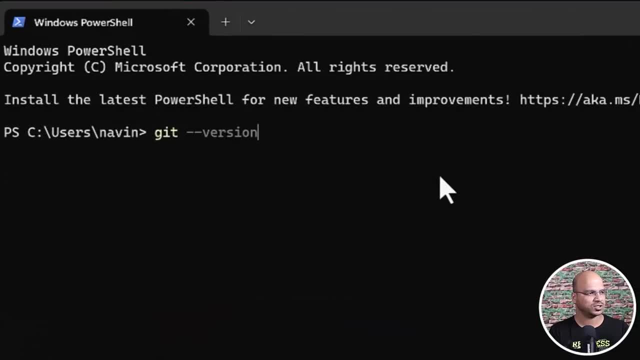 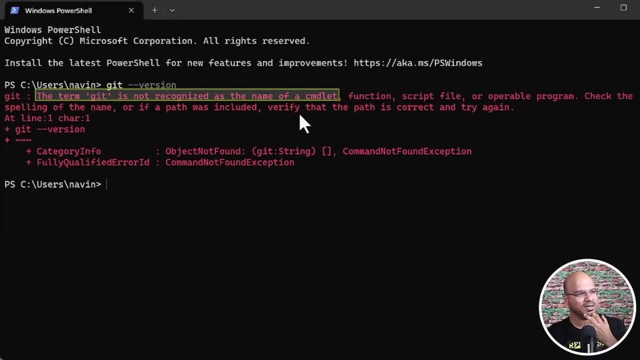 So what you can do is you can search for Git version. So basically, this is the command which you have to fire And when you say enter, you can say it says the term Git is not recognized as a command. Okay, If you want to get Git on your machine, if you're using this on command prompt. 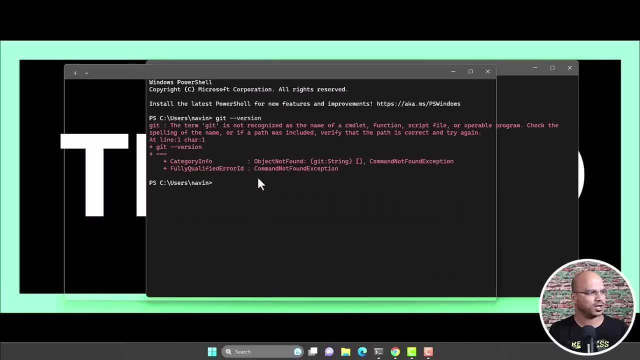 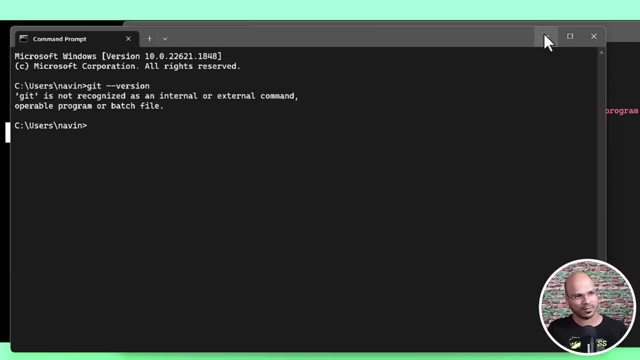 you will get a different message. Example: if you do that on command prompt and if you say Git version, this is the message you will see. So it doesn't matter which window you're using- PowerShell or command prompt, both works, But in both of the cases we don't have Git. 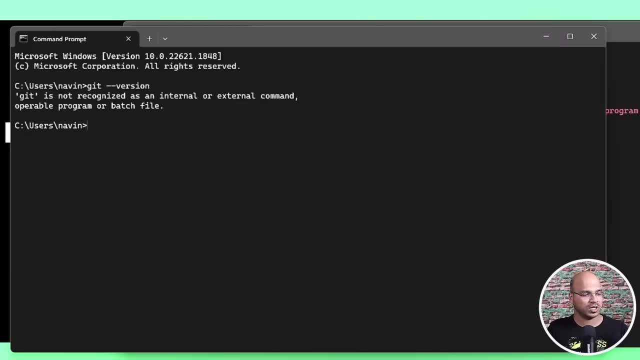 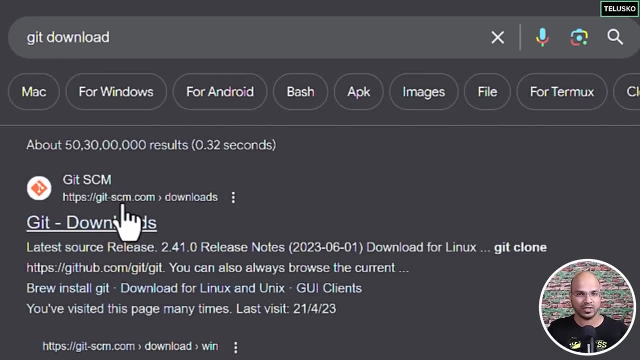 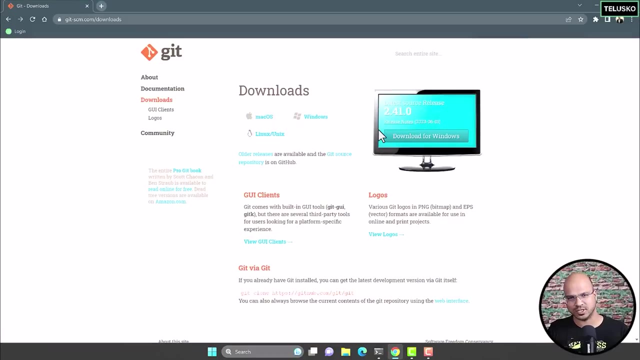 Now, how will you get Git? It's very simple. You can just go to the website, or you can just go to Google and search for Git download. Now this is the website from where you can download the Git. The current version of Git is 2.41.. So we can get that one And it will ask you for which OS you're. 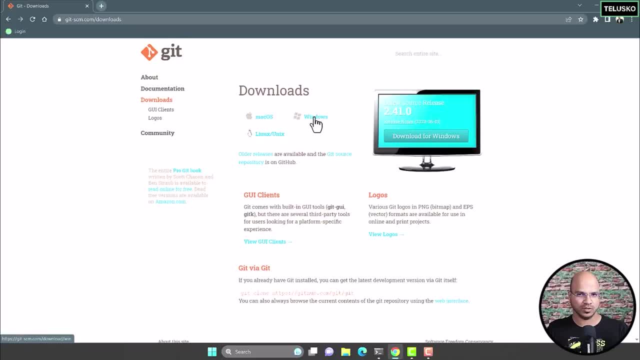 using. Now, since I'm using Windows here, we can click on Windows. If you're using Mac, you can go for that And, as I mentioned before, if you already have Xcode installed, most of the time, for some reasons, you install Xcode even if you don't develop iOS application. So do check if you. 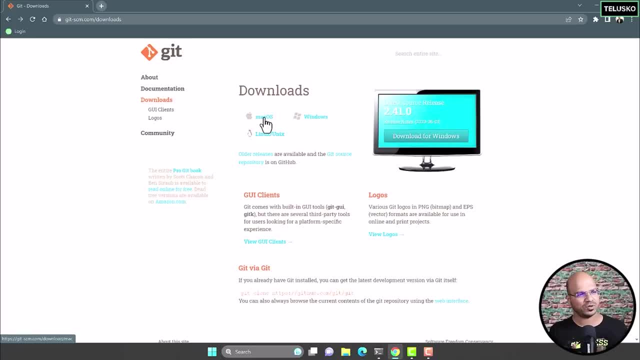 already have Git by saying Git, hyphen, hyphen, version. If you don't have it, you can follow the similar steps. You can click on download there and you will get it for Mac. So that's it, Thank you. For Linux, you have to set the path and that should be simple. So let's go for Windows here. 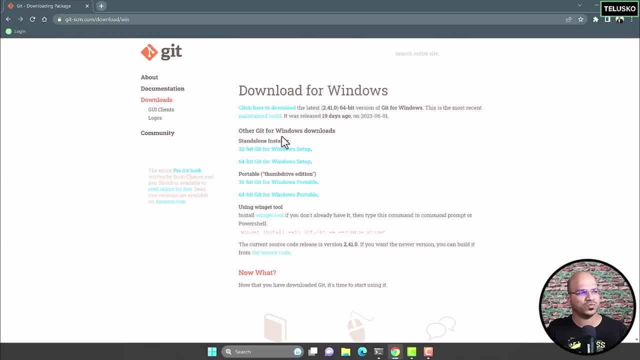 And once you click on that it will ask you for which version. So, basically, you can go for a standalone installer, which is suitable for if you have only one machine. But, let's say, if you want to move between different machines, you can go for portable one, But I prefer to go for a. 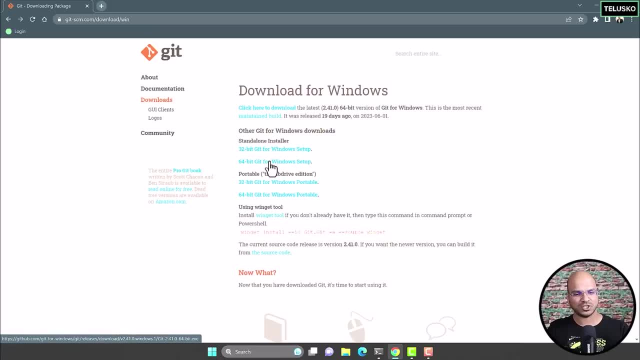 setup inside the machine and 64 bit, because my machine is 64 bit, So I will click on that. So I will click on that And once you click on that, it will ask you for which version you have. And once you click on that, it will ask you for which version you have. And once you click on that, 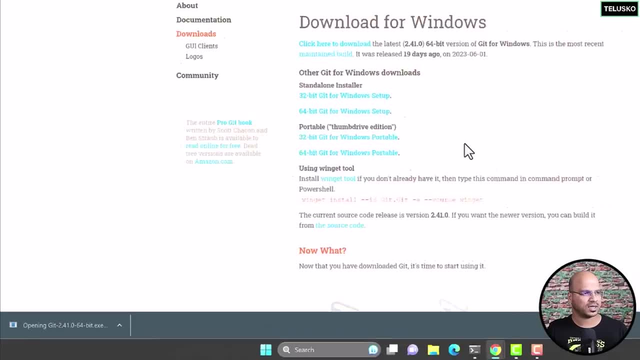 it will ask you for which version you have. Now, once you've got this download, it's very easy to do the setup. You will say click. So, given a prompt, click on yes, Okay, And we don't have a choice right, We have to accept the agreement. 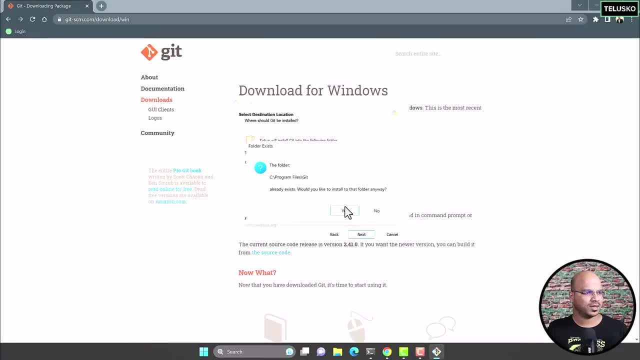 Now this is a place where you will install Git. I will say next: Okay, It says I already have Git in my machine because I think I already installed it before. But I will say: okay, I'll go with that particular folder, That's fine with me. Now it also gives you. 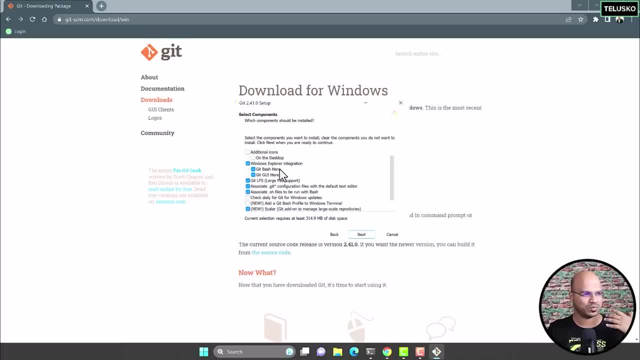 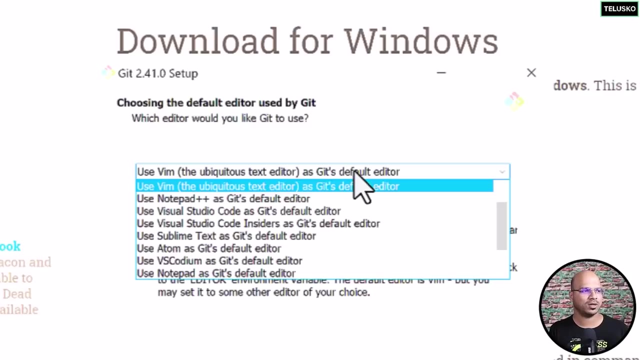 something called Git Bash. Now, at this point we'll not be working with Git Bash, We'll be using normal CMD And anything else Looks good, Click on next Okay. Click on next Okay. So it will give you certain options, You know, when you want to edit something and get which particular IDE which. 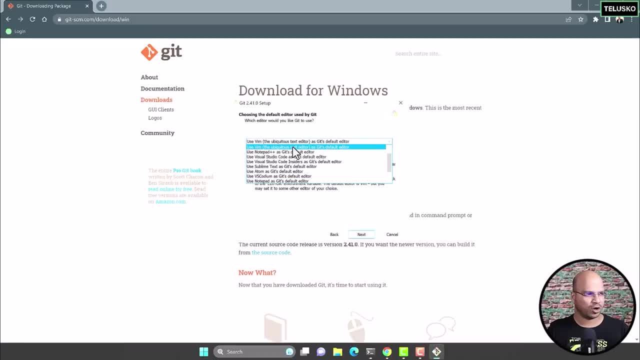 you want to use, or note editor which you want to use. Now I will go for default one, which is Vim, or you can choose whatever you want. Maybe let's choose Notepad for this particular series. I don't want to confuse you with how to use Vim. 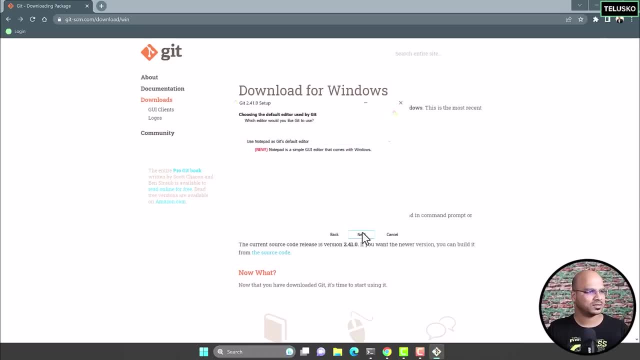 so let's use Notepad here and click on next. Now, this is something important to remember. Now, when you work with the first command of Git, it creates something called branches. Okay, So we have this amazing feature of branch in Git. Now, by default, you will get one branch, which 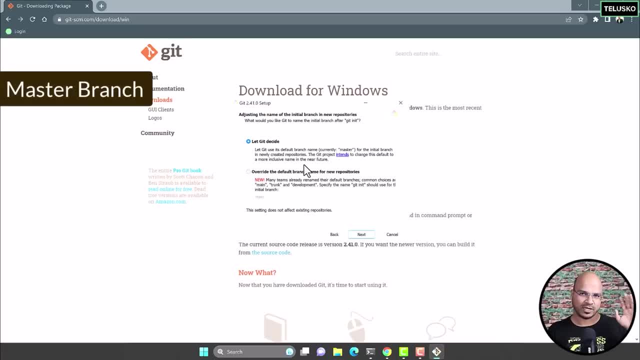 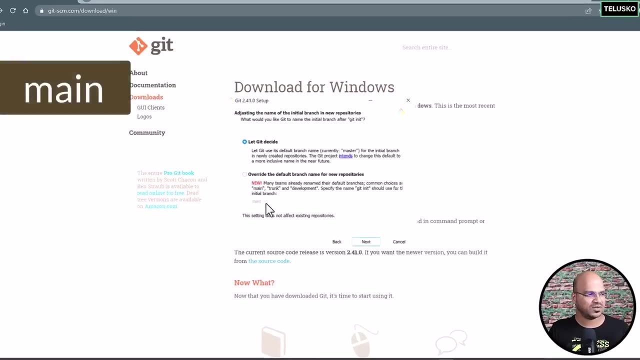 you work with and they call master branch. Now, when Git came into existence, way back, the name was master, But recently again it doesn't look good, right, Master slave. So they went for a normal word which you can use. So we got main. So, if you can see, 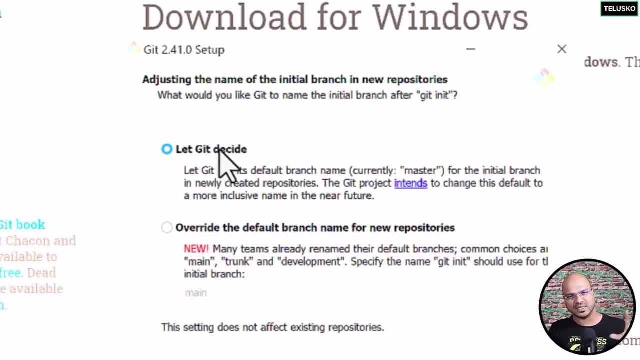 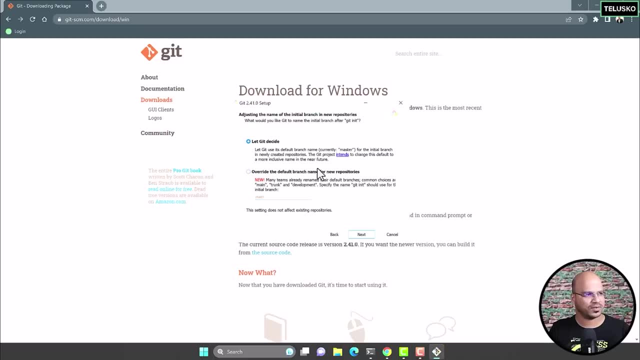 we have an option of main here. So I will go for let Git decide, and when we are creating the project we'll make it main. We'll not be using master, Otherwise you can change it from here as well. That perfectly works. I will say: let Git decide Next, And here you can see I'm going to. 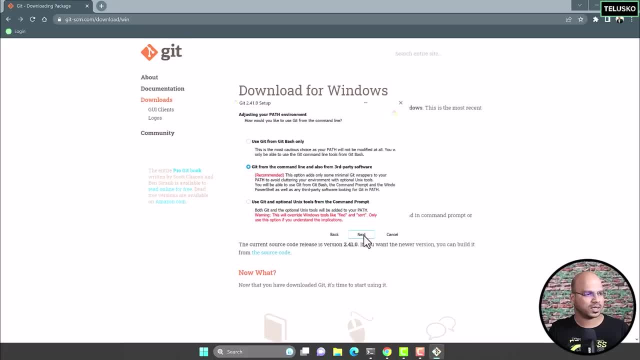 use command line, not Git bash, So I will go with that and click on next. Okay, I will use open SSH and open SSL, So nothing to change much. I will let you know when you have to change the basic. 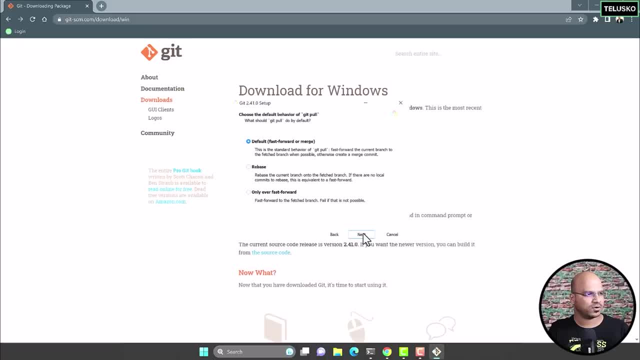 configuration, Fast forward and merge, Yeah, Okay. So when you say Git pull, this is what you do: select, I will say okay, And next Enable system caching required. Now it provides you some experimental features. We'll not be checking at this point. We'll click on install, Okay So. 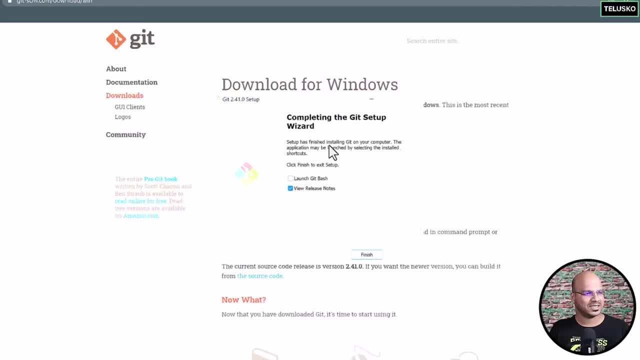 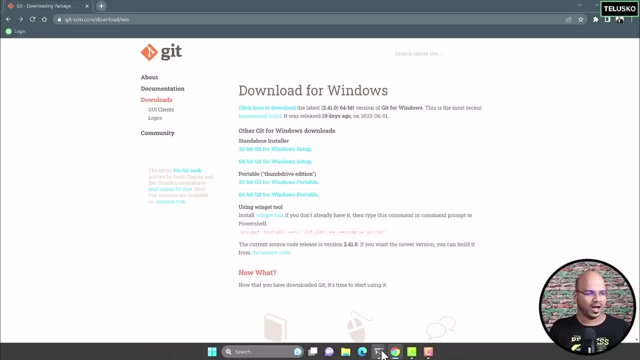 it will take some time to installation. Let's wait For it. Okay, As you can see, it is installed. I don't want to see release notes. I will click on finish And done. We got the Git setup Now. how do we verify? Of course, when you open your 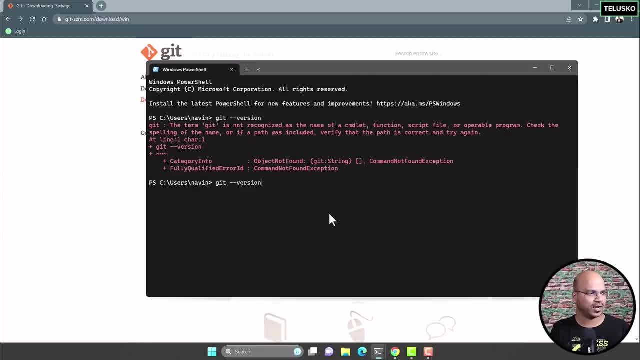 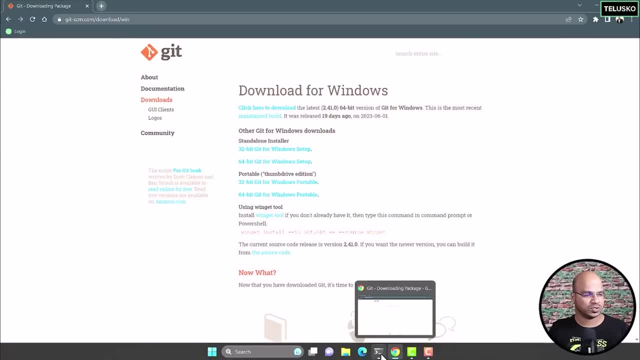 command prompt or PowerShell, let's say here. if I try to do that once again, you can see it still says Git is not a recognized command. The thing is, after installing Git you just need to restart your command prompt And I will again open my PowerShell, Of course. 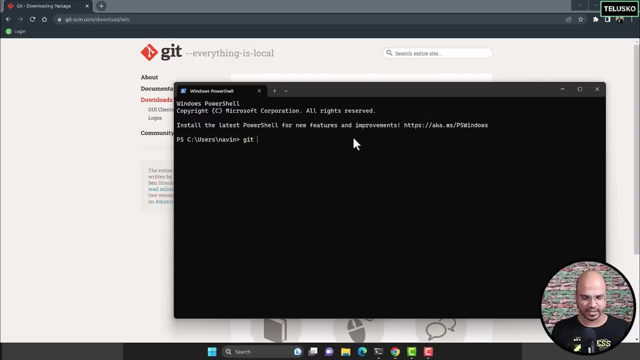 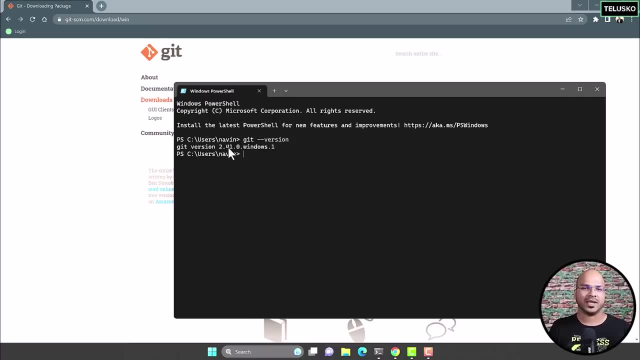 you can search for PowerShell from here And you can search for Git version And you can see we got the Git version. So now Git is properly installed. Okay, Now, once we got the Git installation, now it's there, It's in your machine. But how do you? 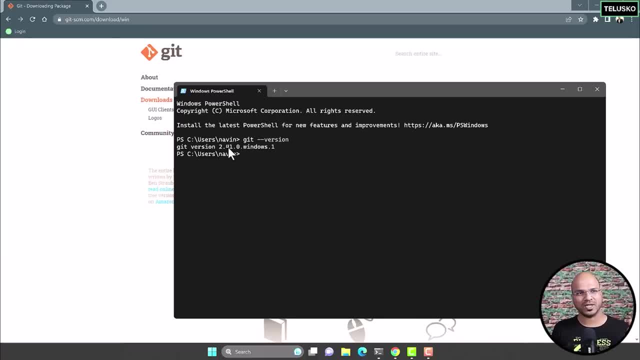 make it your own. Every time you do Git commit. every time you want to push something, you need to have your own identity. Of course, we need to know who's pushing the code, Because in Git we have multiple people working together on the same project, So whenever someone pushes the 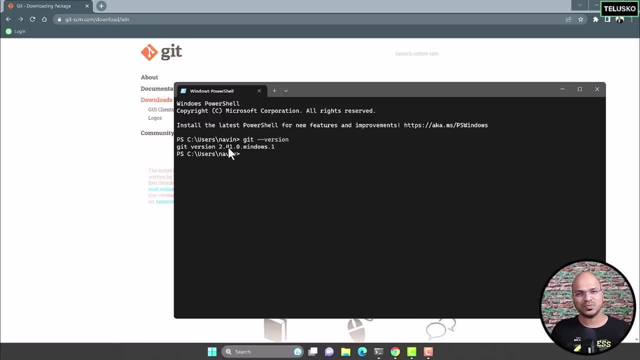 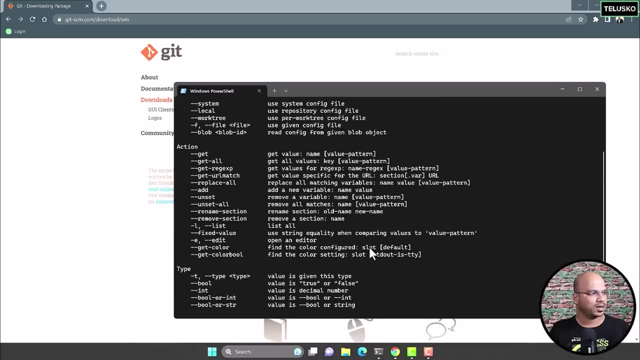 code on the server. you should know who is doing it And that's where you need to have your own configuration. the way you can check that is by saying get config, and when you say enter, okay, you can see, it will give you certain things. now, basically, in get config, there are certain things. 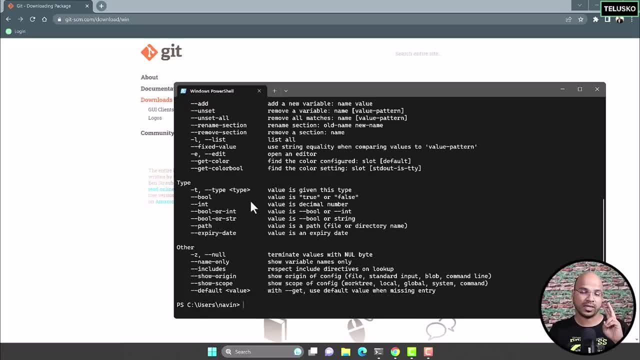 which are to mention at least two things: one is your name, your username, and second is your email. with the same email, if you're using a public repository, let's say git lab or github, you'll be having a public account right with the email id, so you have to use the same thing. so if you 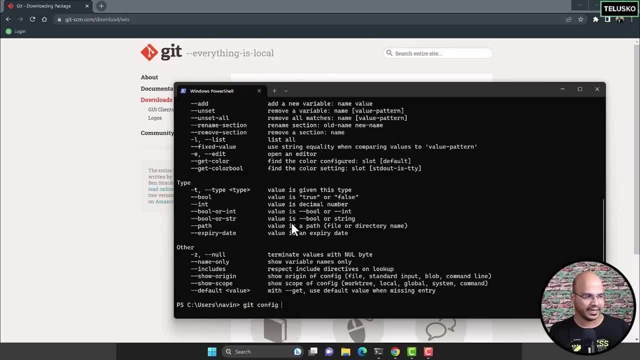 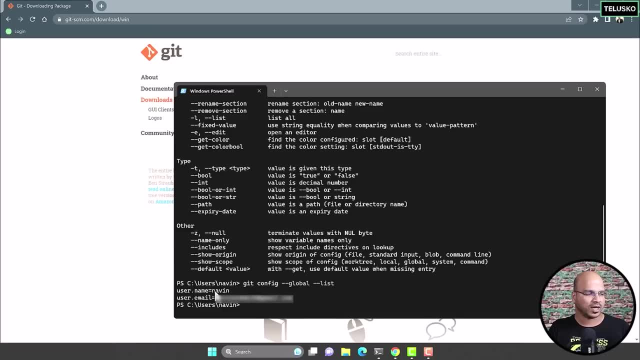 want to know what are the existing variables we have. so what you can do is you can say: get config, i want the global values and i want the list of values when you say enter. okay. so the thing is in my machine already have this configured, okay. so this is not the first time i'm using git. 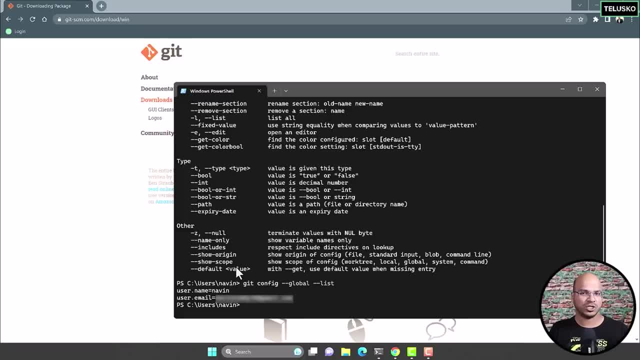 so i have these values, but in your machine you'll not be having this value, so let's do the setup. how do we set the values here now, since i'm using my personal email, so that's why it is blurred because of the privacy issue. but yeah, so you can use your own email id there. so how do you set a? 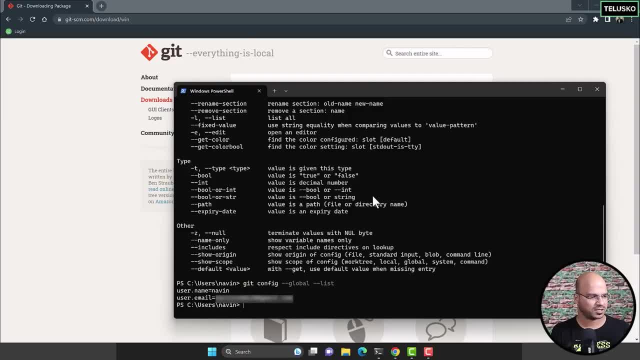 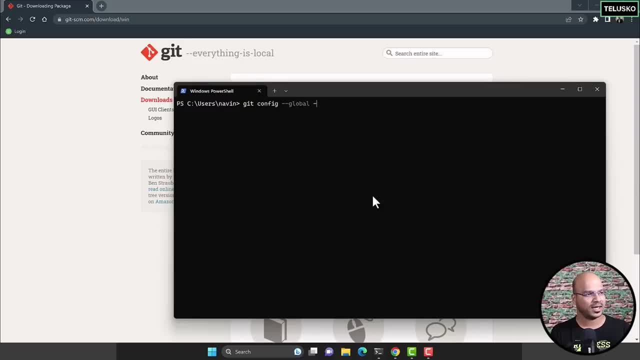 value. it's very simple. you can say git config. so let me just clear the screen once. so if you want to configure, you have to say git config, and then you have to say global, because you want to set it globally, and then you need to mention user dot name and whatever value you have. so let's say i want to set navin here, enter. so 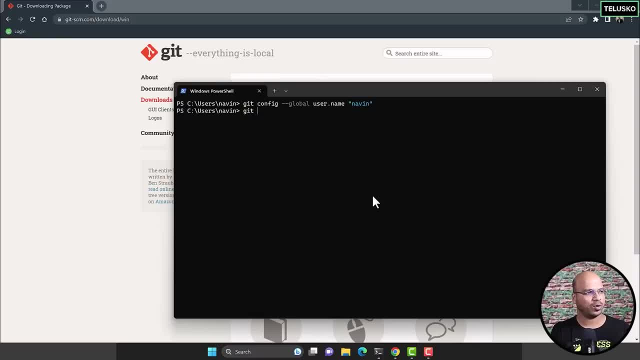 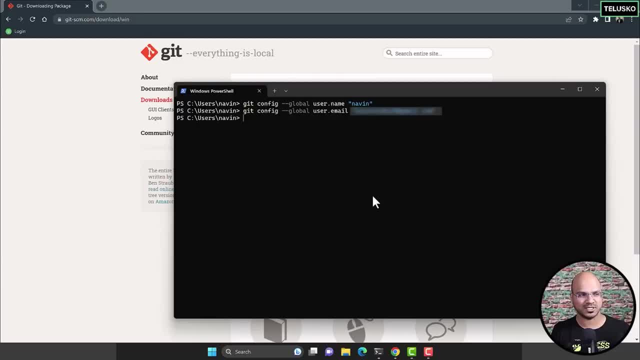 and again for privacy issue, it is blurred. i will say enter and values have been set. now, if you can check the same command, uh, you will get your details there. so that's how, basically, you can make this. get your own. now, how do you create your first project? as i mentioned before, there's not 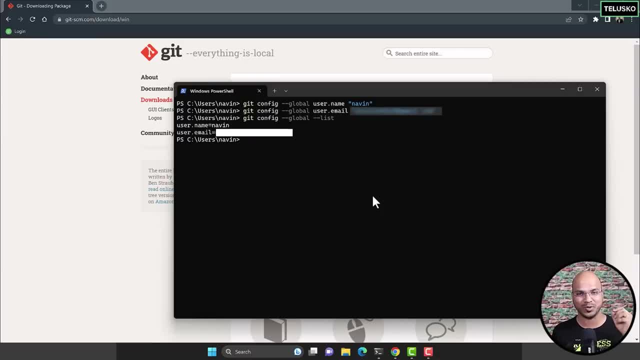 just for coding. you can use git for any purpose. the moment you want to create something with people or maybe, if you want to create something, maybe you want to write a book, maybe you want to write poetries or essays- you can use git there and you can maintain the version of your project. so that's. 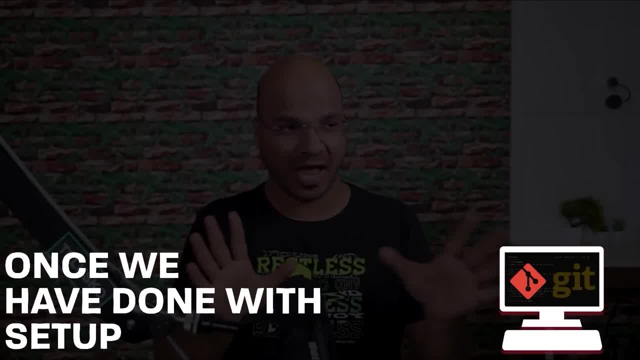 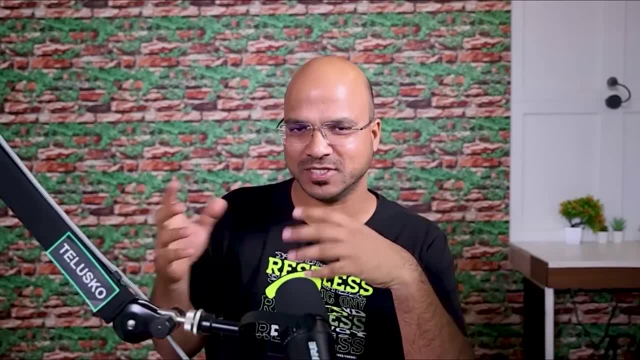 your stories. so once we have done with this setup- so now we have given you know machine right- let's try to use git. now the thing is normally, as a programmer, we use git for different languages. example: let's say, if i'm making a project in java, i can use git to create different versions of it. 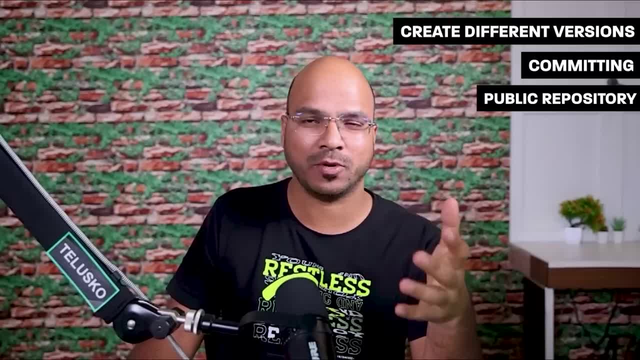 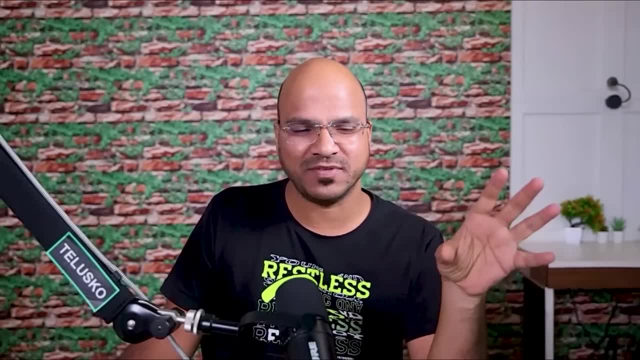 and i will be committing it. i will also push that on some free public repository. and then in the world we don't have just one programming language, right, we have so many programming languages. now. if i go with any specific language here, of course it will create trouble for others. 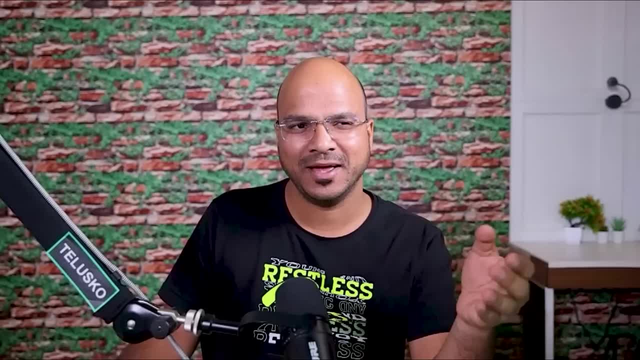 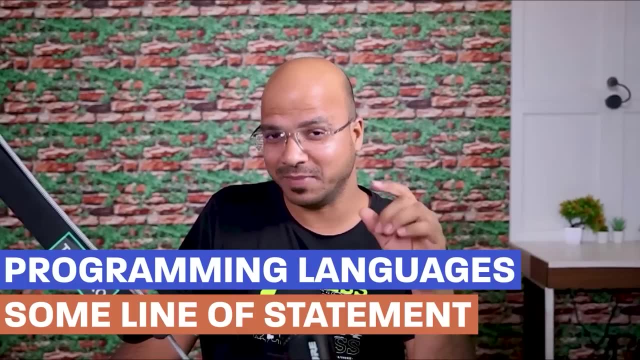 people. let's say, if someone is doing into javascript or python, they will not feel comfortable with java. right, and the beauty is, doesn't matter if you're writing a programming language or a essay, some lines of statement, english statements, it's all same for git it's. 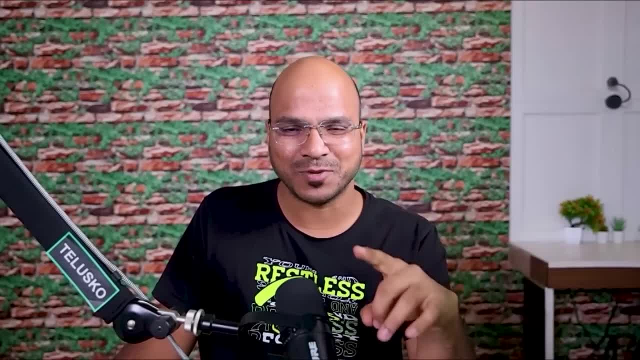 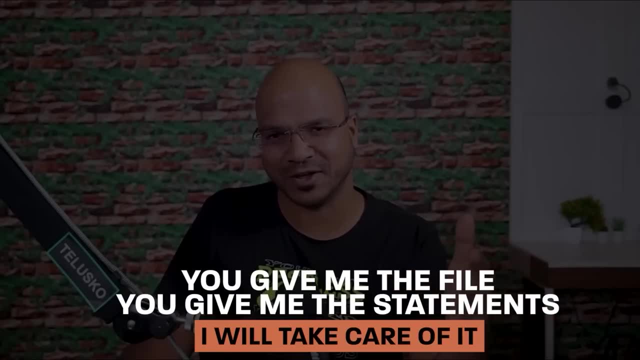 not, like git, recognize the programming language and say, hey, i for this programming language, i will work in this way. no, that's not how git works. git basically says: you give me the file, you give me the statements, i will take care of it. so git will not look for the code, right? so in this, 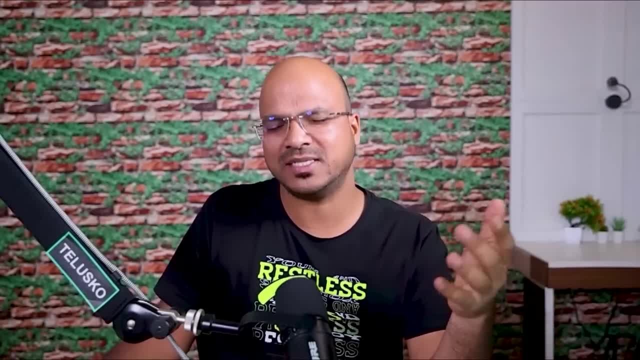 particular course. we're not going to focus on the code. we're not going to focus on the code. we're going to focus on any programming language. let's say we are writing a code in multiple files. it doesn't matter the language, so it's important for us to understand how do you store that file. 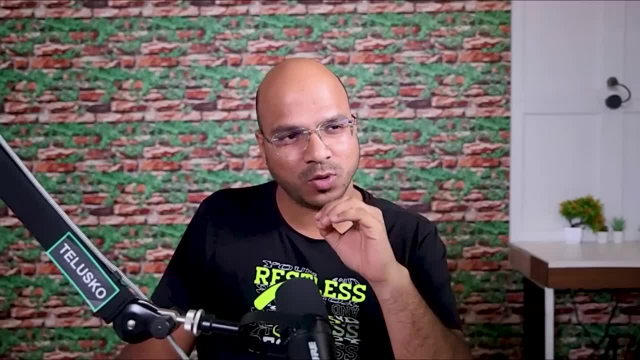 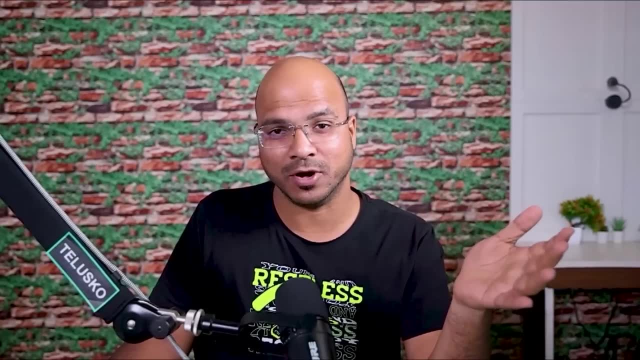 with git. how do you work with git to merge different files? so, whatever lines i write, it will be normal english, maybe a pseudo code for that matter, but this can be used by anyone, even if you're writing a book or if you're writing a script for a video. okay, so let's get started. so. 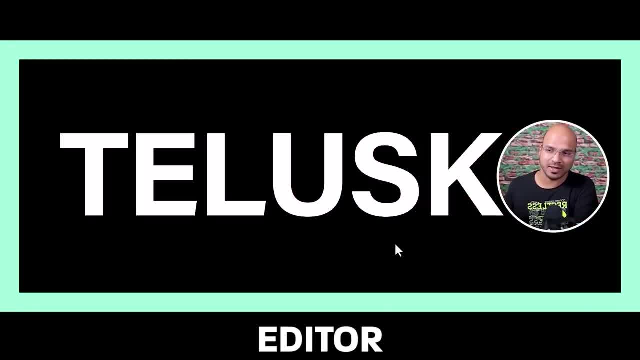 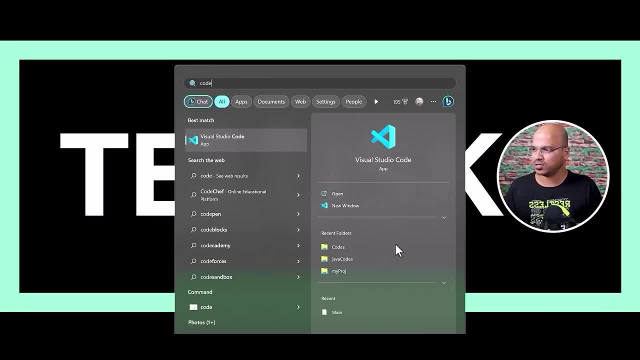 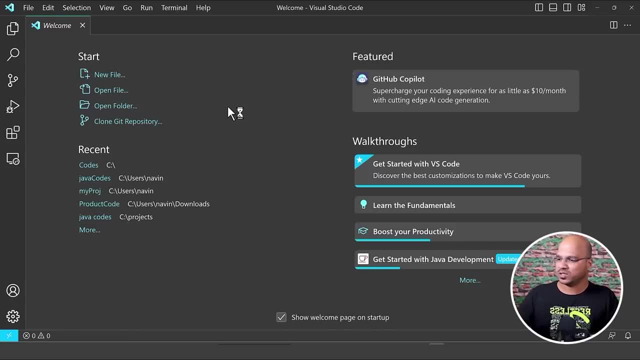 what i will do is, first of all, if you want to type something, you need a editor right now in this. so in my machine i already have vs code installed, so let me open that. so i got my vs code open here and i will just reduce the size of a bit. yeah, okay, so this is. 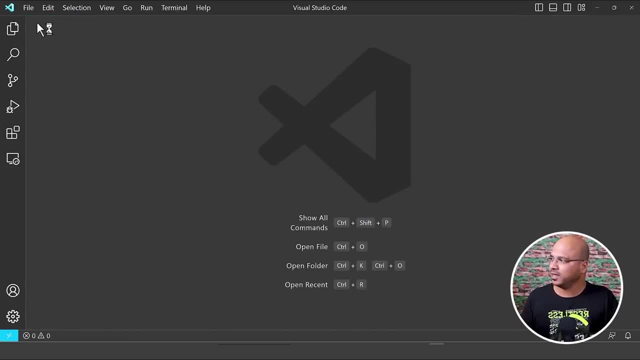 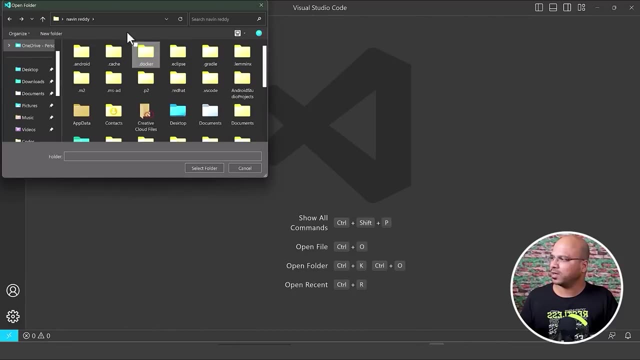 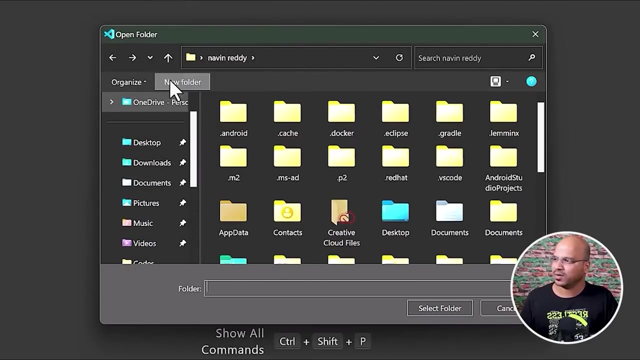 my vs code- you can use any id for that matter- and then in this, i will just open a folder. so this is where i will be working. i will be working in general. so let me open a folder and let me create this folder inside my user, which is naveen in this case, and i will create this. 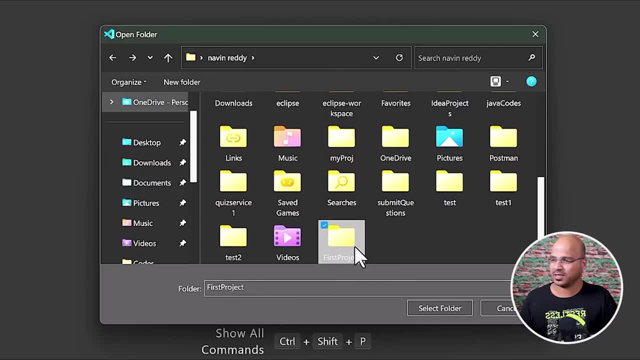 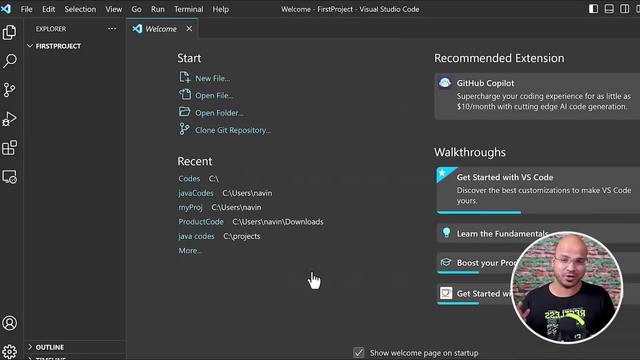 folder as first project. of course this can be anything, but let's say first project and opening it now, imagine this as your working directory. so what is working directory? example: it doesn't matter if you're writing a book or writing a code, you will put that in a folder. this is what your folder is. 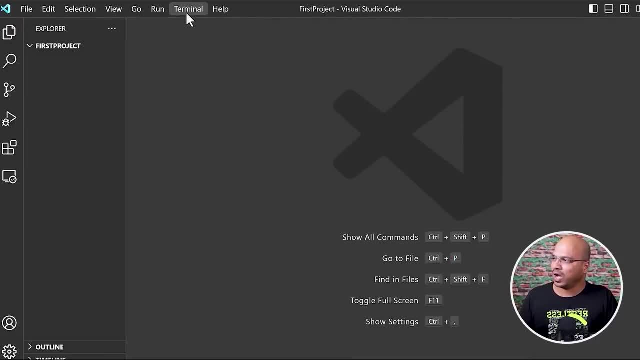 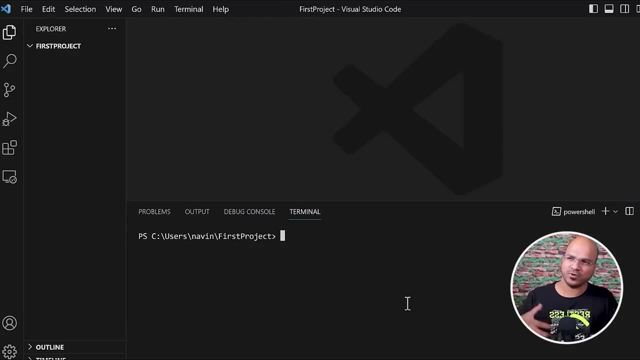 so you can say: this is your working directory, right, and now i will open a terminal. now, as i mentioned before, we need to do everything on a terminal, right? so if you're using vs code, you get a terminal inbuilt, or if you're using some other ide or some other editors, let's say notepad. 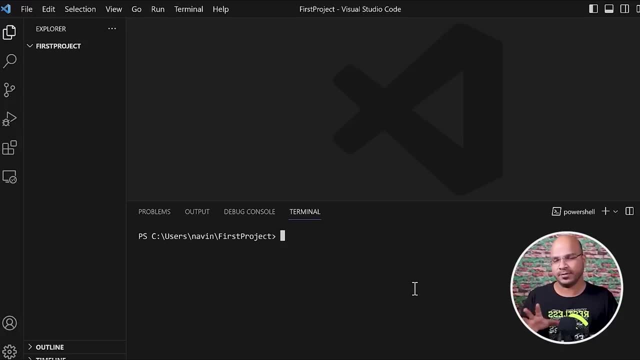 in that case, you will be using your command prompt right now. whatever we did before, we did that on a command prompt. here we are using a internal command prompt of vs code. we call them as terminal. here again, same thing, different terminology. in fact, you can also select: do you want to work with powershell or do you want to work with any? 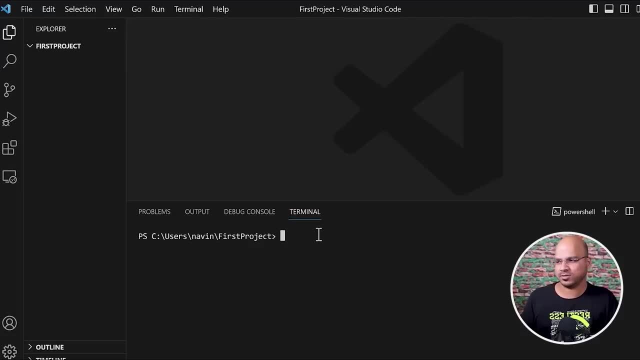 other thing. so in this case, when i say terminal, it is by default using powershell, so that's fine. we have tested this on powershell. it was working, so let's continue with it. basically, if you want to understand git, you have to understand different areas in which git works. now basically for git, or. 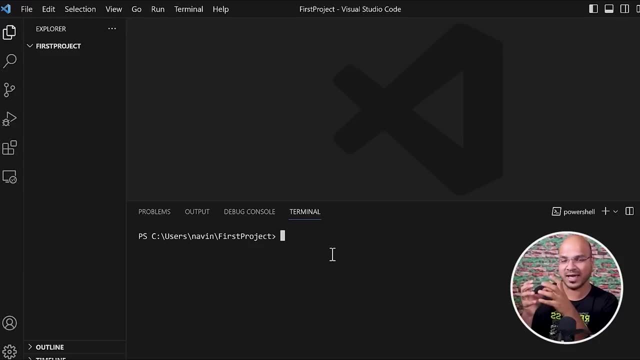 this is your project, right, so you can imagine this first project as your folder. now, whatever you do inside this, git has no idea what you're doing. okay, you have to let git know that. hey, you know, i want to track my progress, i want to commit, i want to create different versions, right, and to? 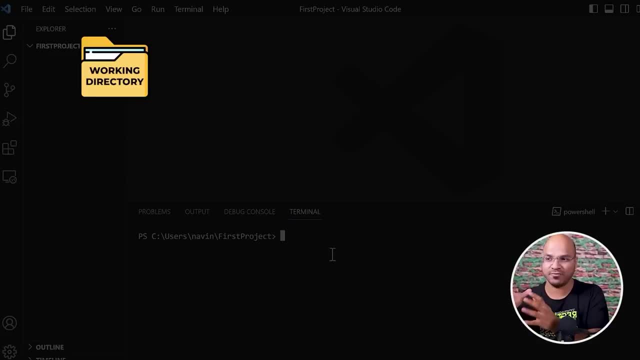 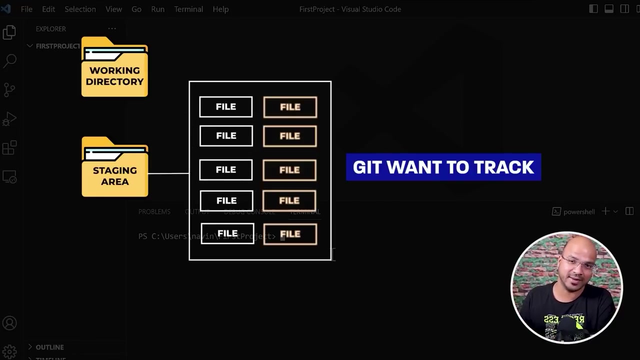 tell that to git. you have to do something. now, basically, apart from your working directory, we have something called a staging area. now, staging area is a place where git knows: okay, in your project you have, let's say, 10 files. out of 10 files, you have five files which you want git to track. now how will you tell that? and 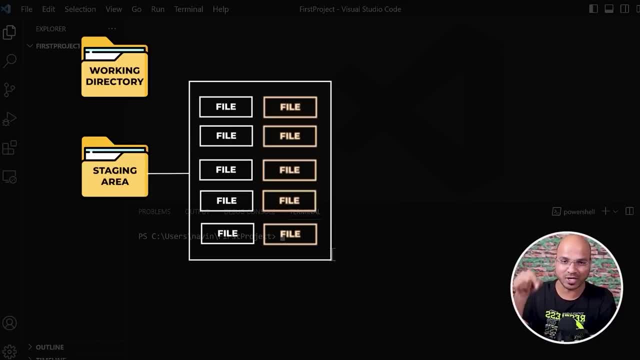 that's where staging area comes into picture. you have to tell git: hey, whatever is there in the staging area, please take care of it. other files- you can ignore that, okay. so staging area becomes important because that's where git works. apart from that, we have something called a commit. 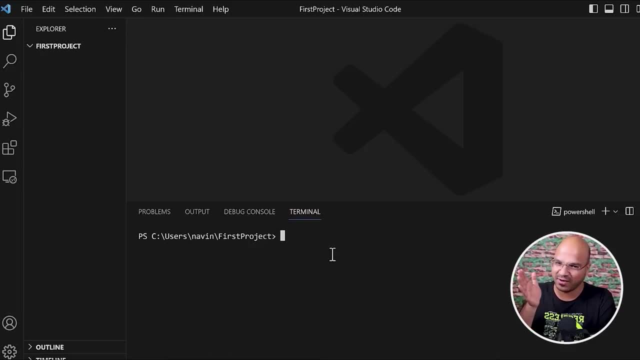 history. as i mentioned before, you can create different versions. right, and every time you commit you create one version, basically, and the beauty is you can go back. of course, i will show you how to do that in a minute, but, as i mentioned before, you have to create different versions. 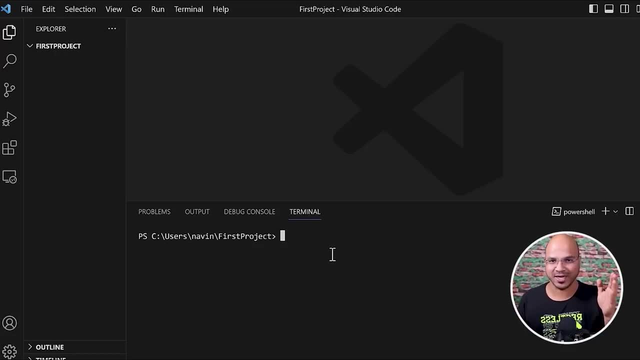 and then you have to figure out how to use those things. but these areas are important. so you are working with this directory and whatever you do in this directory, git has no idea. okay, and if you say, hey, git do something with this, git will say: what are you saying, bro? so, basically, git has no idea. 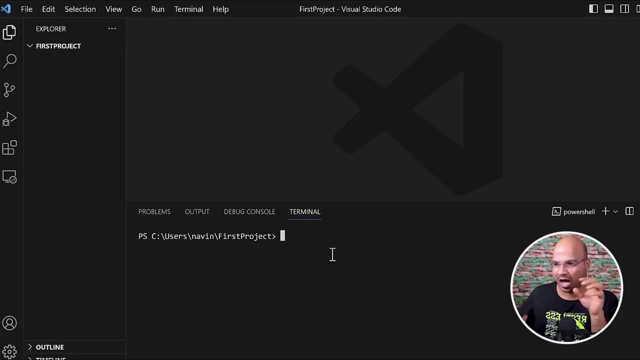 what you're doing. so you have to push that into a staging area. how will i do that? we'll see that later. and then one more area we have is the commit history. now, how exactly all this thing looks like, we'll see that later. but you have commit history where you have to do committing. now this too, which. part of a different box, which is your git. a lot of people do get confused between a working directory and a git repository. there are two different things. it's just that it looks similar. so they say, okay, this is my git repository. no, this is different from, uh, the git repository. this is your. 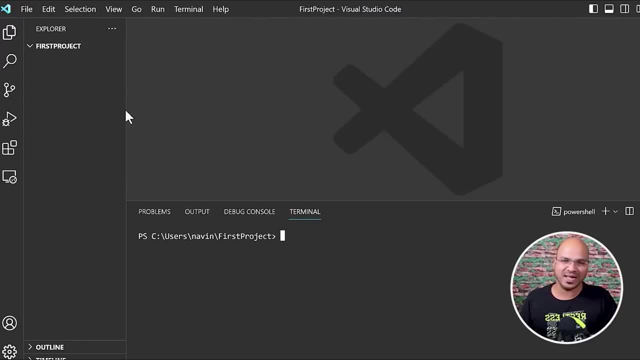 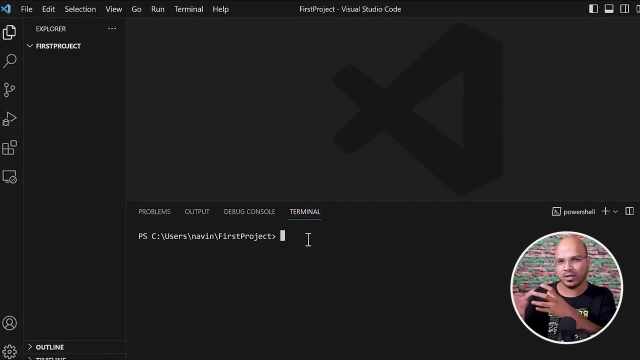 working directory. okay, so now what i will do is whatever files i have i will create here. they have, so git has no idea about it, right? so i need to create a local repository here. so when i say local, it means it's there in this machine. what if i want to share this with everyone else in the world, or 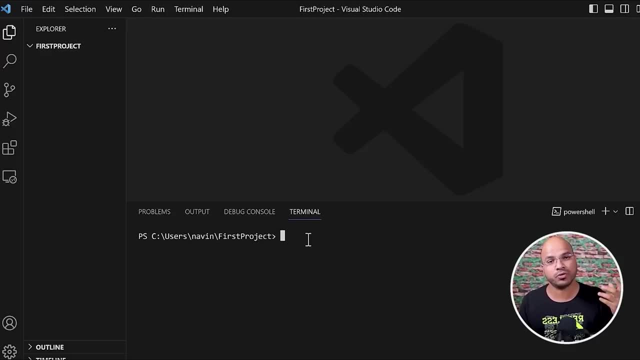 maybe with my, with my team. in that case, i will create a remote repository. this can be done with the help of git lab or bitbucket or github- your choice- but those are the options we have now here. we need to create a git repository or local repository. the way you can do that is very 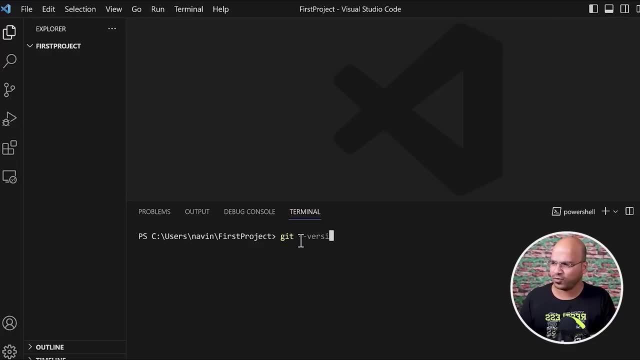 simple. you just have to use a command, git, as we are using. first of all, before we're going forward, i will say git version and you can say there's a version right now. if you want to create your git repository, local repository, you have to use something called init, okay. so once you do that, you, it will create a local repository in your 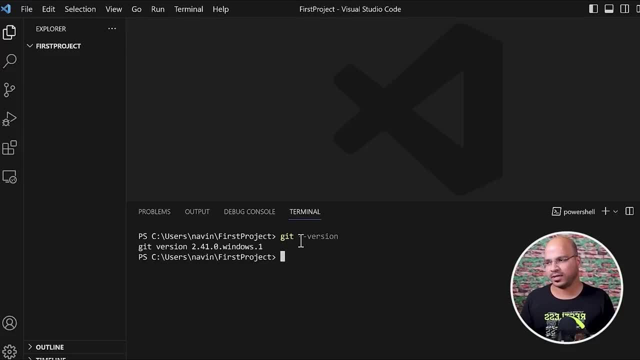 project. okay. so before going this, what i will do is i will use one more command- now. this command is very important, which is called git status, and we'll be using this multiple times. so every time you want to do something, you will use git status a lot. so when i say git status, it says: 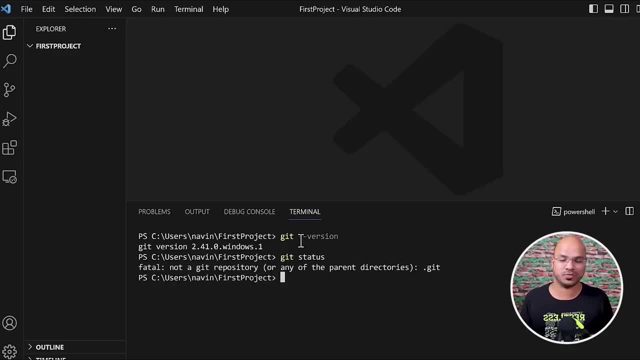 there's not a git repository. okay, so we don't have a deposit. git says: hey, you are trying to run status, but where is a repository? as i mentioned before, the folder here which is first project is your working directory. if you want to use git, you need to initialize git, so you have to say git init. 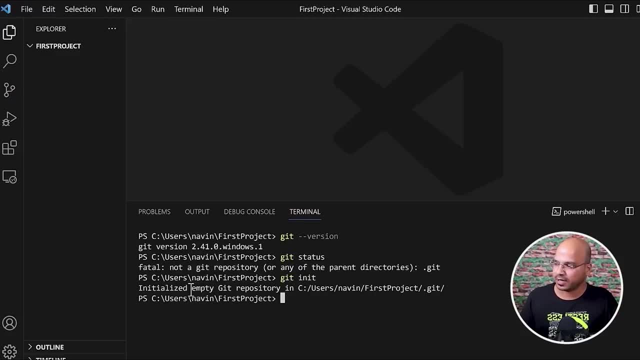 and this will create the empty git repository, and now you have git here. so where do we find it? so you can see, we have this path, which is c slash users, slash, green slash, first project: slash dot git. now this is your folder. of course, this is a. 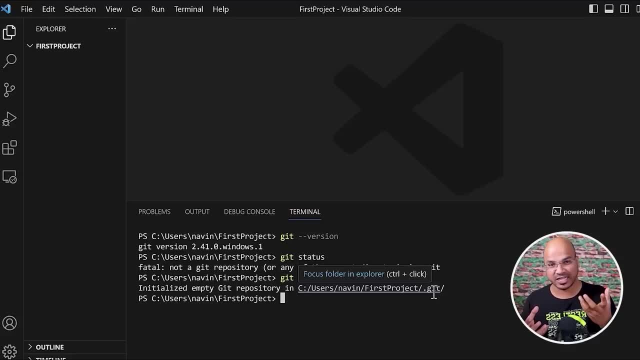 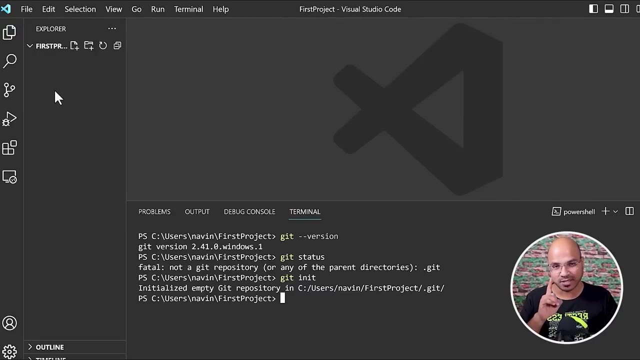 hidden folder, but this is where it tracks everything. so the staging area, the commit history, everything will be present inside that git folder. and this is different from your working directory, example. whatever file you create here will be a part of your project but not part of dot git. that's important to remember. in fact, till the end of the project or end of 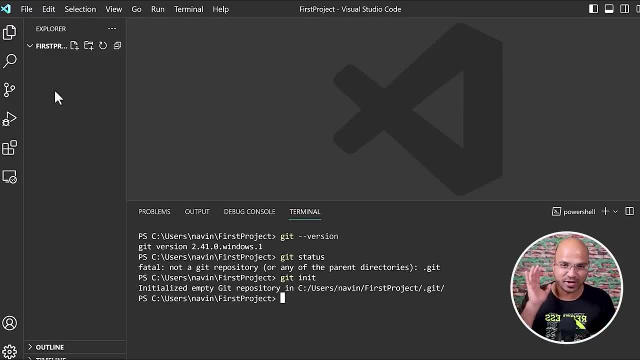 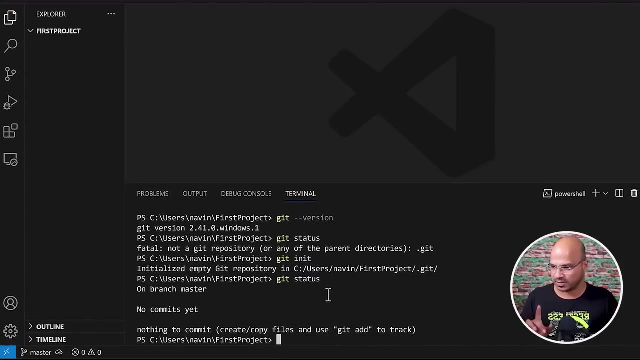 this is something you have to remember. by default, when you create a file, it will be a of your working directory. you have to let git know that this should be a part of git and that goes into staging area. okay, so now again, let's do git status and you can see. now git status works. 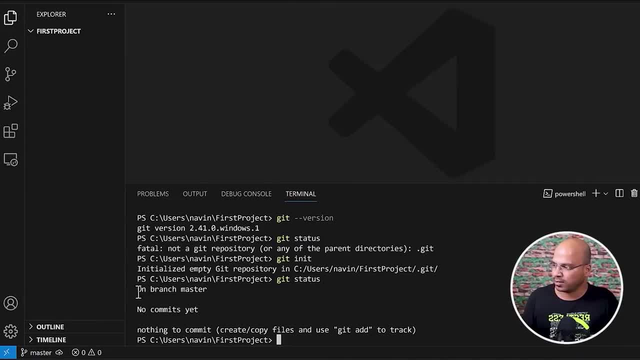 but then it says git status is on branch master. oh, now, this is something we forgot to do. remember when we were installing git. i've mentioned that by default, when you initialize your git project, you will get a master branch, but what we want is a main. we don't want to use master, we want to 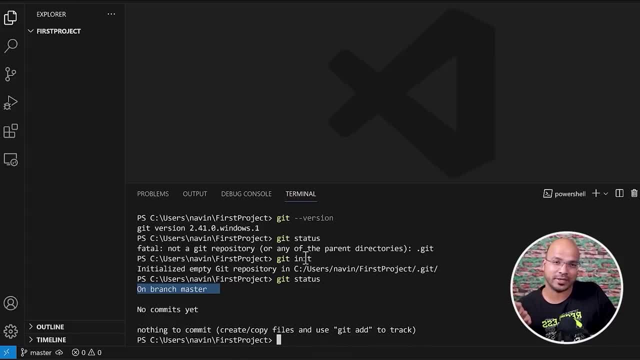 use something else. it can be main, it can be a demo, it can be any- any of the name for that matter. here we have the master. we don't want master. but even if you have master here, it says there is no commits yet. okay, so we have not created something, we have not done the committing. 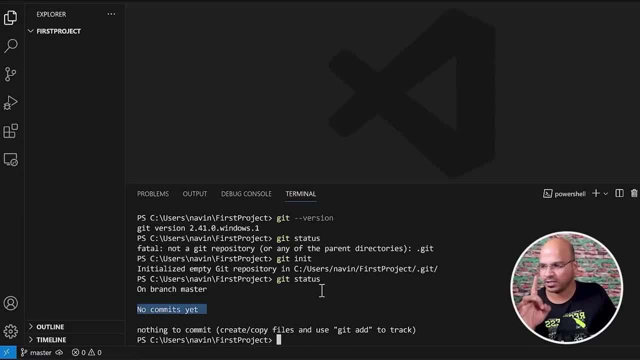 as well. again, what is commit? we'll do, we'll see that later. but at this point we don't want this name, right, we don't want master. so what we can do is we need to remove get now. do we have a way to remove get here? no, we have to delete this folder. so you have to delete dot get. okay, so we can say rm hyphen. 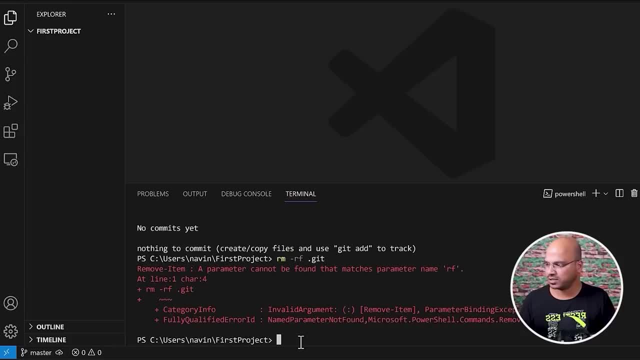 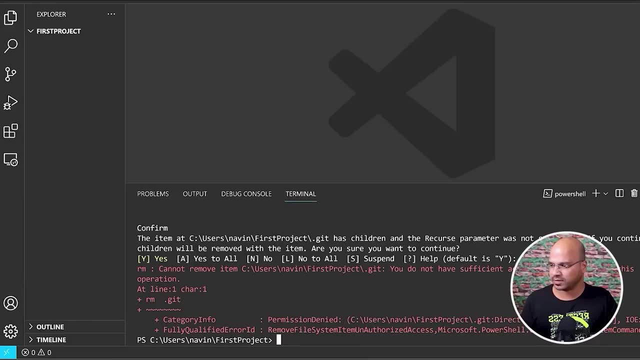 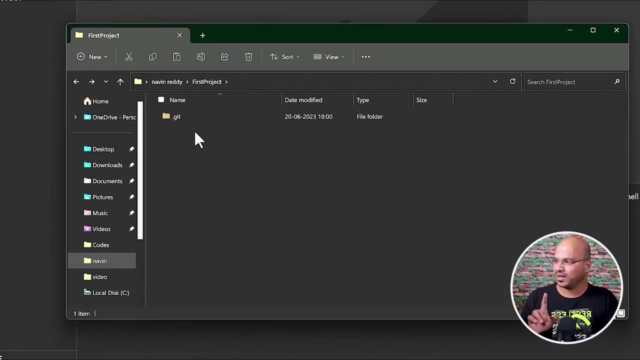 rf and we can say: delete, get okay. it says why, okay, don't have sufficient rights, okay, that's fine, i will just delete that from outside, okay. so how do i delete that? so what we can do is: here we can. we cannot say hidden folders, right, so let me jump to that folder. okay, this is a folder right now, here. 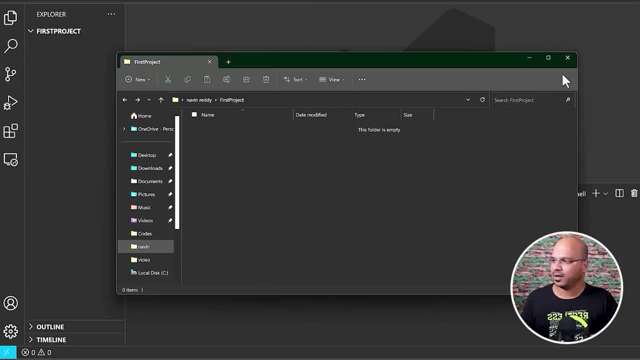 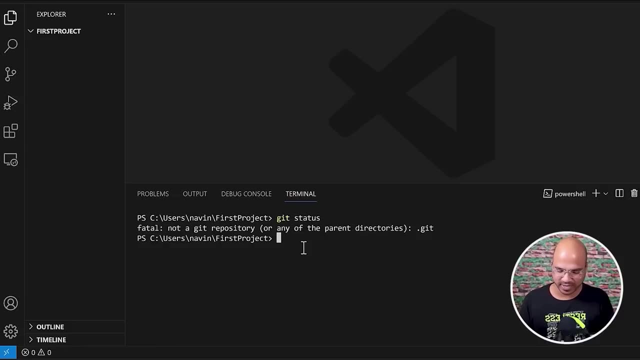 we have dot get, we can simply shift, delete and gone. now, if you try get status, you can say it will say not a get repository. and now let's initialize it now the way you can do that: if you say get in it, it will by default give you a master. we want main right. in that case you will. 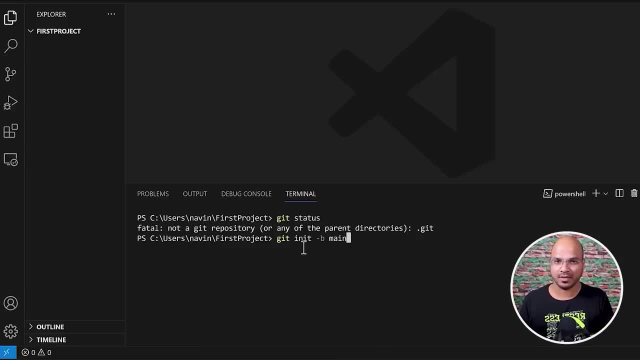 use something called hyphen b and main. so basically now you're saying that. so again, what is? we'll talk about that b later when we talk about branches. but here you can see that we have dot get. we can simply shift, delete and gone. now, if you try, get status. 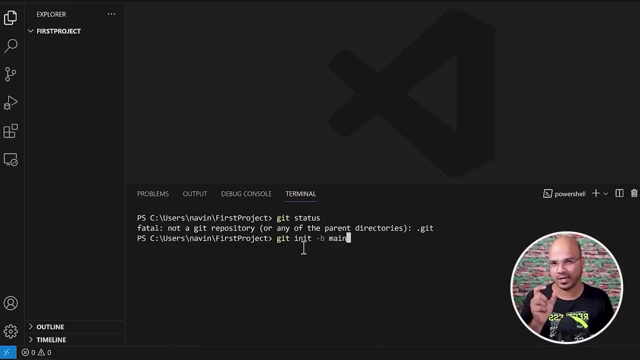 we are trying to say that whenever you initialize this project, make sure that you have the main name, not the master. when i say enter, okay, it says empty project created or empty git repository created, and now, if you say get status, you can see the branch name okay, so it's real right. so the 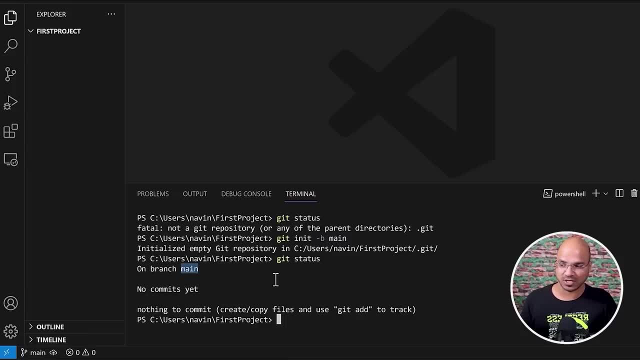 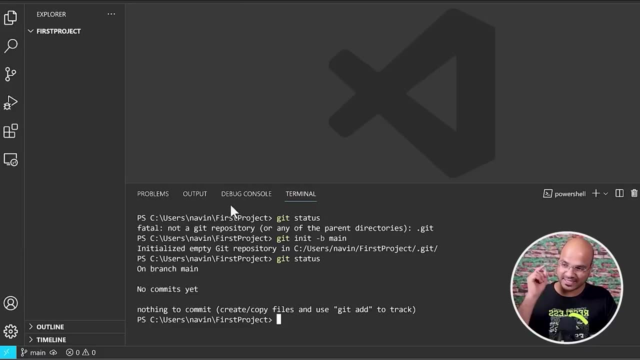 hyphen b is branch here, so branch is main, not master in this case, and we are going to continue with main till the end of the course. now, once we have done with the initializing of the project or initializing of the get, how do you add files that we'll see in the next video? 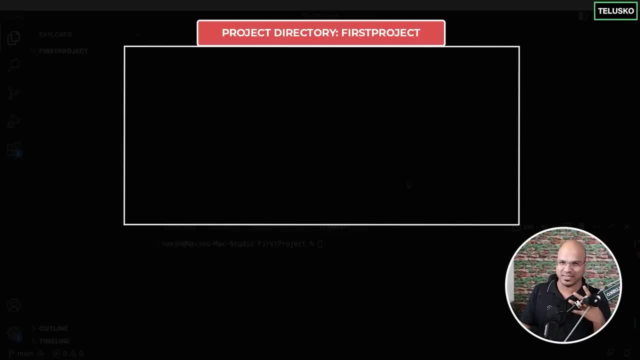 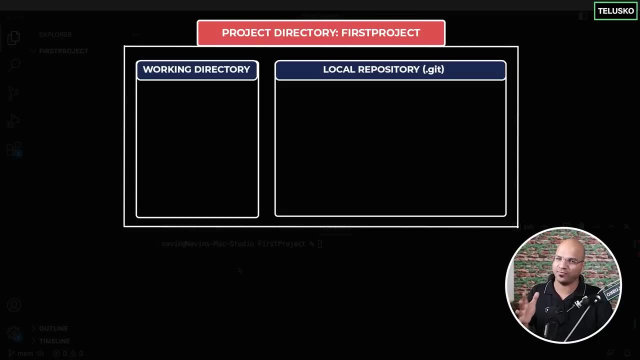 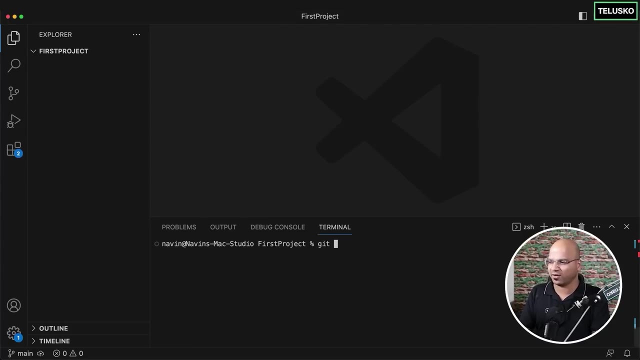 so, basically, we were able to create a project here. of course, we got an empty folder, which is your working directory, and we also able to get the git in it. remember, we have, we got a main branch, we have initialized the git project. now, basically the way you can check if everything is working. fine, you. 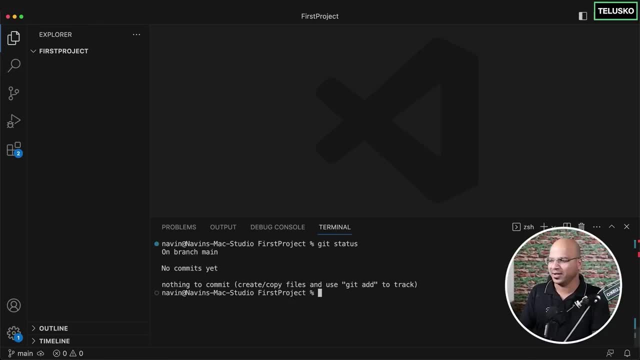 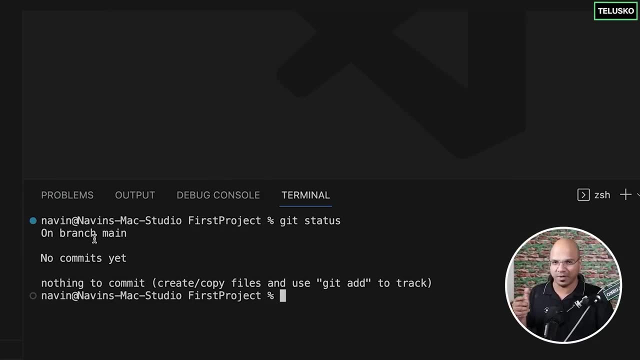 can say git status, and we are doing this from last one video, right. so git status will give you the status of your git project. it says on branch main. that means we are on the main branch now. of course, in future we'll see how it works, but for now let's get started and let's get started with the project. 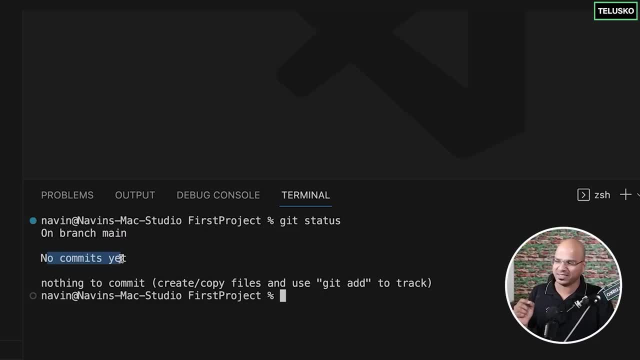 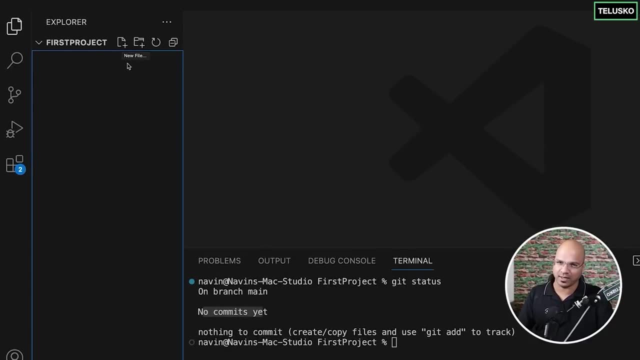 we'll see how do we get different branches and it says there is no commits yet. so of course we have not done the commit yet, and then the project itself is empty. now what i will do is i will create a very simple file. now the thing is, it doesn't matter what type of project you're working. 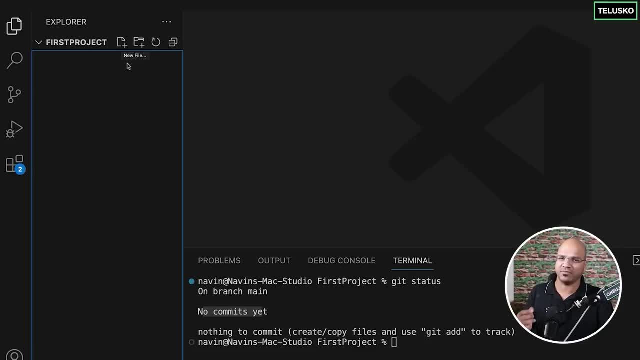 on a software project or a book project, you do create different files. right now i don't want to go for any language, specific things here related to programming. let me create a general file and let me name this as my first code: dot, txt or txt. so instead of going for dot job. 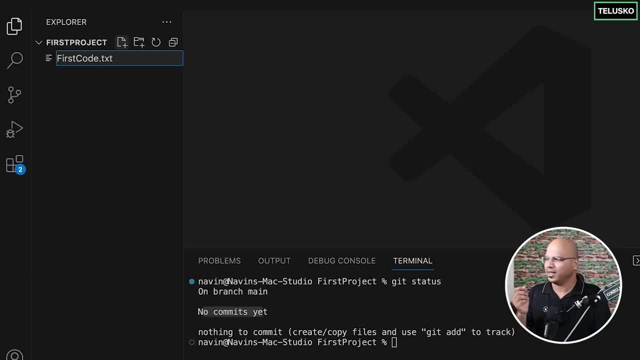 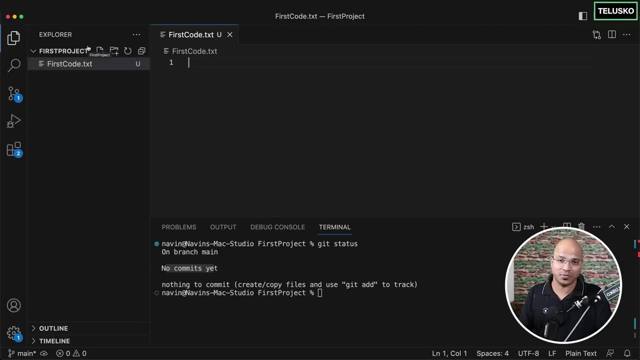 dot c, dot cs, which is c, sharp, dot, cpp. let's go for dot txt. now, this can be a coding file as well. it git forget, everything is same. it will treat txt as any other file. okay, so what i will do here is: well, i will write a very simple statement and i will say: hello world, okay. 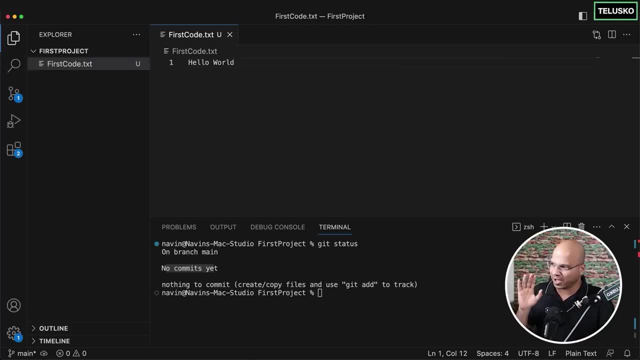 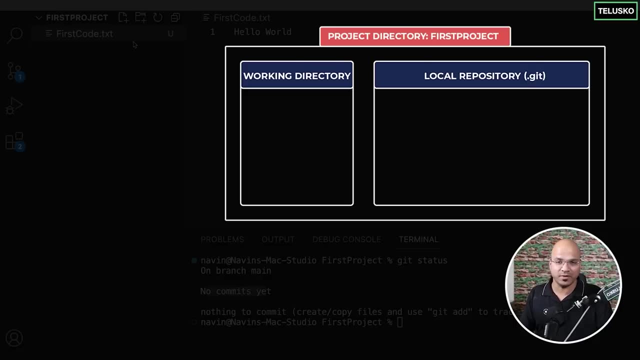 so that's it, nothing much. a very simple line in my first line of code. now the thing is, this project or this file is there in your working project, right? if you remember, we have talked about those different areas. right, we have a working area, so working directory. this is where. 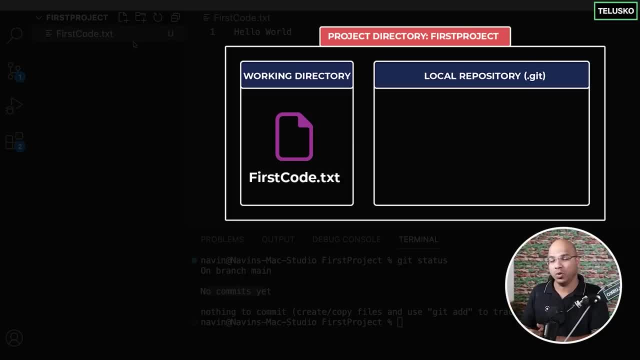 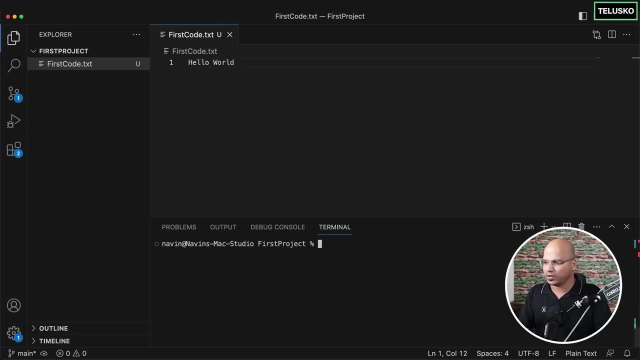 you edit your files and as a programmer, you work with. but if you want git to handle this, you need to add that in a staging area. if you don't do that, what happens? let's say, let's try now here. what i will do is i will say again: git status. it says there is a untracked file. now the thing is: 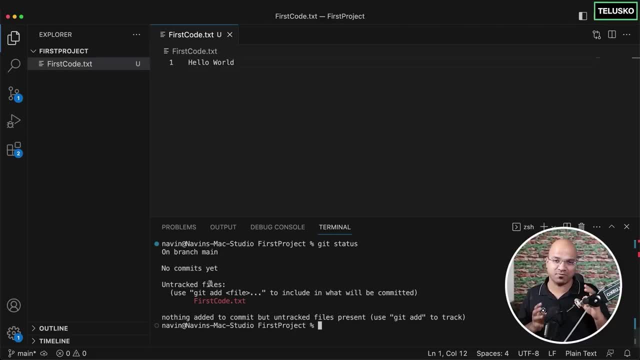 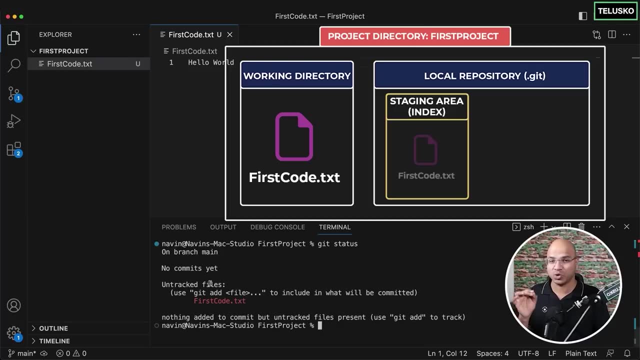 if you want to commit something, if you want git to take care of some files for different versions, you have to give that to git, and the way you can do that is by adding that particular file to this staging area. now, at this point, we have not done that and that's why it says so let's 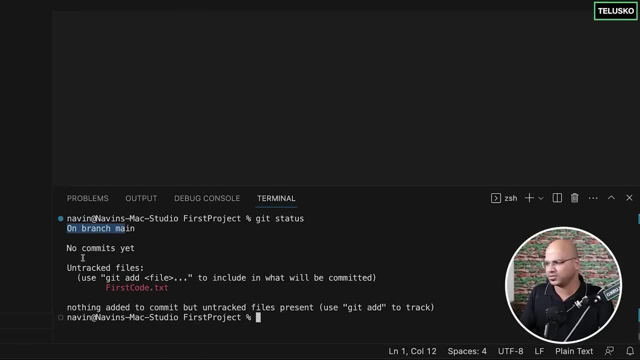 read everything. so it says on branch main. that perfectly makes sense: no commits yet. of course we have not done the commit yet. but it says there is an untracked file. okay, there might be multiple files, but here we only have one, which is first code dot txt. okay, it says nothing to add to commit. 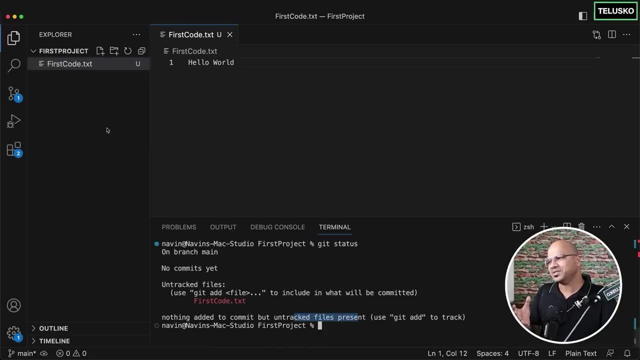 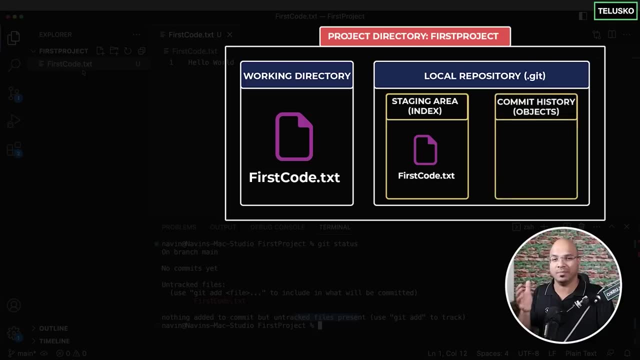 but untracked files present. okay, you know what i mean by that. you know what i mean by that. what happens? let's say, we have this file and now i want git to handle it. now, the way you can add it to the git by using something called a commit- right, so we use git commit. imagine: git commit. 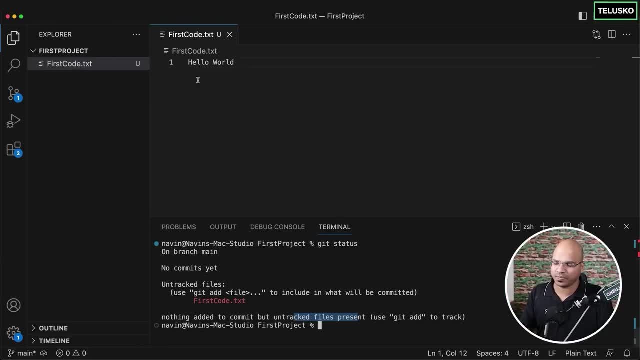 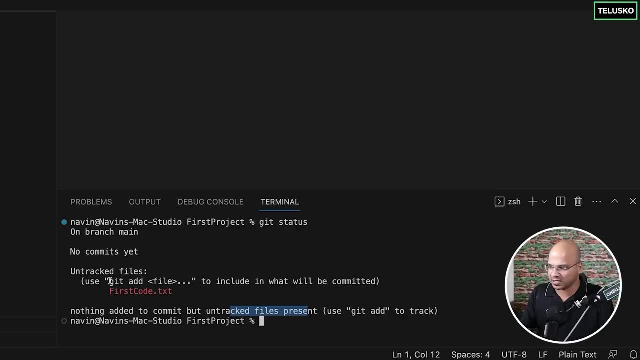 as saving something, but then git will not directly save this. you have to make sure that you add this in staging, and that's what it says here. now, if you want to add a particular file to the staging area, this is what. this is the command you have to use. so what is the command? it is git add, so that's. 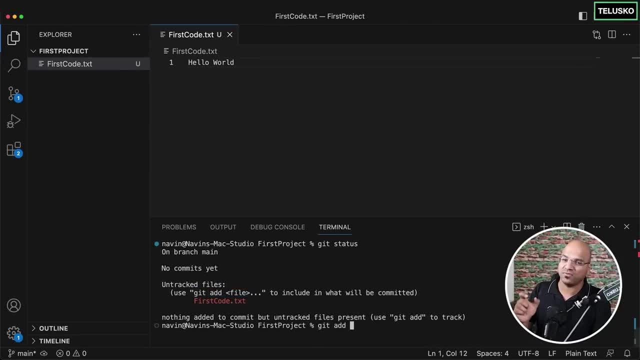 the two words. you have to use git add, and then you have to mention the file name. the file name- here is my first code- dot txt. okay, and when i say enter now, this is added in the staging area. and now, once you have done that, let me just clear the file or clear this screen once. 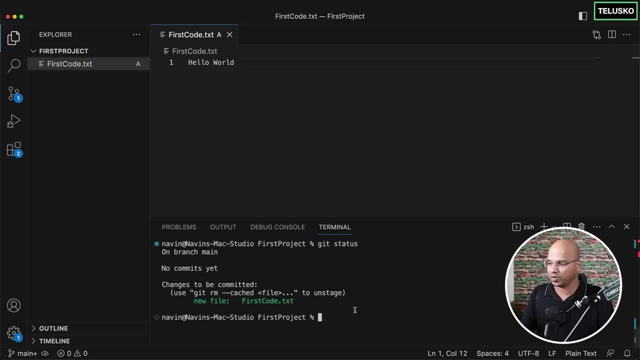 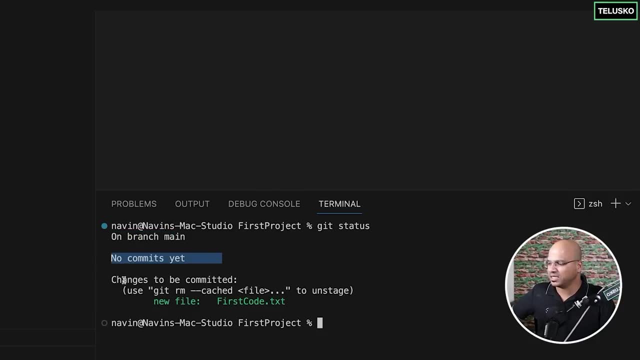 you have added the file to the staging area. when you say enter now you can see it says something. it says on: branch main makes sense, no commits yet, of course. but then it says changes to the committed it may. it says there is a new file added called first code. now, if you want to add a file to the 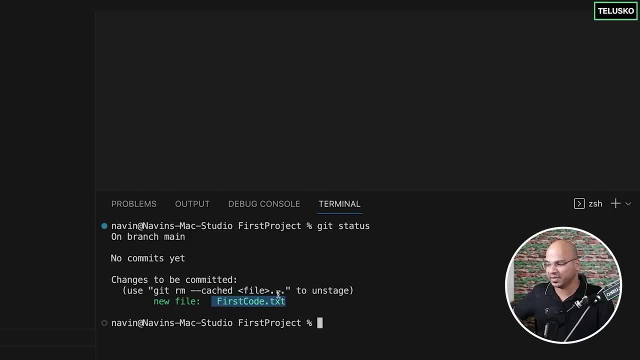 staging area. you can add a file to the staging area. you can add a file to the staging area. now is it available or is it committed? not yet. this is not committed yet. it is just that this is into a staging environment. yeah, if you want to unstage it, you can use something like this. you can say git: 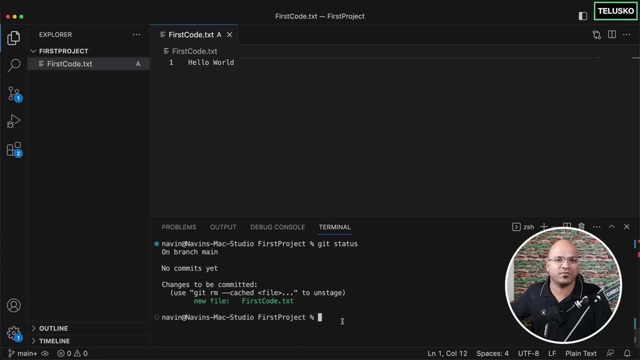 rm cached file. uh, you to unstage, but we don't want to unstage it, we want to commit it. now, how do we know that we have different commits? as i mentioned before, it also maintains the history right. so, whatever work you have done. so let's say, in your project you have till now you have done 50 commits. 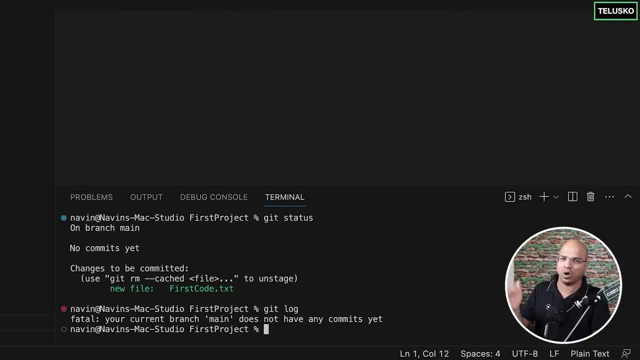 so I am going toistä a commit, which is a very simple command called git log. so with the help of git log you can see all the initial commits and you can see it says your current branch main- because that's my main branch- does not have any commits yet. so that means the file is there in. 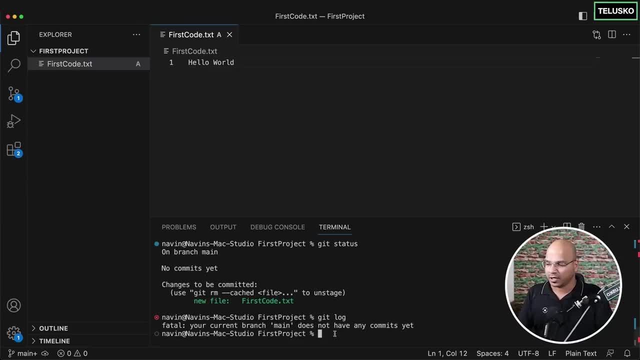 your working directory. the file is also there in the staging, but not in the commit history. now, to achieve that, to commit this, we have to pass another command, and that command is very simple, which is the commit. okay, so the thing is one of the questions you might be having. okay, so once we 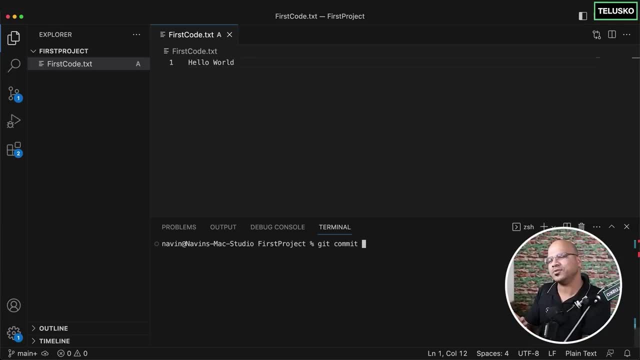 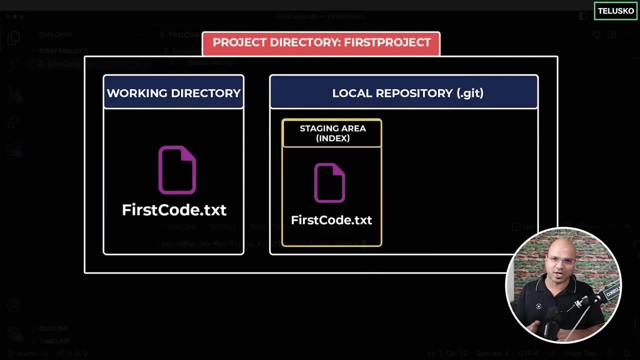 it goes into the local commit right. but how many times we should do that and after how many files edit? so normally let's say, if i can think about my project and if i'm working on one feature i will be thinking: okay, once i complete this feature i will say commit right. so that's why the project 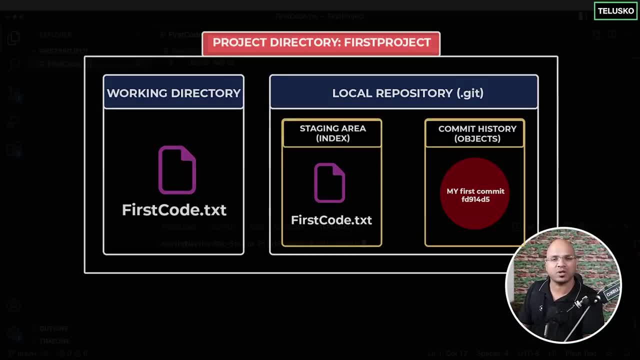 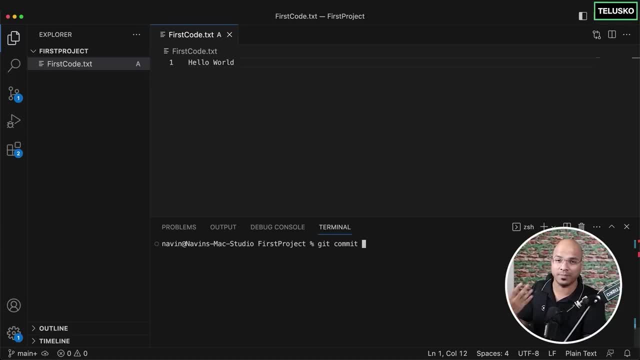 will be stored. that's not the case. actually. it depends upon a lot of different factors. you don't work alone, right? you work in a team. so sometime, your company defines how do you, how should you commit, how often you should commit. your company defines what type of messages you should have. 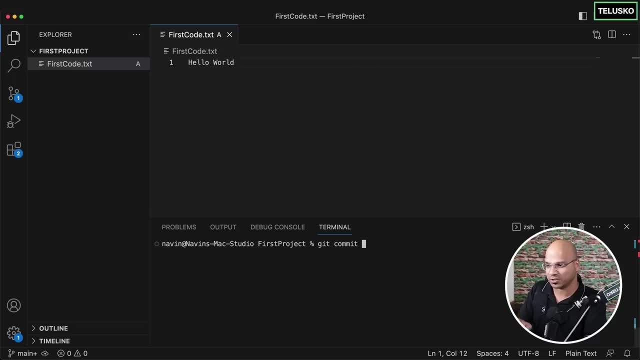 that's right. so for this commit, you have to also pass the message. so for this particular series, we are not going to see when to commit, it's just that we have to understand how do we commit. again, when to commit is something you need to decide based on your project, but then there's a common 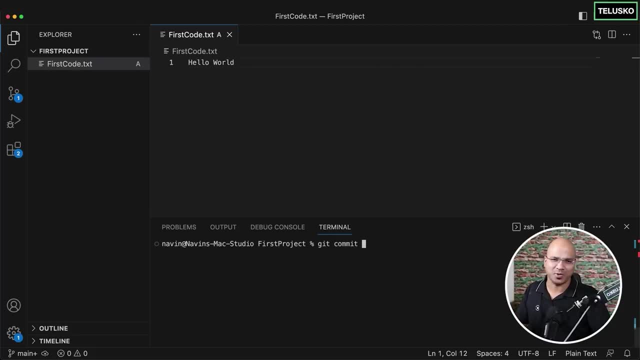 saying commit early and commit often right. so we are doing committing here. now if you simply say git commit, you can see it will not okay. it is giving you some message. you can see it will not okay. it is giving you some message here here. please enter the commit message for your changes and blah, blah, blah. okay. so what i will? 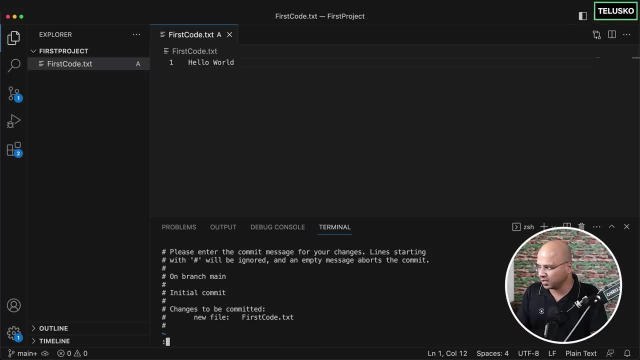 do is i will just edit: uh, go back, because this is the vim. okay, so abouting a commit due to empty commit message: basically, commit has not done. the thing is, when you want to commit, you have to make sure that you also pass a message, of course. right, every time you commit something you have to. 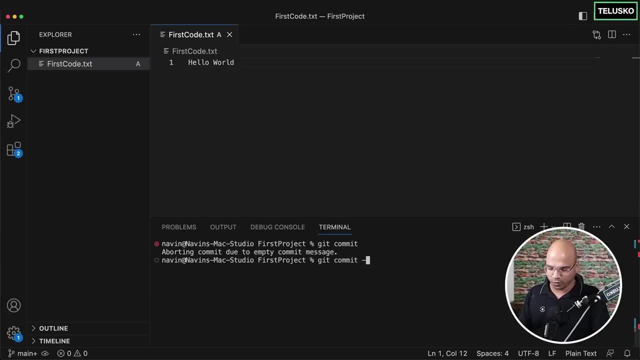 specify what changes you have done there so i can say, uh, if you want to add message, you can say hyphen m and then you can pass a message. my first commit now. of course this type of messages should be logical: uh, it can also define what features you. 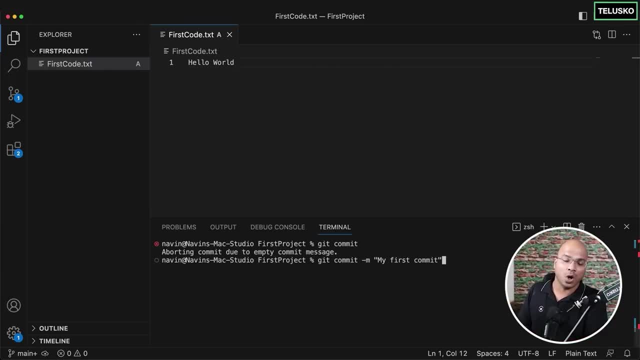 have added. maybe you have resolved some bug. you can mention that there or uh, i have seen few projects or few companies. they also follow something called issue tracking. so let's say if there's an issue created or some tickets created, you also mention the ticket number, which ticket you have resolved. 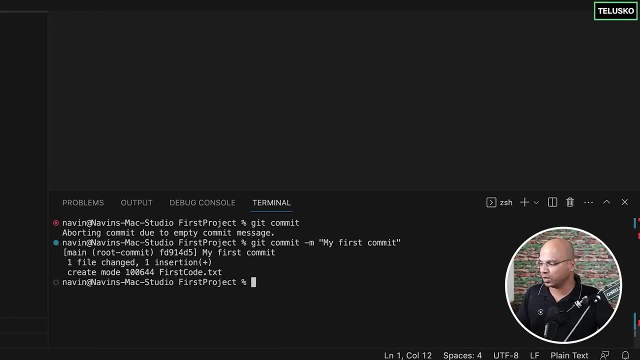 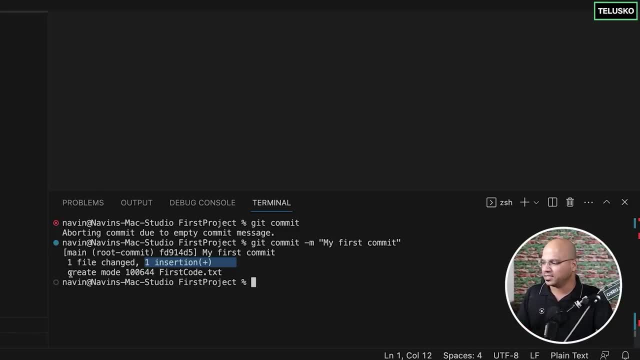 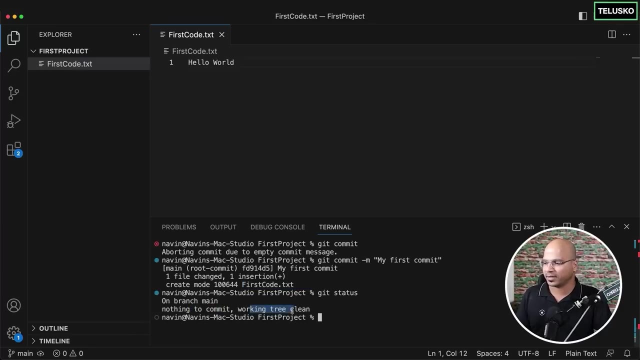 our first commit here, so this is your first commit. it says: create a mode. this is the file name. and now this is getting tracked by git. okay, cool, uh, after doing this, i will say git status. and now it says on main branch, nothing to commit working tree clean. okay, that's good. now, if you observe, there's. 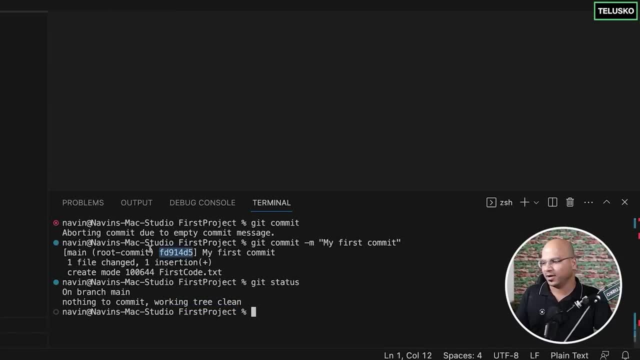 one thing here which i intentionally missed, which is this part: what is this number? that looks weird. right see, the thing is, git also provides you something called integrity. it means once you save something in a git commit, you cannot change it without git knowing about it. so basically, every time you want to make a change, git will know that something has been changed. how? 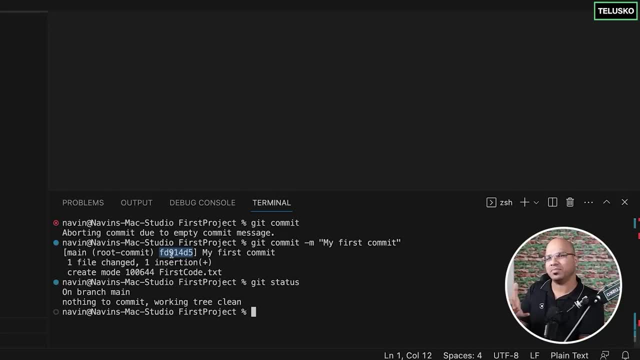 it basically follows something called a checksum. now checksum is something. imagine checksum as a fingerprint for the data. so example: if every time i change something in the data, it will change the checksum as well. okay, even if a small change in your in your code will change the checksum and git. 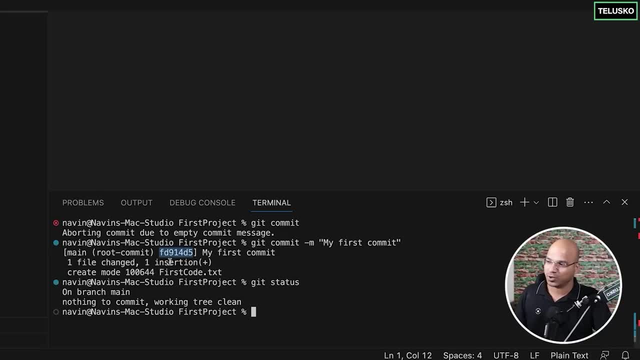 creates a checksum for every commit. so if you try to change something here in the commit itself- because of course a local file- right, if you make any changes, git will come to know that hey, it's not matching. you have made the changes, but i don't have any idea about it. so i have the older version. 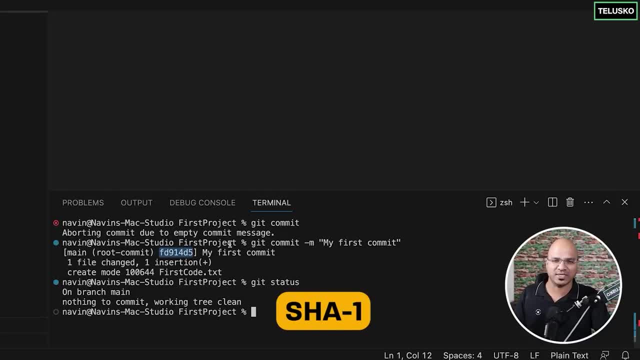 so, basically, checksum is very important. now, this is done with the help of sha1 and it creates not this number of characters, it creates 40 characters, okay, out of which we only focus on the first seven. these are the first seven hexadecimal numbers, so we got fd9145. of course, when you do it on your 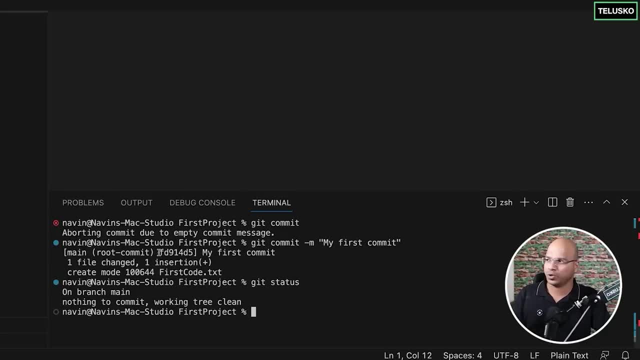 machine, you will get a different number right because this is unique to this particular data. but behind the scene, this is not seven. this is 40 characters to display. it is only showing the seven characters here. okay, now, since we have done our first commit, let's try git log. so git log will. 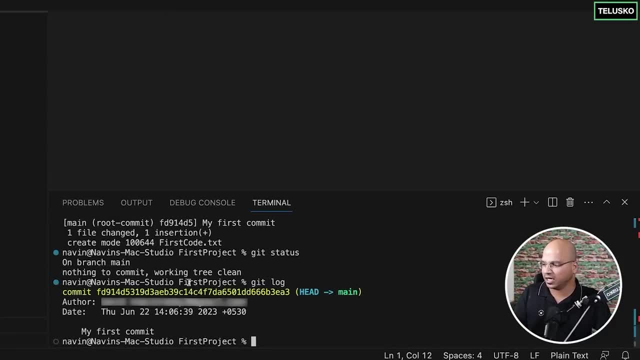 give you the log of all the commits. when i say enter, now you can see. it gives you, it shows something. it says: okay, what i will do is i will just clear this commit and then i will give you in so that we'll only see this particular message. okay, so let's see what it says. it says there's a. 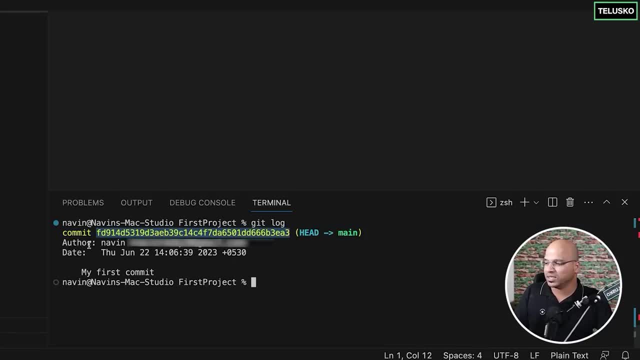 commit? okay, makes sense. and who is the author for this commit? this person, naveen. and that's my email id, which is hidden, which is blurred, and this is a date. so this is when i have done this commit. and now, when you see different commits here, there is also something called header. now this will make 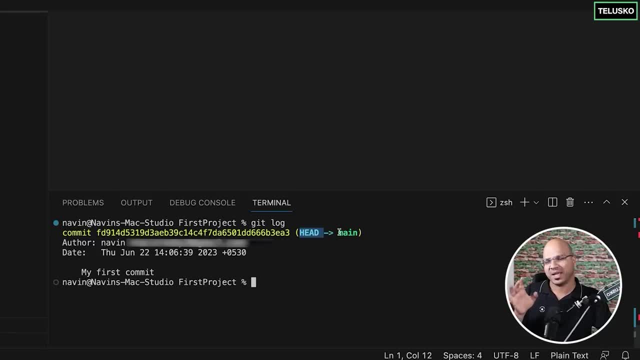 much more sense once we start working with branches. but at this point, uh, we have head to main, and the first commit is my first commit. the more commits you do, you will see, though all those things coming up there, and everyone have a different commit, and this is the 40 characters thing. i. 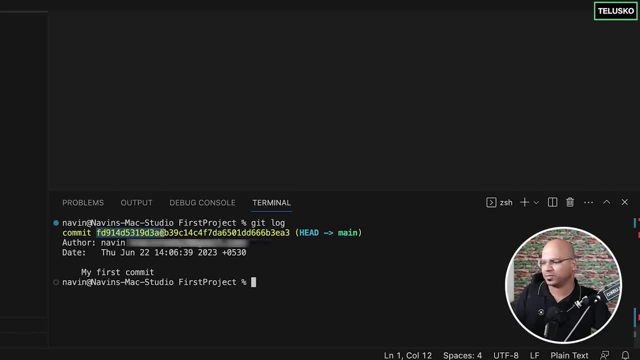 was talking about. so that's 5, 10, 15. oh, this must be 40.. okay, so we only see first seven, right, if you can see up here. so when we created this, this was the first seven characters, right, it's matching with this- the first seven characters, right? but then this is in general. 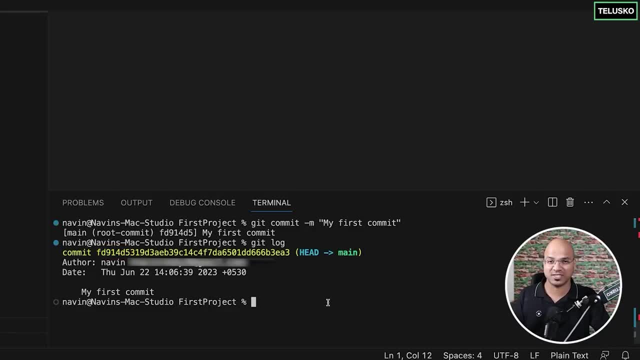 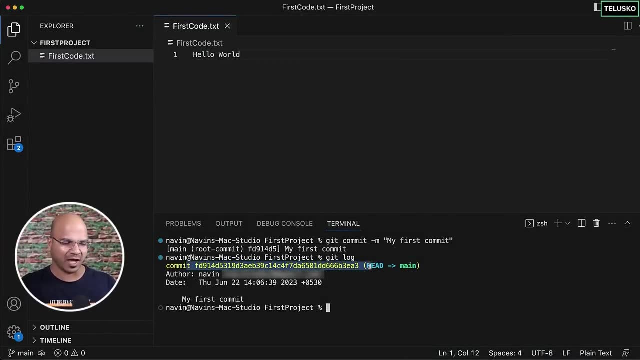 the same, just 40 characters. now that's how, basically, you do your first commit. so we are done with the first commit, right? and when we say git log, we got this particular commit here and we are happy with it, right, we got the first comment, basically. so what i will? 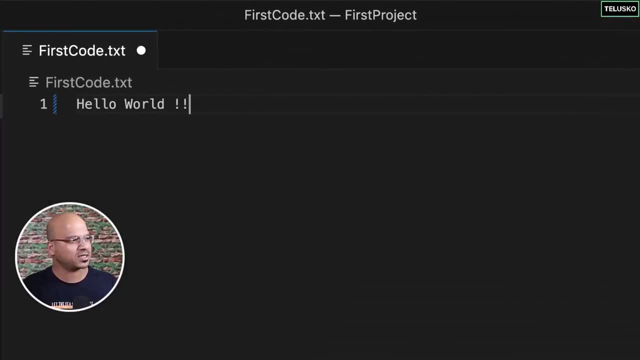 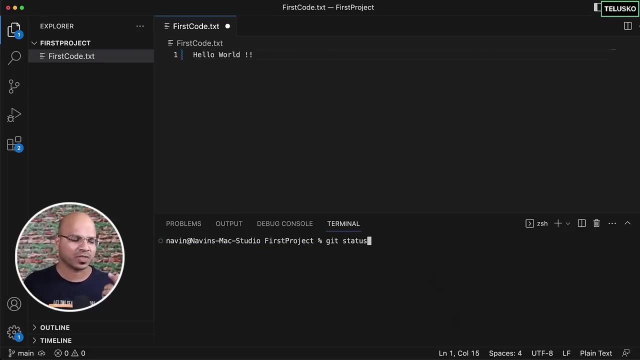 do is i will make some changes. let's say, i want to add some exclamation marks here, okay. so when i do that, and if i want to, uh, let's say i want to do the get status and, as i mentioned before, this git status will be using a lot. so when i say git status, it says, oh, git status on brand. 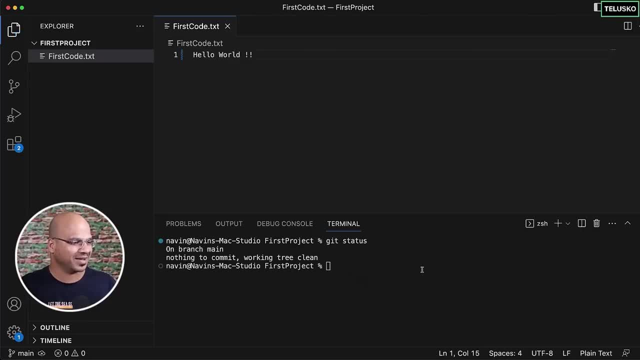 launch, everything is clean. maybe the file is not saved. okay, that's the issue. so you have to make sure that you save the file, because even git is not sure what you have done. so every time you make some changes, save it in your working directory first and now. if you see it says: 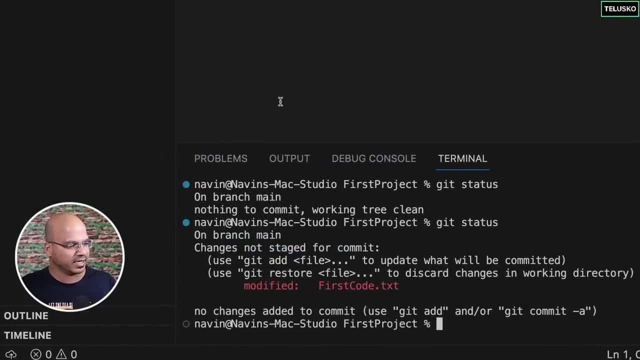 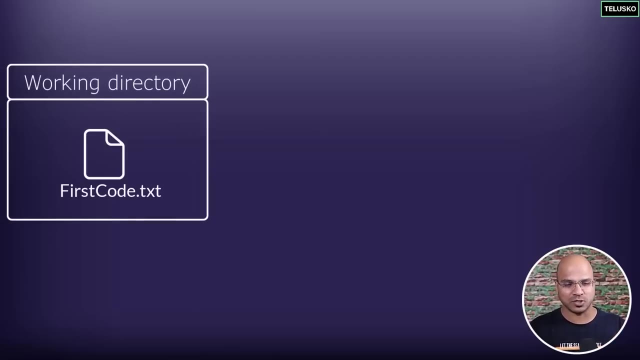 changes, not stage for comment. basically, there's a file which we have created and now this is into a modified stage. now that's right. the thing is, every time you make a change, or let's say, every time you create a file, it is into working directory, right, and then you try to stage it, so that goes into the staging area. so we got a working. 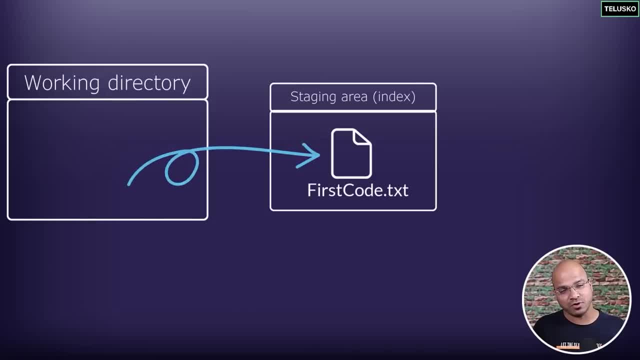 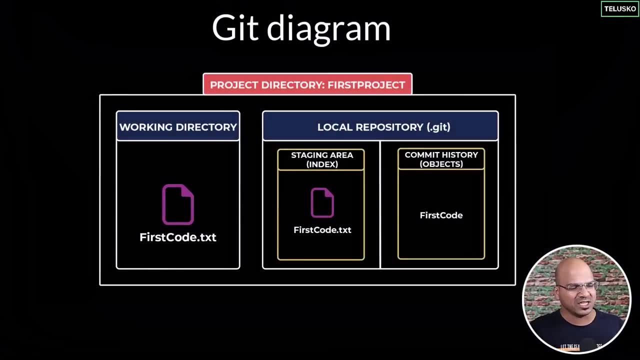 directory, then we moved that to a staging area and then from the staging area we do commit so that it will go to the local commits right? so those are the steps which we take. so before making these changes, we had data in the local commit and then it was there in the staging as well the moment you. 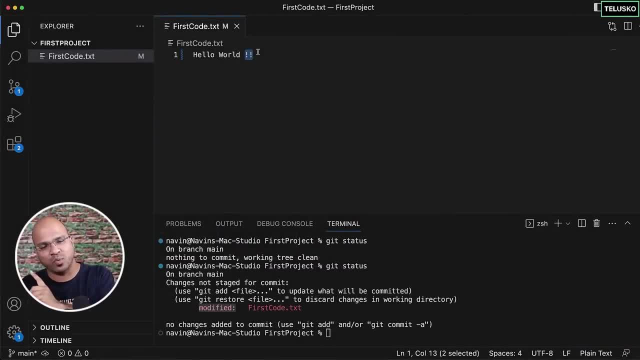 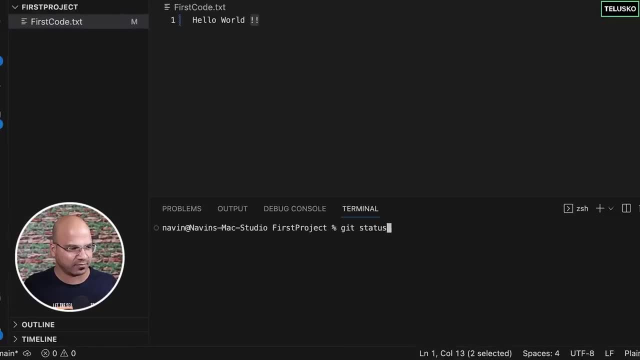 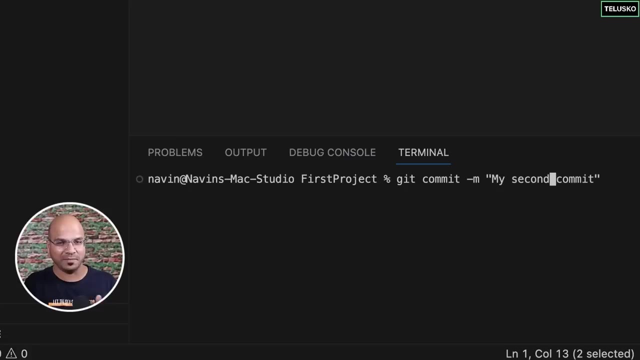 make some changes. now it goes into again a working directory. now this is not stage example. how do i know this is not staged example. let's say, if i do a commit now, so let's say if i'm doing a commit and this time i will say this is my second commit. of course this is not a good way of writing message, but just for. 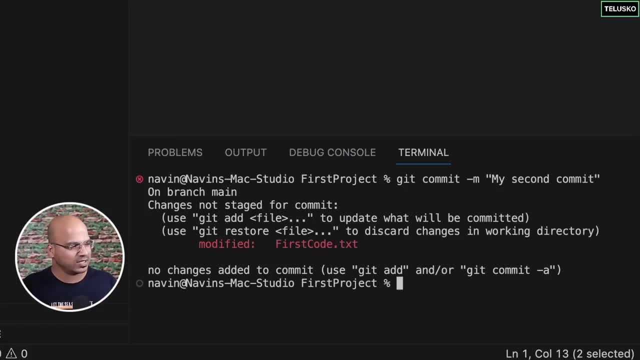 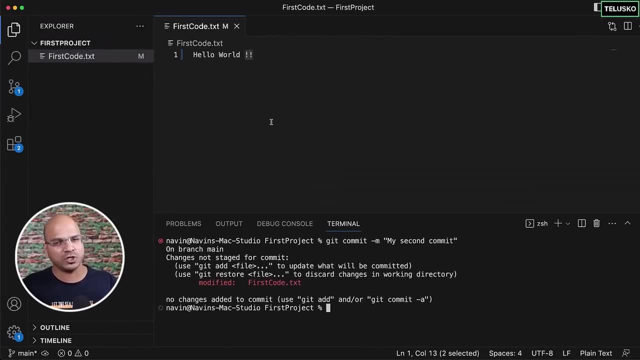 learning purpose. we are doing it. so when i say enter, now you can see it says changes not staged for commit. basically, if you want to commit something, the data, the file, should be there in the staging area. this is not so. that's important. so every time you make a change, 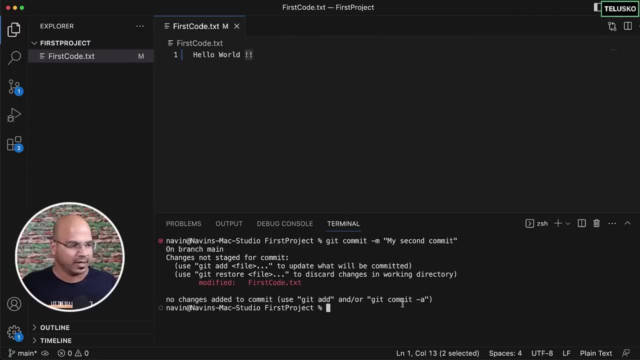 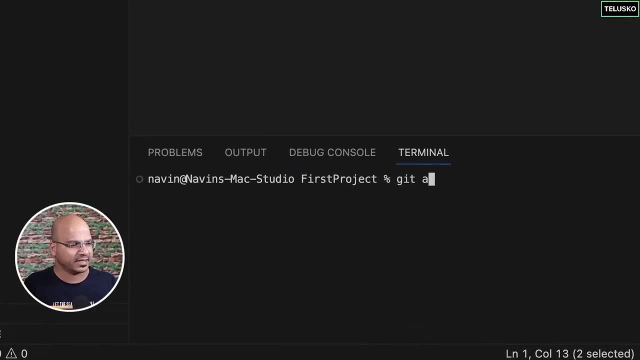 add that to staging area, then move that to the commit. now how do we add it? we have done that before. right, we can simply say git add. in fact, let me just clear the screen. so i will say git add and then i will say first code dot, txt, and then when i say enter, okay. so 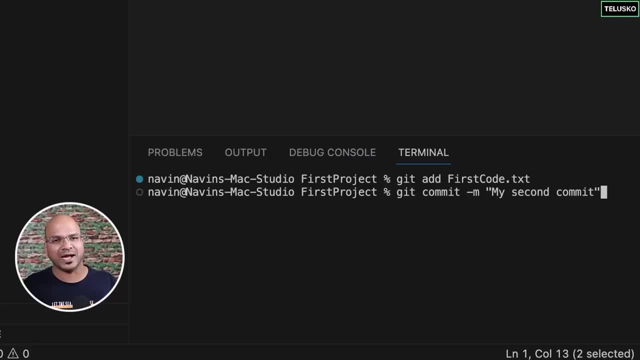 now this is into a staging area and now, once we move that to staging staging area, i can say enter and now we have done with the second commit. so in total we got two commits. okay, if i do a git log to check how many commits i have, so you can see we have two commits here. this was your first commit. 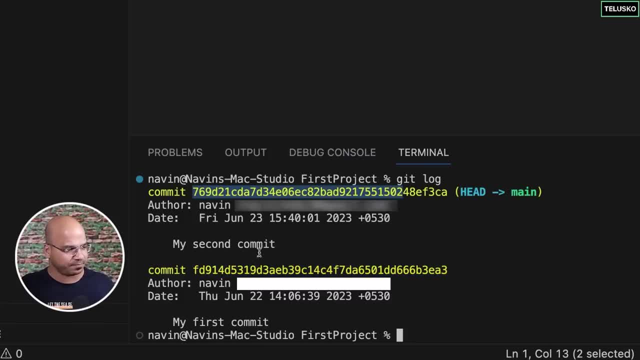 of course, with every commit you get the message there, you get the time which is mentioned here, and then you also get the author who has done that. so maybe if you are working in a team, you are doing some collaboration, so you will also know who has done what commit, and that's important, okay. 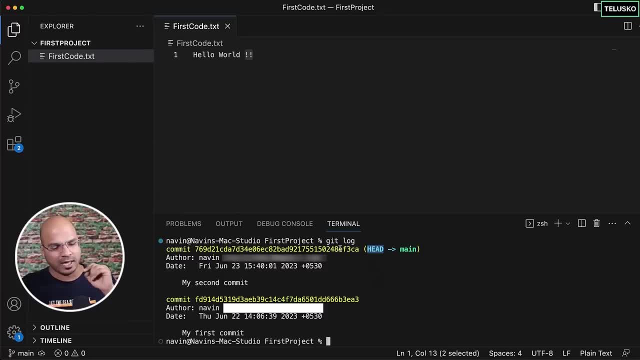 so now, this is where my head is. now the thing is, imagine, head is a pointer. so even if you have multiple pointers in your local commits- as i mentioned local commits- i have multiple. uh, it's basically multiple commits, right? so you'll be having a pointer: which one is the latest one or which one we are pointing to. so here we are pointing to this. 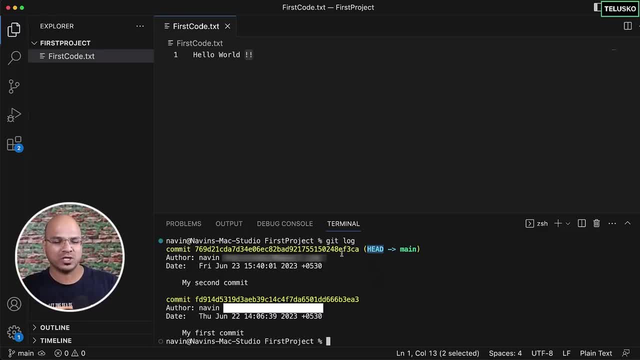 one and again. we'll focus this more once we move towards the concept of branching. okay, now, what do you think if i add one more exclamation? so what's the step? first, save it. the moment you save it, of course, it becomes a modified version. so it is not staged and you can see it. we also get a. 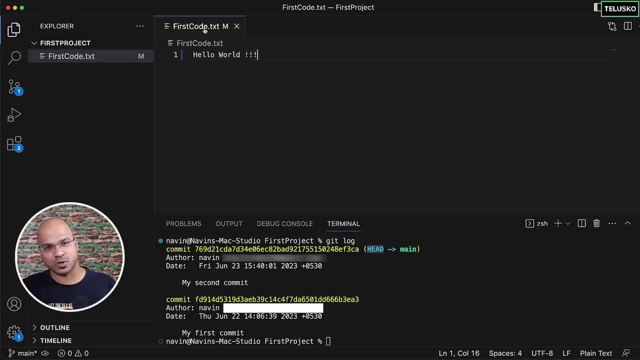 message here, or not a message, but on the in vs code, especially if you are using some uh ides, which supports git in a good way, and vs code does that and you can see. it says m, which is your modified, and the moment you add that to your staging, you will this will be gone. but what if, of course, staging is important, right? so 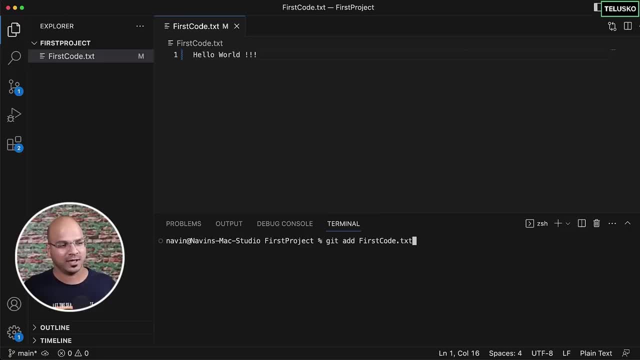 from working, you move that to staging. from staging you move that to commits. but what if you want to directly commit something like this? let's say i want to do the commit and i will say: this is my third commit. i'm very bad with comments, but this should be something like added exclamation mark or 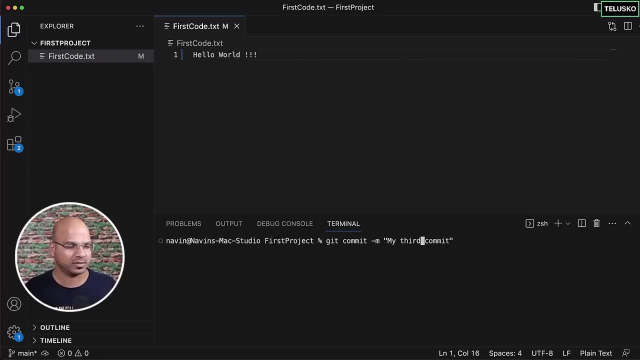 solved a particular story, or if you are working in agile methodology, but here let's say, i have this particular commit and now i want to do the commit without staging. can we skip staging? and we can. if you want to skip the staging part, you can simply use a hyphen a as an option. so say: git commit- hyphen a, then hyphen m for the message and then 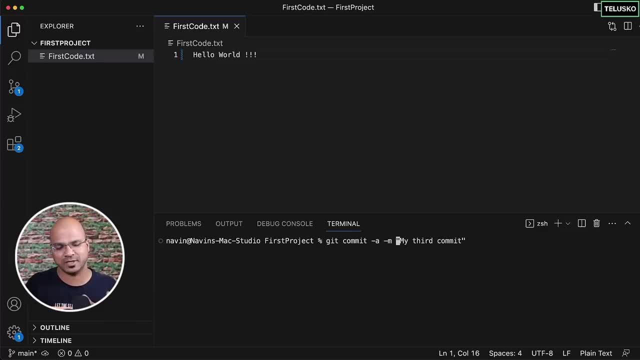 you can pass the message. basically you are skipping the staging thing. so if i say enter now, you can see the commit has been done without going into staging area. okay, so that's important. if you want to do it without staging, it will say it is not tracked. so if you, if you want to move from the 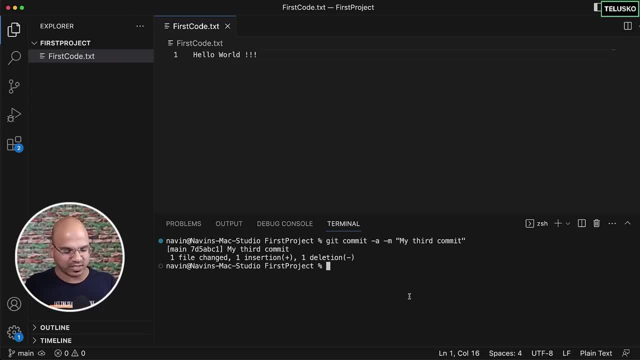 working directory to commit. this is how you do it. okay, now, uh, if i do git log once again to check, everything is good, so you can see we got three commits. uh, this is the third one, recent one, and if i say enter, you will see also see the previous commits. so this is how, basically, you use hyphen a. 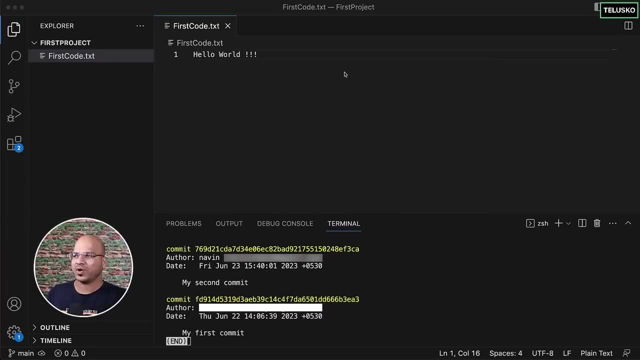 to move the file from working directory to the commits. so let's try to understand the diff command. so basically, in git we have this option of using hyphen a to move the file between what you have worked and what is already there in the commits. so let's say, if i make some changes here. so what i will do is i will first of all check. 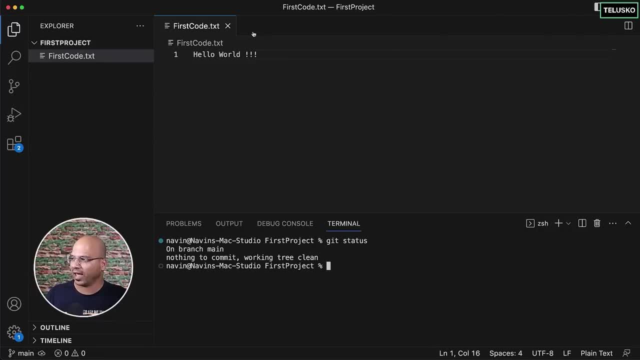 the status of this and you can see there is nothing in my staging or nothing to track and i will make some changes now. so if i say hello world, so that's the greeting, and then i will say take input from user and add the values. so let's say i'm writing a pseudo algorithm here. 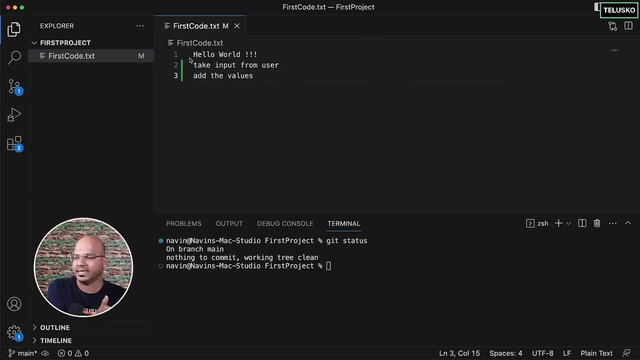 and when i say save and if you can observe, especially in in vs code, you can see this green line. this basically means you have added something okay in the file. and now, if i go back here- and of course i can simply do a git status, of course git status will give me the changes here. but what are? 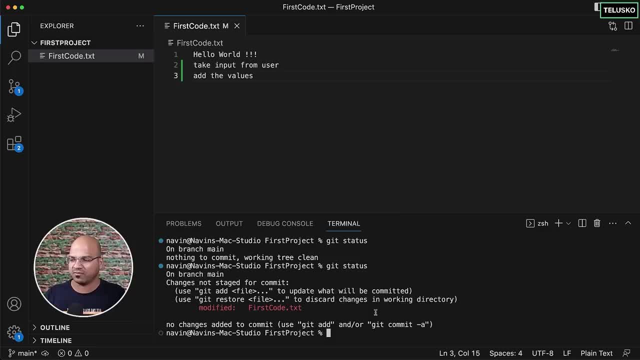 the changes. i mean, of course, git status will show you that this particular file has been modified, but what exactly is modified? i want to know that. so what i can do is i can say git and i can type. now, when you say git def, and when you say okay, when you say enter, it will show you the changes. 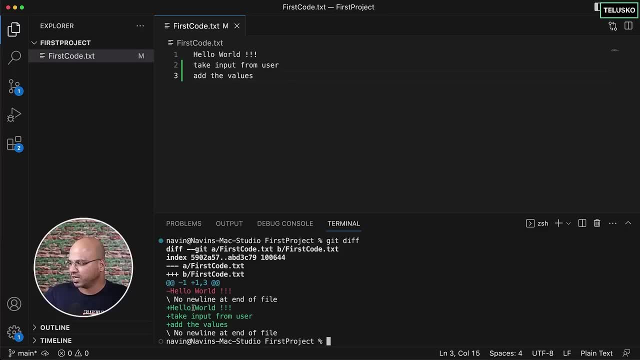 which happened in the file and these are the changes you can see. it says: uh, there have been few changes. the number of lines now, this are the number of lines which you have added. uh, so we got hello world. in fact, there's a change here as well. of course, we have not changed here. the only thing. 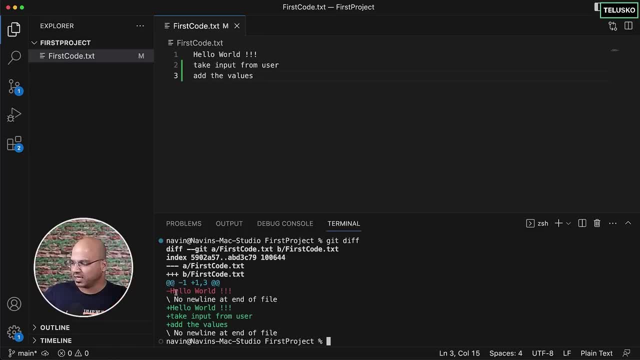 is. i said enter: right, that's a new character now. now, basically this is the older one and these are the changes. now, if you want to see- okay, i'm doing a commit, it says it is untracked. i want to know what changes i have made so you can use something called a git div. so basically it will check the. 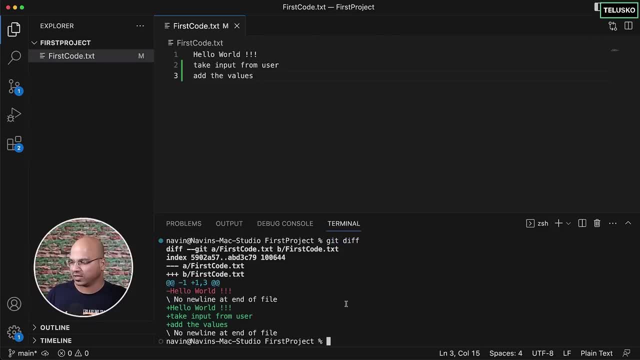 commit, it will check what data you have in your working directory and then it will track the changes. and now, once you have done that, maybe i want to add this. so i will say git, add first code dot txt, and it's enter, enter. and now, once you have added, let's say git, diff. now you can see there's no difference. the reason: 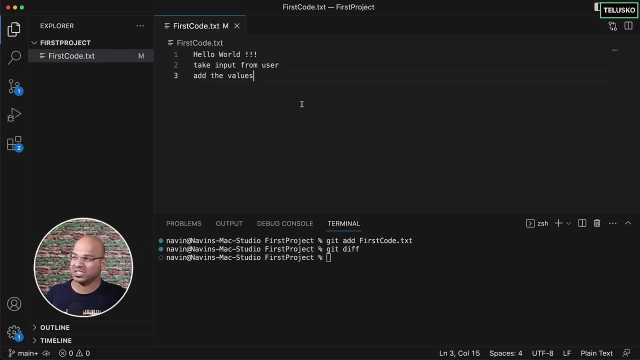 this is not into a modify, this is into a staging right now. once you move this to staging, i can also commit. but now what if i want to find the difference? i have added that to staging area and now i want to find the difference. in this case, again, you can do git diff, but since we are 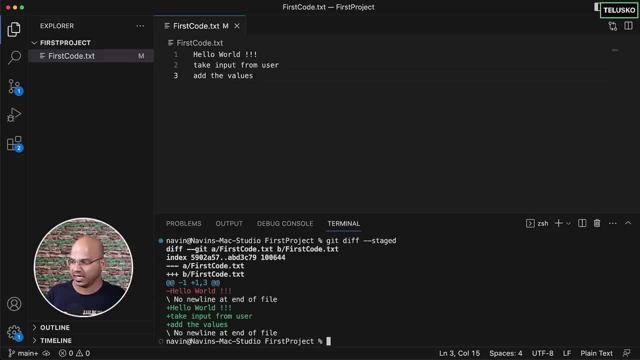 into staging. i can say hyphen, hyphen staged, and now you can track it. so if you have your file in the working directory and if you want to check the difference, you can use git diff, which is differences, and if your file is into staging area, then you have to use hyphen iphone staged. 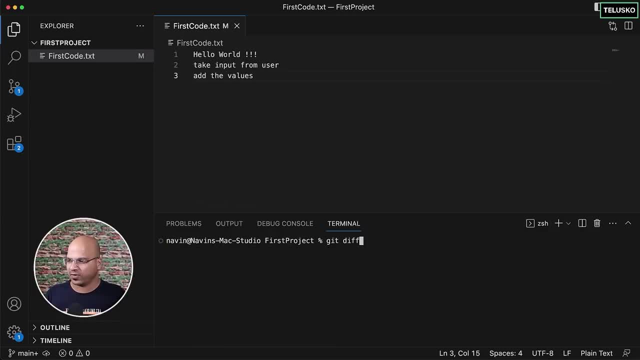 to check the changes, because it's already into staging area. once we know the difference, we can simply do the commit now. and of course, for commit we have to pass the same thing. we have to say git, commit and let's say: i'm basically working on a project where you have each task given a number. 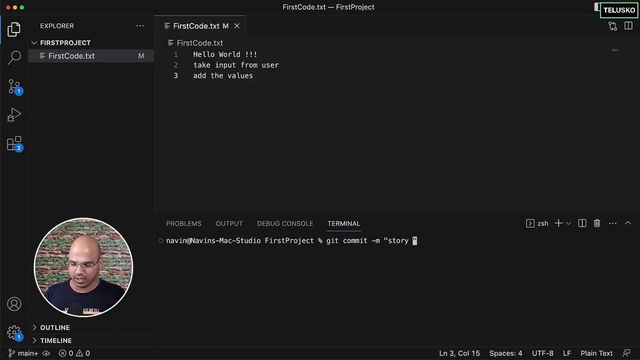 a story number, so i can also say story 3.1 and i can say: message is user input. so basically, that's how you can mention some messages which should be logical. yeah, and now if you see git log, you can see the entire history. so this is the recent one which you have done. 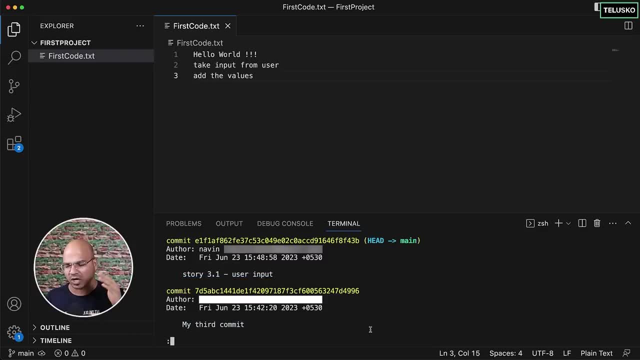 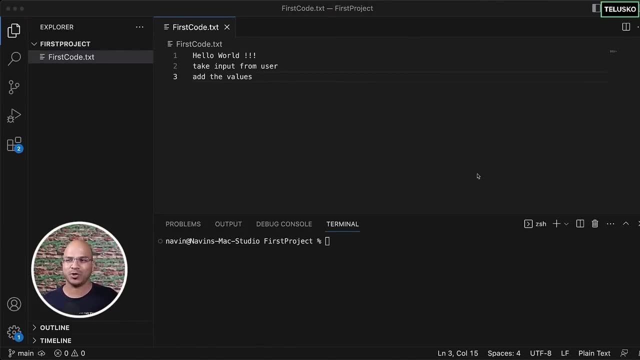 and then this is the. this is your third commit and if you go down you will, you will find more. let's try to understand how do we remove a file from a git repository. so let's say you already created a file and then you have pushed that to a git repository and now you realize, oh, that's. 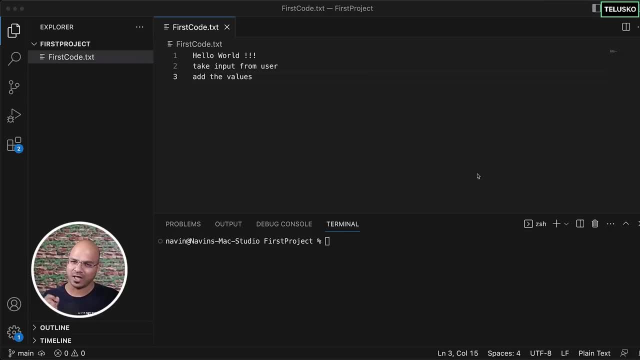 not the file. i wanted to put that into git repository. now why you will not put something in a git repository? think about this: you're working on a project and you have multiple files, and one of the file is basically where you put your credentials. let's say, i create a file here, so this is where i will put. 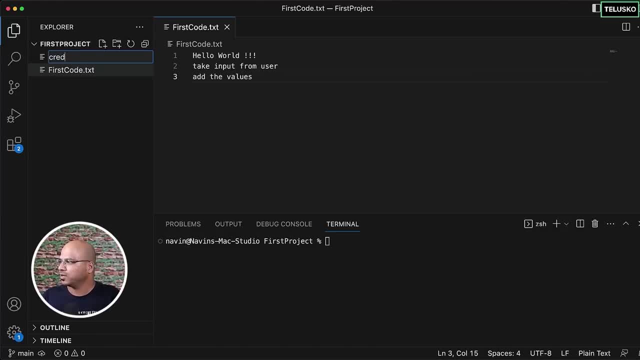 all my password, just for my references. so i will say all my creds dot txt and this is where i will basically put my username password. so i will say username is nvn02 and my password is rdy03. so this is my basically username and that's my password and i just want to save it for my. 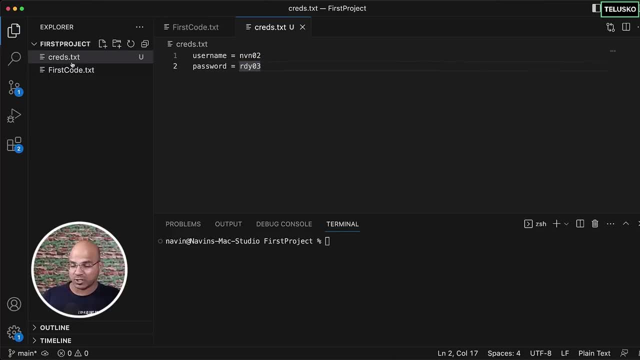 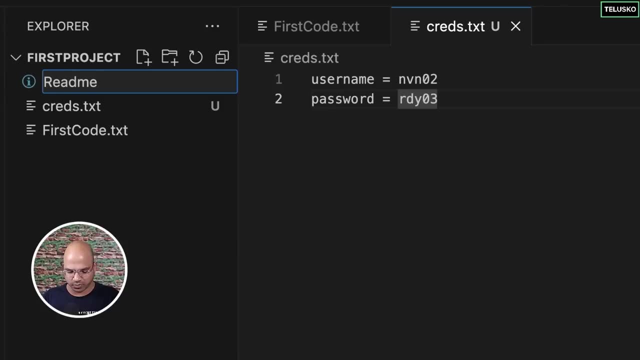 reference so that i can just connect with the database or something. and i want this to be only in my particular machine, i don't want to push to the server right. and after this, let's say we also have some readme files. so we got readme dot txt or readme dot md. basically, we have a concept of 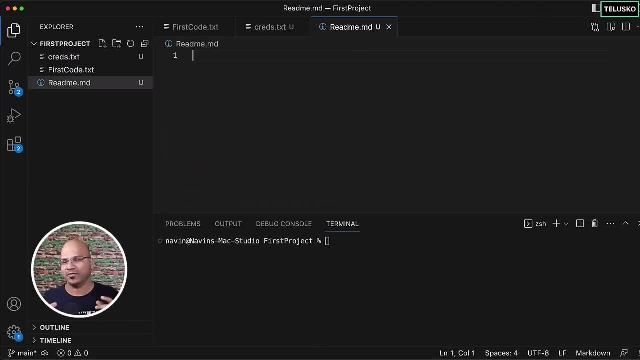 markdown. you know, if you want to make some document beautiful, we can use markdown to make it more beautiful. that's what git uses. so basically, we get readme, dot, md and this is an important file to make it more beautiful. so we can use markdown to make it more beautiful. that's what 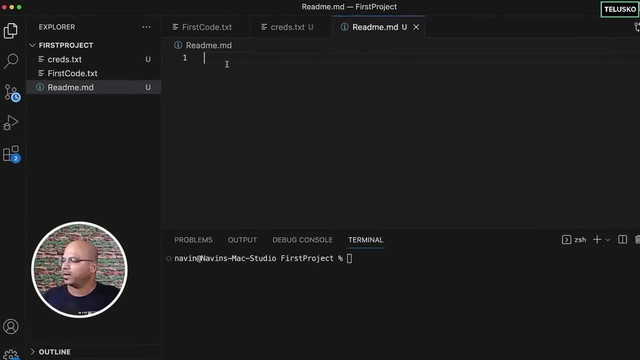 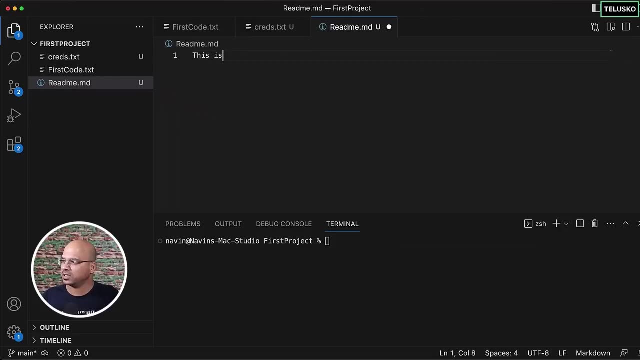 git uses in every project. so we'll also see that and okay, so you can see we got you here, which is untracked, basically. so let's say in readme i will say: this is my first project, author is nvn ready, company is teresco. okay, so let's say: we have these values here, credentials, we. 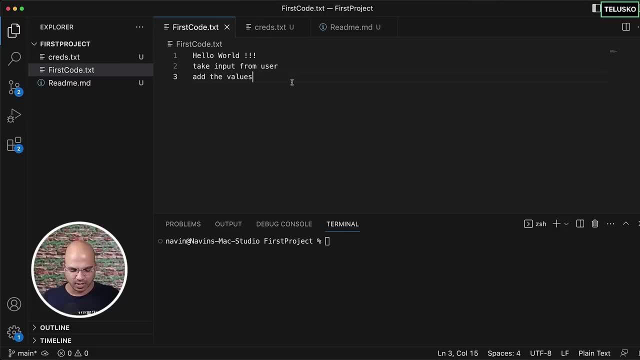 already mentioned, and let's also do some changes in the first code, in the first code. now you want to submit data to the database, so let's say we have all these changes in the code. okay, this imagine: this is a coding file of any language which you love and we have made the changes here. 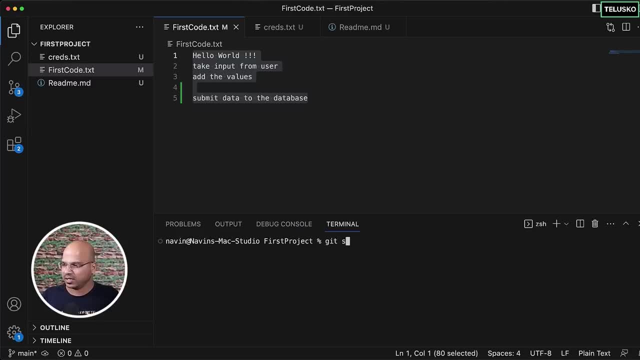 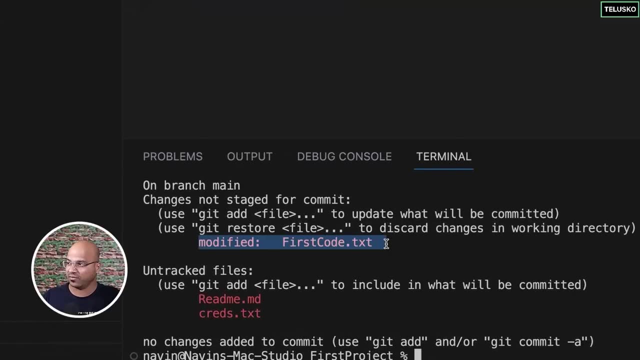 and now what i will do is i will just see the git status. when i say git status- you can see it is. it is showing that you have one modified file and that's correct. we have done the modification and you've got two files which are basically untracked, and that's why it says you can see if. 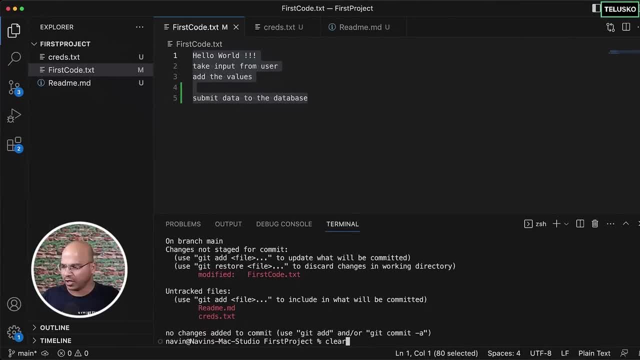 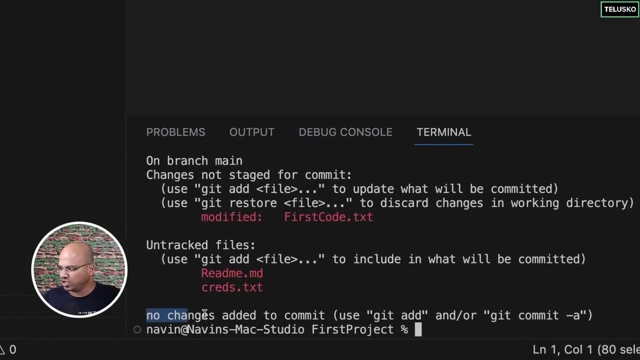 you see here and you want to submit data to the database. so let's say, we have all these changes, we have u, which is untracked. okay, now i know what to do. uh, in fact, if you do one status once again, you can see there's an option here as well. uh, no changes added to the commit. use git add or. 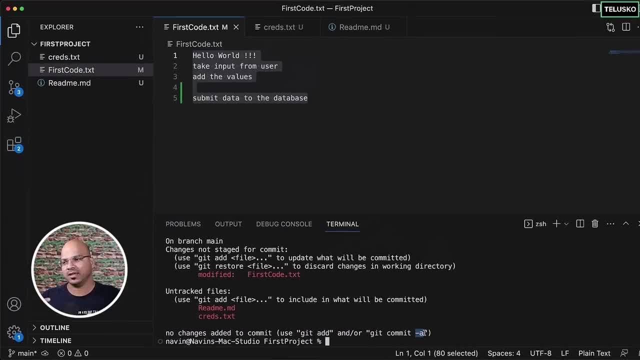 git commit hyphen a. so hyphen is basically an option of adding directly in one line itself. but let's say, if i want to add all the files in the staging, how will i do that? of course, uh, if you want to add all the files, you can simply say git add and mention each file. so this is. 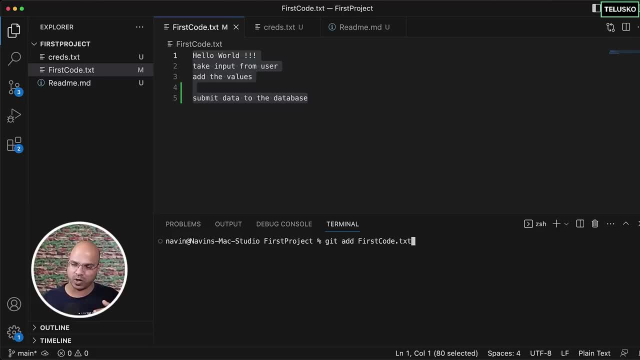 first code: dot, txt. then you say enter again, do it for the next one. or what you can do is there is a shortcut. you can simply say dot now. dot simply means you can add all the files in the in the staging area enter and done. now all the files are been tracked, so you can see. now it says: 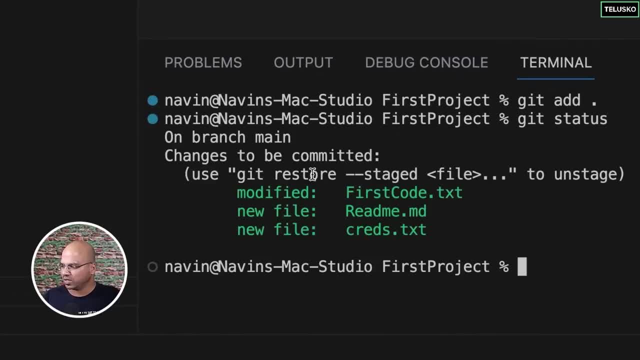 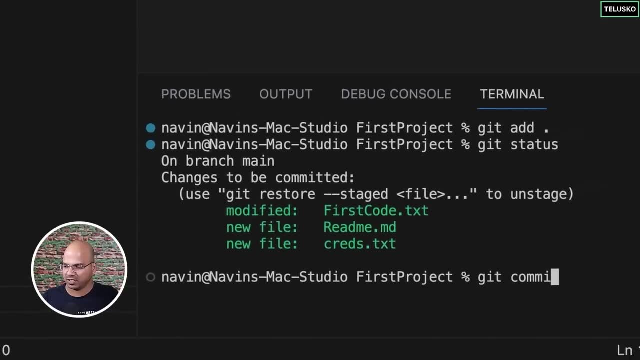 a, which is added, and if i say git status now. so you can see we got a new file, two new files and one is modified and the other one is not. so you can see we got two new files and one is modified, one. and if you want to make the changes, you can simply say git commit hyphen m and you can pass. 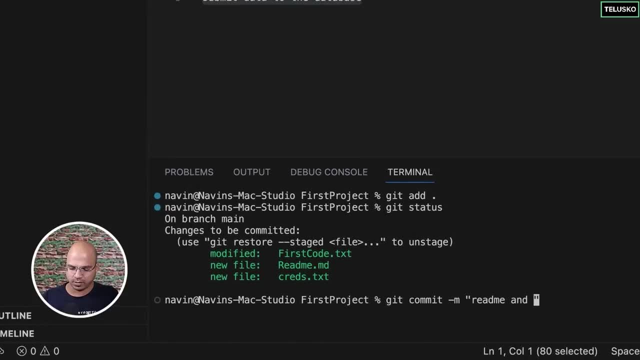 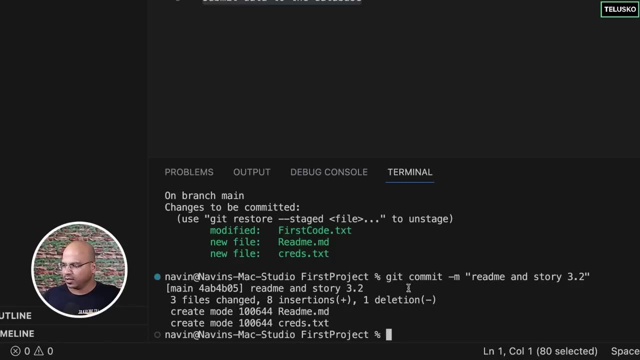 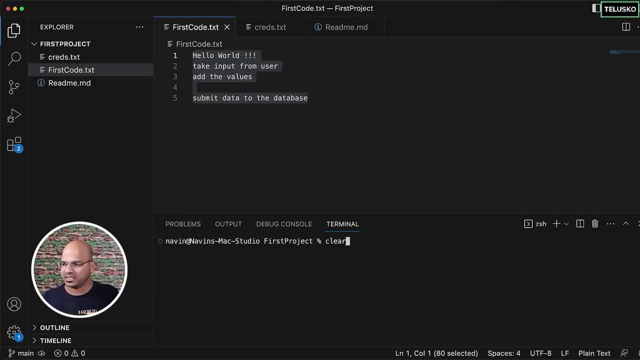 the message you can say readme and story 3.2. okay, so let's say i'm adding this three and then you can see we got the files in the database now. but basically your git database. now if i say git status, what happens? if i say get status, it says everything is clean, nothing to commit. and now 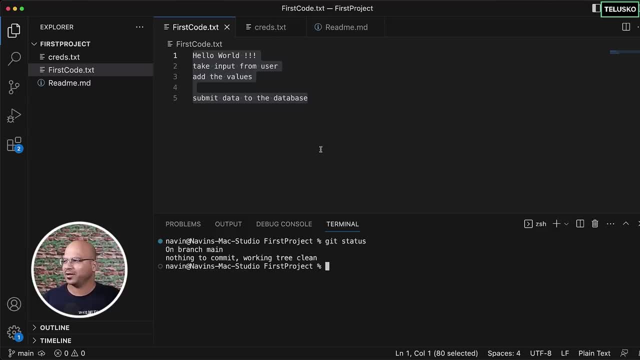 it's been tracked in the git repository. that's cool, right, but then the thing is, i will now, after working for, let's say, a few hours, i will decide to push this to the github repository or some public repository. now, at that point, what happens is everyone can see my username password. 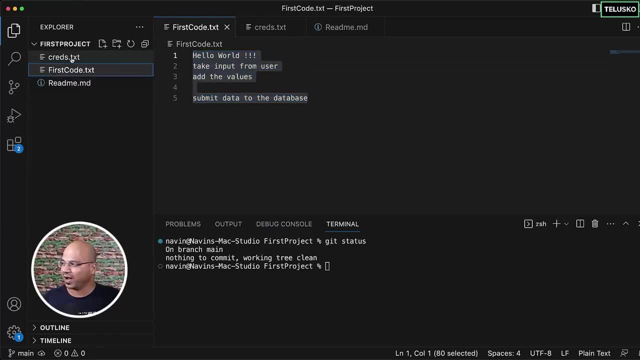 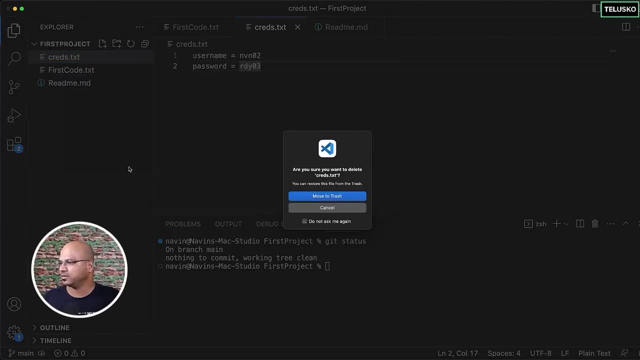 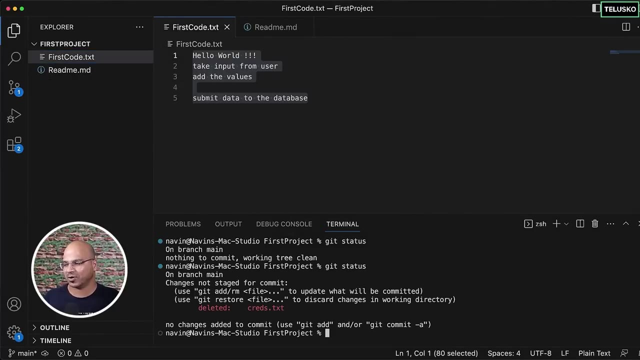 i don't want it. basically i don't want this file to be there in my git. one way you can do that: you can just right click here and you can say delete, move to trash and done you're done, job is done. but the problem is if you say git status, it's already there. it says it is deleted. 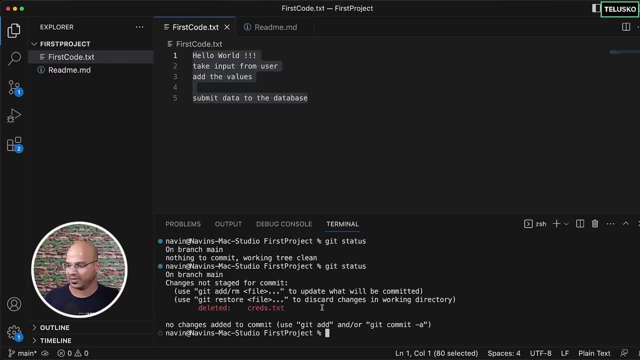 but it is deleted from your working directory, not from your git, right. so one thing you can do is you can say: but if you do git commit, that's, that's tricky now, right. so what was the idea here is: don't delete it from here. once i get status, everything is clean, don't delete from your. 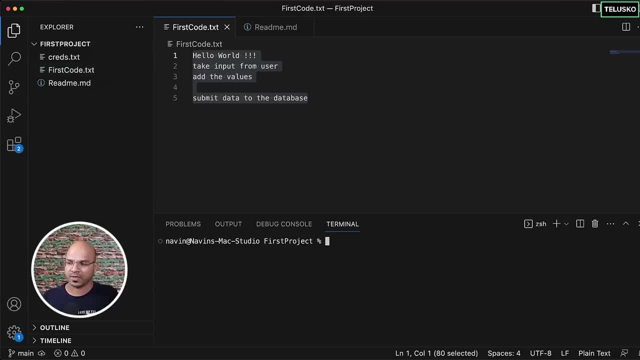 working directory. you have to delete from first from the git, and the way you can do that is by saying git rm. that's the command you have to use, and then you have to mention that it is basically cached. so we have to say cached and then mention the file name, which is: 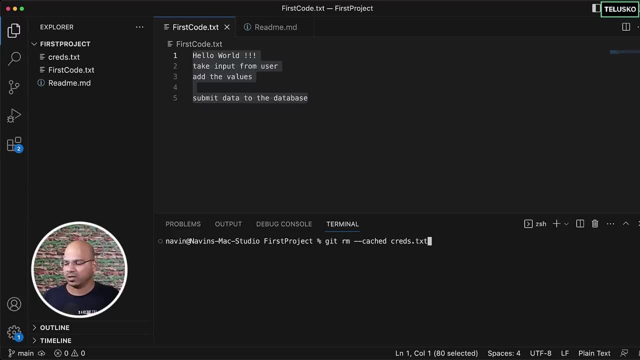 creds dot txt. now when you say enter, it says removed and you can see: now it is untracked. so basically, first you have to delete your file from the git, now it is untracked and you can happily delete. now delete moved and now you can say get status. 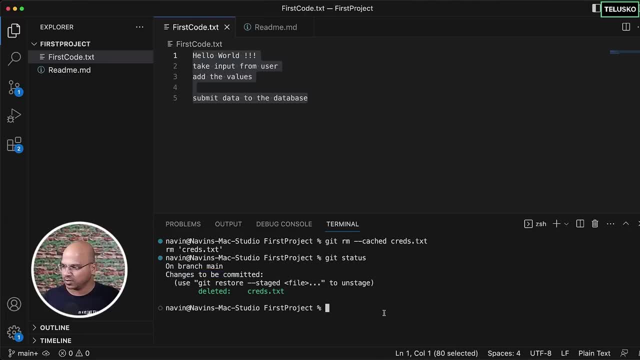 everything is cool. you can say changes to the changes to be committed. so i will simply say: git commit hyphen m- remove the credits. fine, and done so. now you can see we don't have anything here and we don't have anything in the git, and that's how, basically, you can safeguard yourself. 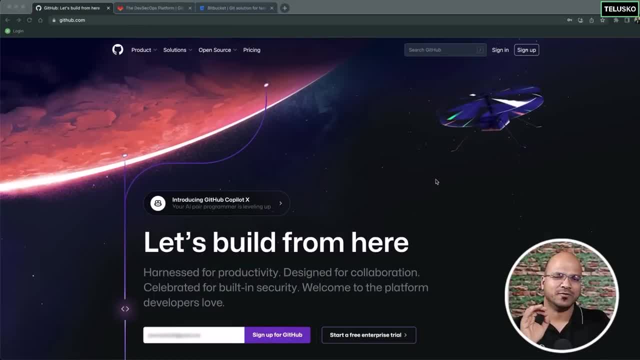 from your unexpected file uploads. now, if you remember, when we talked about git, we have mentioned there are different types of repositories. right now, basically when you can have git tool, which is a built-in version control system, you have a commit history in your machine, right. and then, of course, 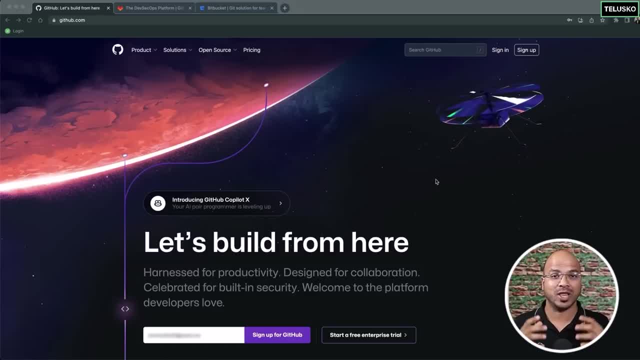 you can jump between the commits, but what if you want to collaborate with everyone? so let's say you are working in a team and then they are working on some feature. you are working in some feature, how will you collaborate? and that's where we have to use something called a remote repository. 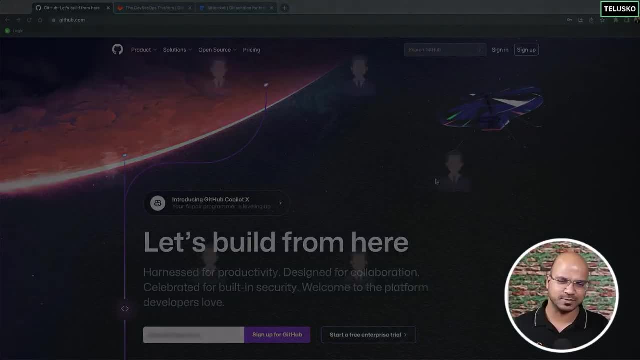 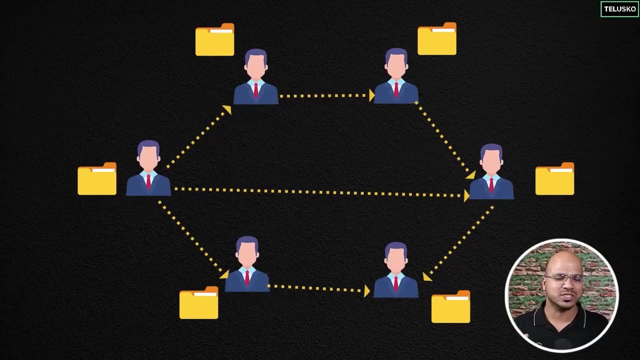 now, what is a remote repository? so, example: let's say we have six people in the team, they have their own machine, they have a local copy or local repository. and now if you want to share, we need to use some remote repository, some server which will be public, so that they can fetch. 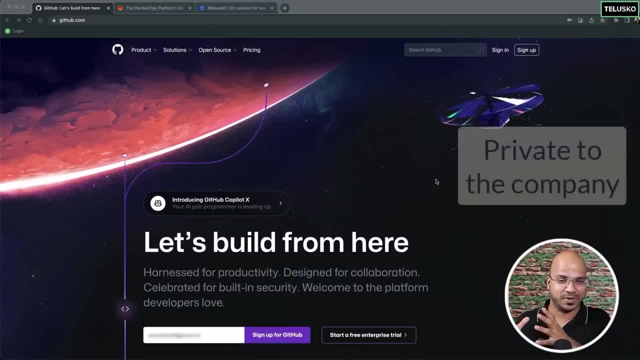 and they can do something. of course, this can be a private to the company, or this can be public so that you can access it from anywhere. but let's say at this point, let's talk about public, because we are not working for any organization. where the security is most important, we are learning git. 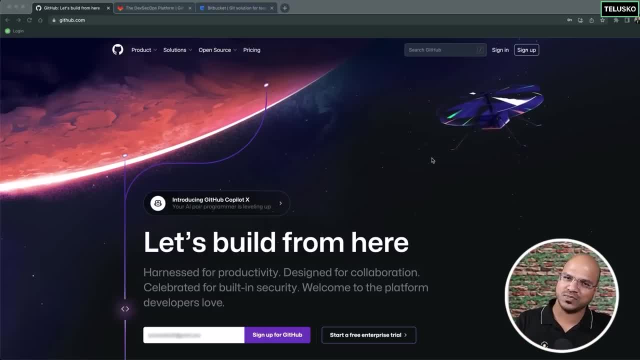 right, so let's talk about the public here now. there are different options. we have, in fact, the options which are talking about. they also provide you something called private again. we'll see those options there. okay, so we have three options here. there might be multiple repositories, but, or multiple remote repository options, but here, uh, the most famous is github. 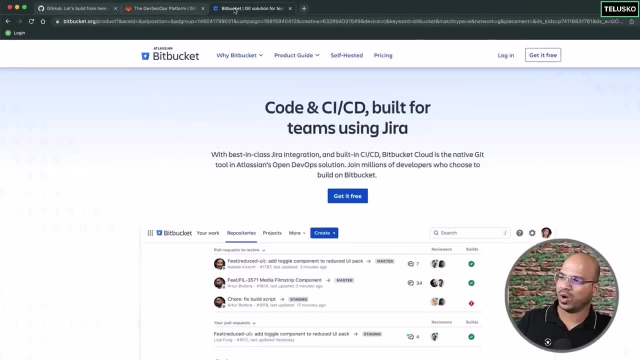 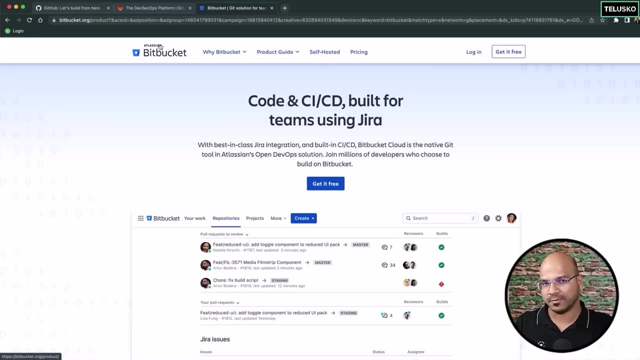 then we have git lab. the second one and then third one is bitbucket. now bitbucket is given by atlassian, which is a very famous company. they provide different tools for the developers, so you can use this and few companies are using it. most of the companies who want to use the private 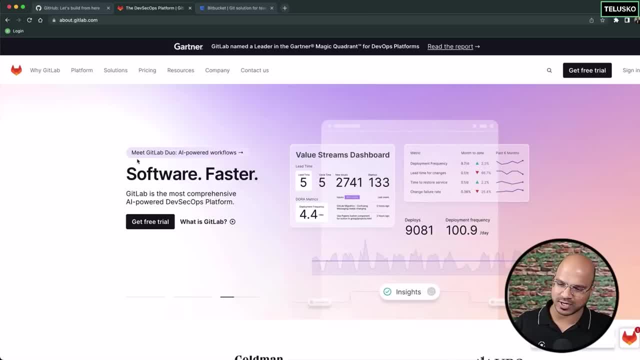 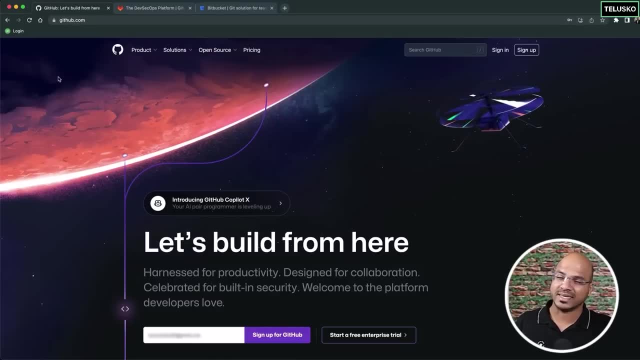 features, the paid private features are using the private features and they are using the private features. they can use git lab or they are using git lab basically. and then for the public- for the normal people or for the public- we have something called github. now github also helps you to create. 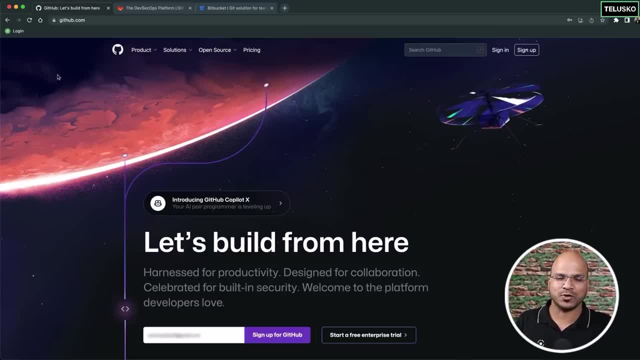 your own profile and that's why, if you go for the interviews or if you talk to people, they will say: hey, give me a github profile. it's not like you can't work on git lab or bitbucket, it's just that github is very famous among a normal public, so we are going to use github here, of course you. 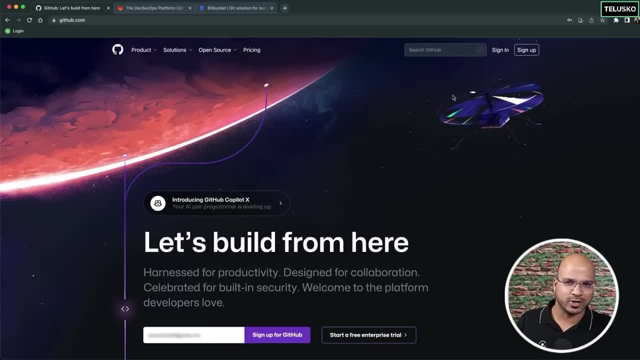 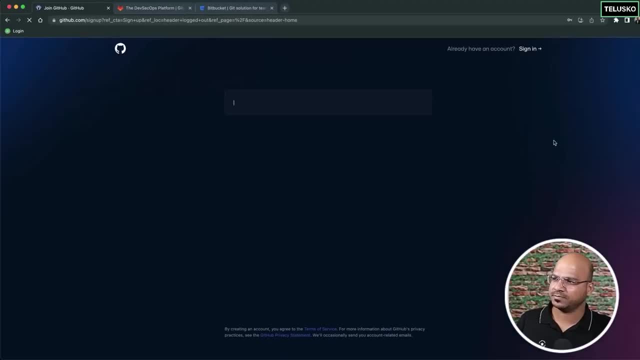 can switch to any repository, your choice. but let's talk about github now. first of all, you're going to get on with uh, just first of all, you need to have your account on github, okay. so how do i get that? it's very simple: click on sign up, enter details here, whatever email you have, and you can log in once you are signed up. 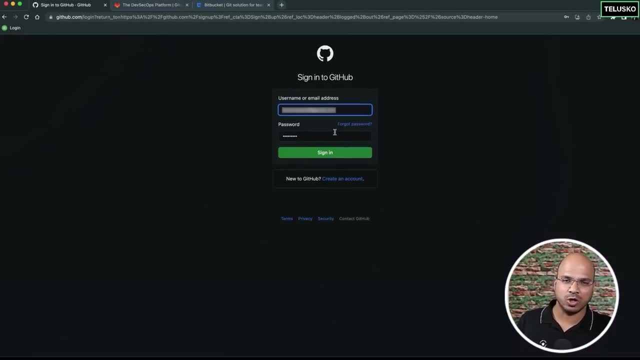 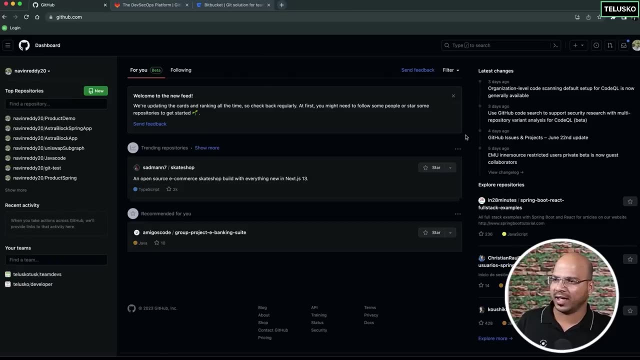 you have to also make sure that you're logged in, and let me just do the login first, and i'm just hiding my email id there so that we can keep it privacy. and here we go. so i'm trying to log in and that's my github repository. okay, so i have a lot of repositories here, because when i teach 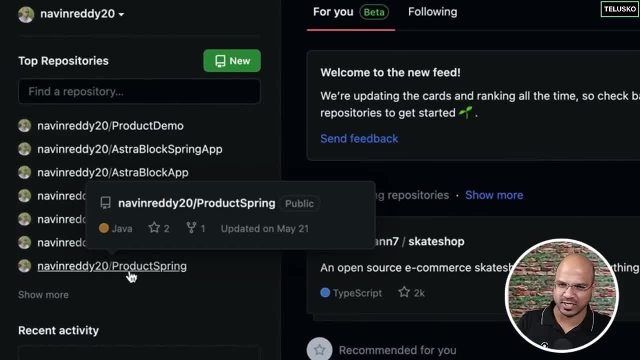 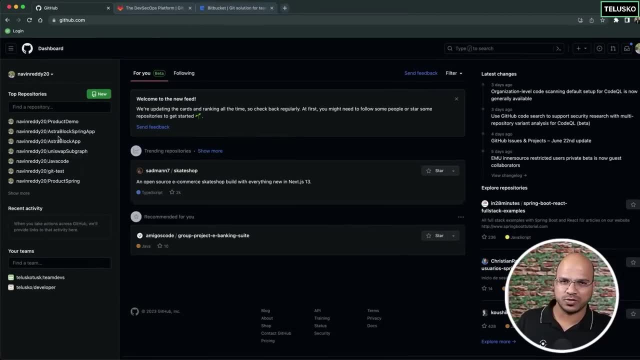 something. i also push that code on github so that you can see, and you can see all the repositories here. there might be some private repositories which you cannot see, but that's how it is okay. so we have some repositories here now what if you want to create one now? first of all, how we can use. 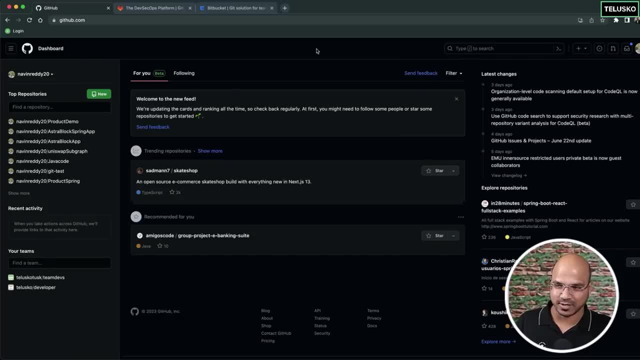 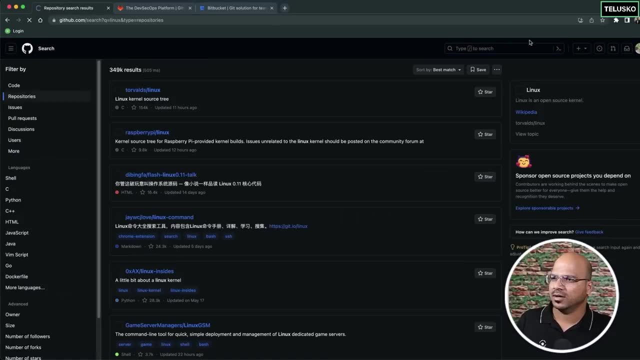 github. it's very easy. let's say, if you want to search a particular project, so what you can do is you can search for something. example, let's say i want to search for linux kernel, which is a very famous repository. so you can see, this is linux, the linux kernel, which is a very famous repository. 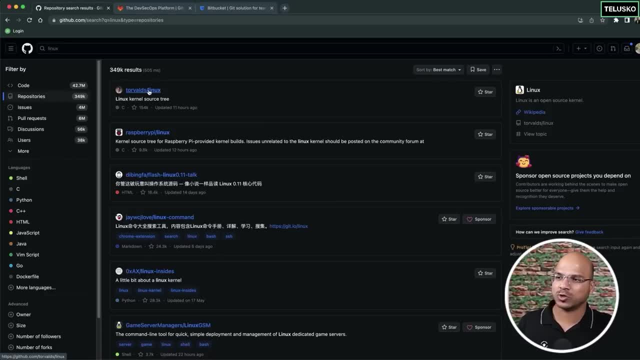 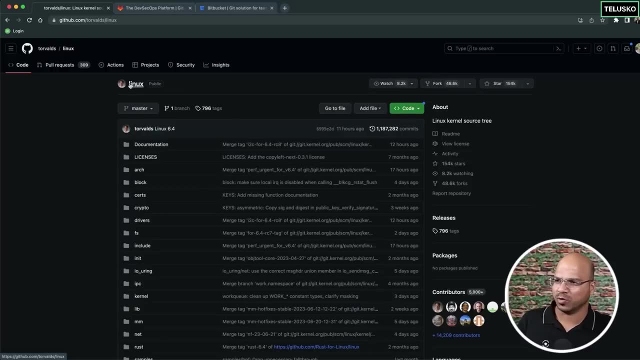 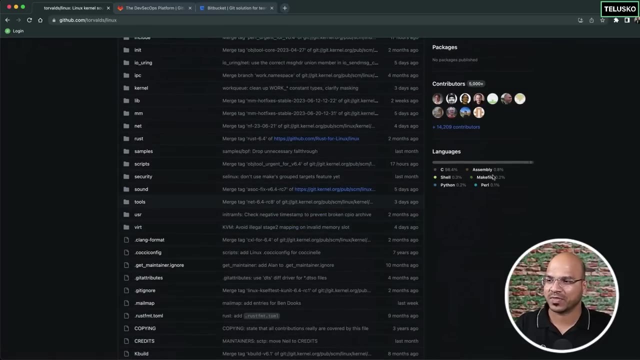 we use. it is open source and the entire source code is available here now. the owner of this is linus, which is linux torwald. everyone knows it right, so you can see, this is the entire code of linux and you can get this on your machine. okay, it's very easily. now it also analyzes the entire 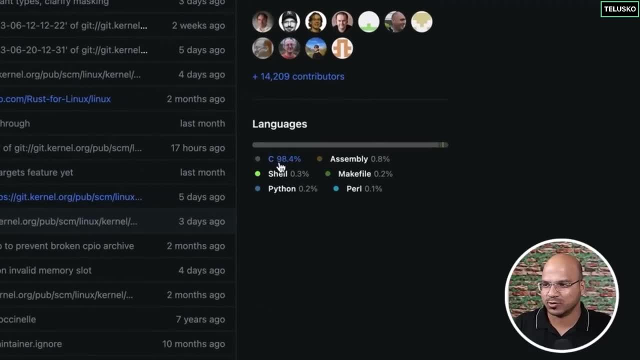 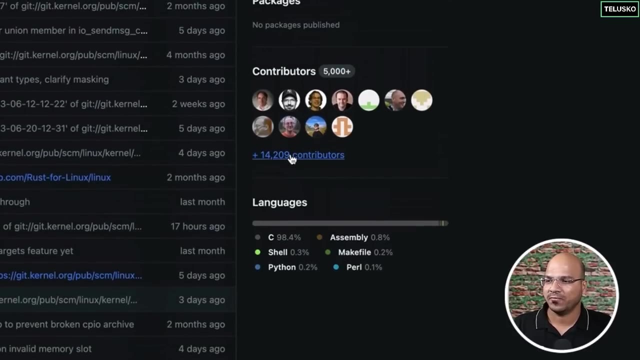 code base. it will tell you which languages it has used. so you can see: 98.4 percent of this code is some shell script, some python script and makefile. so these are the languages they have used. contributors: you can see more than 14 000 contributors we have for linux and you can see these are the some options. so at this point, 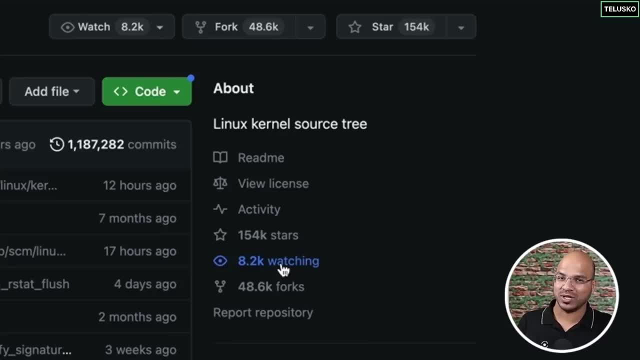 when i'm recording this video, there are 8 000. more than 8 000 people are on this page, okay, so that's interesting. everyone want to look at the code and they might want to modify it or they want to add some new features. so basically for the 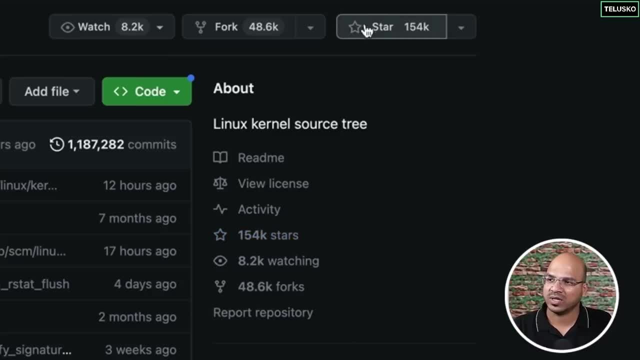 project. you can also give stars. example, if you like this project, you can give a star here. or when you create a project, people can give you star, and that's how you become a good github star. otherwise, or you can pay some amount. okay, i'm just kidding. so so let's say, we also have option. 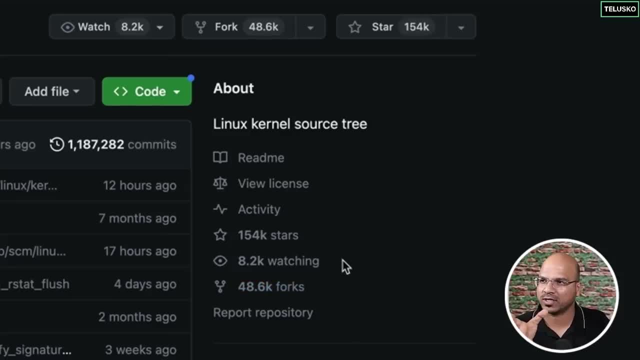 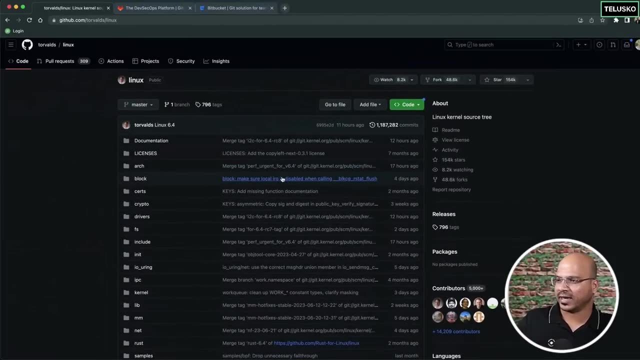 of forks here now. example: we'll talk about what is fork later. and this is 48 000 forks already happened here now. this is the entire source code. i can get this code on my machine. it's very simple. you can click on this code and you can click on the source code and you can get the source code. 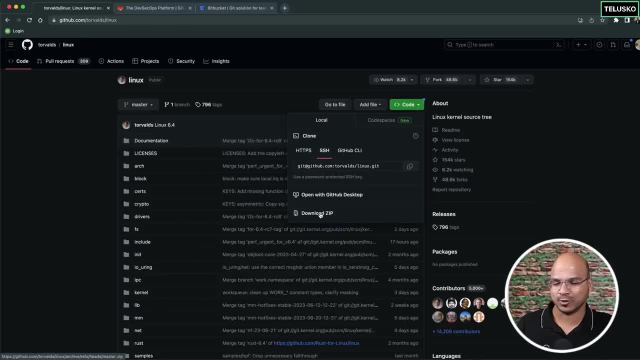 on download, zip okay, and you will get the entire source code, but we are not going to do that. options: we have two options here, which is https and ssh. we are going to do this, but how will you use this? it's very simple. now, when you have this project, what you can do is- or for this even to 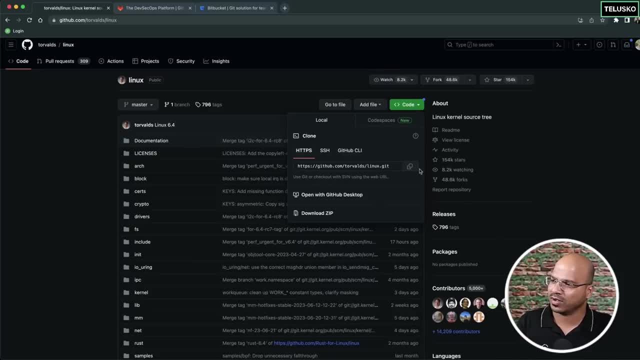 browse this. you don't need a github account. i'm uh, if i'm not wrong, uh, you can get this. you can simply copy this, okay, so you can copy the link, okay. first of all, we have mentioned the option right download, zip. that's one option. second is: you can copy the link and you can copy the link. 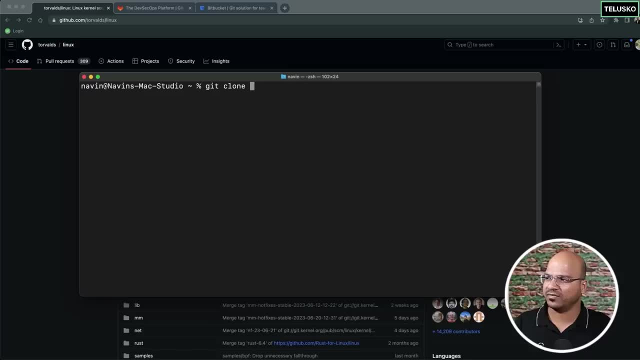 to your terminal and here you can come pass a command which is git clone. now, clone is basically copying something, right? so you have a code in the repository and now you want to copy it. so you can say git clone and you can mention the address, and the moment you say enter, it will copy. 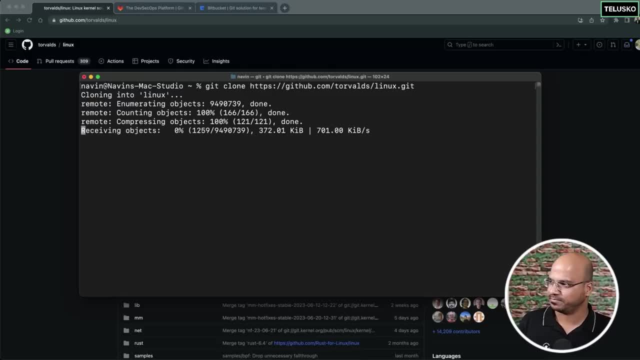 the entire linux source code on my machine so you can see it is downloading. it will take a lot of time because i think it's it's heavy. i've never tried it, or maybe i've tried it before but never completed the entire download. you can see, even with this speed, only two percent completed and 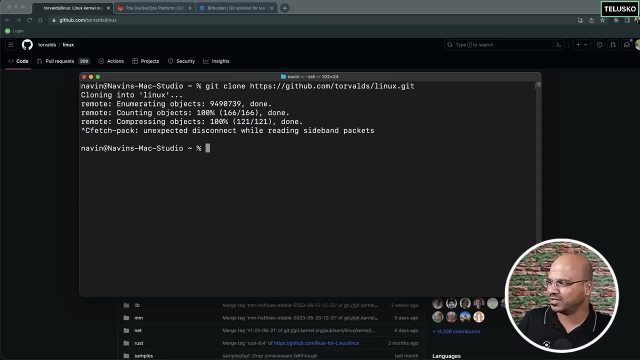 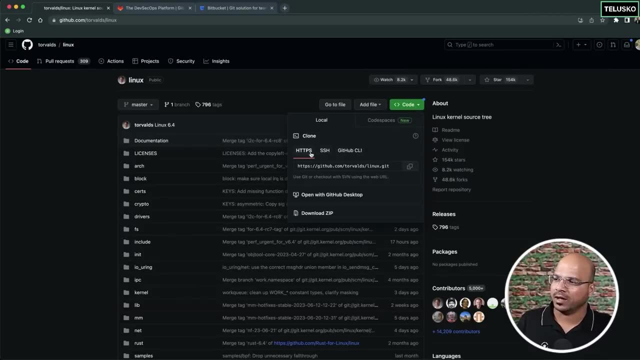 that's the entire size. so i don't want to do this. i will just cancel this. okay, i don't want to download the entire stuff. i just wanted to show you how do you get it. okay, so that's how you can copy. uh, there are different options here. we have https and then we have ssh. okay, so we'll see. 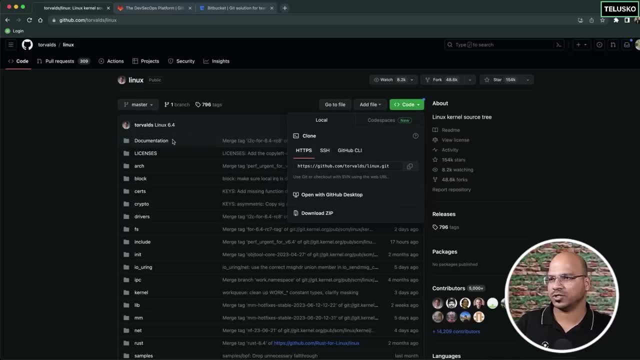 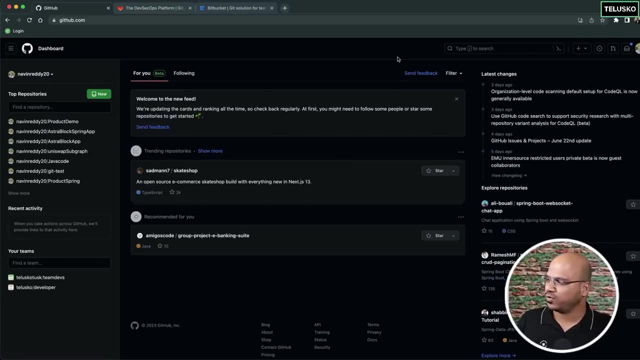 later. how do we use this? but at this point you can see we have some repositories, but what if you want to create your own repository? it's very simple. let me just increase the font a bit. yeah, so, if you can see, there is an option of plus button. so 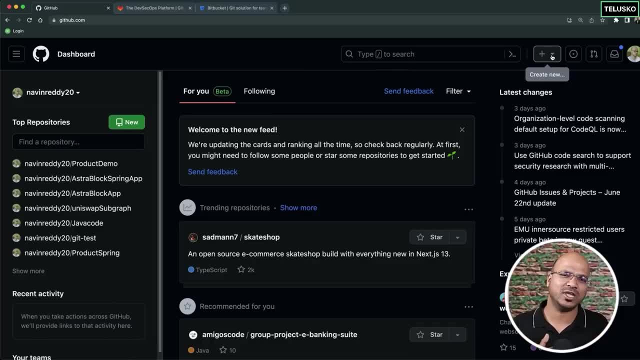 i want to create my own repository. we have done that for the local machine, right? so when you say git init, it creates a local repository in your machine. now i want to create a remote repository. for that you just have to click here and click on new repository. click on that. 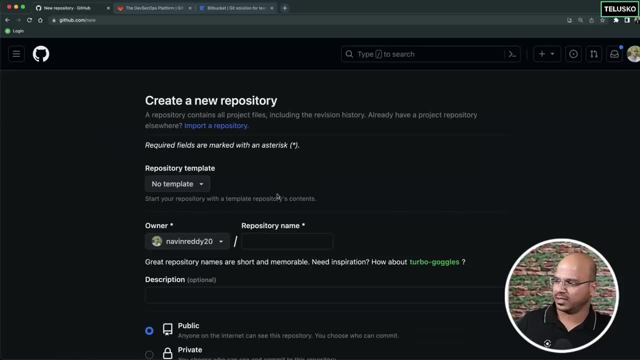 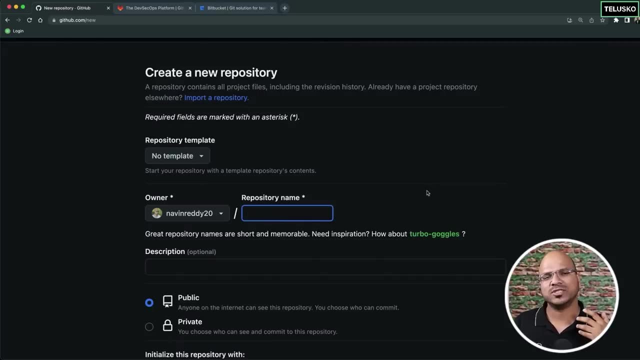 okay, just creating. yeah, now this is the page you will get. now that's my id- github id- and this is my repository name, so let's give a name to it. of course, the repository should have a good name, and we have done that for our own machine as well. right example, when we were doing vs code. 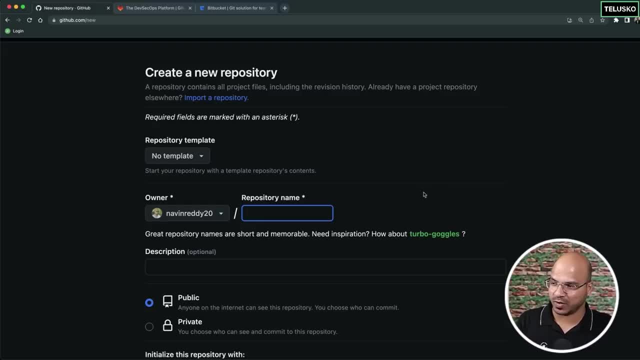 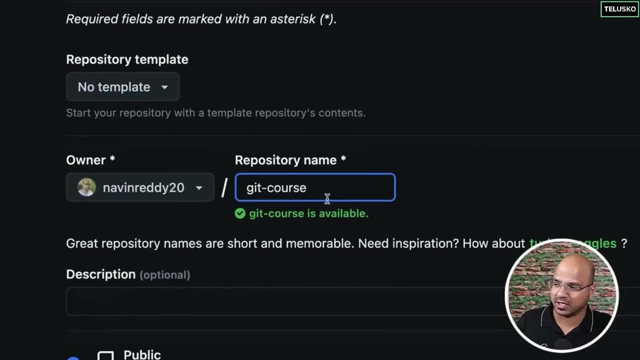 remember we created a project and that was your repository name as well. here let me create something. so i will say git course, because that's what we are doing and it is available. so again, this is not publicly checked, it will just check. do we have in my account? so i don't have this name. 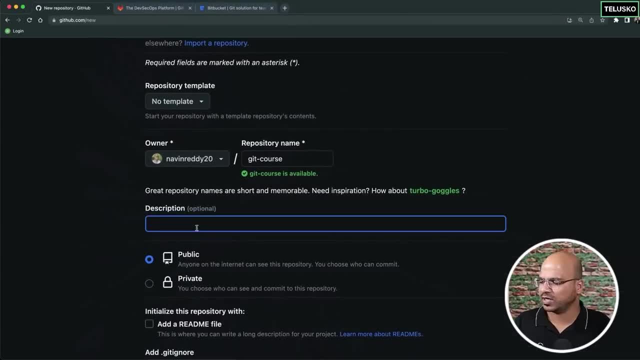 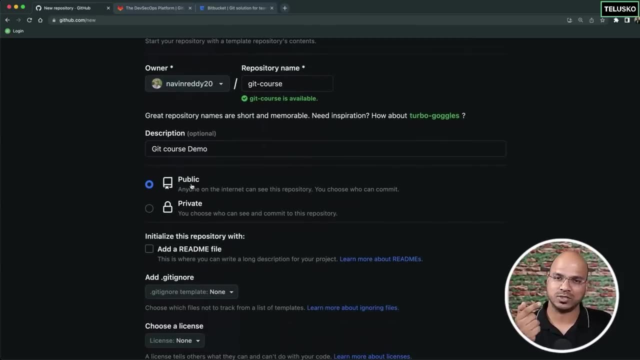 in my account so i can use it. you can give a particular description here so you can say git, course, demo, and then you can make your repository public or private. now linux- we were able to search it because it was a public repository. now let's say, if you're, 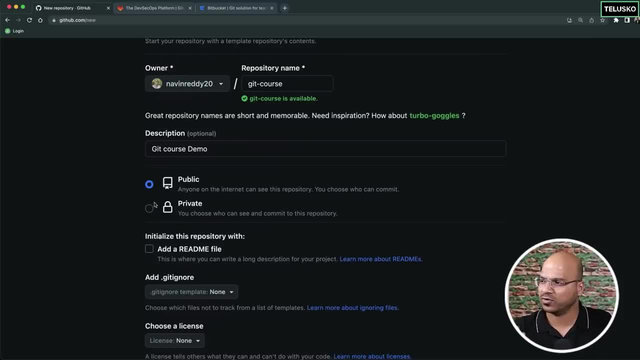 working on a project and you don't want to share the code with the entire world. of course, at that place you will be using a private one. so of course you can share the link with your friends- or not for the friends, but with your colleagues- and then you can work on it. public, anyone can search on. 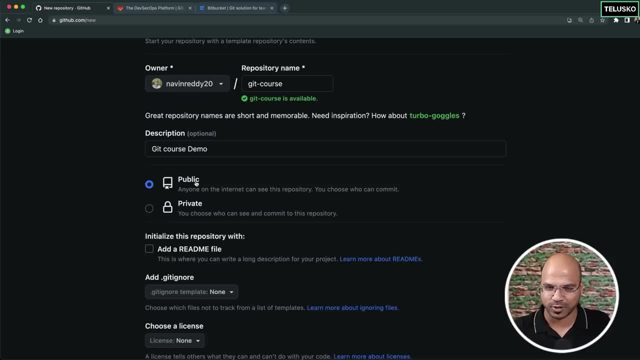 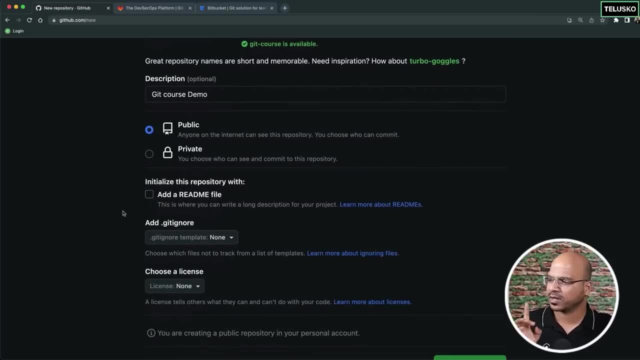 github. so for this i will keep it public, so that you can also see the repository later when you're working on a project, and then you can also add a readme file. so at this point i will not do that. now. readme file is important is because let's say, if you have built a project and if you want, 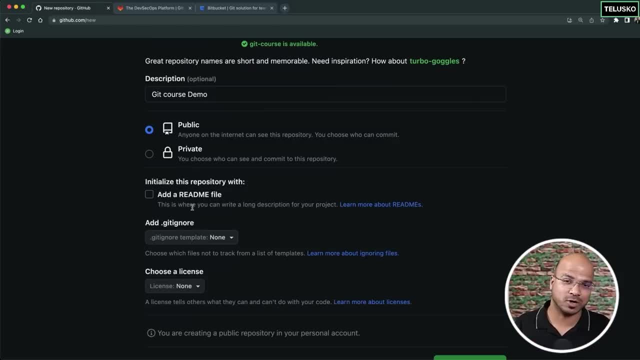 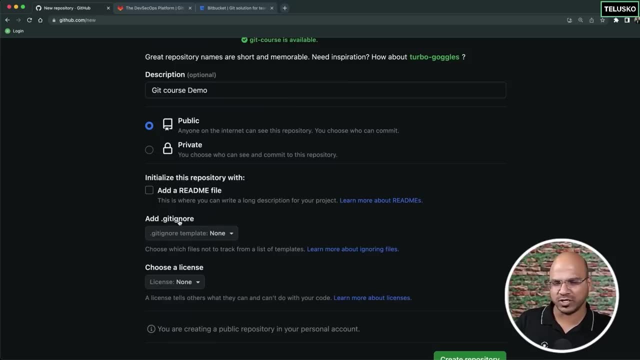 to mention some steps. what is this project? how do you run this project? how do you contribute? so all these things you can mention in the readme file, but at this point i don't want to add it. there's also option of git ignore, which we'll see later, and then you can choose a license. there are 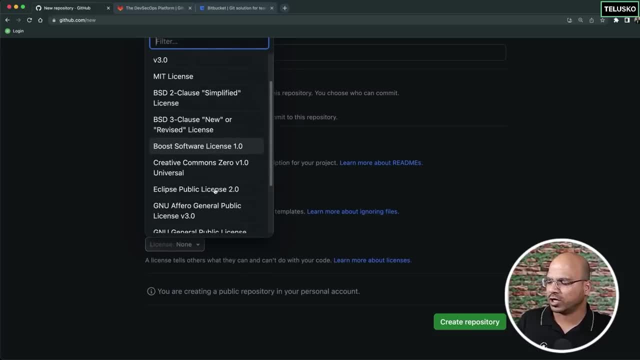 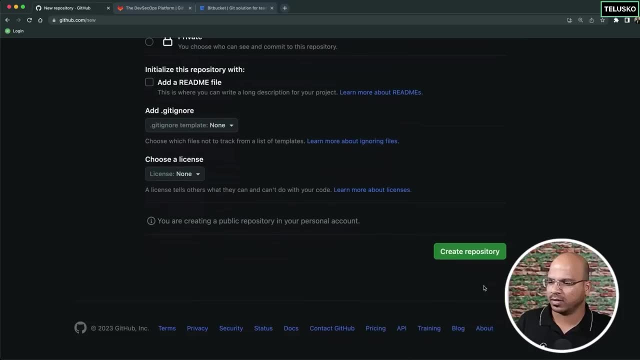 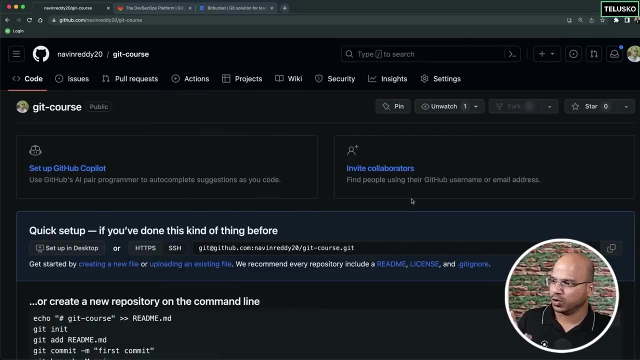 different licensing option here. if you want to keep it open source and if you want anyone to use things at this point, i will not choose any license and click on create repository and done so. you can see you got your repository here. now, when i'm recording this video, there's 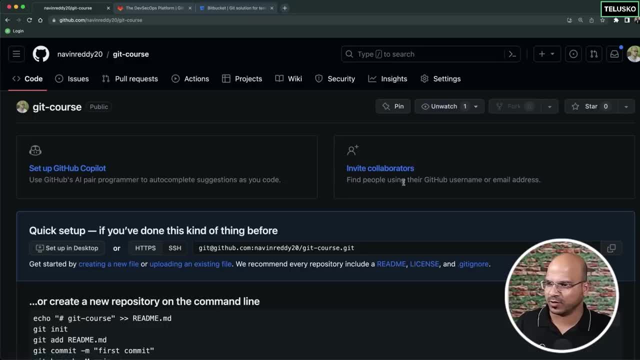 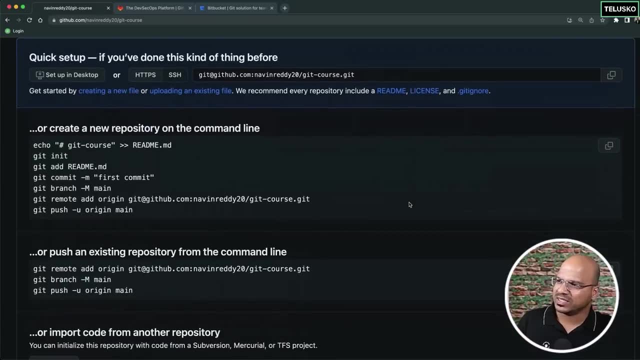 option of go pilot for ai programming and i will not be using that. also, i can invite collaborators at this point. i don't want to do that. just scroll down and you will see all these steps now. first of all, certain things, which is very important. you can see a. 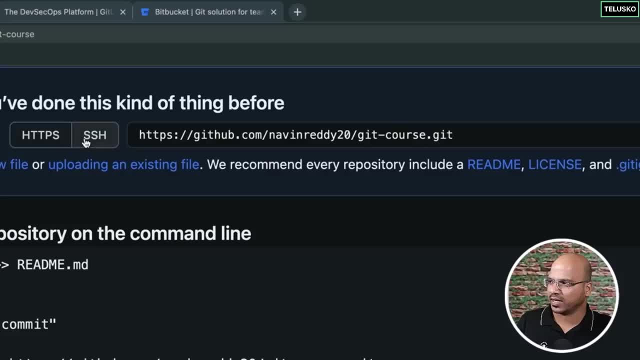 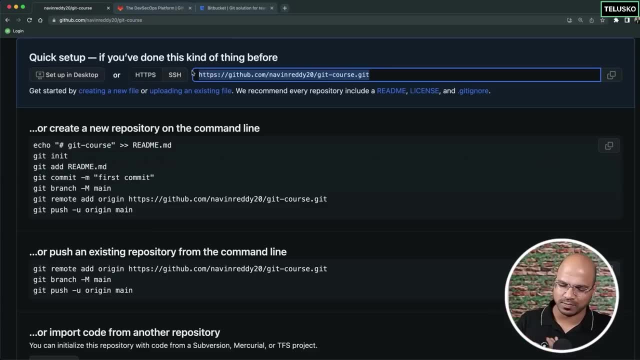 link here now. this link will change based on where you are clicking. so if you're clicking in https, this is what you will get, and most of the time, when you're downloading url or some repository, you will use https, but we will use ssh, so the advantage is. 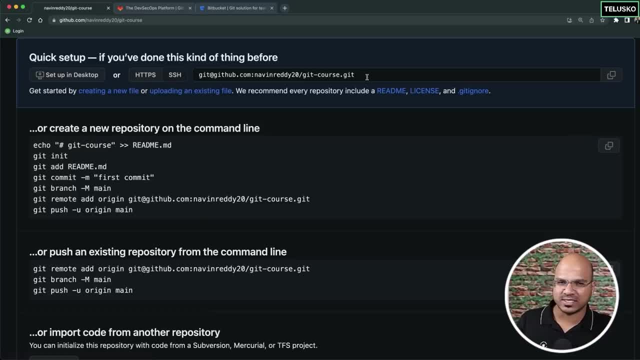 okay, let's talk about this advantage later, in some time. so let's say, we got this link here. just try to remember: we get, we do get a link, a unique link for your repository. this is unique. now, how do you create, how do we work with this repository? now one thing to remember. 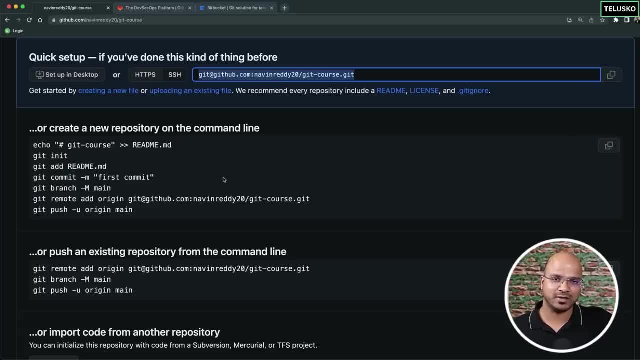 we have a github repository which is on the internet somewhere- i don't know where it is, and then i have a local repository. what if i want to make some changes? how do i do that? how do i push the code from my machine to the local repository or to the remote repository? now to 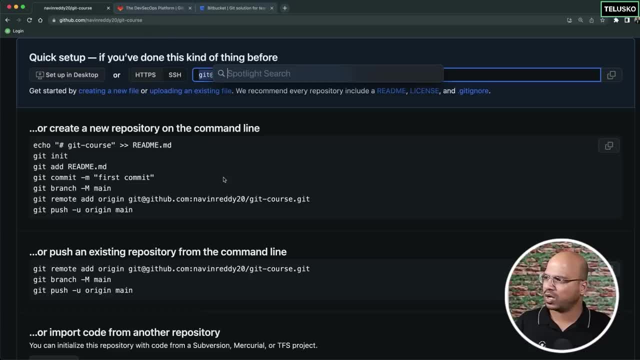 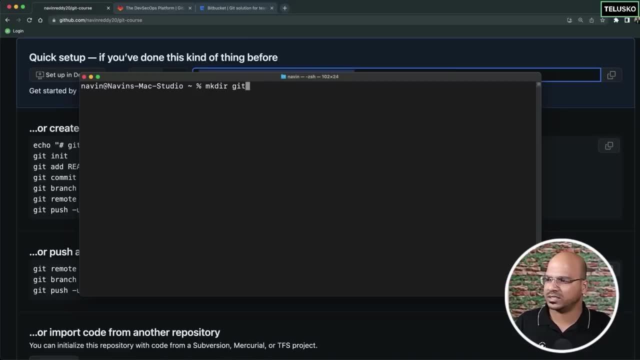 do that. what i will do is i will open my terminal. so my terminal was already opened, it's clean. first of all, let me create a folder here and let me name this folder as git course- okay, same name, but with my remote repository- and then i will jump into this particular folder, the git course, and i will 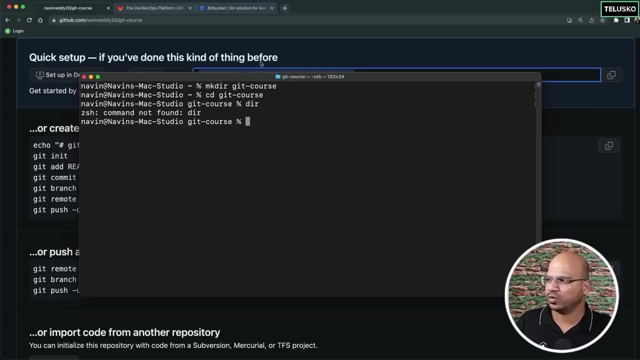 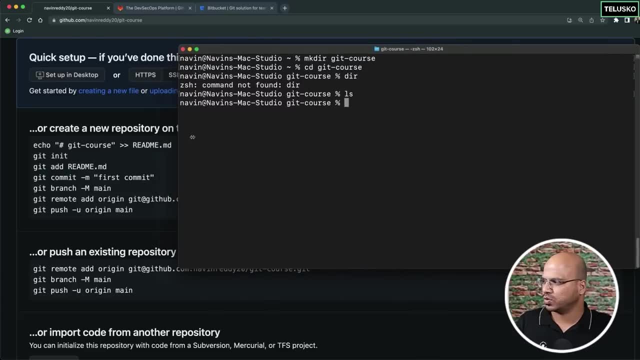 say i will check. do we have any folder here? you can see i don't have any files or folders. okay, first of all, i'm into mac, so ls, there's no folder. that's cool. now what i'll do is i want to create some files now. first of all, we don't have any file. let me create one file now. it can be any file. 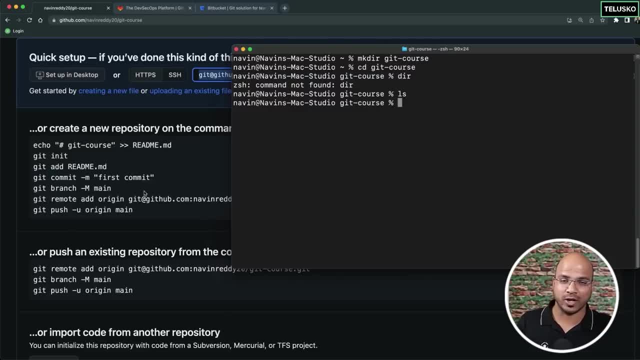 okay, and you can simply follow these steps here to do that. i want to push one file from my local repository to the remote repository and you can simply copy, paste and run. it will work, but let's try it one by one, just to understand how it works. so the first thing that we do is we will be using: we. 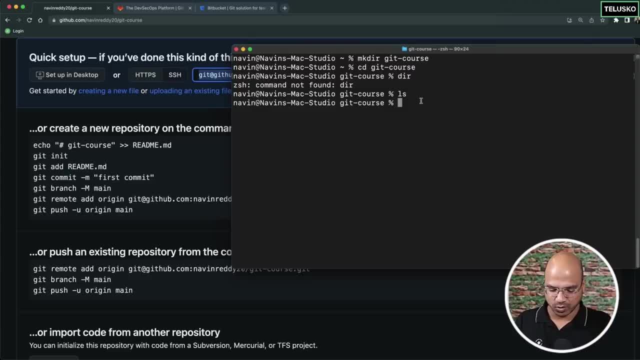 will be creating a file which is readme file. remember we have talked about readme. so to do that i will say echo and i will push some data here so i can say git course, demo and i can type multiple lines of data here. but let's say we have single line and then i want to create a file. 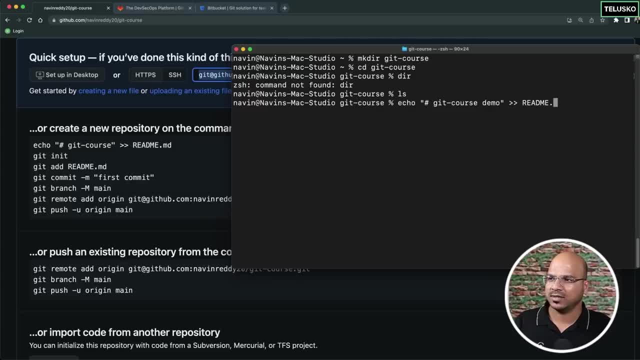 called readme. so basically this is a command. echo is a command using which you can echo this message to this particular file, so we will say readmemd. now md is basically stands for markdown. if you want to design some readme file and it should look good, so you can use something called markdown. okay, 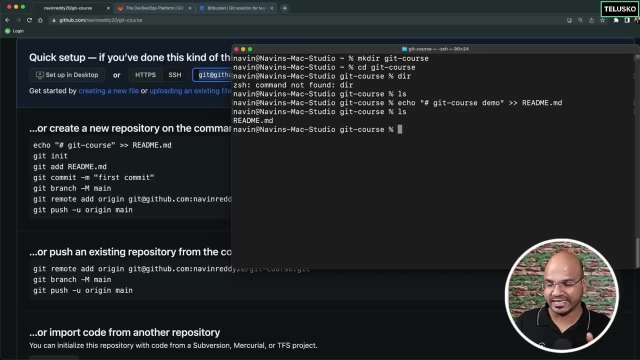 and you can see. if i say ls, now we got a file created and if you want to see the content of that file, you can say readmemd and you can see. this is the content. so using cat command, i can just see the content. so i do have a content now. so ls, we got a file. the next thing that we do is: 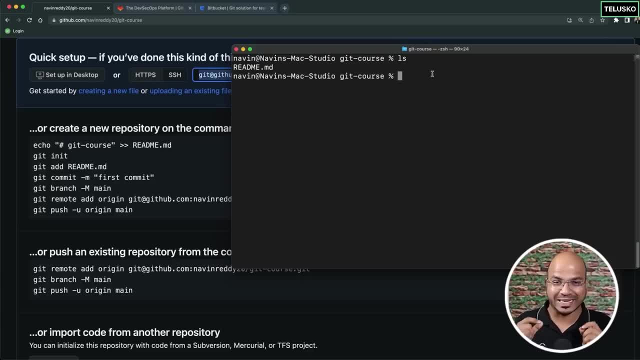 we need to create a git repository, the local copy, okay, the local git, which is not done yet because we got a folder but it's not git enabled. so to do that, i will say git init and we can follow the steps, or otherwise. we can also create a branch name because by default it will create master. 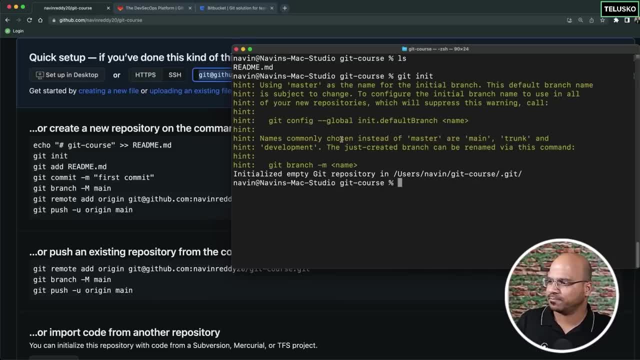 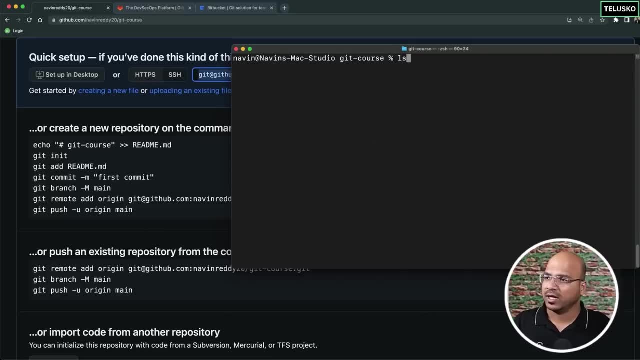 right, we don't want master, we want main, but let's follow the same steps. so you can see it has been created and that's done. so let me clear this. we got a repository as well. if i say ls, you can see we got. we should have got the folder. i think it's hidden. so yeah, so you can see we got a folder. 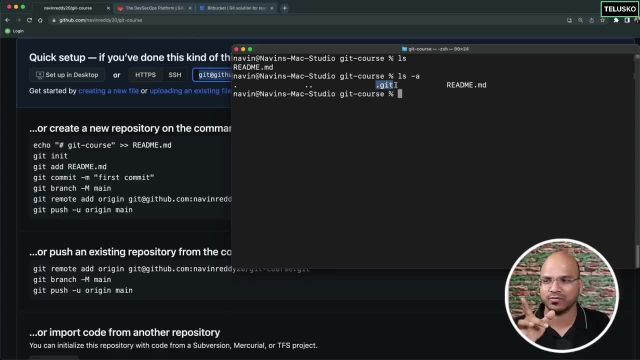 here, which is dot git now. this is where it will have all the folders which we have talked about before. so this is done. the next step is we need to add, because if you say git status, now we got a file, but that is not a part, so it is a untracked. remember, we have a working copy. then we have to. 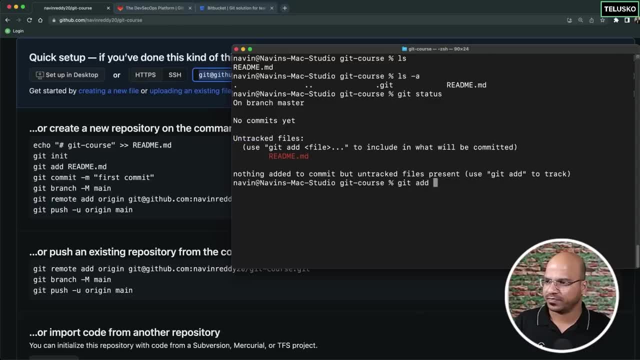 stage it now. how do we stage it? we have done that before. say git add, read me, dot md. so now we have staged it. now, after staging, if you say git status, you can see we got a new file and this will be committed now. now how do we commit? it's very simple, you will. 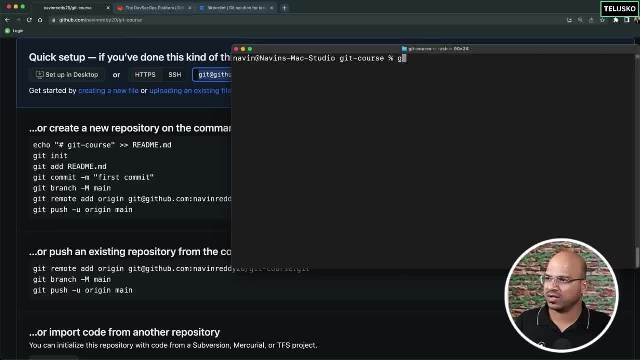 say git. okay, i'm just trying to copy the code from here. okay, so on the left hand side you can see we have the code or the commands. we'll say git, commit. we'll mention hyphen m for the message, and here i will say first: commit, enter. 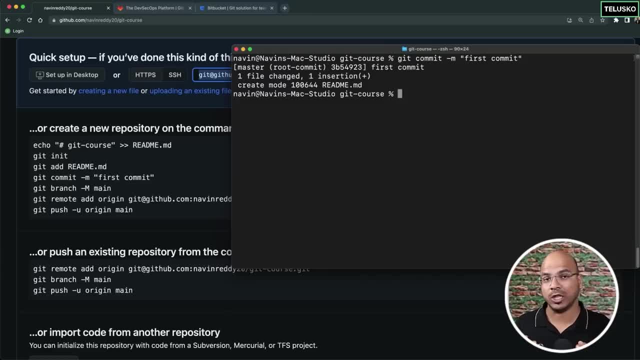 so that's my first commit, right, but again this commit is happening in my local machine, so that's done. next we have to create a branch. so i will say: git branch. okay. now why do we have to get a branch here? the thing is by default. we got a master branch. 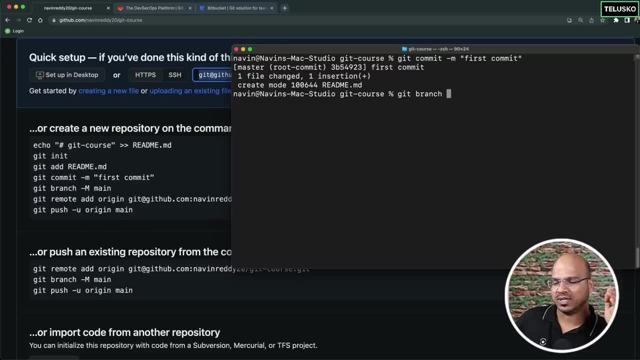 right, and we have mentioned before, let's not use master, let's use something called main, and that's what github is also promoting. so i will say: main, enter, and you can see. now we got a main branch. okay, now, once you got a main branch, what next? it's time to connect to the remote. 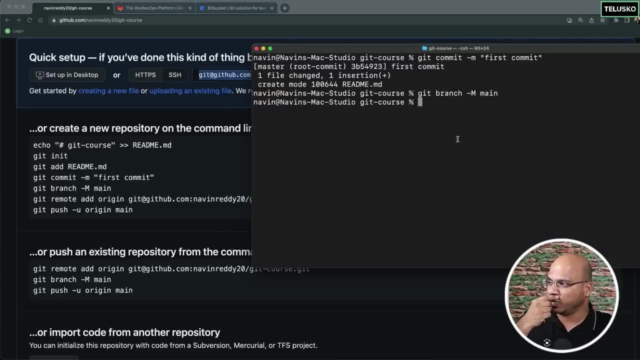 repository. now this is a local repository. we need to create a remote repository, but the problem is: how will you connect your local repository to the remote repository? now? that's a big issue. so we have to set something called an ssh. now how do i do that now? basically, there are two options. 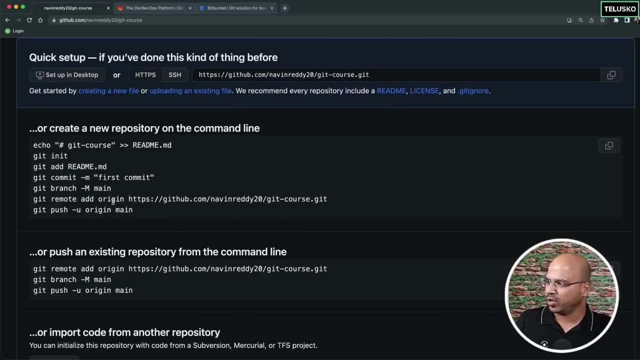 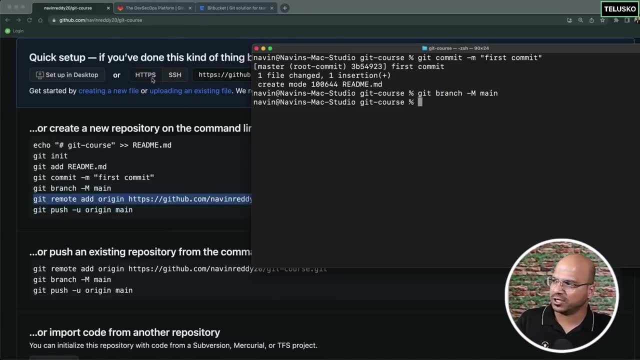 one is https. you can also get these steps here and you can see something is changing here if i click on ssh, things are changing the advantage of using. so, first of all, when we use https, basically anyone can push. right, this is my remote repository, you can also push. how do i know? 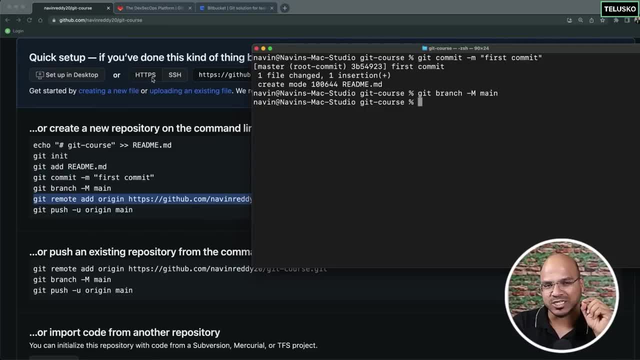 that who should, who should be allowed. now that's where, when we use https it, it will ask you to log in. so if you are saying you are naveen, how do you prove yourself? so you have to log in, otherwise you can use ssh. the problem with login is you have to log in every time. what if you can just 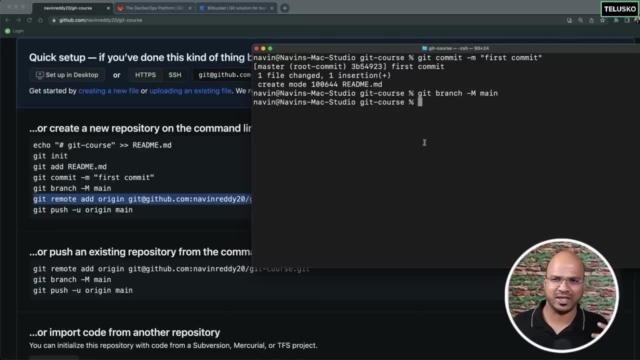 set up your machine once with a key and then, every time you do something, it will automatically detect who you are, and that's why you have to set up the ssh now, the way you can do that is by you using very simple thing, which is ssh keygen hyphen. oh, this is the command we have to use: ssh. 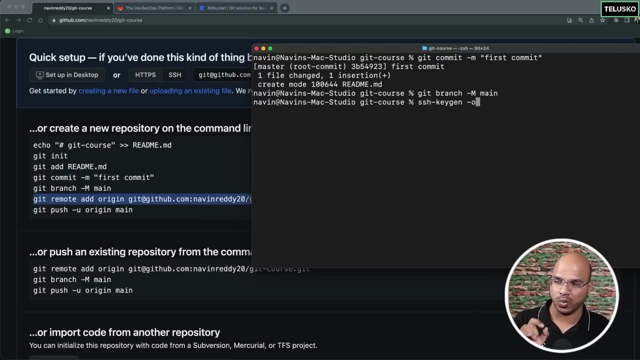 hyphen keygen space hyphen. oh, now, this is the only time you have to do it. okay, you have to do it only once. it's not like for everything, you have to do it for one machine, you have to do it only once. okay, i just messed up there. so say: ssh keygen hyphen o enter and you can see. now it says: 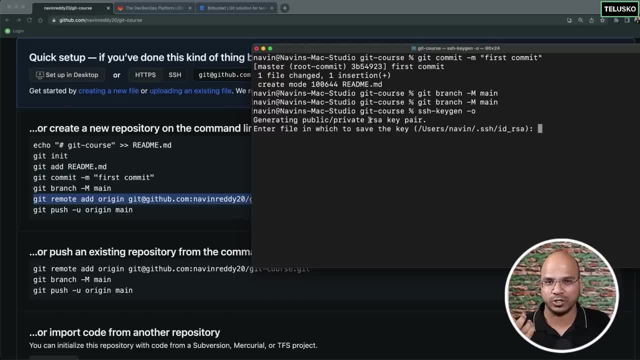 generating a public and private key. basically that's how you get a key to communicate between client- i mean your local copy- and the server. so it says: enter the file name in which the file will be stored. i don't want to mention anything here. it will go for a default name. i will say enter. 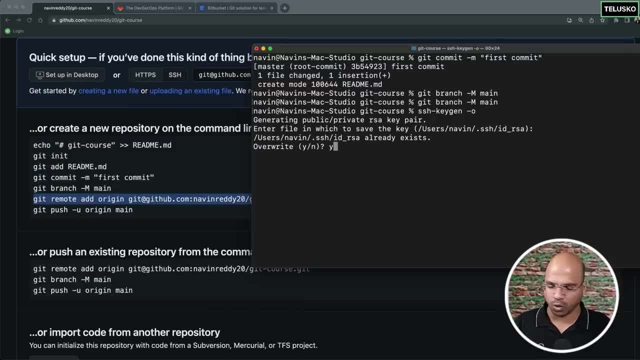 oh, the thing is in my machine already have this created. i will just overwrite. i will say: yes, you will not get this option. if you don't, if you have not done this setup before, then it will ask you for a passphrase. i don't want to mention any passphrase, it's like a password enter. don't want. 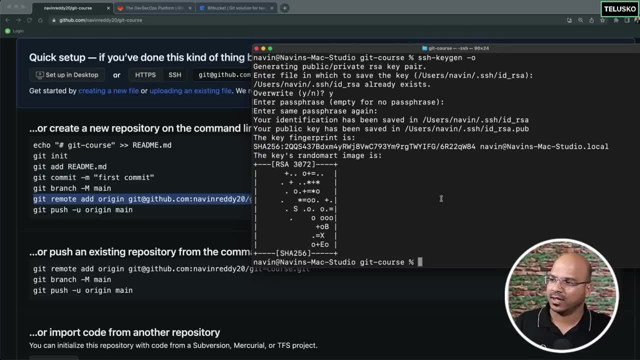 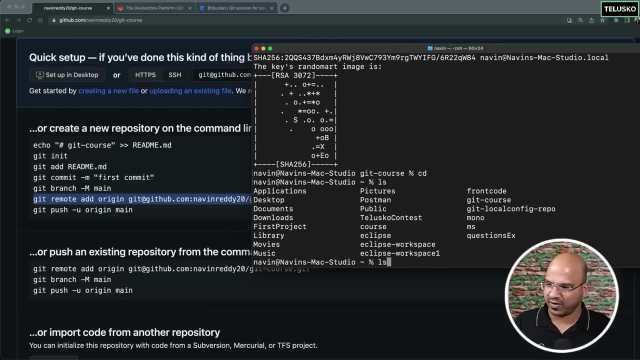 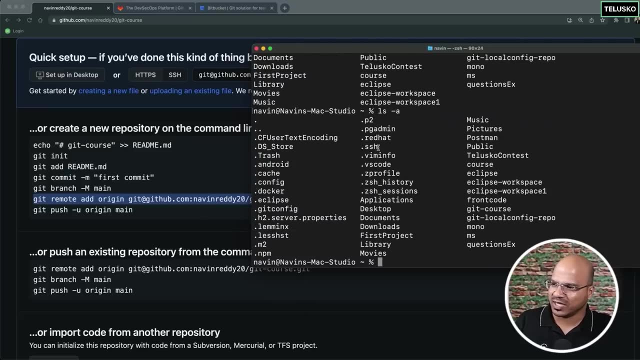 to mention anything and done. i got my file created. now, where will i find this file? what i will do is i will go back to my folder and if i say ls, in fact ls- hyphen a- okay, first of all, we got ssh created. this is not the ssh. okay, let's see the ssh way it is. so, if you can see, this is the folder which we. 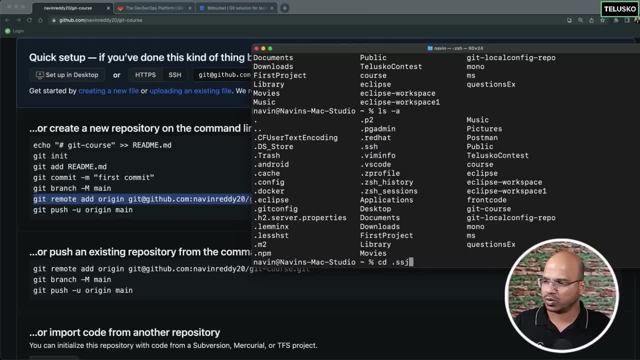 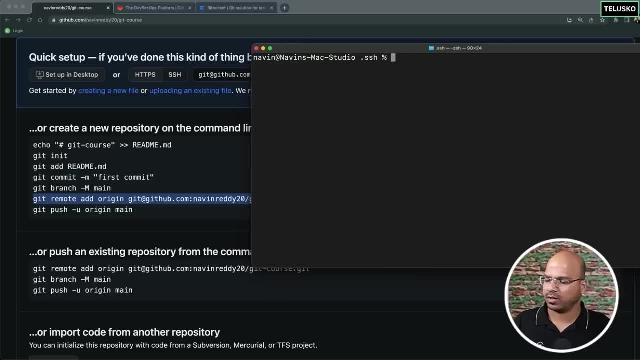 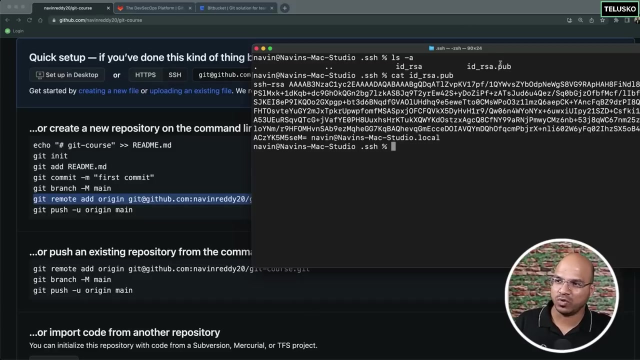 are concerned about. this is where it went, so i will just go to that folder using cd space, dot ssh enter. let me just clear the screen and now if i say ls, hyphen a, you can see we got our publish here. let me open that. so i will say cat id dot pub and we got the key right. this is where you will find your key in the 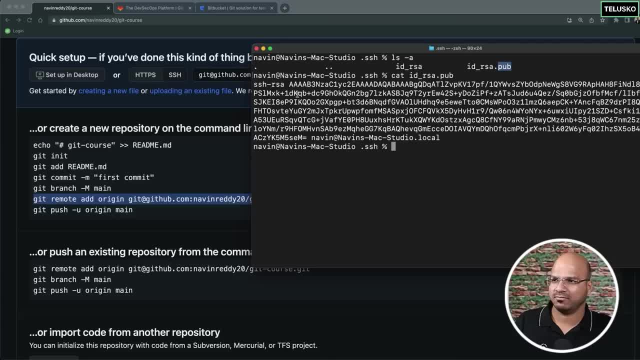 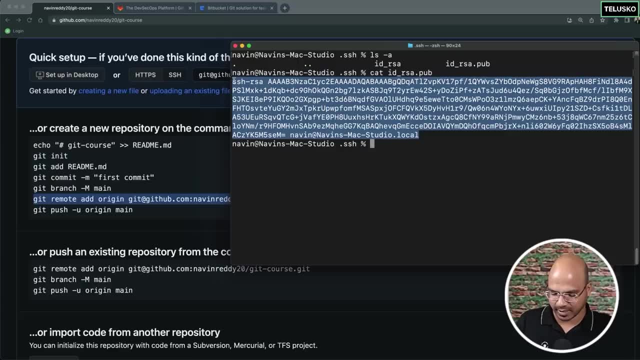 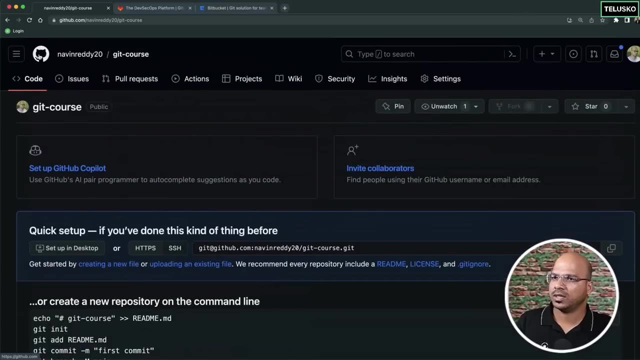 pub. now, where do i use this key? we got the key here, right, but how do i use it? it's very simple. you can just copy the entire key. okay, copying is done. where to paste it? it's very simple. if you can see here, let me click on here. i don't want to lose this page, so i will just open a new. 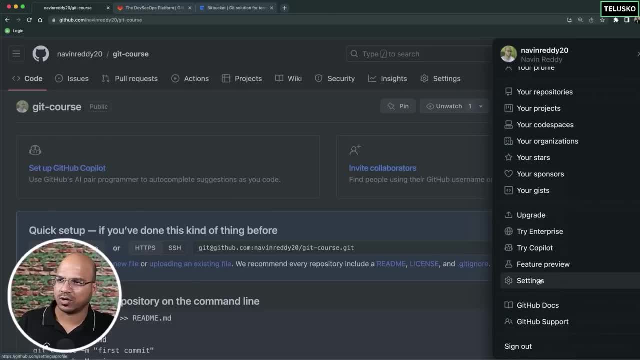 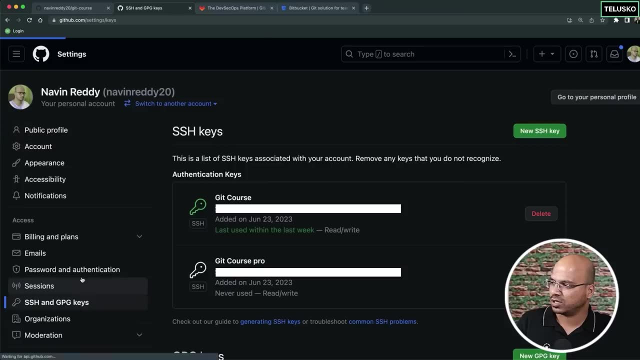 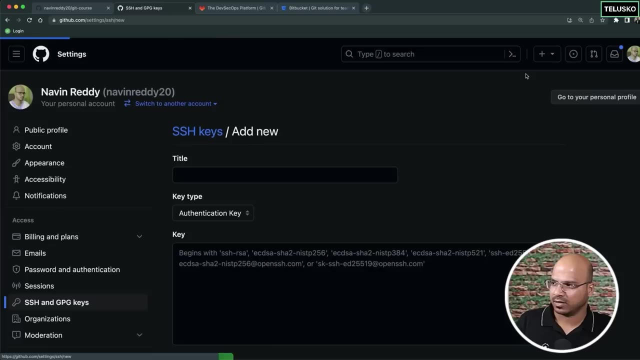 tab using the control or command button. i will click on settings and you can see setting is open here. and then, if you scroll down, there's an option of ssh and if you see this, i already have some keys here. ignore that. i will click on new ssh key. i will give a title to it: git cool 1. 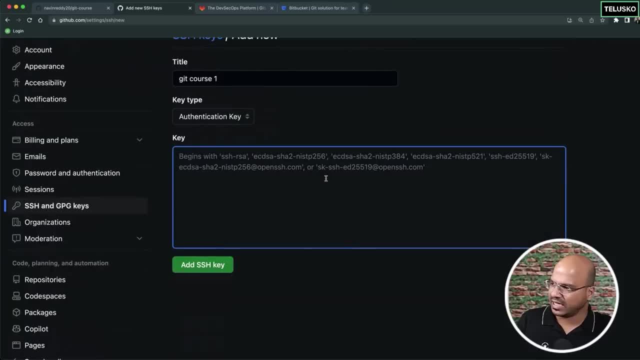 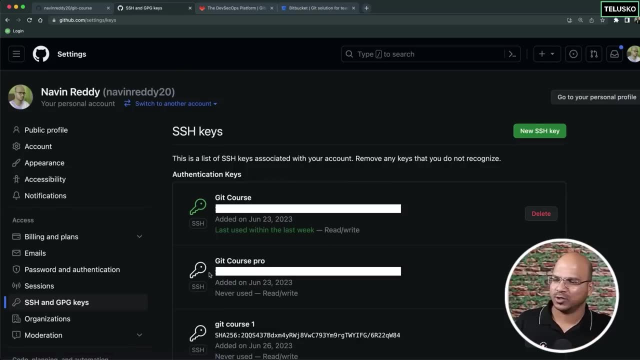 because i already have one before, and then you paste your key, that's it, and click on add ssh And now your client and your server is connected. So connected does not mean it's continuously connected. Every time you push something it will verify. okay, it's coming from the right person, because 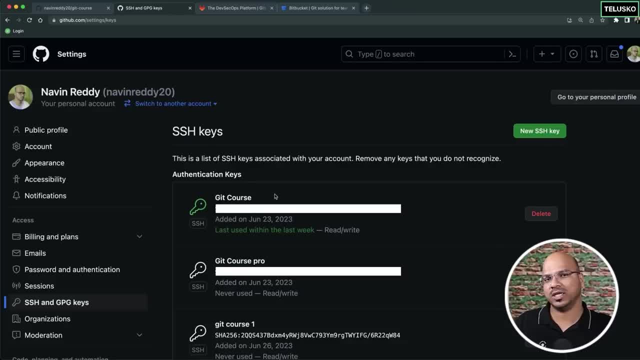 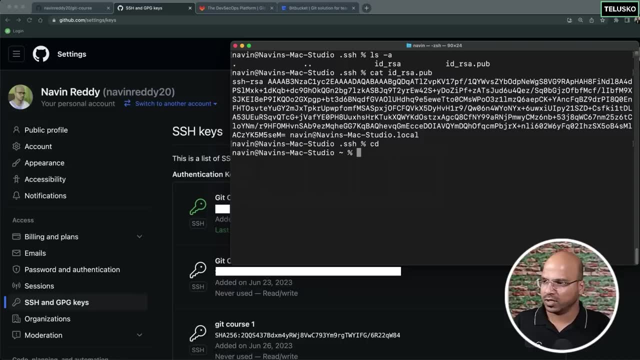 I can see the SSH key, which is mentioned here, and on the local machine they are the same. Okay, so now, once we have done that in the terminal, let's go back to our folder. So which folder we were working with? 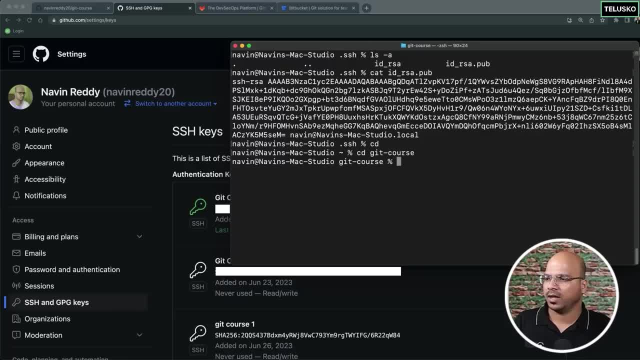 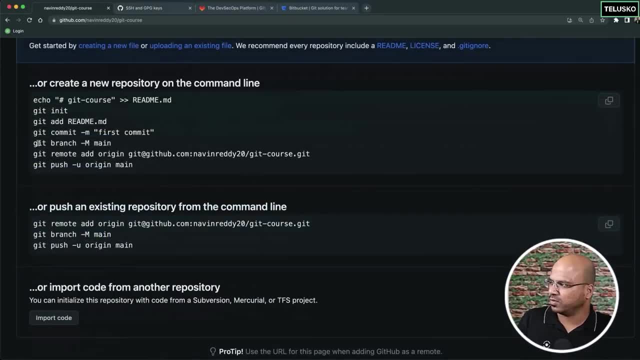 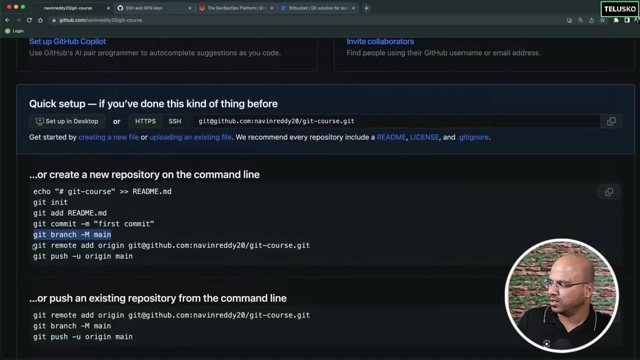 I think git goes, and if I say ls-a, just to verify, and you can see we have the same thing Now, if I go back to my steps, so we are done with this step right branching. Now we'll just use this particular one and DAC2 for SSH. okay, 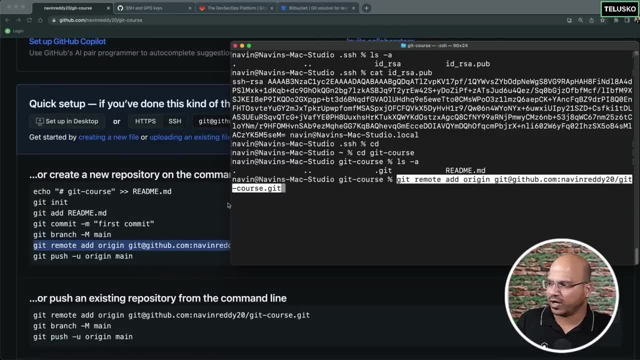 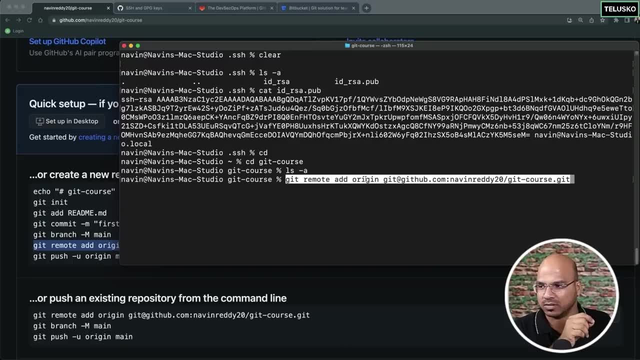 So we'll just copy this and paste it here Now. what we are trying to say in this is: we are doing git remote, because that's a remote repository of GitHub. we are adding a origin with this link. So this is where we are trying to connect and when we say enter, connection done okay. 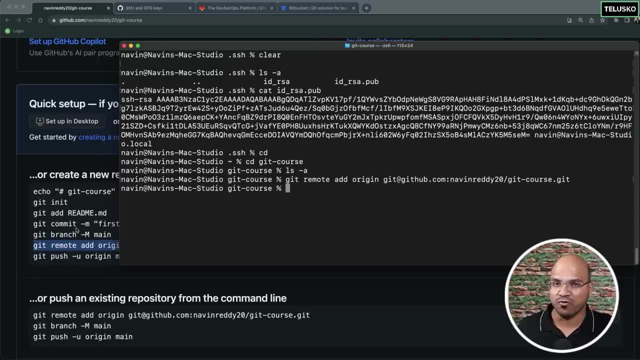 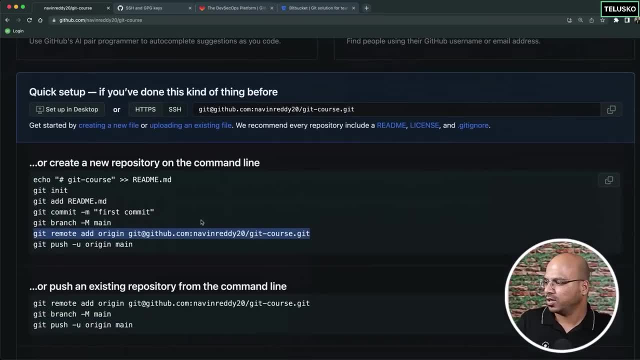 So, basically, we are trying to map it Once you have mapped it, now we have to move This file, which is in the local repository, because this is in local right. the remote is empty at this point, So what I will do is to push the code, just copy this paste. 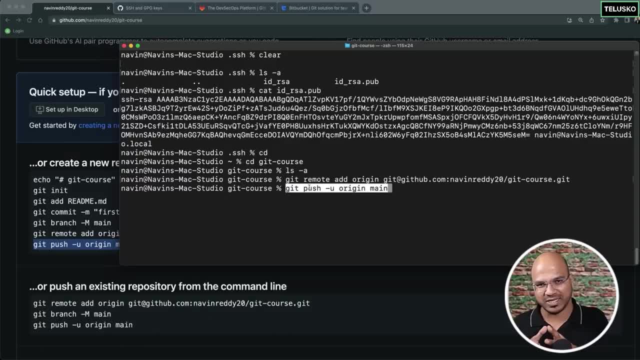 So what we are saying here? we are saying git push. Push means we are pushing the data from the local copy to the remote copy, And then we are also mentioning that there's a different branch and origin. So basically, u is upstream, set up the upstream, and then the branch name is main. okay, 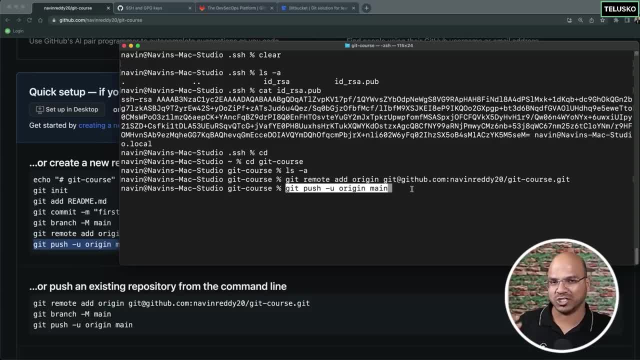 This is something you have to remember. Sometime you will mess up with main and master if you are referring to some other documents. In the earlier documents, earlier versions, people used to mention master And now we are mentioning main, so you might get confused there. 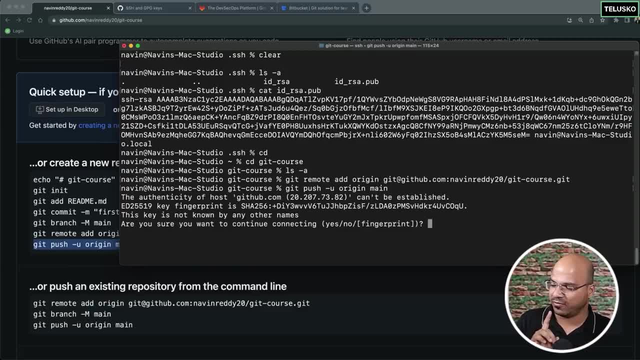 And if I say enter, it is pushing the code. okay, It will take some time, But before pushing, it is verifying. hey, the key is there. Is it the right key? Yes, I think I only have one key here. 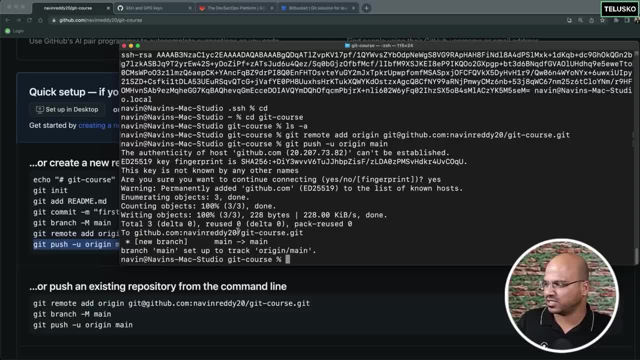 Enter and done. The pushing is done. That's what it says. It says: counting objects done, Total Done. Set up to track. Okay, It looks like everything is done. How do I verify? I can simply refresh my page and we got it. 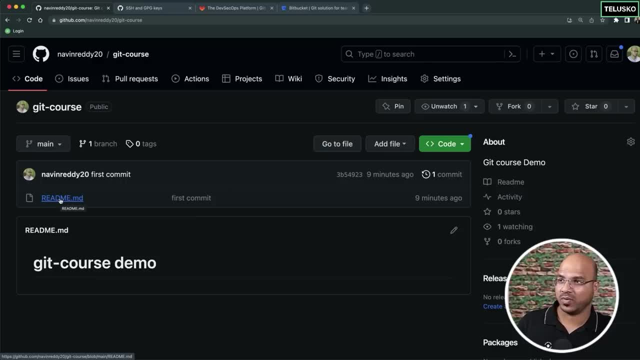 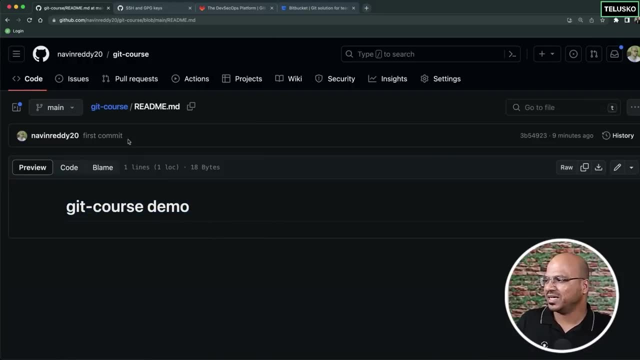 Now, this is a file which we created in the local machine, right? And if I open this, you can see this is the data we got. Okay, Now this looks cool, right? So basically, we were able to push the repository from the local machine to the GitHub. 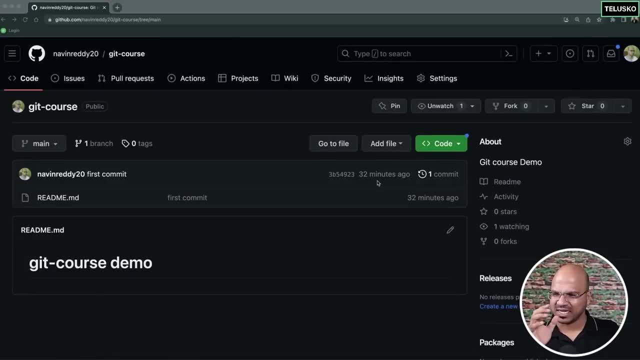 And every time you work on a project now, these are the steps you have to follow. So, basically, we were able to push, We were able to push the code from our local repository to the remote repository right, And then we followed some steps and it is done. 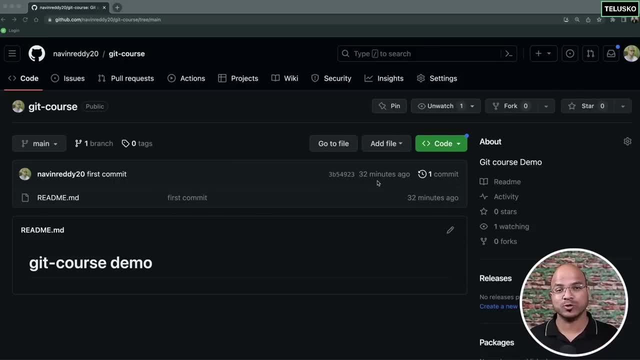 Now, that was your first commit right. But what if you want to do some more? You want to build the entire project and you want to push. Of course, you will not do it from normal command prompt. You will be using some IDE to build your project. 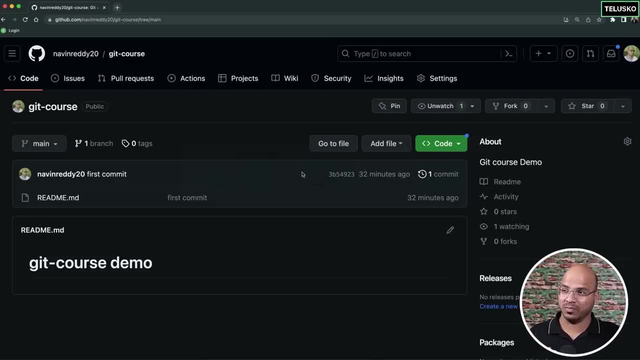 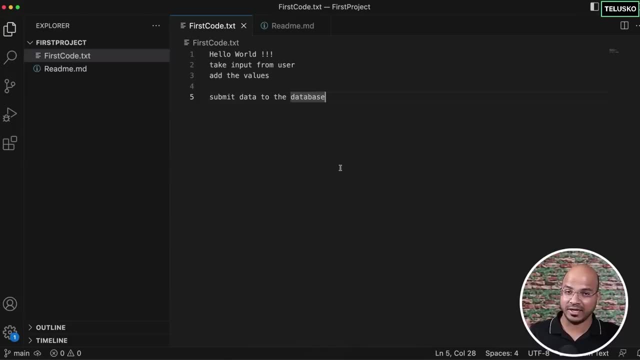 Now this can be for normal book writing as well, or making a video script as well, But let's stick to VS Code here. So of course, you can use any IDE for that matter, Or any editor. So if you're using a normal notepad, of course you have to use a terminal or command prompt. 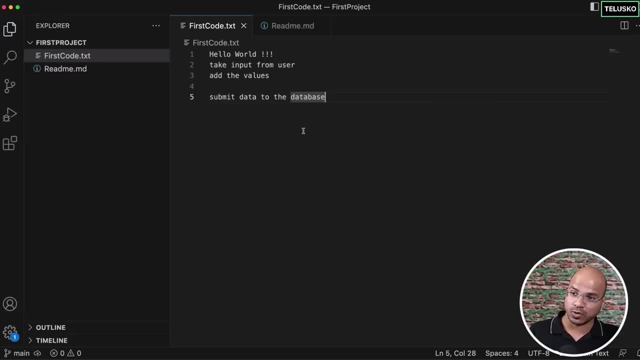 external to your editor. But since in VS Code we have an editor as well, and then we got terminal, So what I will do is, first of all, if I want to use VS Code, I have to open that folder. Now, which folder? 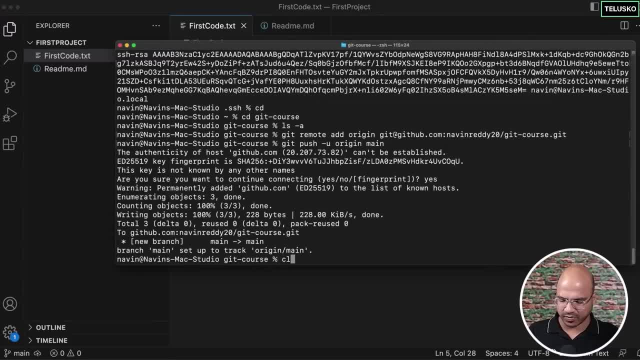 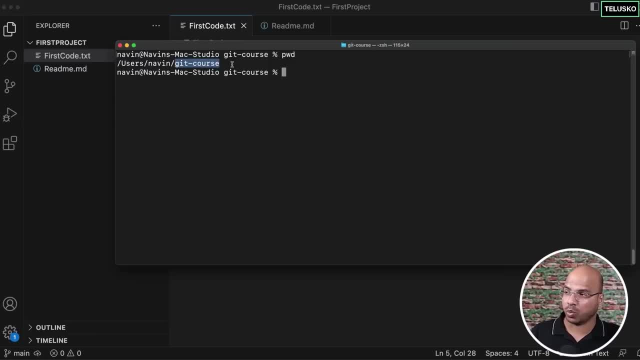 Now, if you go back to your terminal, this is where we are right. So, if I clear, and if I say PWD, which is present working directory, I am into this folder which is Git source. So whatever files we have here, 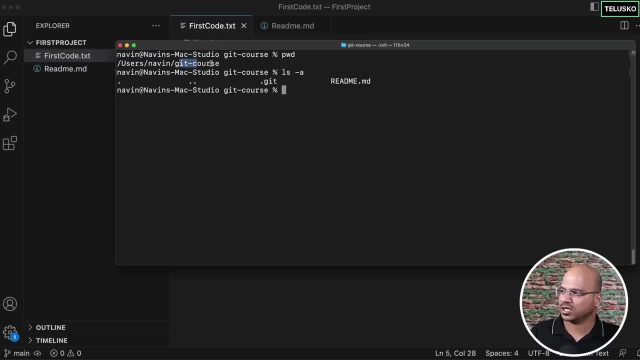 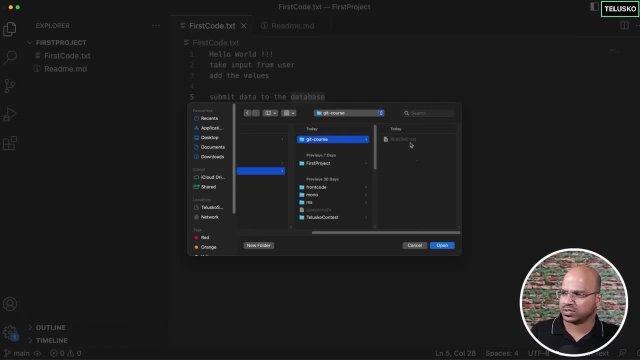 Is into this particular folder which is Git source. Now I will open that in VS Code. So I will click on file. I will say open folder. It's going to be in Git course open. So basically I have opened the same folder. 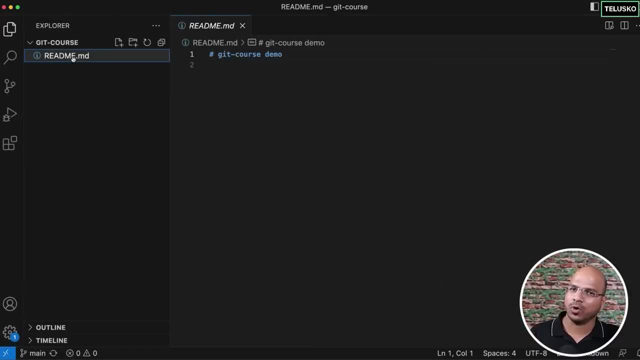 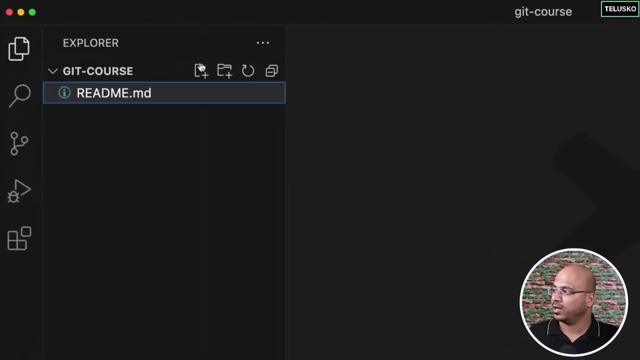 Okay, So we got that file here, right? So if I open this, this has the same content which we had earlier. But what I will do is, instead of working on this file, let me add some more files, at least one file. 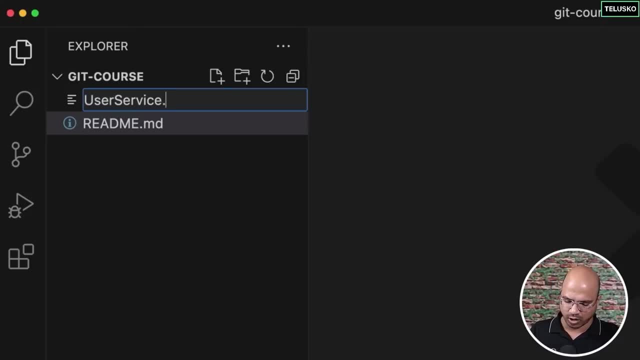 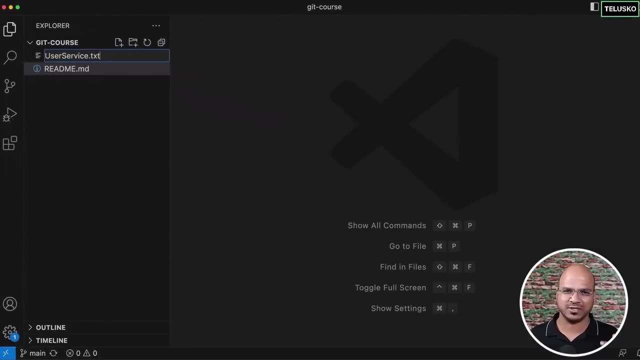 So I will say, let me say this is my user service dot txt. Now, basically, This is my application. The reason I'm doing txt is because it can be any programming language, right, Java, Python, C, sharp, it's your choice. 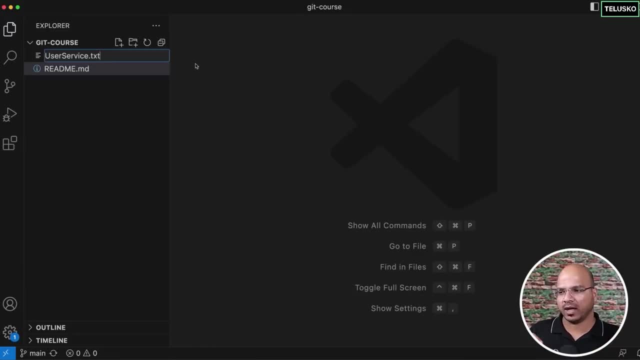 So let's say, if you're saying user service, we are building an application where I want to do something with user service. Maybe I want to accept user data, I want to process some data on it. So let's say user service and here I will say: get the user data. 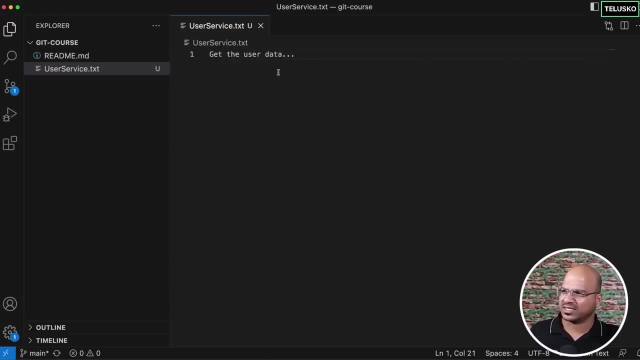 So that's it, Nothing fancy, Just one line of code. In fact, this can be a normal programming code as well, but just to keep it simple for all the languages, We are using a normal text. So we are saying: get the user data and save. 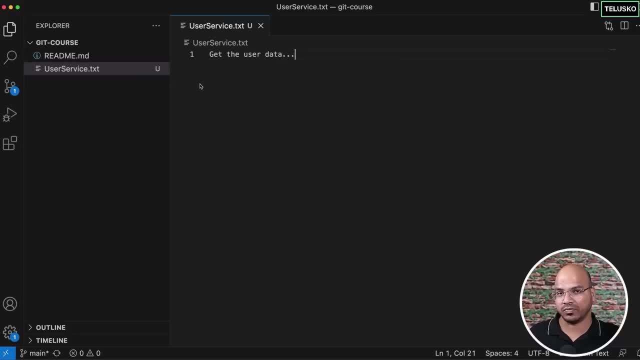 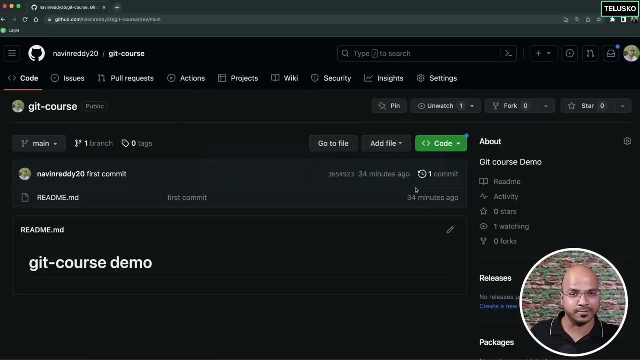 Now, if you see, this particular file is there in your working directory, it is not even there in Git. And also this file is not even there on the GitHub. This is what we want to push on GitHub. How would I do that? So let's go back to VS Code. 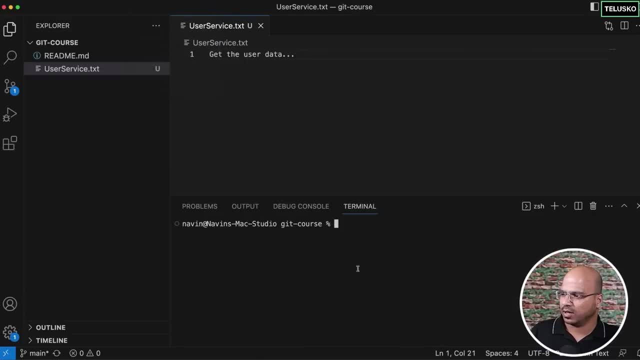 And if you want to do any of this, we have to say new terminal And we've got a terminal here And here. basically, we have to say git status. Now, When you say git status, You can see we have a git repository inside this particular folder. 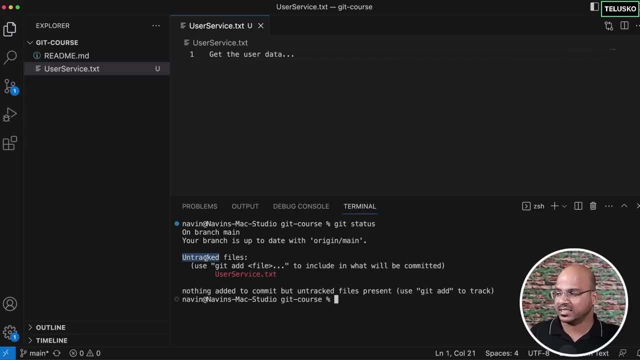 But this file, which is user servicetxt, it is untracked. We need to track it. So how will you do it? It's very simple To track it. we can simply say git add And you can mention the file which is user servicetxt: enter. 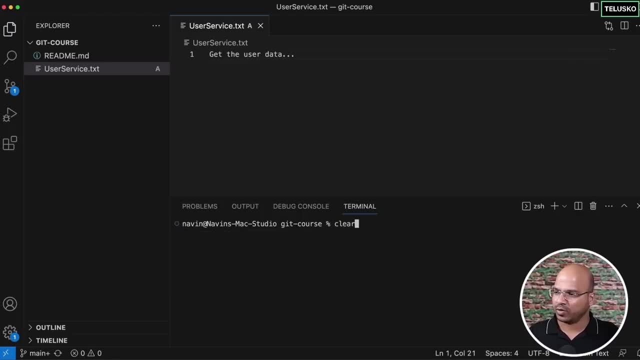 And now we have added that into staging area. How would I know that? Let's say git status And you can see, now it's into staging area and we can commit it. How will I commit Git? No, no, At least I think at this point you remember all the commands, right? 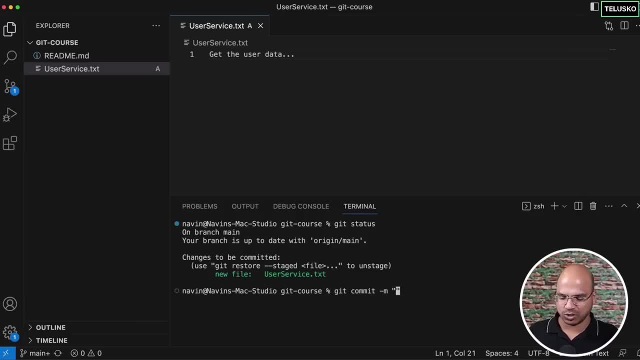 So git commit hyphen m and you can pass a message So you can say: user service created Now. it's always a good idea to type at the same time when you're watching this video, so that you will know what is happening, right. 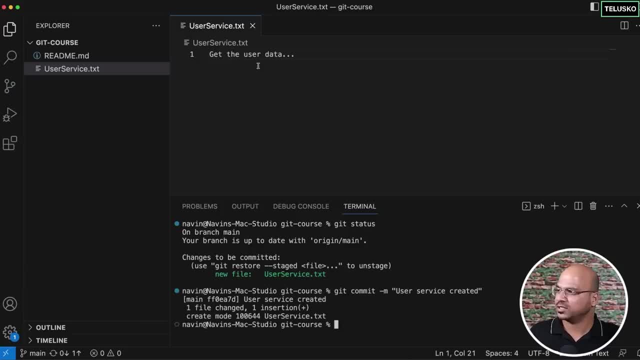 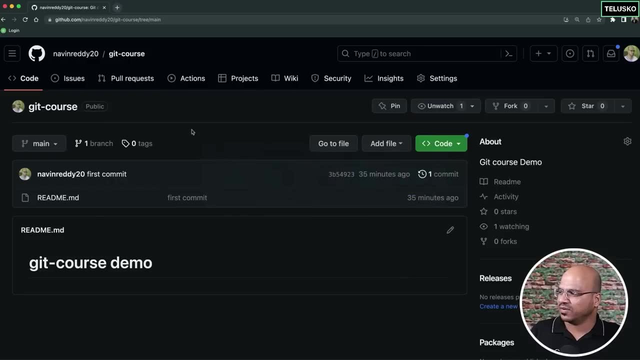 So here, if I say git commit, and now we have committed it And that's why you can see the U here went off, now, Okay, Committing done, But does that mean it is available on GitHub? No, We have done the commit on the local machine, right? 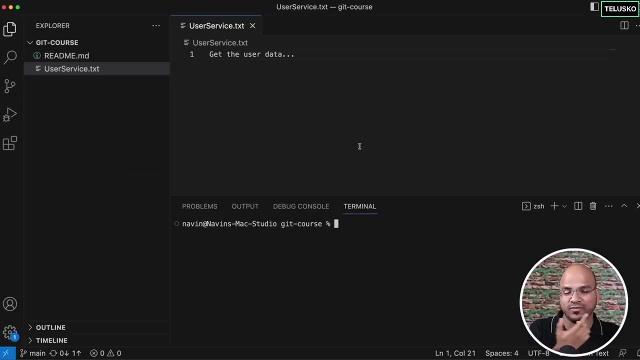 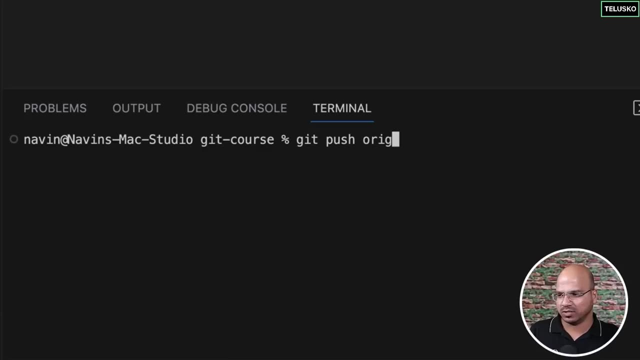 Now we need to push it on the GitHub And for that we have to remember that command git push. So let's use git push. and then you have to mention origin. So basically, for pushing you have to say push And the origin is the URL. 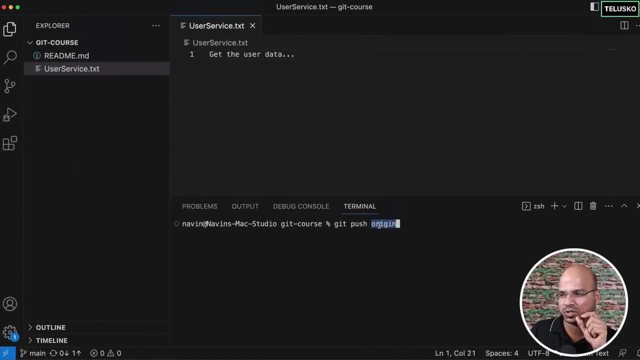 Remember the URL which we have used before. That is what is representing this origin. And then you have to mention the branch. The branch is main. We are pushing on main branch. I will say: enter. It will take some time And done. 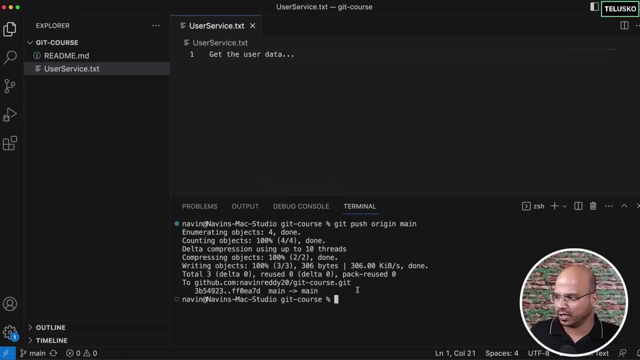 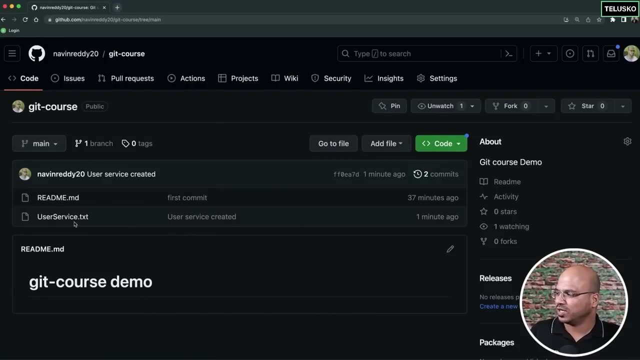 You can see pushing is done, So from your local machine to the GitHub. Let's verify. Go back to GitHub. now It's still not here. Refresh And you got it. So you can see, we got this file, which is user servicetxt. 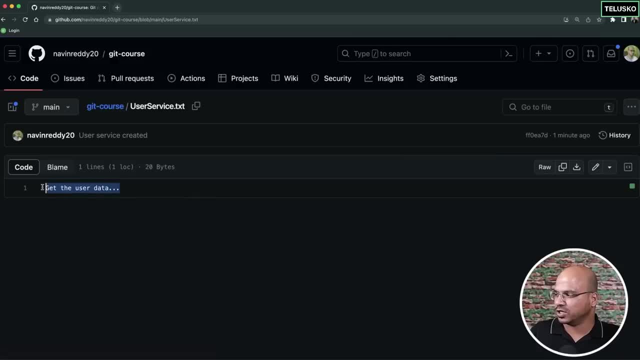 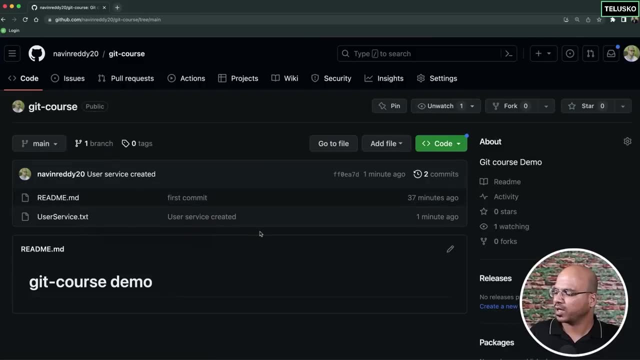 And if you open this, you can see we got the data which says get user data, which is available now. Right, So let's get back to our project. These are the two files we have And, if you observe, we have the user service. 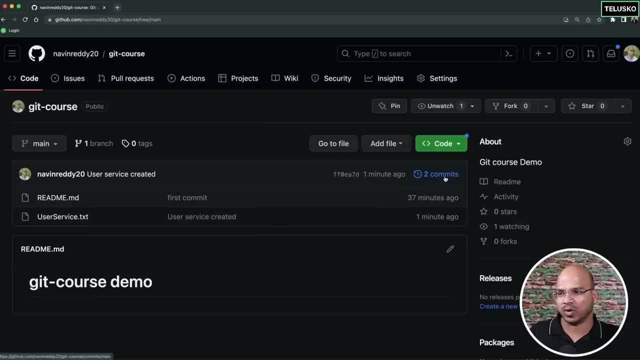 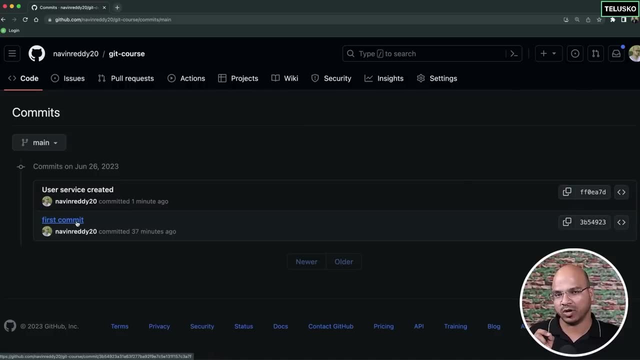 And, if you observe, we have the user service And, if you observe, we have two commits here. Now, what are the two commits? If I open this two commits here, this is the first commit which we have done where we created one file which is readmemd. 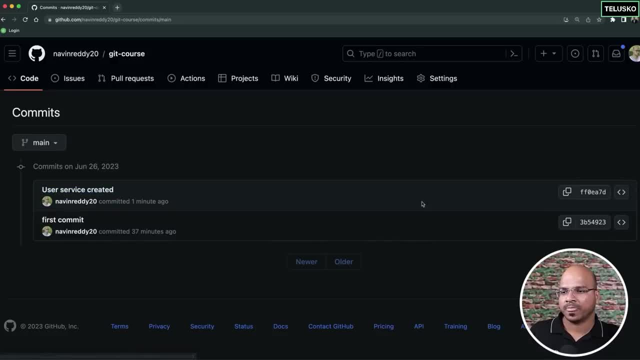 And this is your second commit, which is user service, created. Now you can actually, at any given point, you can go back to the earlier version where you don't have. let's say, if you don't want user service, I can click on this particular file. 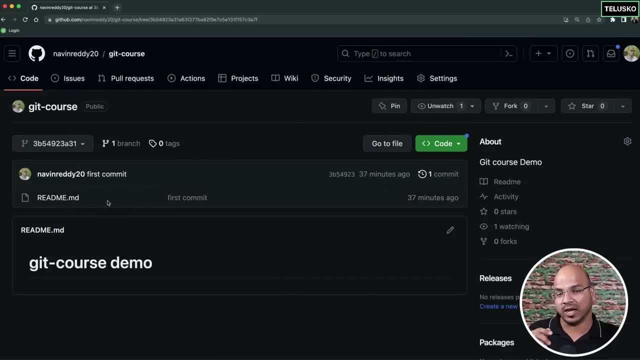 And it will give you the status of that commit. So in the first commit we had only one file, right? that's what you can do, so it's it's fun to navigate between different commits. if you want to go back to any commit and if you want to see what changes you have made in fact, you can click on the. 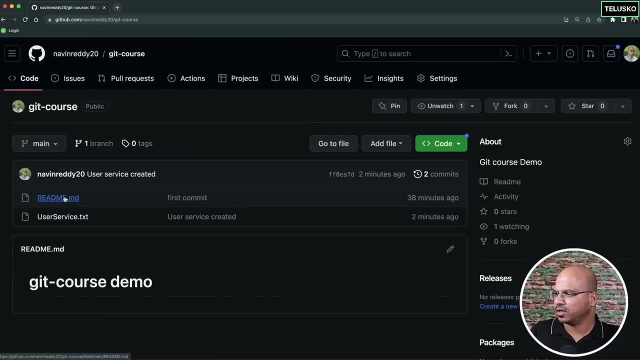 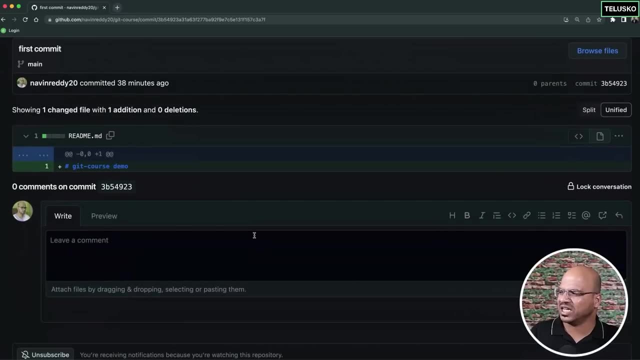 file as well to see the changes. so if i go back here and if i mention, if i go back to any file, okay, let's go to commit and click on any commit here, so it will mention what changes you have made. so we have created this file, which is readmemd, and this is the change you have made. 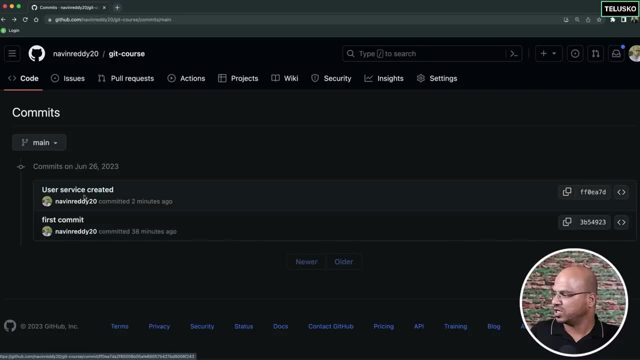 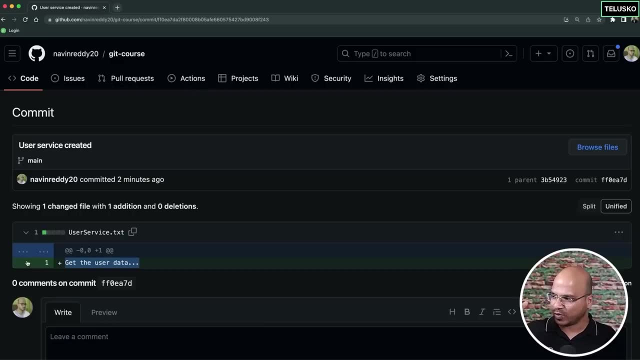 in fact, you can go to the other commit as well, which is here, and you can see what changes you have made. of course, it makes sense when you have multiple files and you can see all the files which are changed. okay, so that's how, basically, you add your files to the remote repository. let's talk. 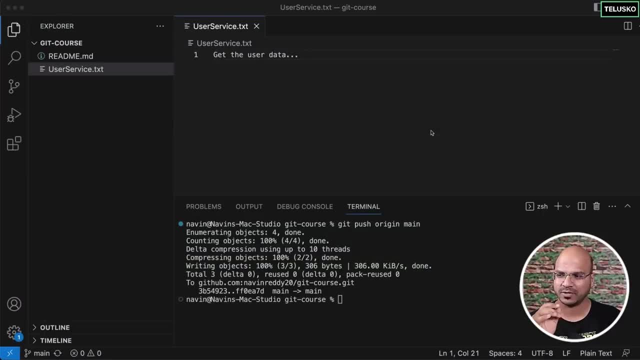 about tags. now, what is tag? we'll talk about that later, but before that i just want to show you one more thing, which is about this remote. now, if you remember, in the earlier video we have done this push right. so from the local machine we were able to send the data to this server right. so basically, we were able to push it. now it has. 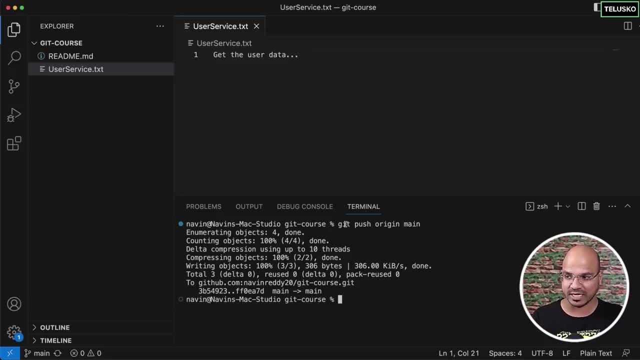 four things. first of all, we have a git command, of course, because we're using git tool. next, we have push. basically, we are pushing the code right, whatever data you have, and then we have something called an origin here. okay, so we'll talk about origin, because that's very important for this part. 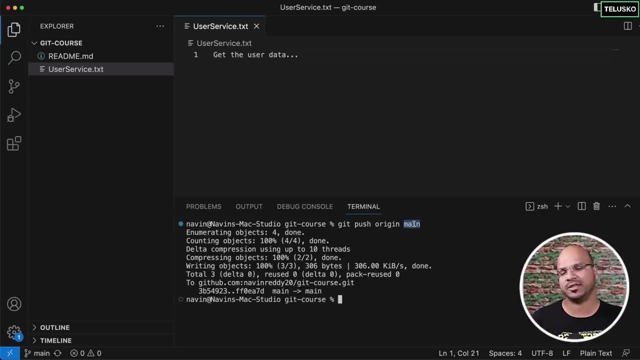 then we have: we are specifying the branch name, so it can be main, it can be master or any other branch which you create. let's talk about this origin, why it has to be always origin. of course we have done origin, but it can be different as well. the thing is, for this particular 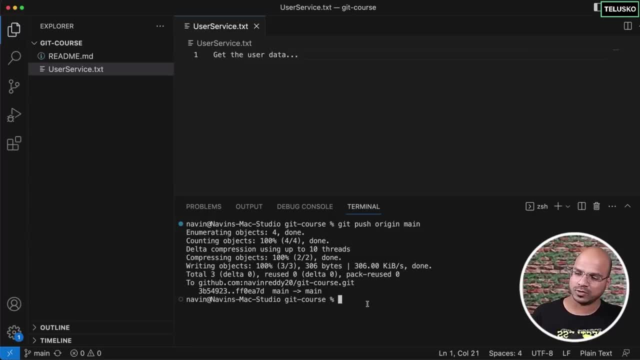 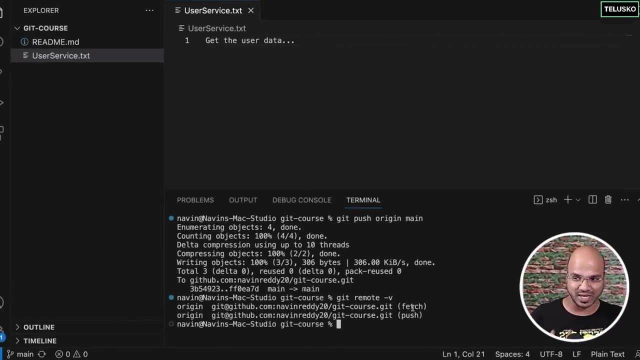 repository. what we have done is, when we talked about the remote server, we only have one example. if i say git, remote, hyphen v, so this is the command using which you can see which is your origin, so we can have a origin for fetch. so, from the server to client, this is the link we have to. 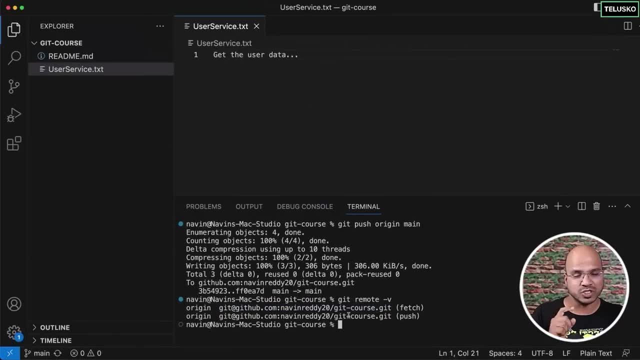 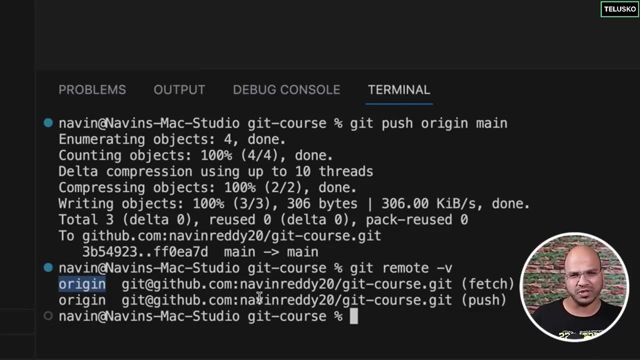 use and from client to server. again we have the same link because we only have one remote repo. the name is origin. of course, this can be any name. you can change it as well, so you can rename it, or you can connect to different repositories, not just one, and you can pull and push to any other. 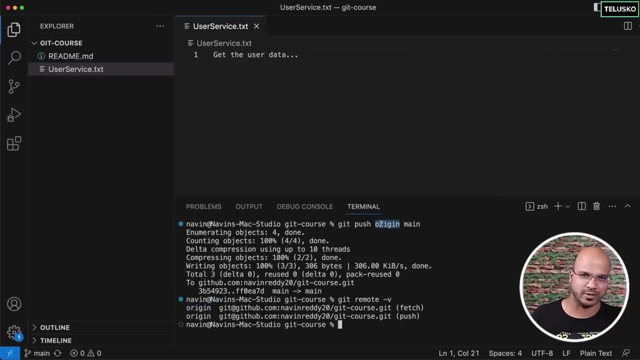 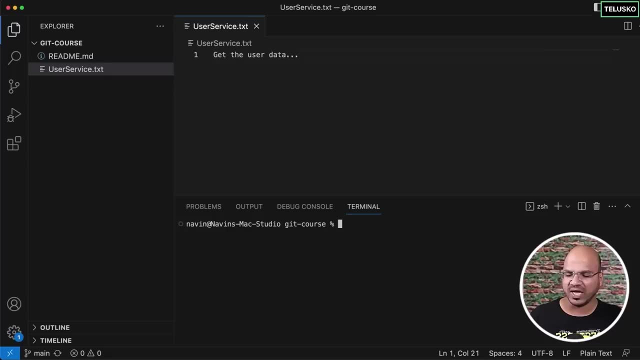 repositories, if you want. the only thing you have to do is you have to change this one, so, instead of pushing it to origin, you can push it to something somewhere else. okay, so keeping that aside now, let's talk about tags. now, basically, we have a concept of tagging. now, if you have observed every 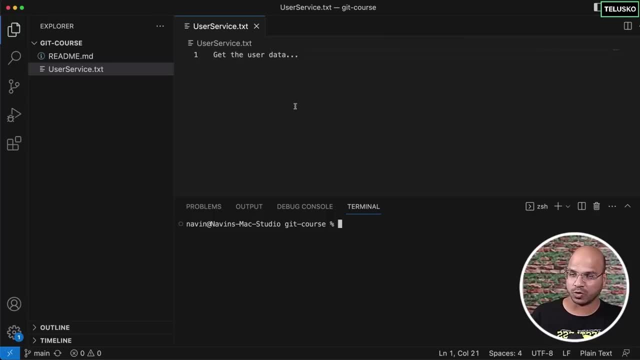 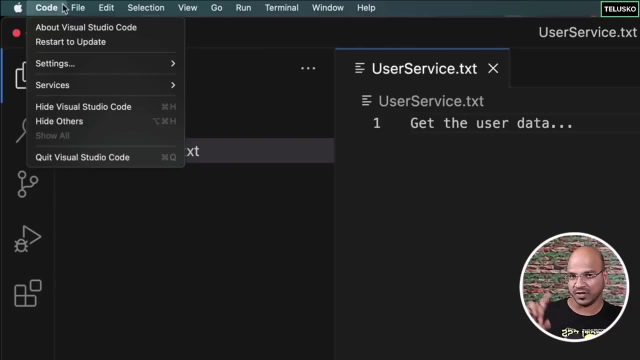 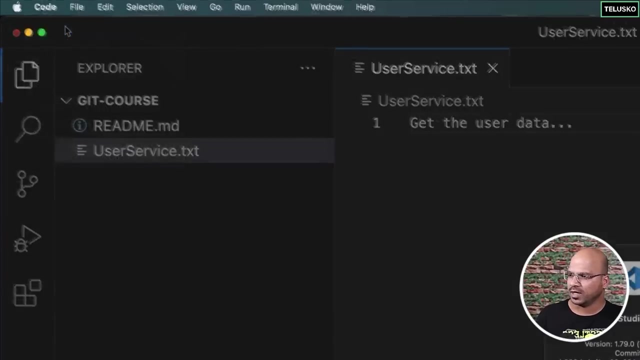 software which we use, it has a version number. example: i'm using vs code here and if i go to about or not co, not help here, because in windows you will, you will get that in help. in mac you will get that in the about. so if you go to about vs code here so you can see it is giving you a version. 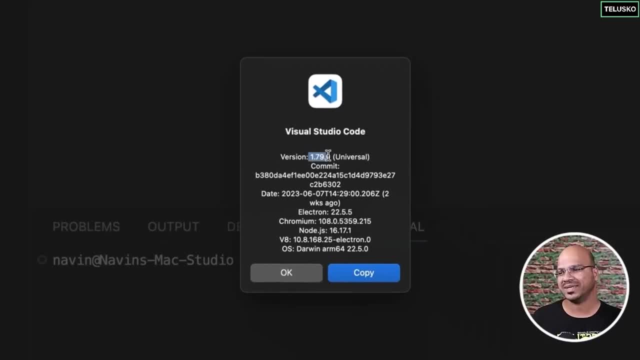 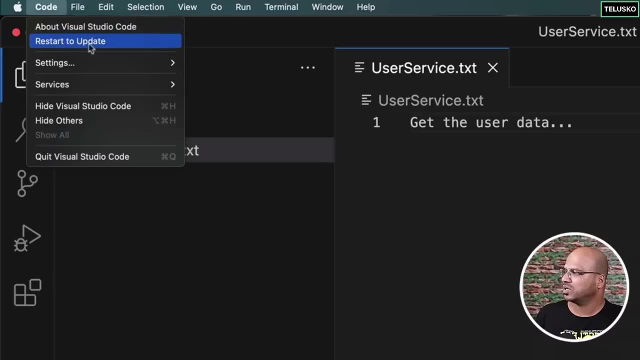 number here. so every time you download a software you will get a particular version. of course you will also get the updates for it. so you can simply go here and i can check for the updates so you can see it says restart to update. but i don't want to restart now. but you will also get update there. so 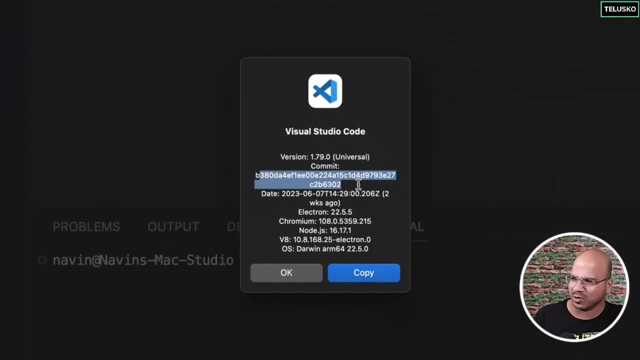 this is the current version and this is a commit. now this looks weird, right. why do we have a commit in the about that? we'll see in some time and also observe some things, because in the next video we'll talk about this thing in detail. okay, so we have electron, we have chromium, we have nodejs and all these have versions, okay. 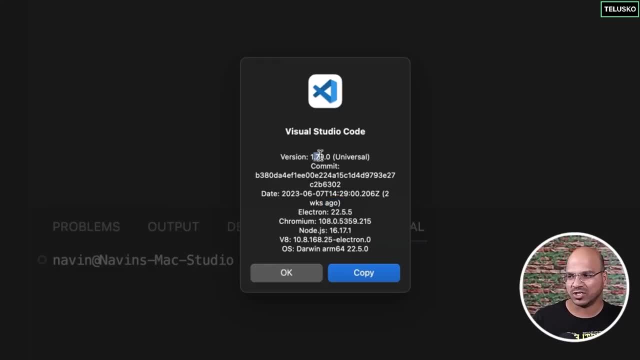 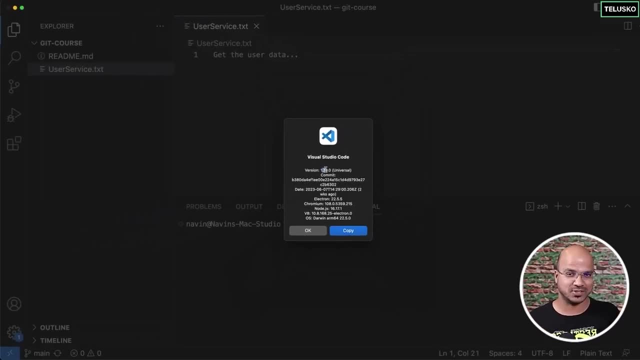 so we'll talk about it in some time. but important is, we have a version here now. this version is basically a tag. so let's say, if you're working on a project and then you have done several commits and now you think, okay, i'm all set to release my next version, so you can give a tag to it. 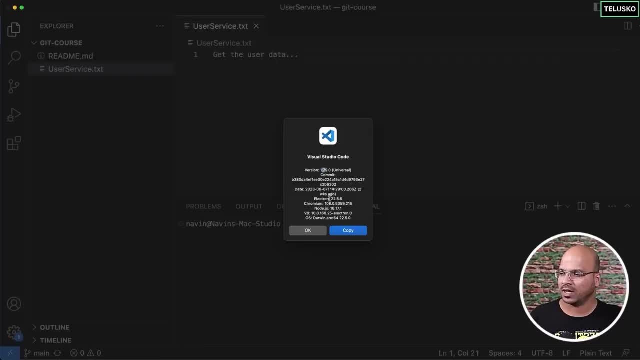 once that, once that version is done, you can go for the next version. so, basically, how do you give this tag the version number to each commit, so not exactly each commit. let's say you have done 10 commits and then now you think, okay, the software is up and running, we can publish this. 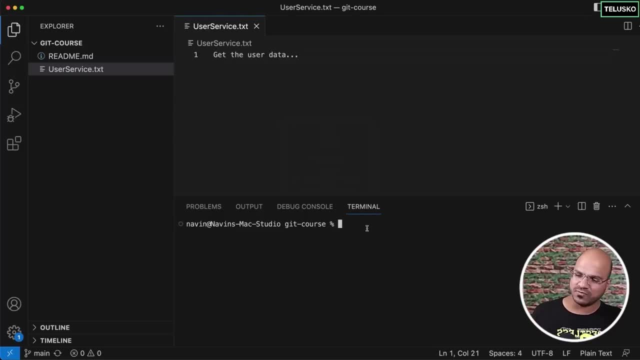 particular product to the users, we can give it a tag. first of all, how do i check how many tags i have for this project now? the way you can do that is by using something called get tag and when you say enter, it will show you all the tags which you have given till now for this project. 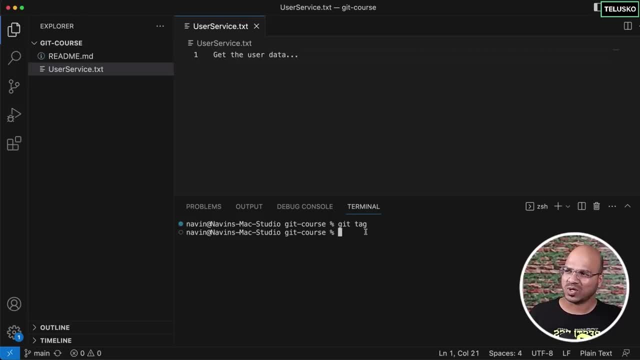 and this is empty is because we have not given any tag. so let's give our first tag here. how will i do that? it's very simple. you can say get tag and then, when you say tagging, there are two options here: one, you can use annotated tagging, or you can use lightweight tagging now, if you really want to. 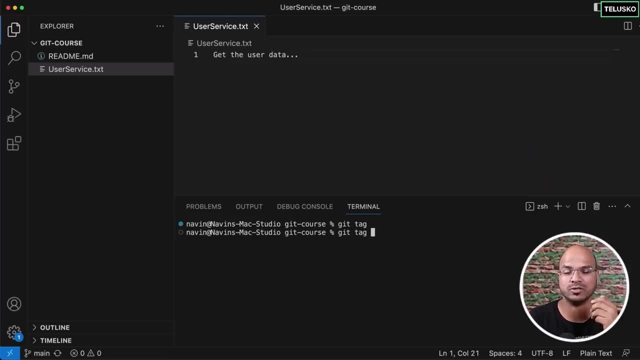 release this to the users and if you want to give more information about the user- i mean who is committing it or who owns it- so if you want all those information use annotated, okay, otherwise you can go for lightweight, which we're not going to say. so let's see annotated here, where every version will have different uh information about it. so 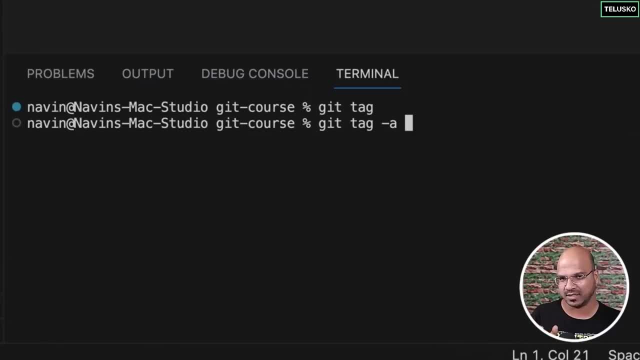 for that we have to use a hyphen a as a option for the annotated one, and then now you can mention your tag number. so basically, these are your version numbers. so there are different ways of using version number. uh, some people simply go with 1.0, like this version, or you can also mention v. 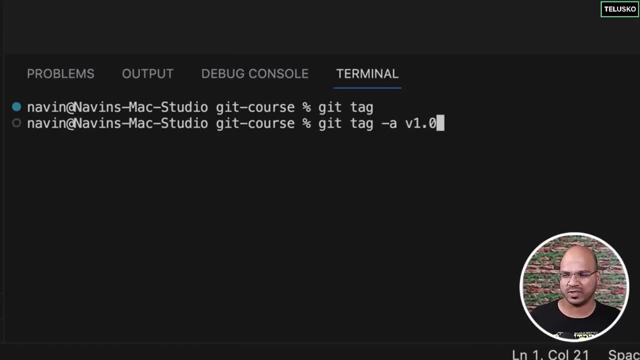 here, so v 1.0. so we can go with this particular one, which is v 1.0- this is our version which you are specifying here- and then you can go with this particular one, which is v 1.0. this is our version which you are specifying here, and then you can. 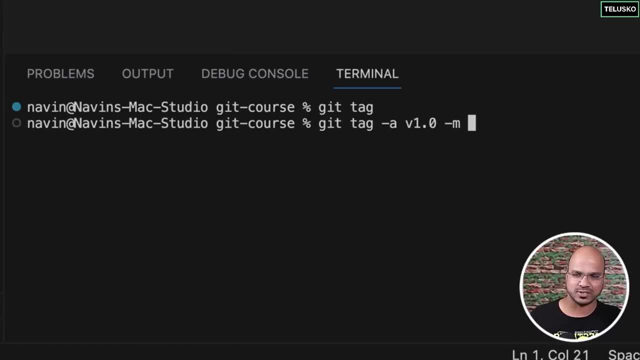 also provide a message. in fact, we need to do that, otherwise git will open a editor which will where you have to mention this, otherwise let's say m to give the message and i can say first release. so you can give something like this as a message and when you say enter now, tagging is done. 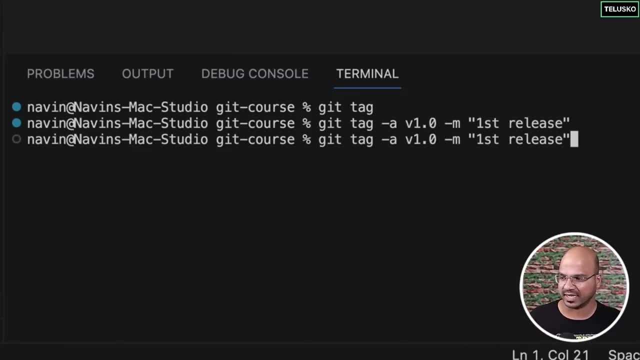 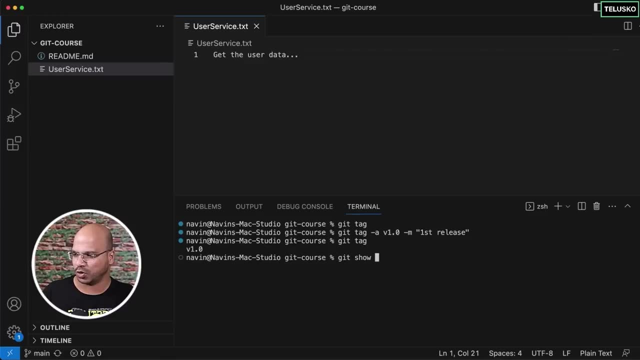 so you got the first tag. now, if you want to check, you can say git tag again and you can see we got one tag here. and, of course, uh, you can also see detailed information. uh, so you can say git show v 1.0 now. this will give you the information. so you can say git show v 1.0 now. this will give you the. 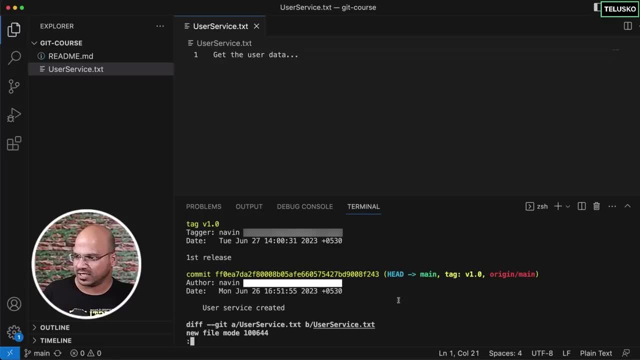 description about this particular tag and when you say enter, this is what i was talking about. so, for this particular tag here, uh, this is the tagger who has given the tag, and then, so that's my name and my mlid, which is hidden. uh, so the commits which i have done here is: this is the. 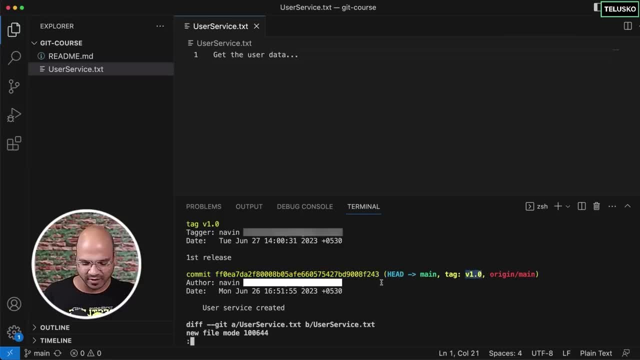 commit, which we have done, and this is it. so i have done this, okay. first of all, let me check all the thing done, okay. so if you see here we have done the tagging right, but the tagging is available only in my machine, in the local copy. so every time you push example, let's say, if i do some, 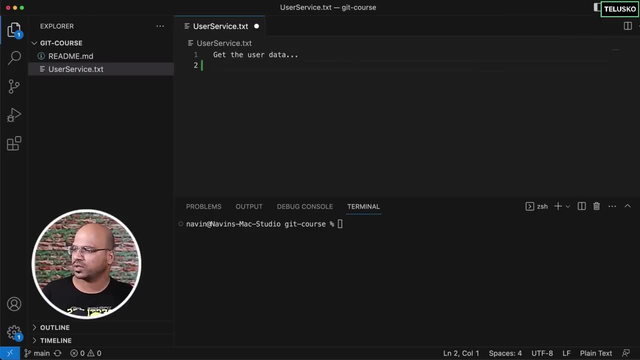 changes here. uh, i want to say this is: get user data and i will say process. so basically we have done some changes right, process the data. so we have made some change to the software and now every time you make a change, you can say git status. you will get the status. what's the next? 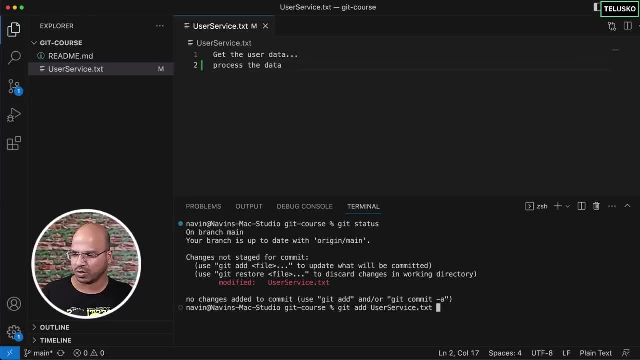 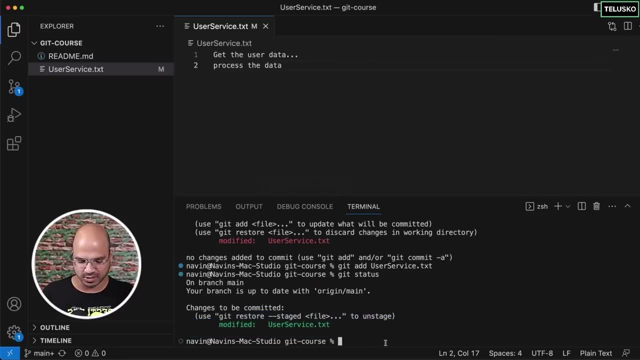 step, okay, so we have to add. so we have to say: git, add user service dot text. what next? again, we can say something. it says: now we can do the commit, let's do the commit here. so it's a git commit different m, and you can give a message. now i can say: uh, processing user data. so we have. 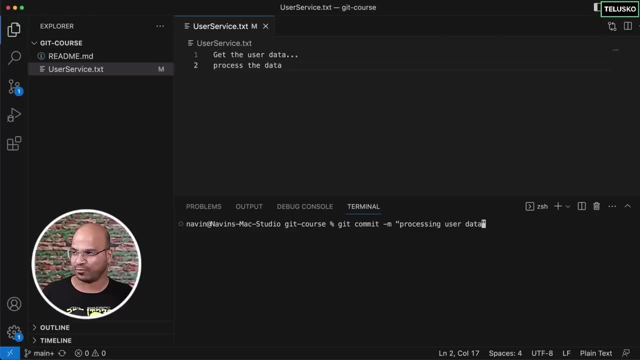 added the new feature right, so let's do that. and of course in the real life project it will be a bigger code which, just trying to keep it simple, enter committing done, but the commit has happened only in local machine. we have not done on the remote because, if you see, this is a local one. 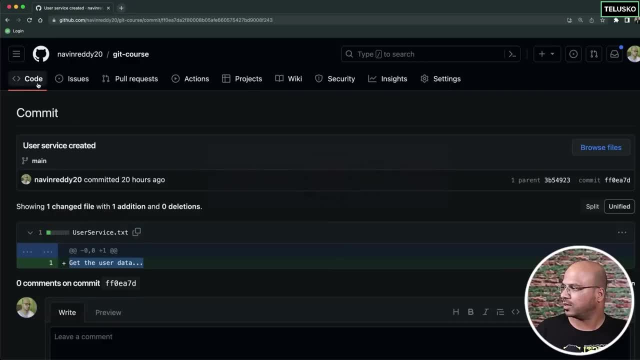 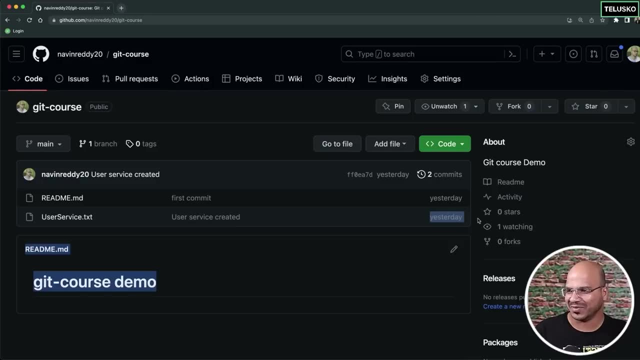 right, if you go toichtex, i don't know what you think. if i open this here there is a underscore: go back to your remote. and if I go back to get course, you can see we have done the commit yesterday. So basically I'm recording the video one in a day. So we have not done the 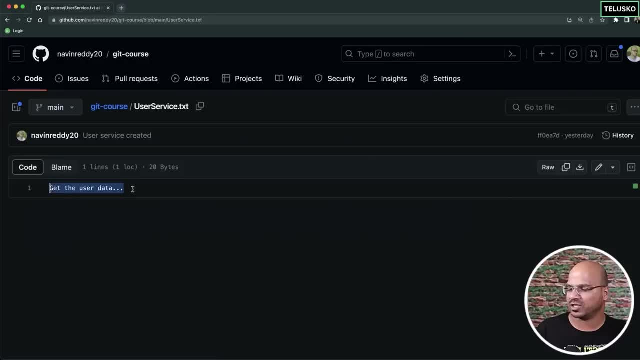 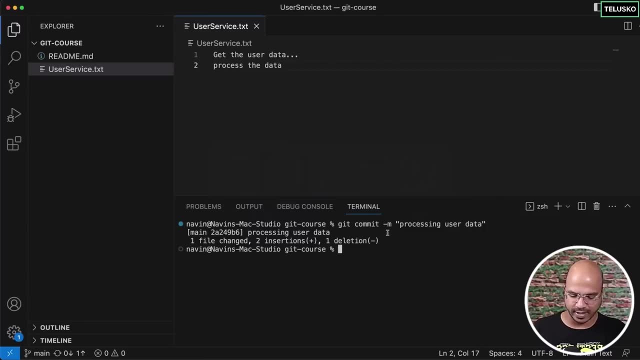 commit here. So if I open this, we only have get user data. We don't have process user data. So we have to push. How will I push? from my command line I can say get push origin main. This is the command you have to use And when you say enter, it will try to push. 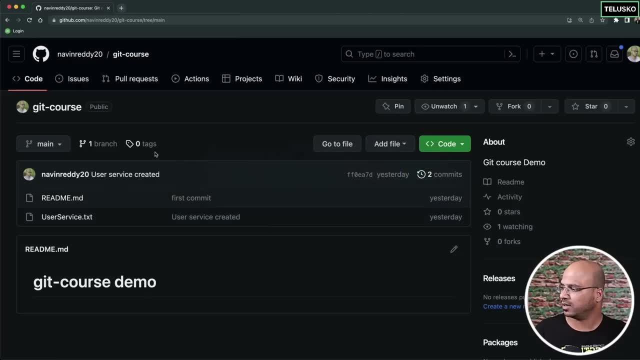 now And that's done. So pushing on the server done, Let's go back and refresh So you can see it says now, And this is a new commit, which we have done, And if you see the data, we have added new line. This is working. But then if you observe on the server there's 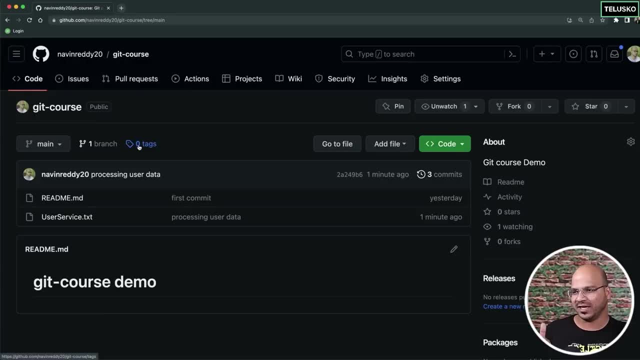 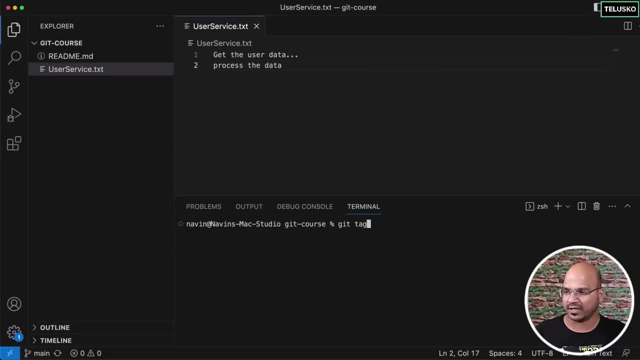 no tags here. You can see zero tags. In fact, before the commit we have created the tag. In fact, you know, after the commit we have done the changes right. We should create a new tag here now, which is: 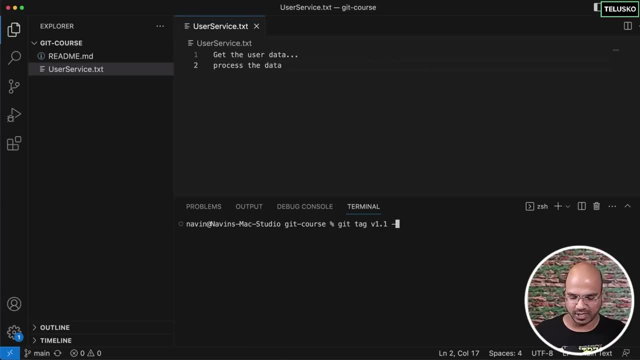 v1.1.. This is a new tag And we'll say a message. We can also do a daily release right 27th June release. So normally you know a lot of companies they release their product in six months or one month. Let me do it every day So I will say: enter now. So we've got. 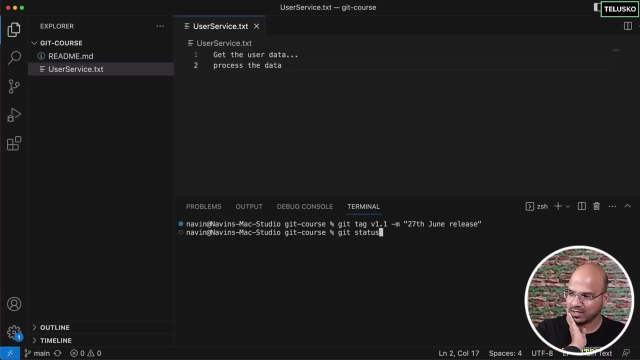 a new tag. How will I know that we have different tags here? So we have seen the command right, Which is get tag. Now you can see we have two tags, But if you go back to the server it shows zero tags here. So if I refresh, zero. 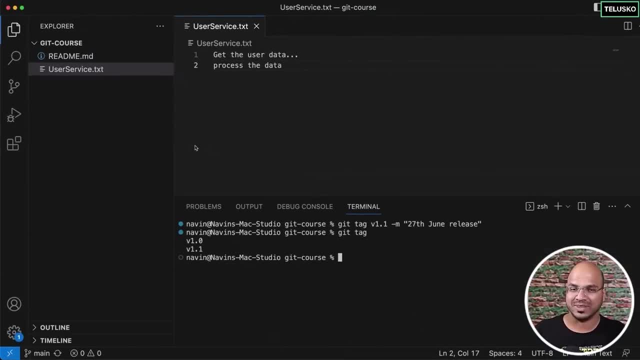 tags. So what we do is we need to push the tags as well, separately. We cannot simply push the code and it will have a tag. No, you will not get that. So what I will do is I will say: get push origin And we have to mention the tag. So let's push the 1.0.. And 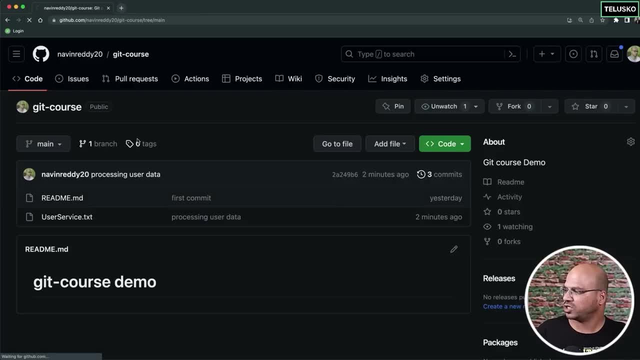 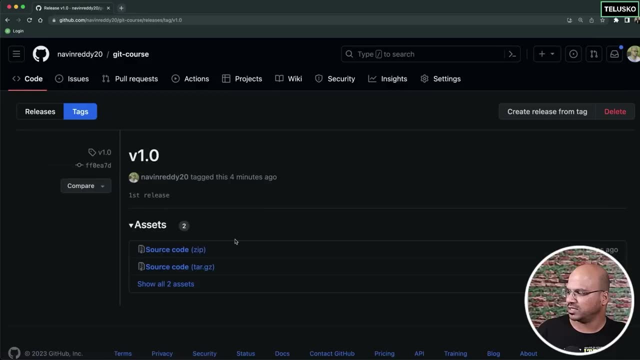 that's done, So you can see the new tag is created And if I refresh, you can see we've got one tag And if I click on this tag, this is a version 1, and, if I see, in fact you can download the source code. and it happened 4 minutes before right. 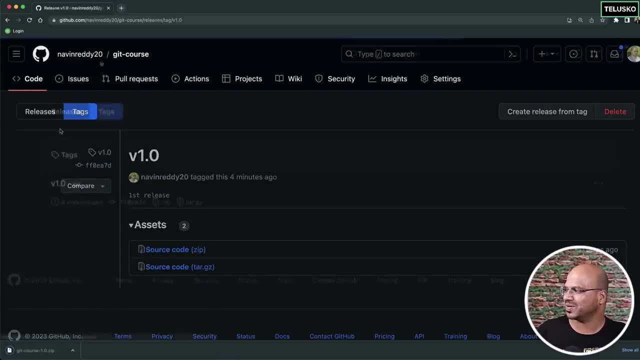 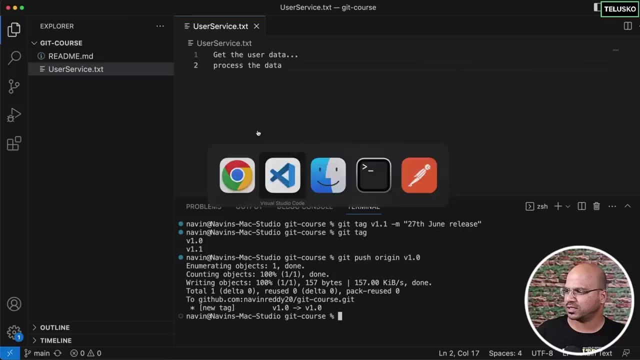 Okay, so it will give me the source code itself. Okay, we don't need the source code. Okay, but you got the idea right. So, basically, we can jump between different codes based on the tags as well. And now, let's see, let's also push the version 1.1.. 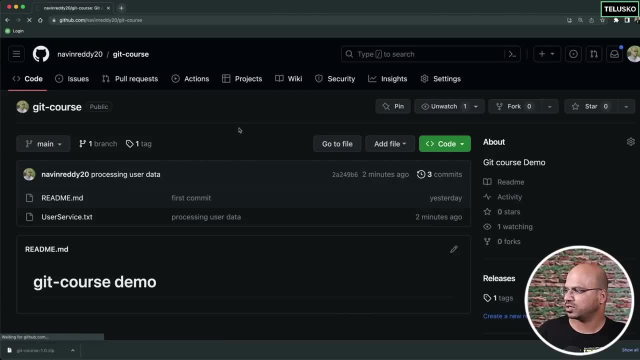 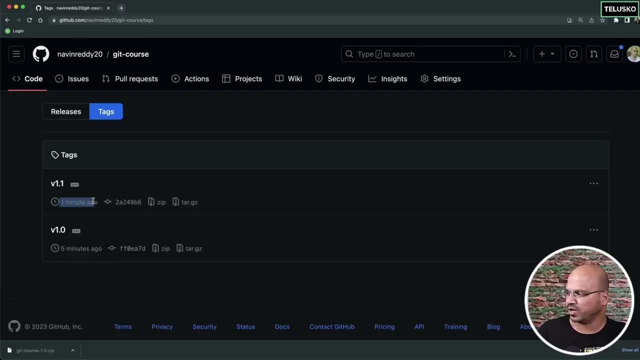 So we got two different tags and if I refresh, you can see we got two tags here And based on which tag you have, you can download it. So this is 5 minutes before and this is 1 minute before. So different tag will have different codes. 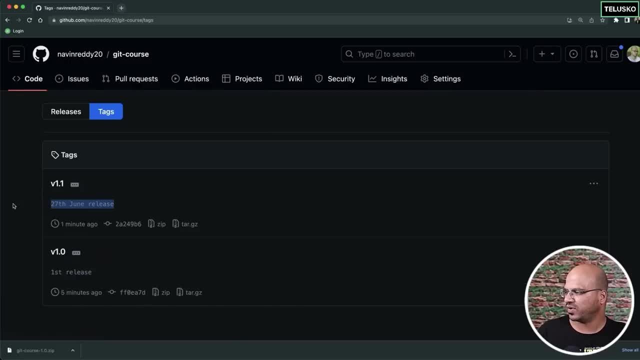 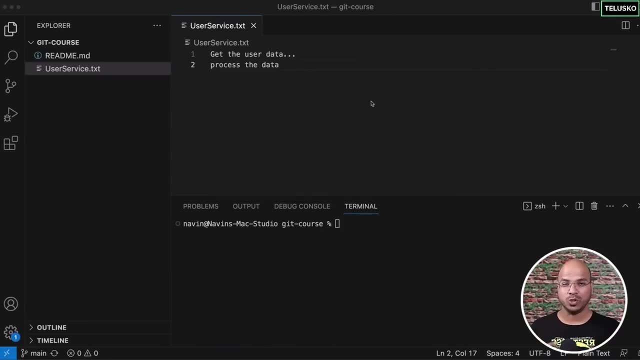 Okay, so you can see this is first release and this is the 27th June release- Awesome, so this is working. This is how you basically work with the tags. So till this point, we were able to work with our own repository on GitHub and local as well. 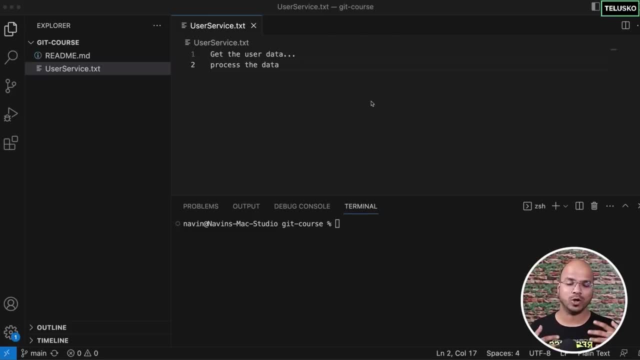 But what if you want to work with some other repository? Maybe you want to clone the code and you want to see what is happening there, Or maybe you want to push, or maybe you want to do some changes and use it for yourself. 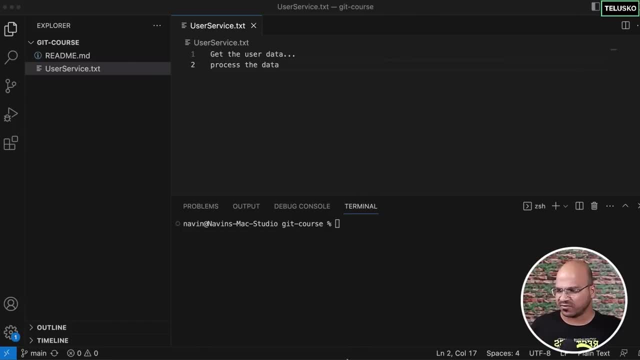 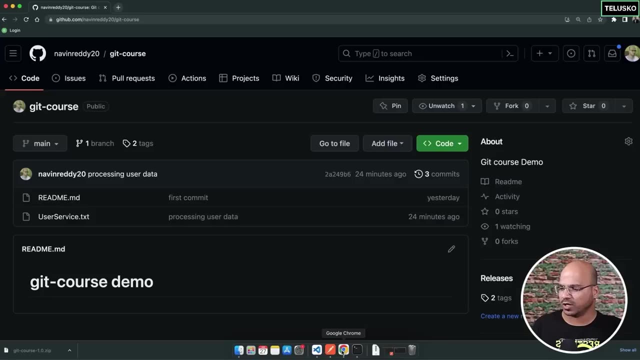 or push it to this remote repository again. How will you do it Now? first of all, let's go. let's find some project Now, since we are using VS Code, which is open source, so what we can do is we can go to GitHub. 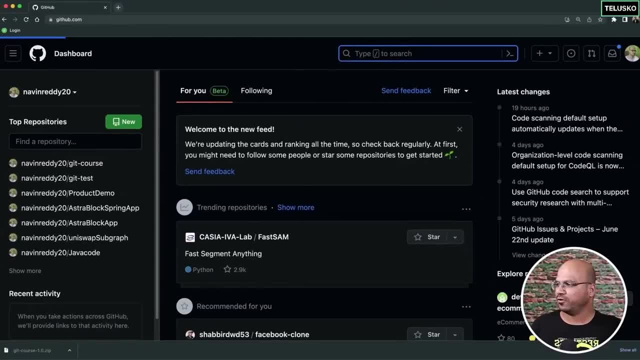 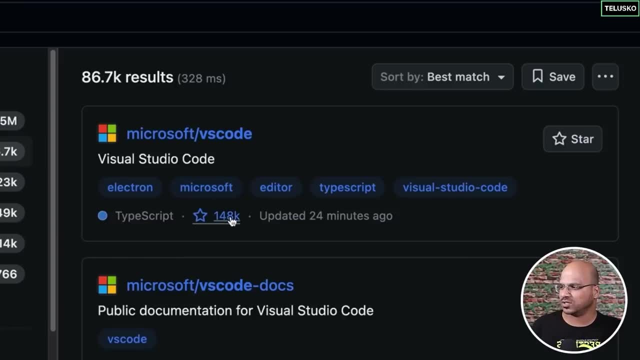 So you can do a search here, which is VS Code. Now, if you search for VS Code, you can see you will find the source code. This is the source code. It has so many stars here and this is from Microsoft, so let's use it. 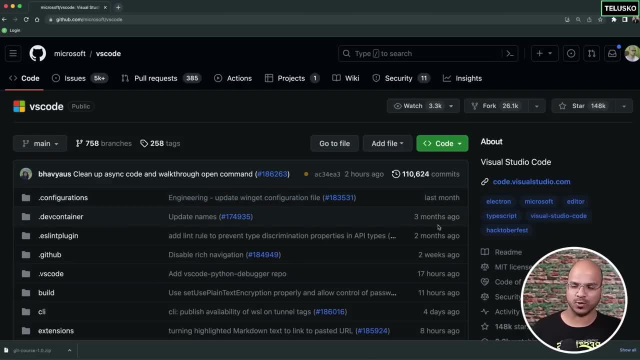 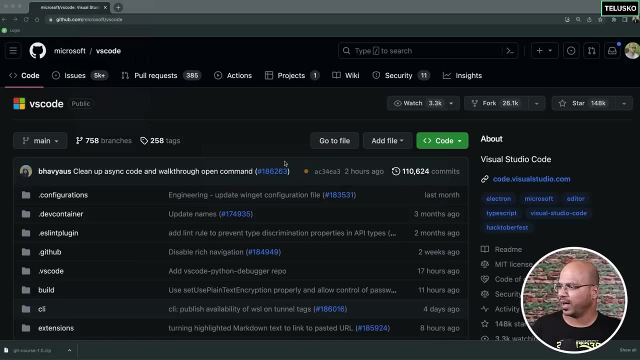 Now this is the actual source code of VS Code. Now the version which we are using is 1.79.. Remember when we were doing the last video? if you go back, code about. So this is the version right: 1.79.0.. 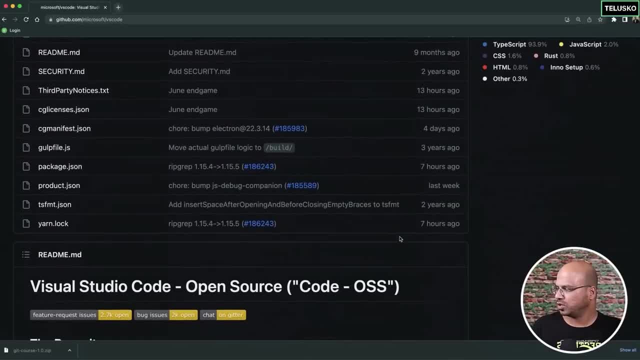 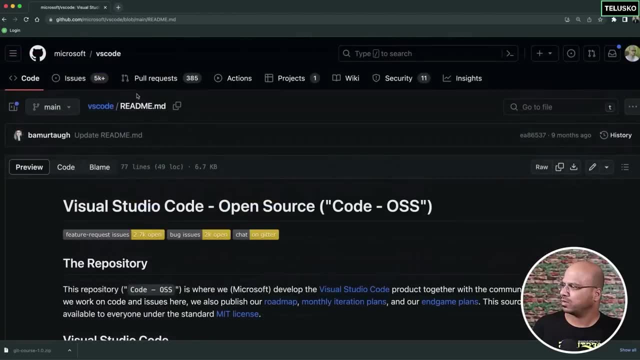 So the current version they have is what? So you know, every project will have a readme file. You can open readme file, which is here. It will have some updates, right. Otherwise you can just go here and you can look at the commit history as well. 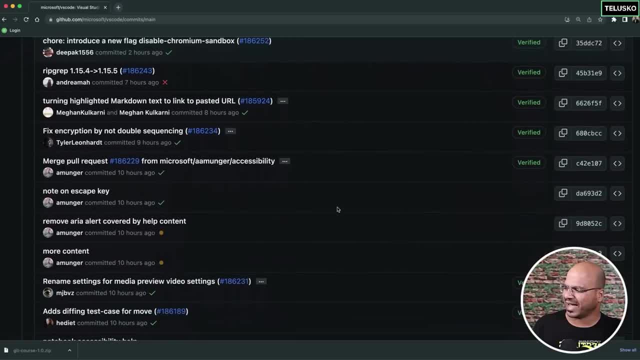 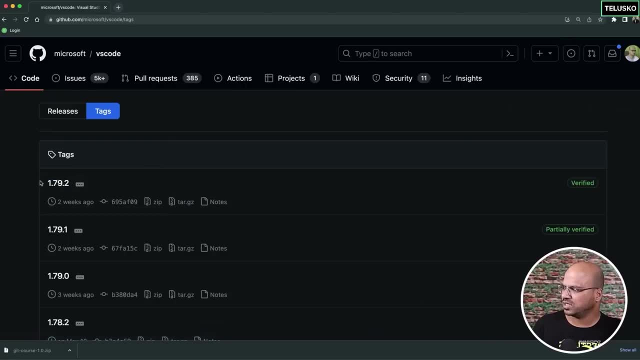 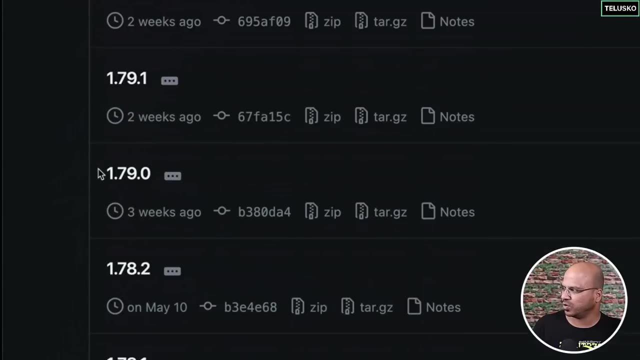 So this is the commit history And you will also find tags here. Okay, so if you go back to code and if you see tags, so you can see this is the latest version, that's verified, which is two weeks back, And this is a version which I'm using- 1.7.0. 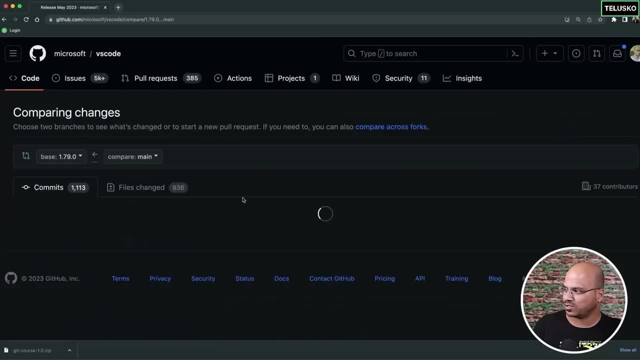 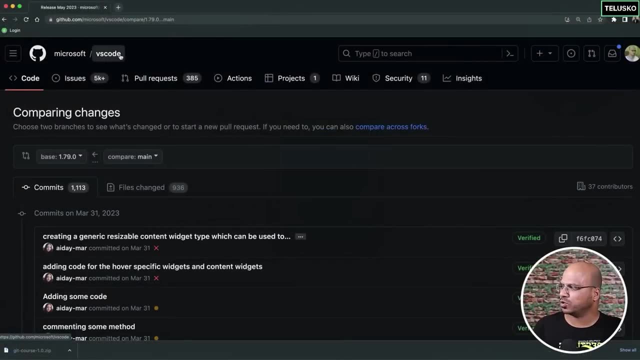 And if you want to see the commits of it. so there are so many commits for this particular tag And you can also see the numbers. So how will I get the source code? So if I go back to VS Code- and we have seen that right- 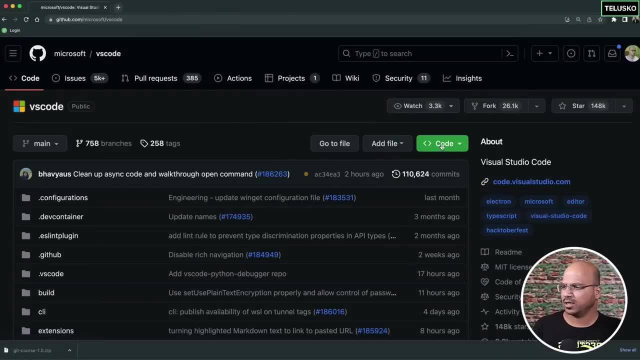 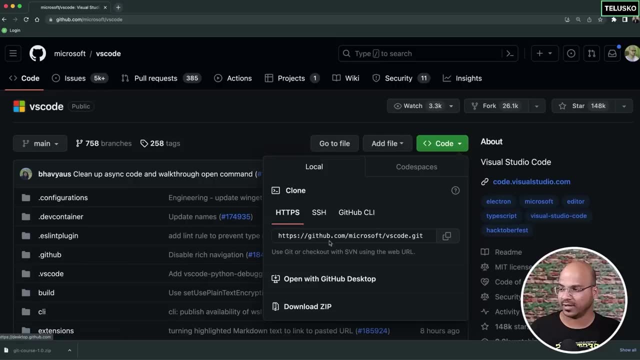 So if you want the source code, of course this will be a bulky project. So if I click here, you can see this is where local, this is where you can get the thing. You can also download the zip, but we don't want to do that. 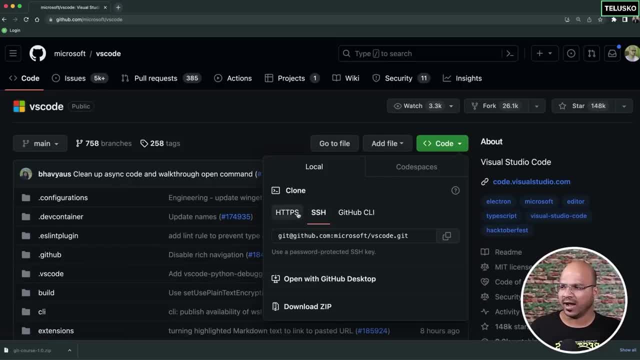 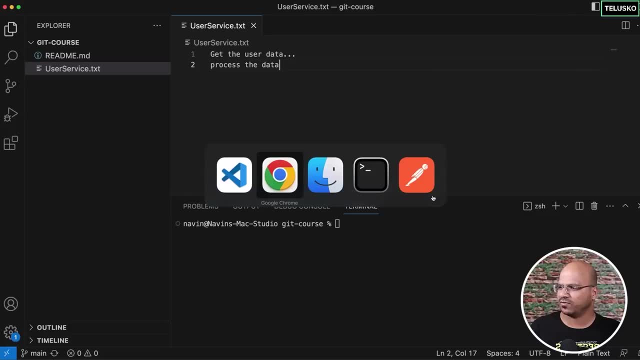 What I can do is I can use HTTPS or SSH, And of course I will not be pushing any code. So HTTPS works for me. I will just copy this and go back to. in fact, I will not do that in VS Code. 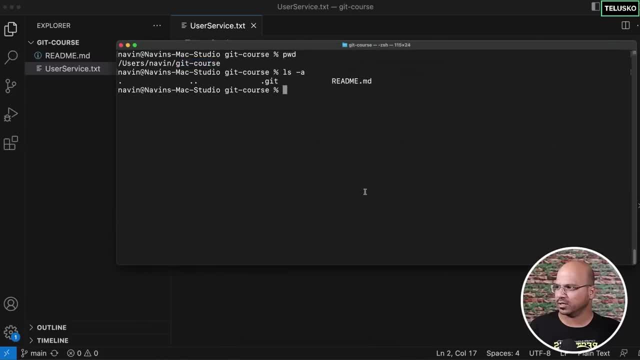 Let me use a normal terminal. So we'll go back to terminal here and I will say: let's go back to the folder. Okay, Let me see where I am. So I'm into my home folder. Let me just clear the screen. 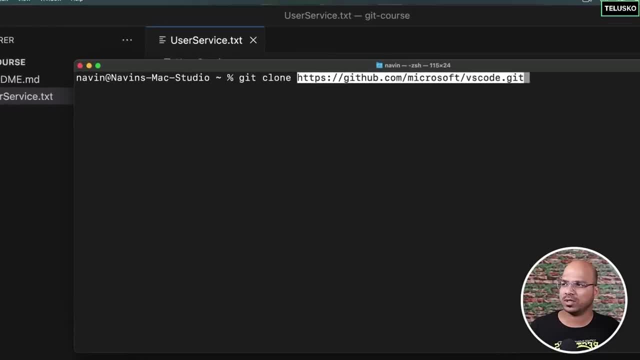 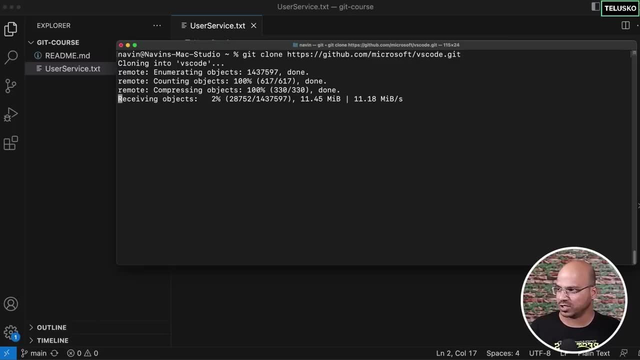 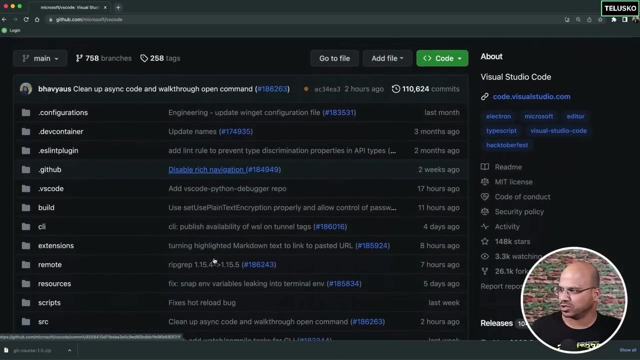 And this is where I will say git clone. I will mention that particular URL. The moment you say enter, it will download the entire VS Code repository in your machine. So it will take some time. So basically, the entire project which we have here, we are getting that in this machine. 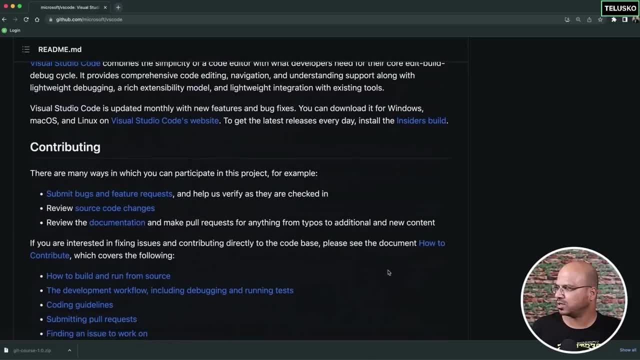 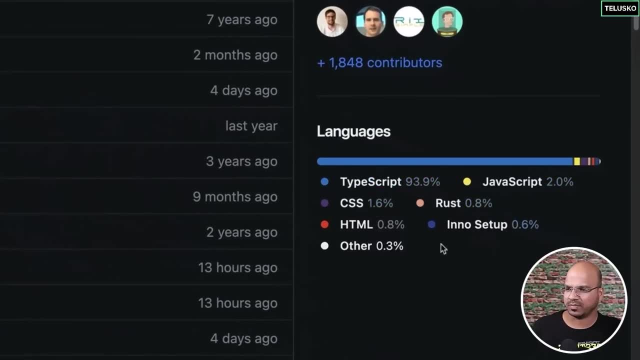 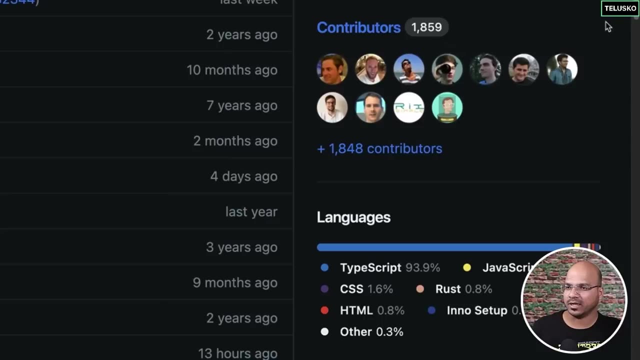 So, by the way, it is downloading. Let me see if I can find something interesting here. So the entire VS Code is built using TypeScript, 2% JavaScript. There's also Rust elements here and CSS, HTML and others. And you can see the number of contributors: more than 1800 contributors. 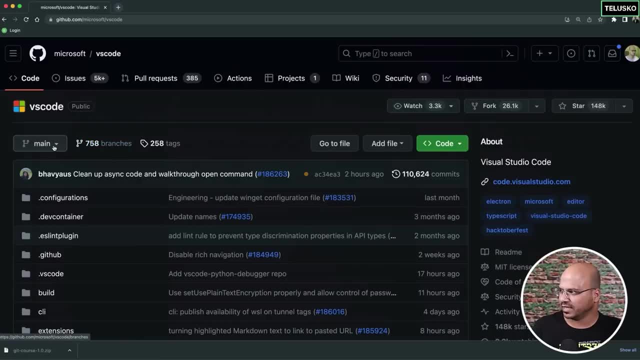 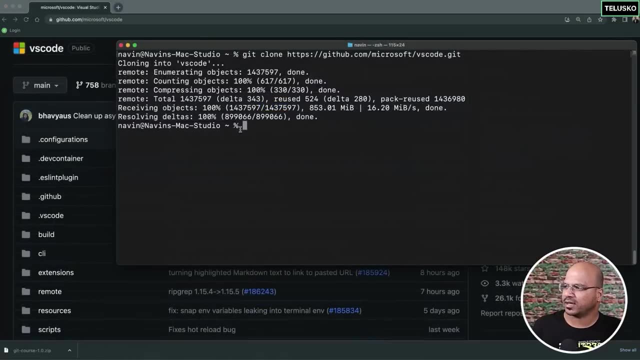 That's great. And then there's also branches here which we'll see later. But if you expand this, you can see there are so many branches here created. Important is the main branch, which is the most important branch here. Okay, done. 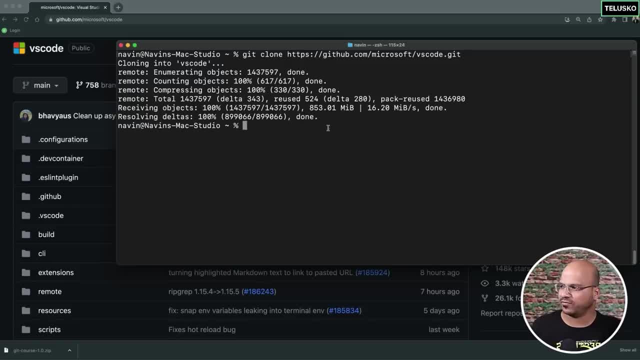 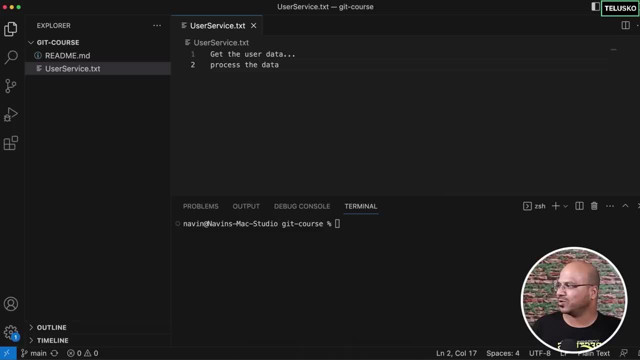 So you can see, I got the VS Code And what I will do is I will open that VS Code in my VS Code. Okay, this is inception, right: Opening a source code in the VS Code. So let me go to VS Code and open that folder. 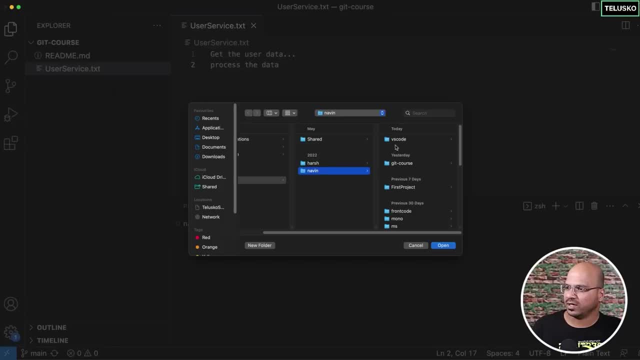 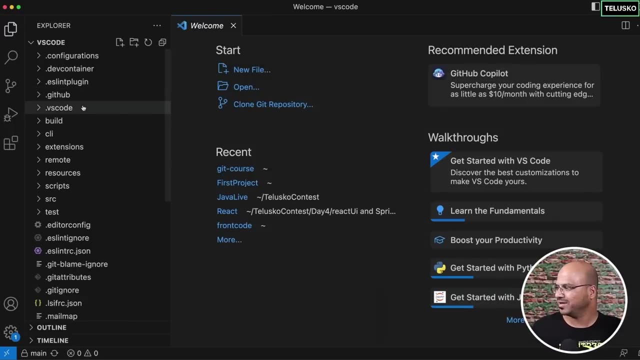 So I will say: open folder And in Naveen we got VS Code. Open And voila, This is the entire VS Code source code, right? So this is the entire code. In fact, you can also verify with the README. 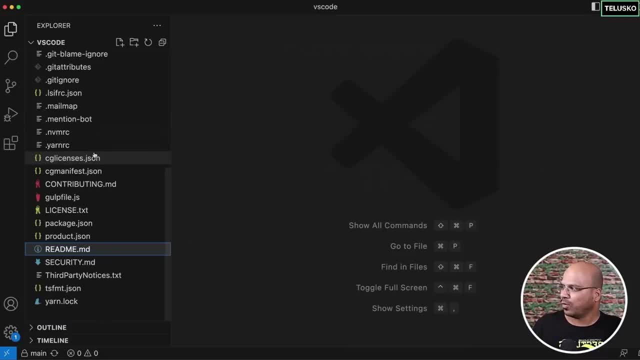 This is the README which we had there, right? Okay, Now what I want to see? I want to get some information about it. So what I will do is I will say terminal, and I want to know some things from this. 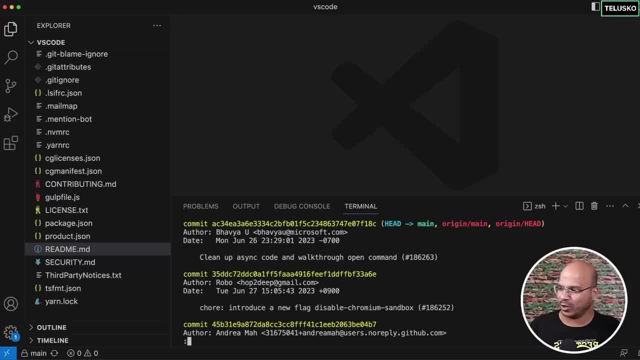 So basically I want to see the log first. So when I say git log and look at all the commits which happened here, So you will see their name, who has committed it and what is the email ID, You can see the time when it is committed. 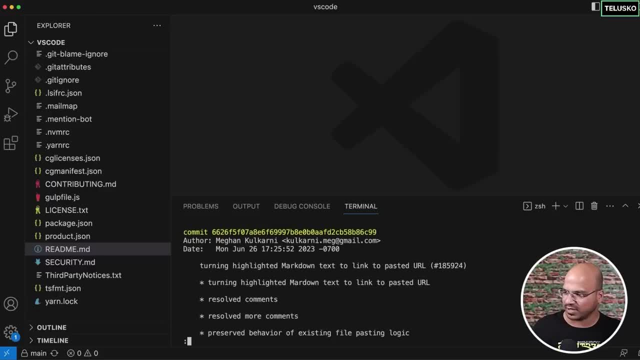 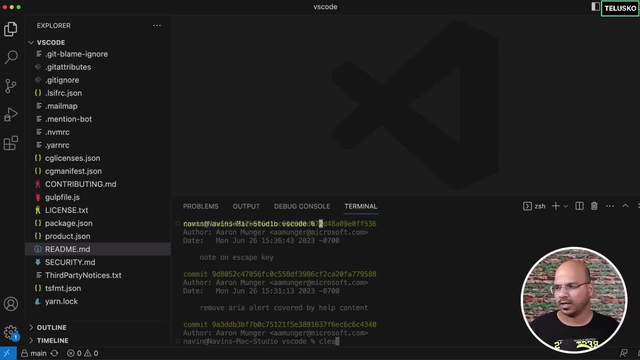 And if you say enter, you will see all the list. Right, We got the entire list And it will be huge. Now, if you want to come out of this, just type Q and you are out. Okay, And now what if you want to see all the tags? 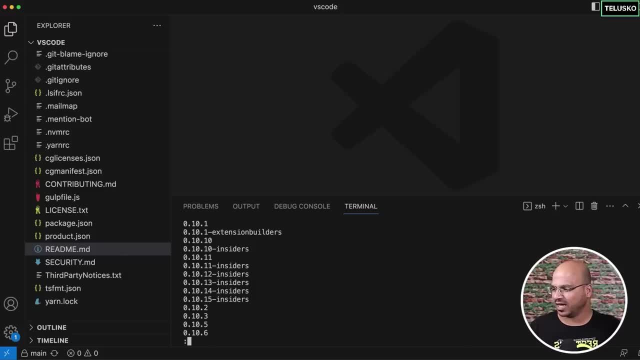 I can say git tag, because now we know the commands right And these are the tags. So they started with 0.10.1.. And if you go down, the latest one is 1.79.2.. Let's see. 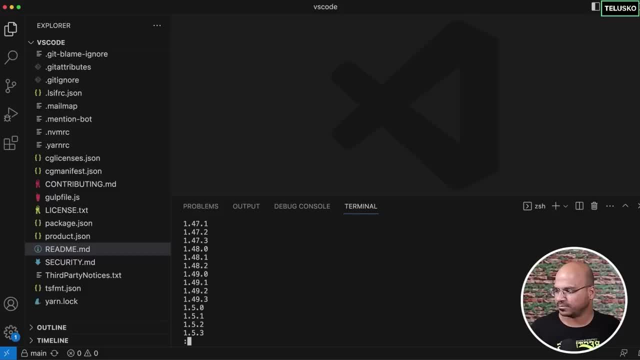 So if you go down, okay, still searching. So these are all the words, These are all the versions of VS Code. So you can see 1.9.1 is the last release. They have the tags. I'm not sure if they have publicly released it, but they have the tags. 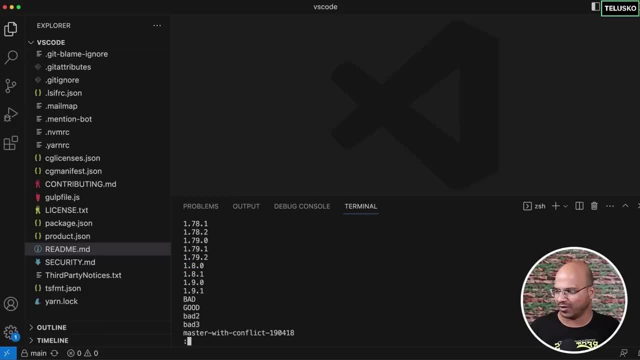 And this is the version which I'm using, And maybe I want to know more about my version which I'm using. So what I can do is I can say git show 1.79.0.. That's the version I'm using. 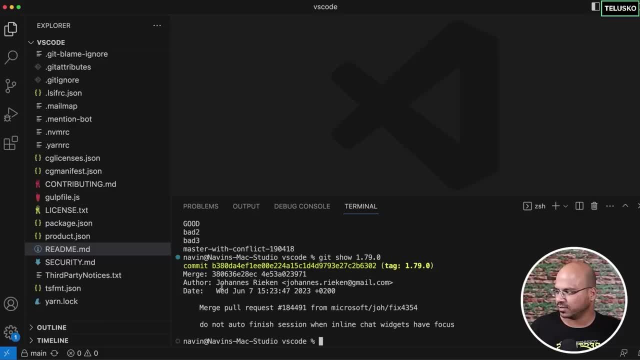 So you can see this particular tag got a commit from this particular author. So I can see the tag And I can see the version. This is the author And on this day, Oh great. And I can also see what they have done by exploring this commit, this particular commit. 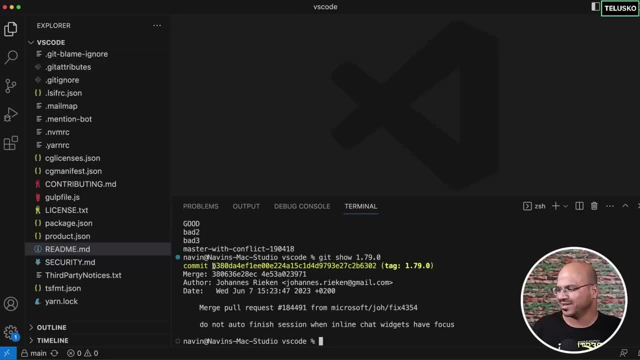 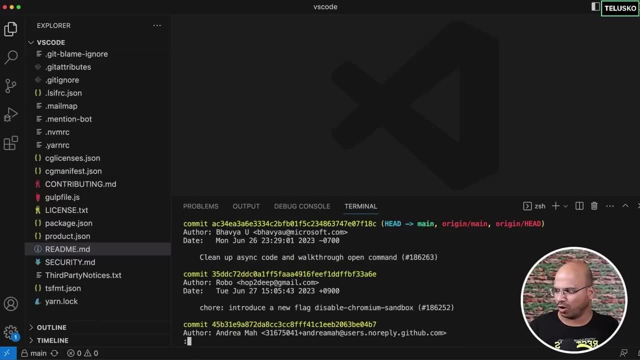 Okay, you can see I got the commit number now, So this was what I was looking for, right? So I don't know why I was not able to find that, But yeah, it's here. In fact, when you say git log, you can see there are a lot of logs here, right? 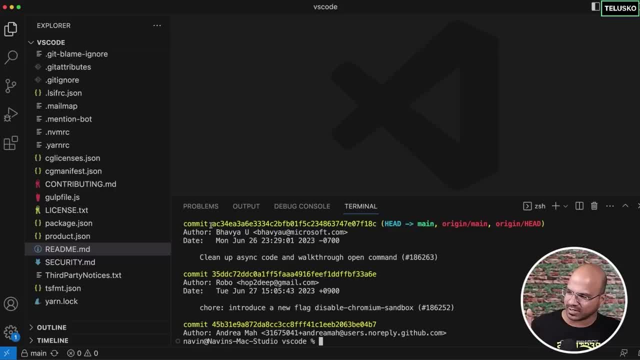 Now, if you want to print only one, I mean the commit number and just some information, there's one more way you can say: git log- Print Pretty One line. So what will happen is by entering this command, which is: git log- pretty one line- you will. 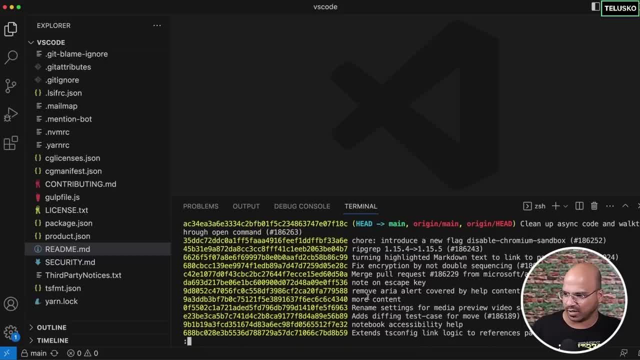 see the commits and the message there And this is how you message, right. So you will also get an example by looking at other people's commit how they message something. So you can see we also have some number, issue number and upgrade numbers. 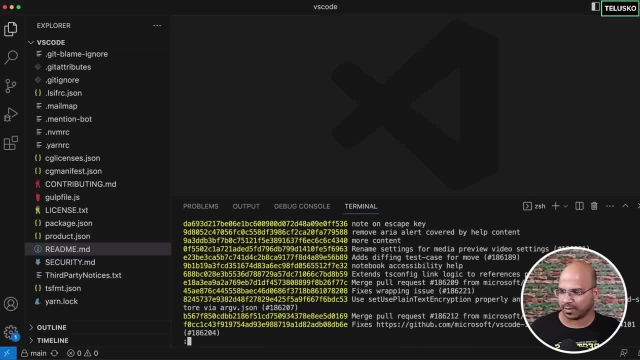 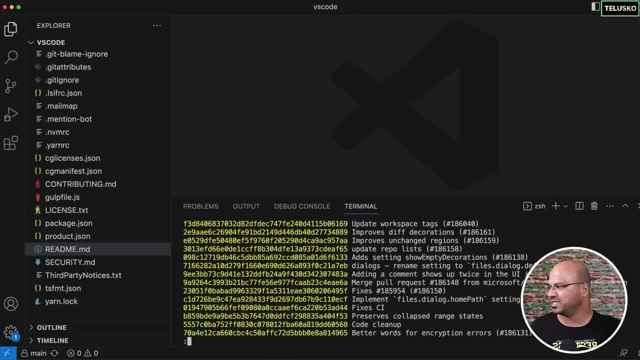 So it was always helpful to look at other people's comments or messages so that you will know how you should be writing your message. Now what if you want to make some changes? Let's say, if I go back to any of the file? this is the first time I'm downloading the 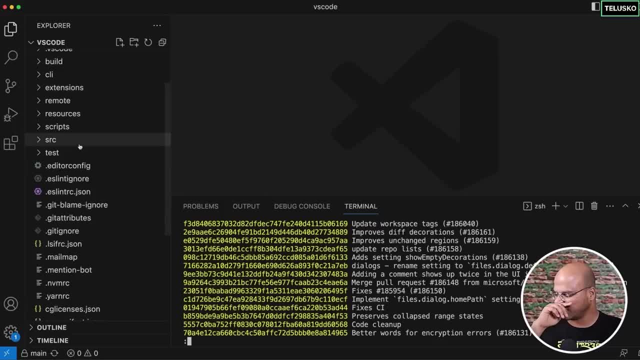 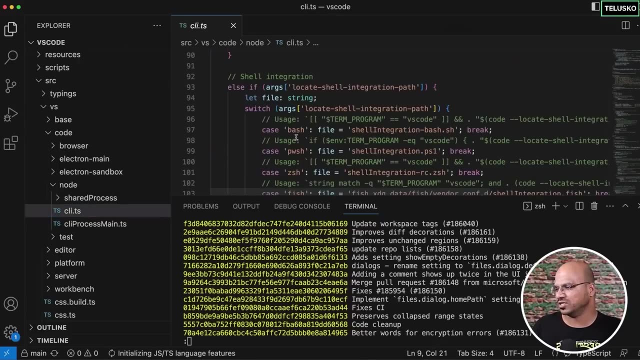 VS Code on this machine or exploring the VS Code source code. I can just get into source code and VS, let's say code. There is some node code here, Okay. So let's say, in this particular file if I want to make some changes, I'm not sure will. 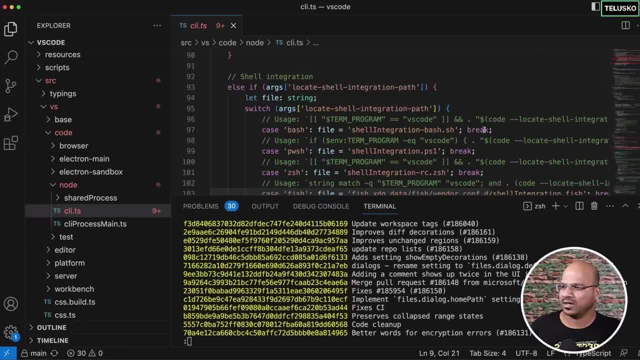 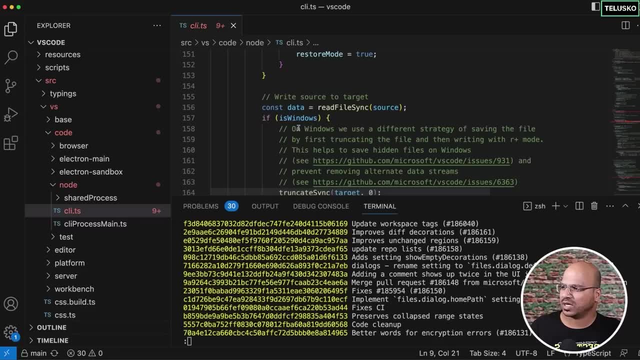 it work if I make a change. But if I make some change, let's say, is it here? Is there anything where I can type any message here, an existing message? Let's say, I just want to say on Windows. let's say, I give a colon. 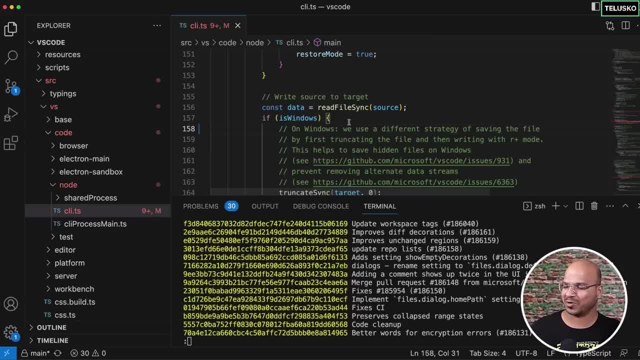 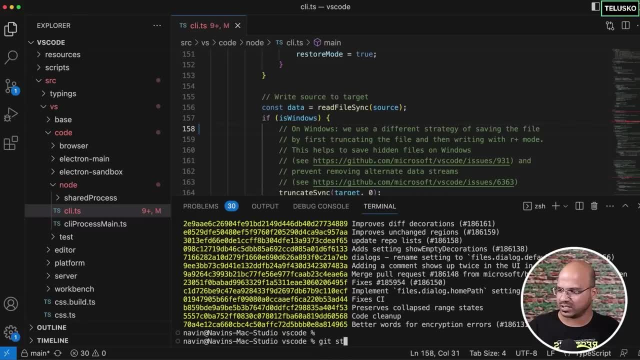 Maybe I have done a very big upgrade to this particular project. Now how would I push it? Of course you have to commit in your local machine first. So what you will do is you say, if you say get status, and you can see that I have changed. 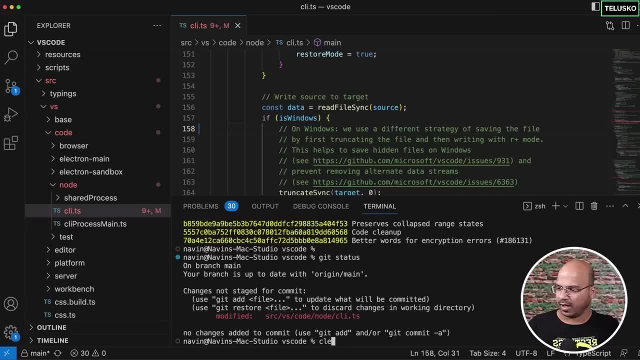 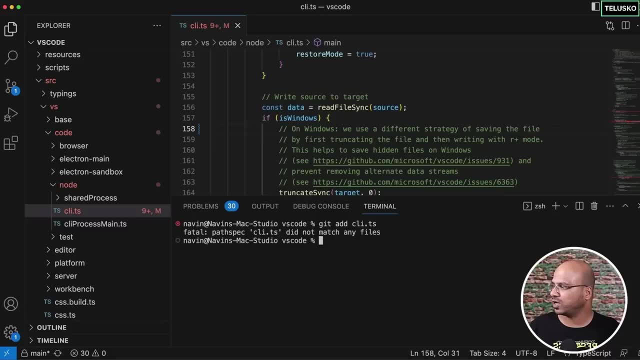 one file. This is a file which we have changed a CLIts, And if you want to, you have to add it first. You have to say CLIts, Okay. So first of all you have to get the path right. 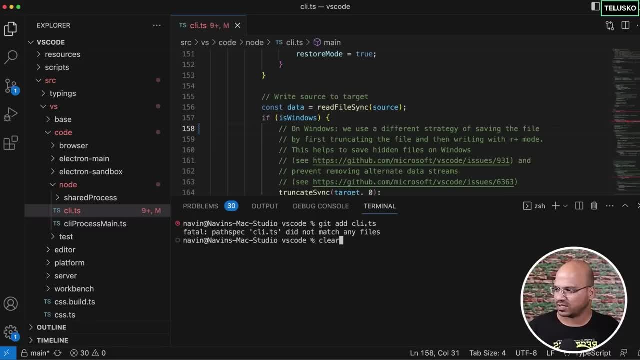 You have to go to that particular path and then you have to say commit. So if I say get status again, this is the path which you have to go for. So I will just copy this. Let's say: git, add, Enter. 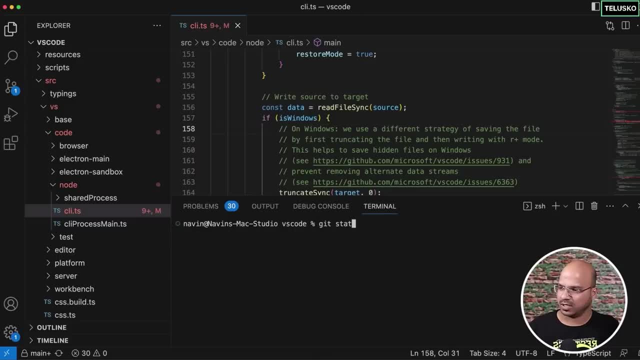 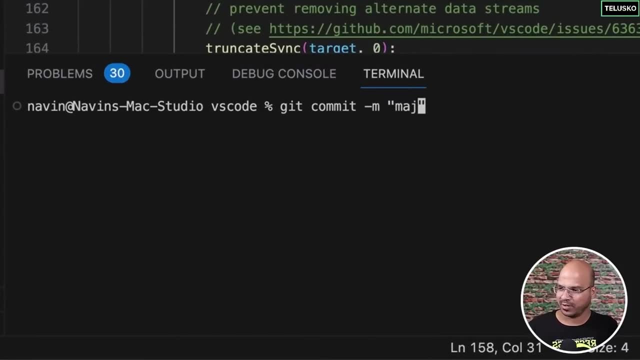 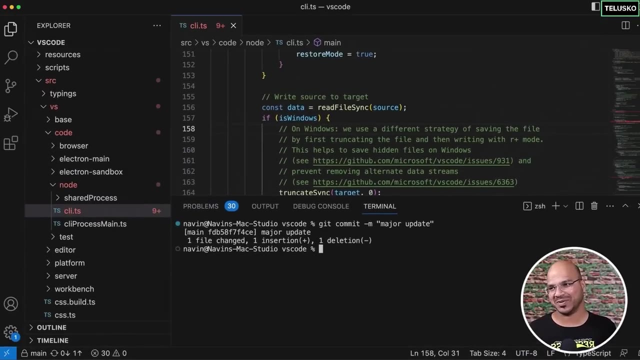 So that's the path Done, And now I can simply say commit, So git, commit hyphen m And I will say major Update And I will say enter And done. The commit is done. But that's only in my local machine, okay. 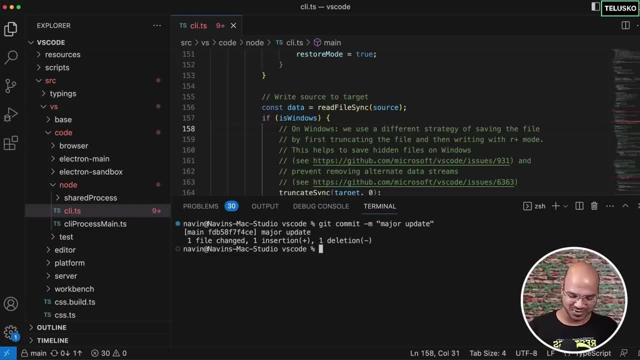 And now, if I want to push this to the server, let's try what happens. Even if something goes wrong, we'll see later how do we solve it Now. first of all, I want to know the remote right, Because how will I push? 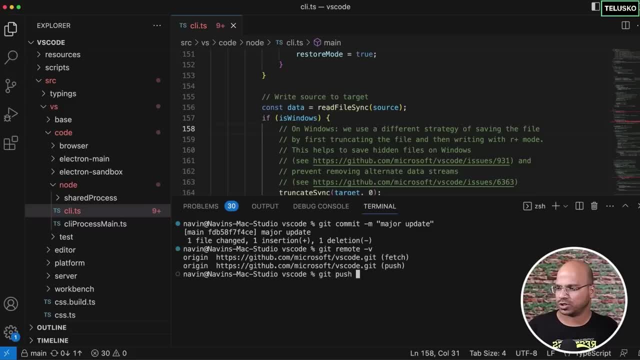 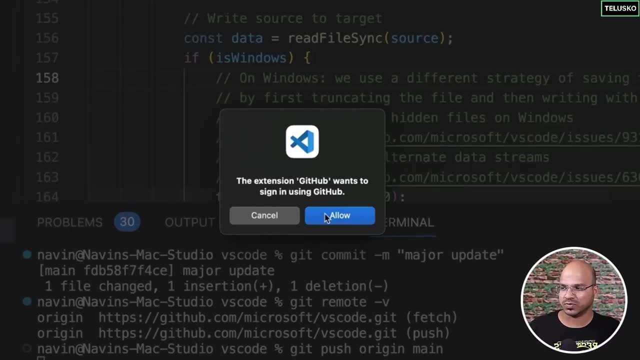 So remote is origin. So I will say: git push origin main. I'm just trying to push in the main Enter, And it will ask you for the username and password. The reason it is asking me to sign in is because I want to know the password. 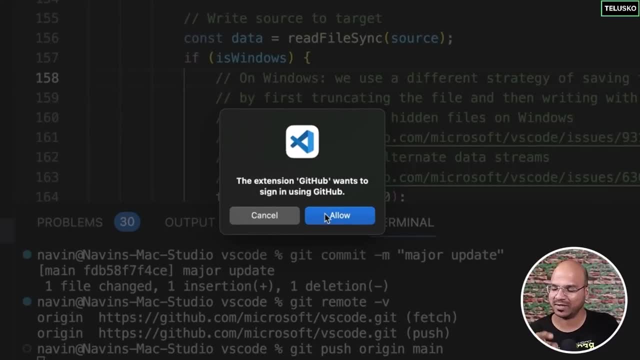 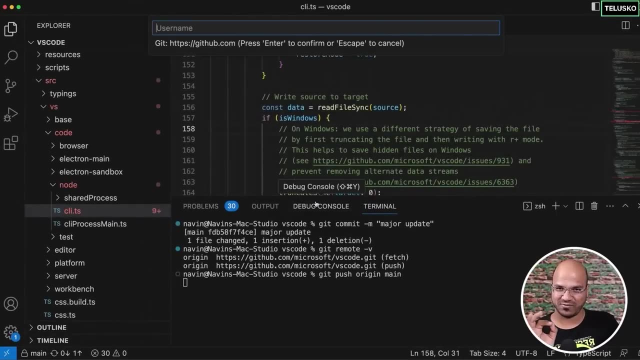 The reason it is asking me to sign in is because we have used stdps right And if you don't want to mention username and password, basically we have to use the SSH. Now, even if you are logged in, it will not allow. 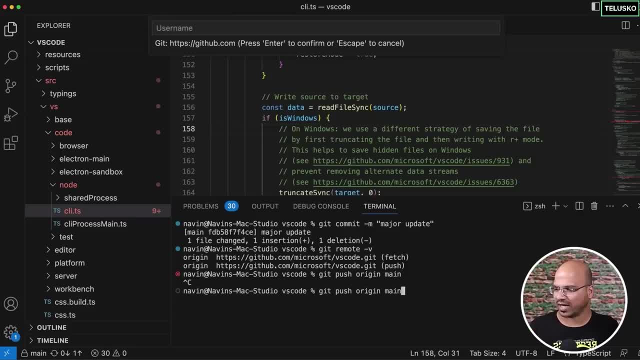 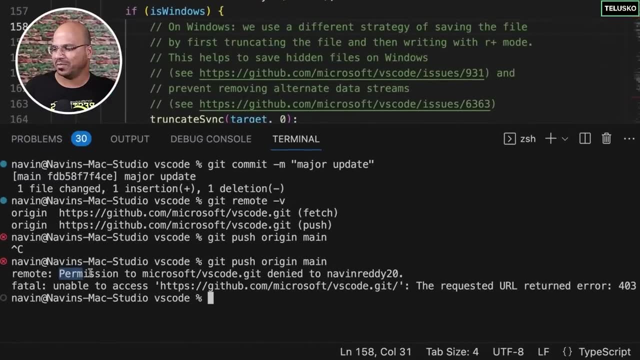 In fact, let me just try that once again. I don't know why I have canceled it. Okay, So it's authenticating And done, So you can see I'm logged in, But it says permission to Microsoft VS Code git denied to this particular user name. 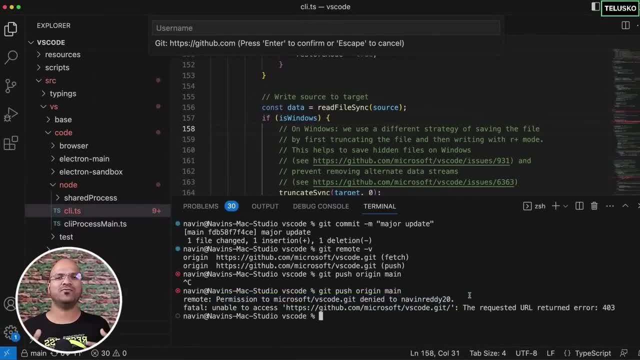 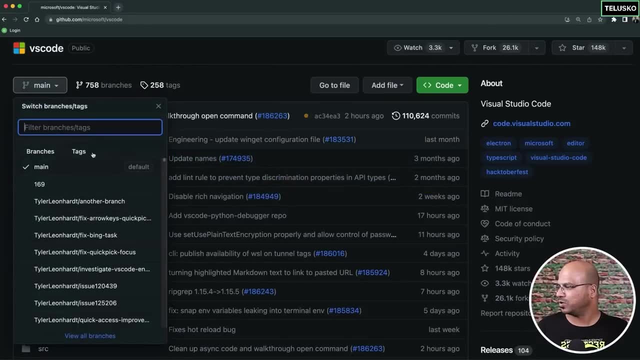 So I'm not allowed to do that, Right? So I can basically fork this project, Or maybe I can just create a branch. Even that is not allowed, Let's try if I can create a branch here. You can see, you cannot create your own branch. 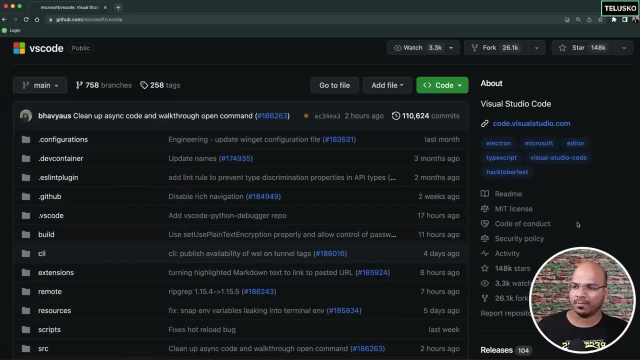 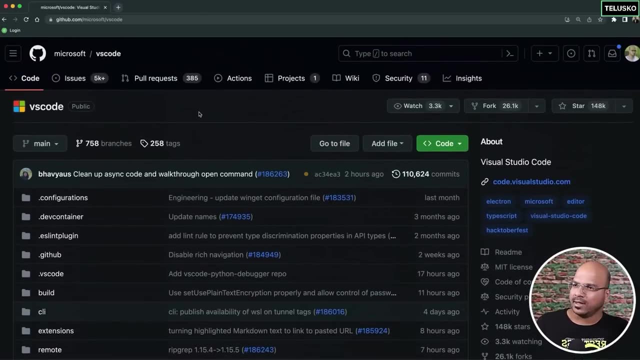 Right, So you're not allowed to do that, So you have to be a part of a contributor here. So once you're a contributor, then you can do that. That's how you basically work with the projects, Okay, So we have done enough talk on this. 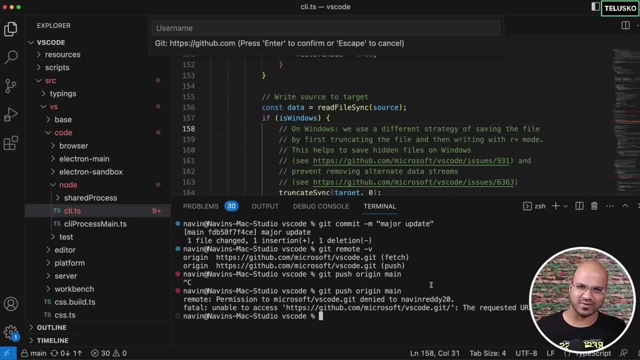 We'll try to see how do you push in your own project. In fact, we have seen that in the upcoming videos, we also work on branches, which will be quite fun. So, yeah, that's it from this video where we have seen how do you download a source code. 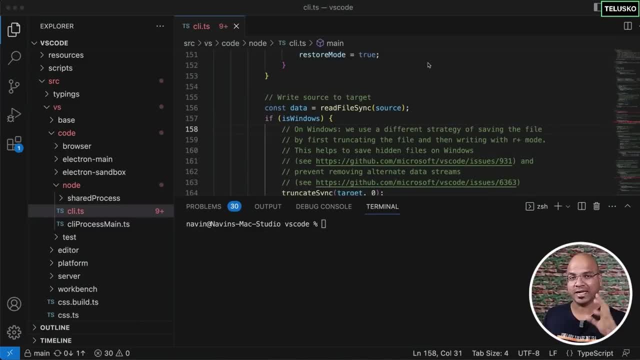 and do some experiment with it. We'll talk about the git branch. Now, this is a very awesome concept which is there in git, And this is what makes git one of the best version control system. Now, what exactly branching are? How do we use it? 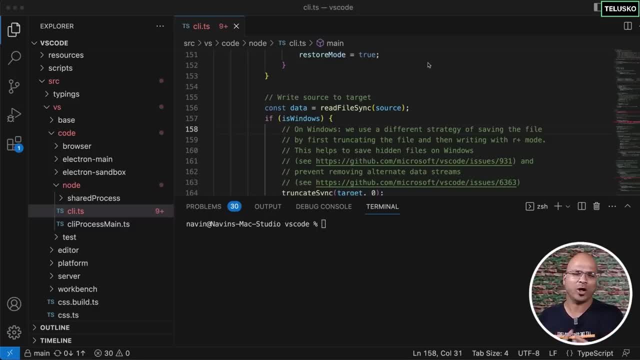 How do you merge two branches And what may go wrong when you merge two branches. We'll try to understand that in the next few videos. So let's try to understand what is branching first, And for that we need to get back to our project. 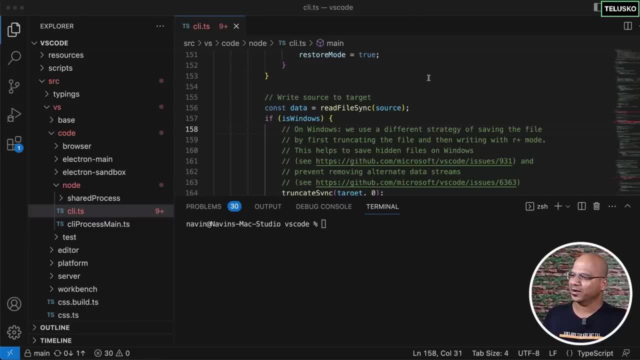 Now, this is what we were doing right on VS Code. We were able to get the source code from the GitHub, But then we don't want to work with this, of course, because even if we can do some changes, I will not be able to push on the remote repository. 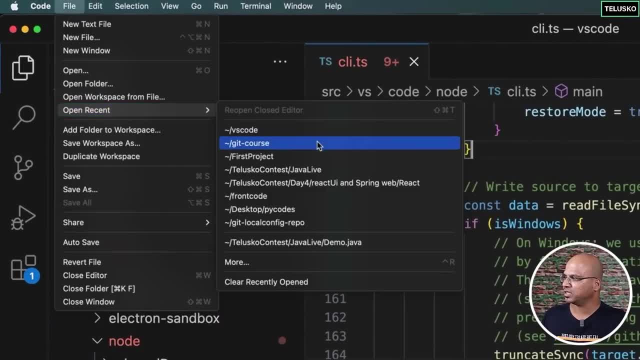 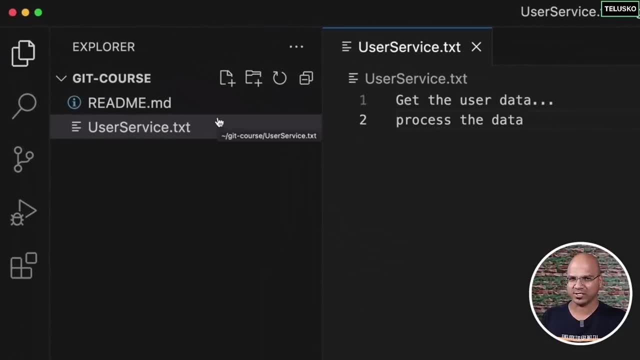 So let me go back to our repository, So I will say: open recent git course. Now this is what it looks like. This is a project in which we are working right And, if you observe, we only have two files here. 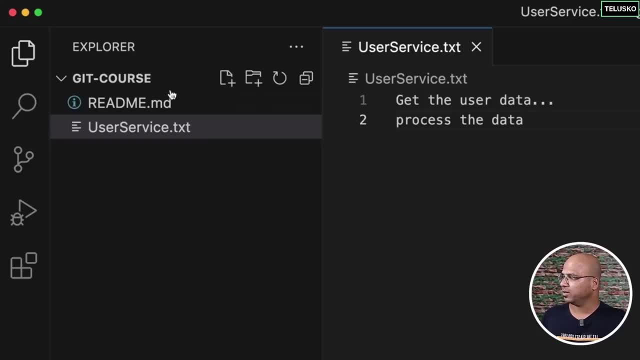 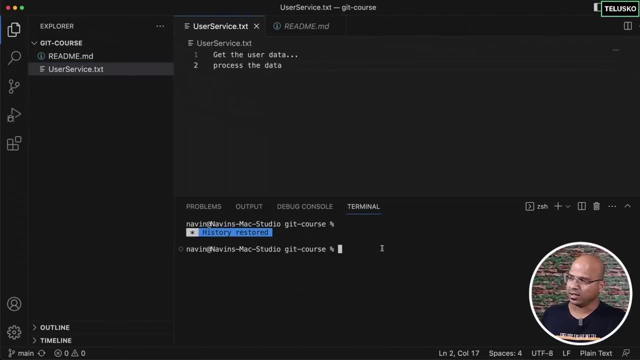 Nothing fancy, just two files, And we got readmemd, We got user service text- Okay, makes sense. And then the first thing you have to do is you have to always check git status. if everything is committed, You don't have anything in the unstaged or modified stage. 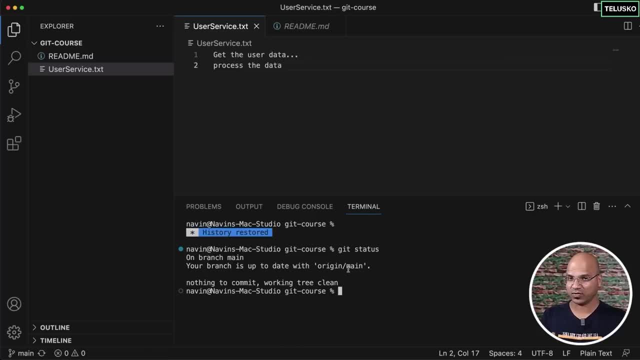 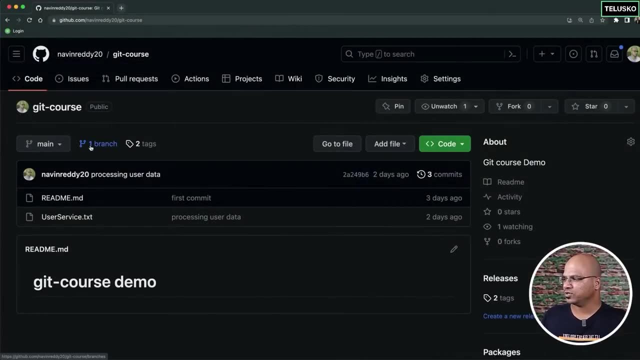 So you can see we have git status. Everything is clean, So we can go forward Now if you go back to your GitHub and if you see we are into git course now. So basically, if you see there are different things on the screen, 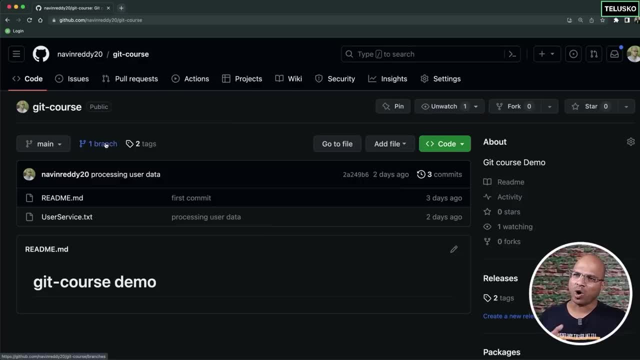 One thing interesting is we have one branch. Now what exactly this branch means. See, the thing is: whatever you do, okay, whatever work you're doing and you're pushing from your client side to server side or your remote repository. 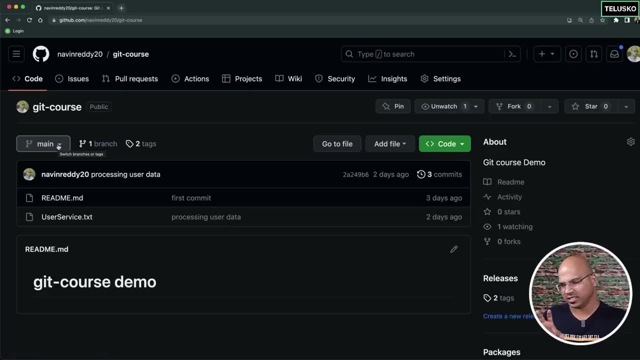 you have a branch and this is going into the main branch. Now, this is the name of the branch, which is main, And by default when you create a project, of course, you do get either master branch or main branch, based on which version you're using. 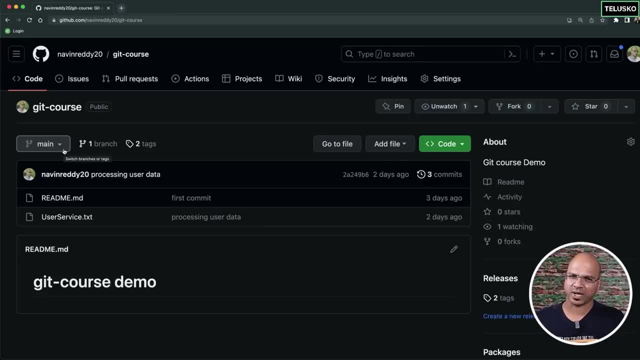 and which tool you're using. So you have to check this. What is your branch name, first of all? So for me it is main, And you might have some other branch. That's completely fine, And there is no rule in the world that you should have only this branch name or that branch name. 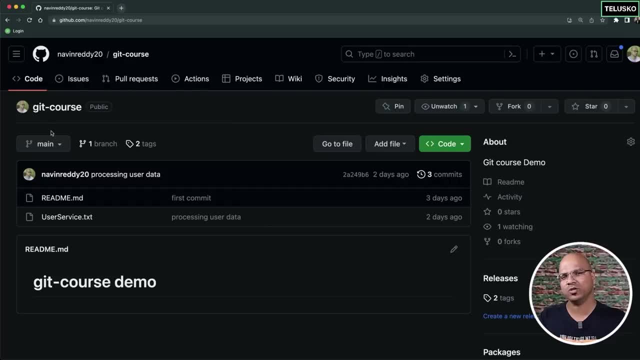 You can go with any branch name. That's your choice, But commonly we use main nowadays And you can see we have one branch. That also means we can create more branches, right? So whatever by default you're doing, that goes into the main branch, right. 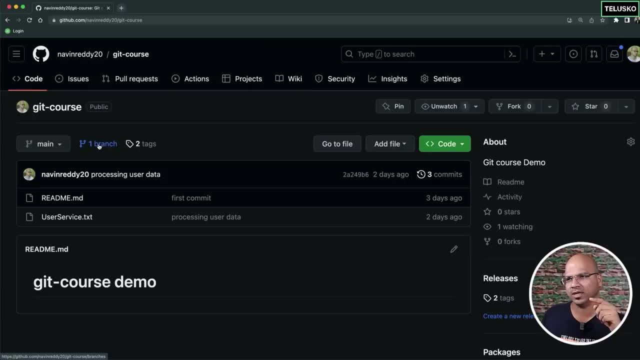 And if you remember, when we were pushing the code from the git client or the terminal to the server, we were using main as a branch. So we used to say: git push origin main right. But what if everything is working? So let's say you have a project, everything is working. 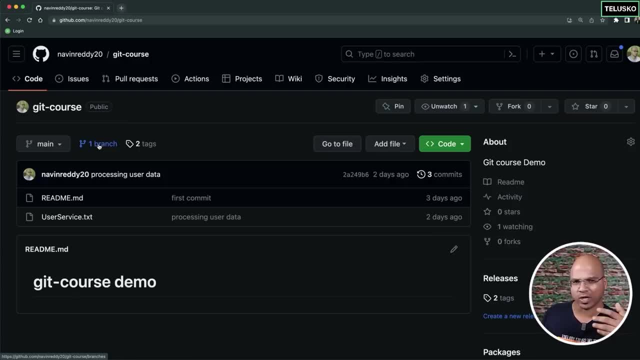 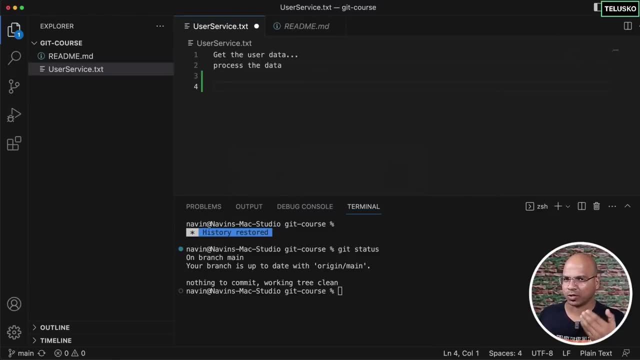 and now you want to do some experiment. Now, one of the things you can do is you can, of course, you can do experiment. Let's say, I'm happy with my code, which is working fine, And then I want to do some experimental code in this user service. 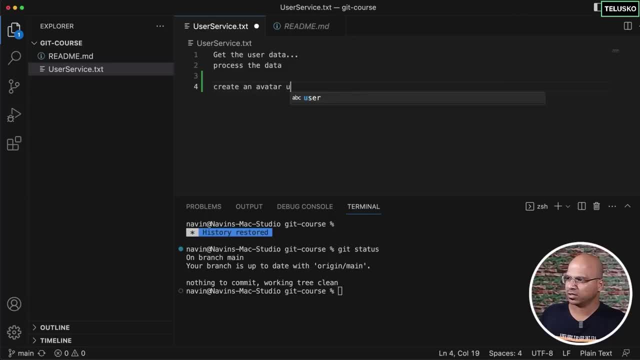 Maybe I want to create an avatar for a user. Create an avatar for a user, And all these are experimental. okay, I'm not sure how will I do it, So I'm just trying to add this feature. And now, let's say, this is a very bulky code. 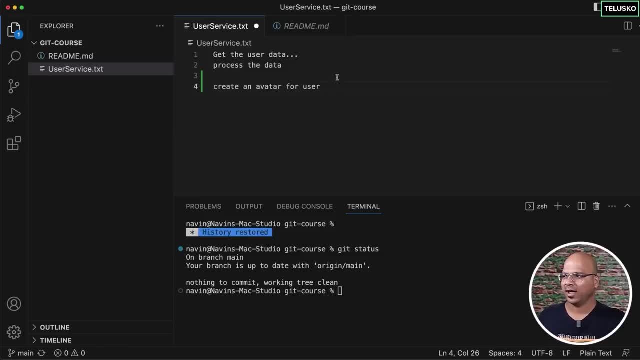 And this is not the only file you're changing. Maybe you're changing multiple files And you thought it would work And now it's not working, okay. And then the release which you did to the users, the earlier version. it has some bugs, okay. 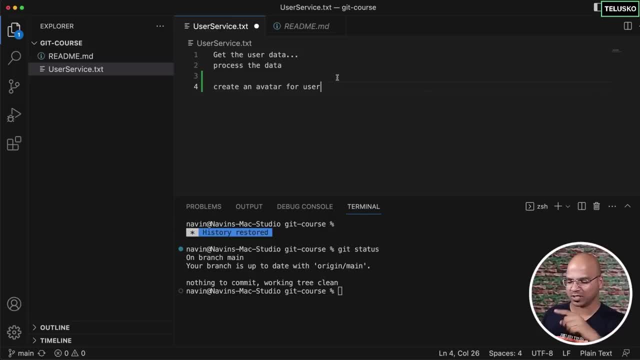 And how will you solve this? How will you solve that bug now? Because the moment you make changes and when you push this to the server, when you push this to the GitHub repository, how will you come back? Because you have updated your main? 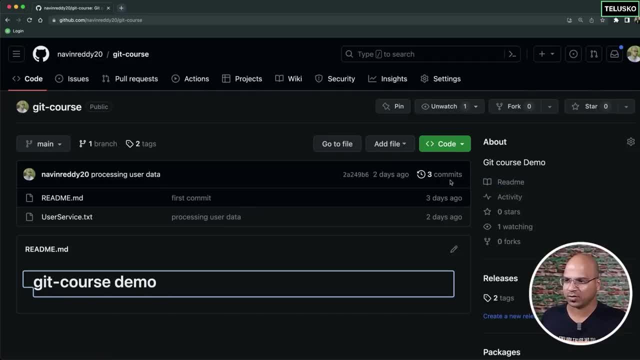 See, one thing you can do: you can go back with the commits. You can. you know we can actually try and travel between the commits So you can go back to the previous commit. But again, why to do all those things? 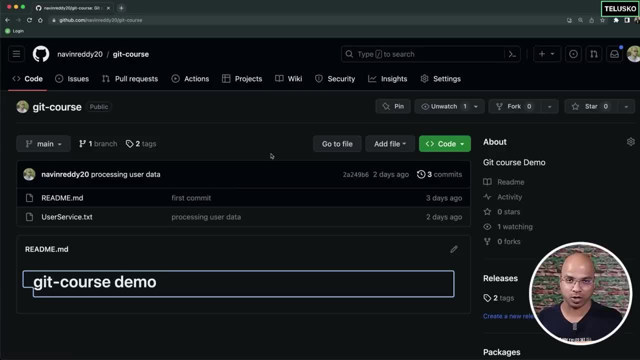 What you can do is whatever experimental feature which you are working on, or maybe your colleagues are working on, so you can work on a different branch. Now, this will not affect your main branch. okay, Example something like this: You can just click here and you can have an option here of creating a new branch. 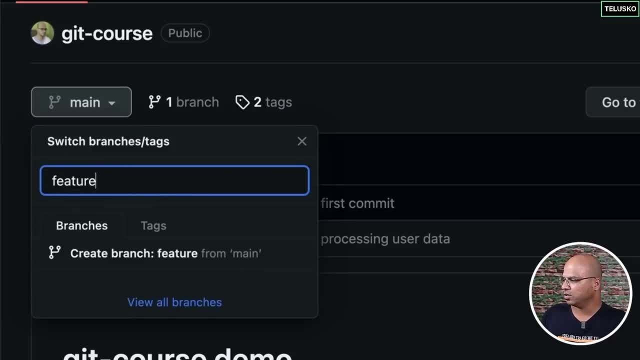 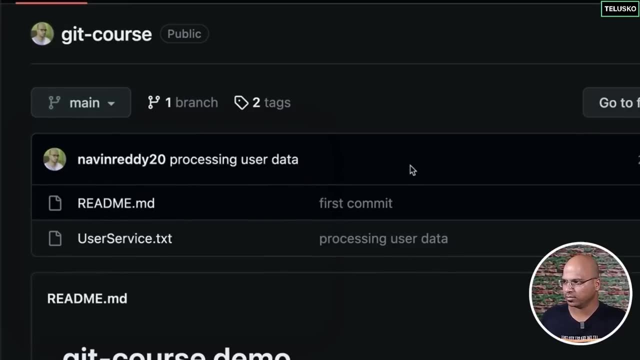 You can simply type, let's say, feature 1.. Now, this is a new branch which I'm creating here. okay, So you can do it from here on the GitHub or, which is the best way we can do it, from the command line, right? 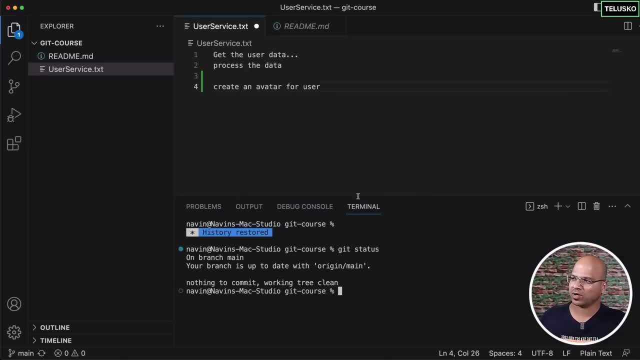 So let's go back here and let me create a branch. So what I will do is, whatever changes I want to make, I will not do that in the main branch, I will do that on the main branch, I will do that on a separate branch. 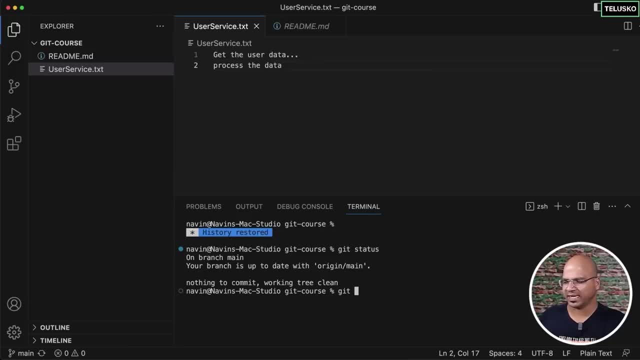 Now, first of all, we have to create a branch. So how do you create a branch? It's very simple. You simply say get. There are two options basically for branching. One is checkout. Now, this is the older one and most of them are familiar and used to checkout. 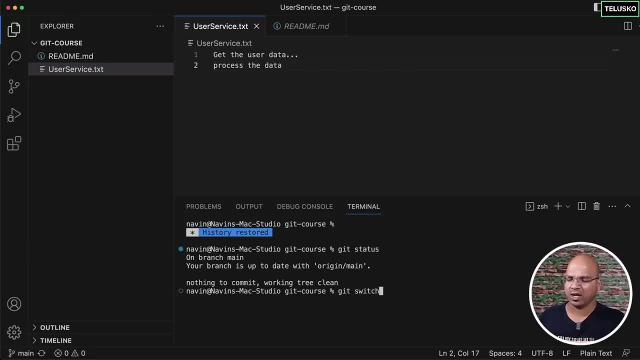 The new feature or the new command which we got is switch. I think this came in 2.23 version, So both are okay. If you want to use checkout, if you want to switch, that's your choice. Now, for me, I feel switch looks much better than checkout. 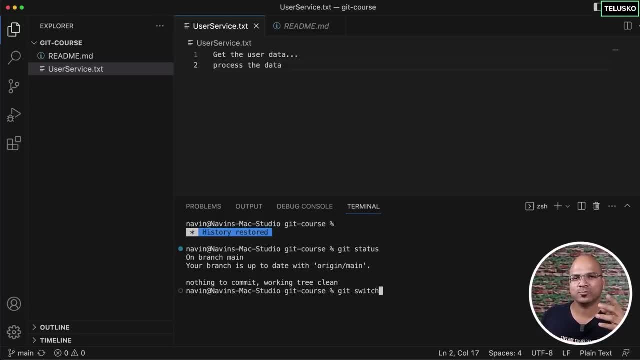 because sometimes you get confused with all these words. right? When do we use pull? When do we use fetch? When do we use checkout? So switch actually makes sense when you want to switch between two different branches, right So. but then let's go with the older one, which a lot of people are familiar with. 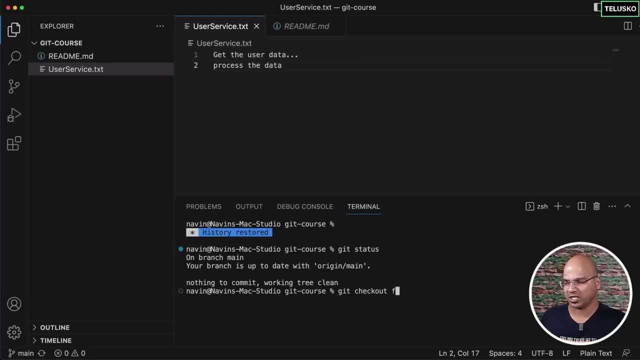 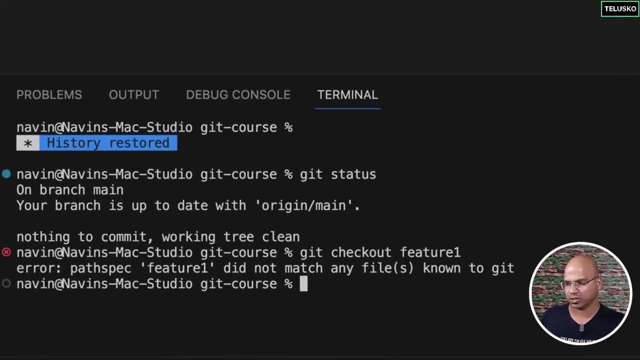 So you can simply say checkout and you can mention the branch name. So the branch name is feature one. Now this branch is actually not created. Okay, So we don't have this branch yet. And if you type this command and if you say enter, you can say it will say the feature one did not match any files known to git. 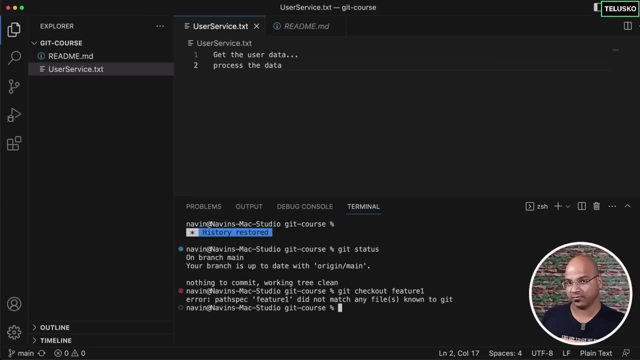 So basically, we don't have a particular branch name feature one, So we need to create one. So for the first time you have to create a branch right. Once the branch is created, you can switch using git checkout feature one. 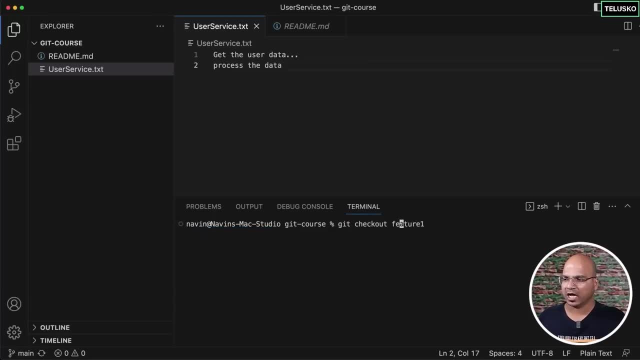 So what I will do is I will just type this command once again: git checkout. Now, since we are doing this for the first time, if you want to create a branch, you have to say hyphen B, or you can also say hyphen of a branch. 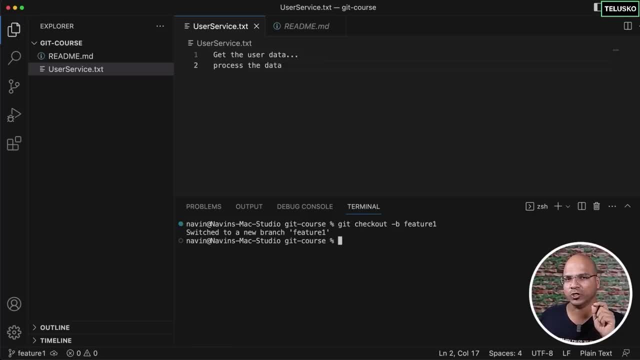 Both works And the moment you do that, it will create a new branch. Okay, So now the branch name is feature or feature one And it also says: you know, switched to a new branch, feature one. So basically now you have two branches. 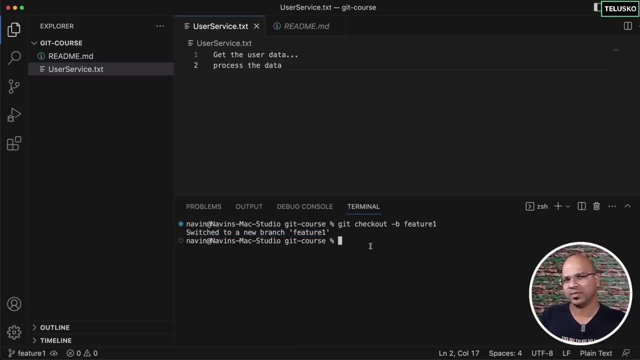 You've got a main branch and you've got a feature one branch. How do you know how many branches you have? So what you can do is you can say git branch and you can see: now we have two branches, We have feature one branch and we have a main branch. 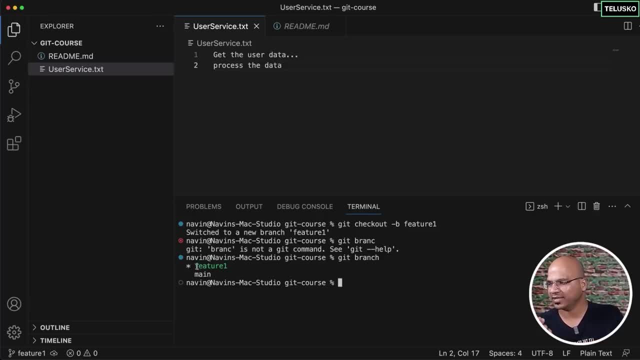 Now the question is which branch is active, And that's where you will see this star. Okay, So star means you are. I mean, this is basically a pointer which means currently you are on feature one branch And you can see. it's also in green color. 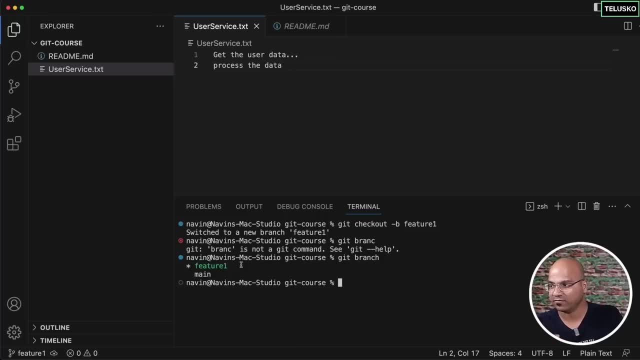 Now, whatever changes you make will be happening in feature one. Let me show you. Let's say, I will do some changes here. Okay, So I'm adding new feature because this experimental branch right. So I will say: Create an avatar for user. 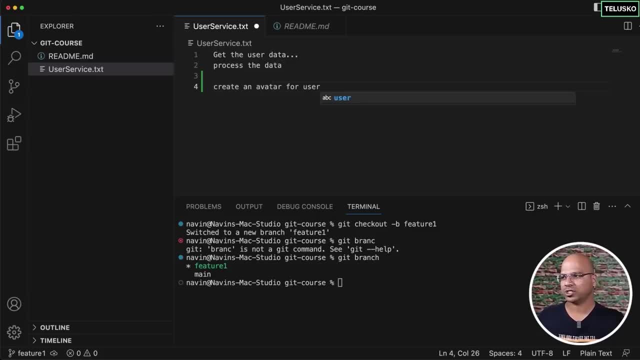 Okay, I will say save. And imagine this is a lengthy code. I'm just typing one line, But yeah, it can be a lengthy code. So once I do that, what I can do is, of course, I can say git status. 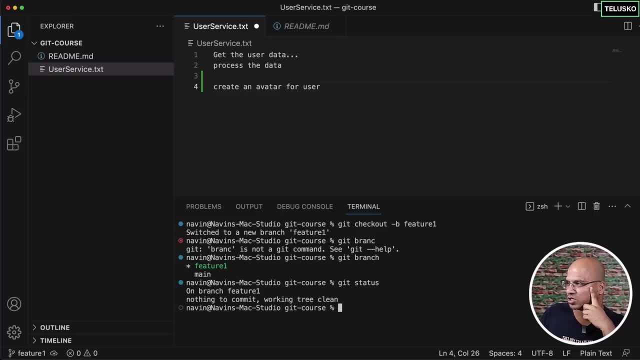 And you can see in git status it says on branch feature: Okay, It's not saved. Okay, My bad, I was expecting some unstaged and then it was saying something: Okay, Now it is. You can see, I failed to save it. 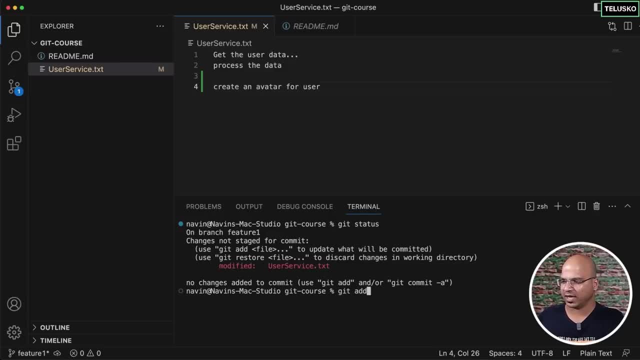 So it says modified. Now, once it is modified, you have to say add and you have to mention the file name, And then you have to say git. You have to commit this right. So you have to say git: commit hyphen m. 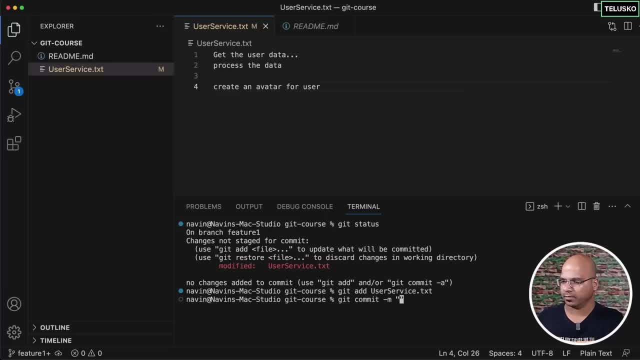 And you can send the message. You can say: experimenting with user avatar, Okay. So basically, we are doing experiment with the user avatar, That's what I'm saying here, And I will say: enter Now, this is committed. Okay, Now question arise. 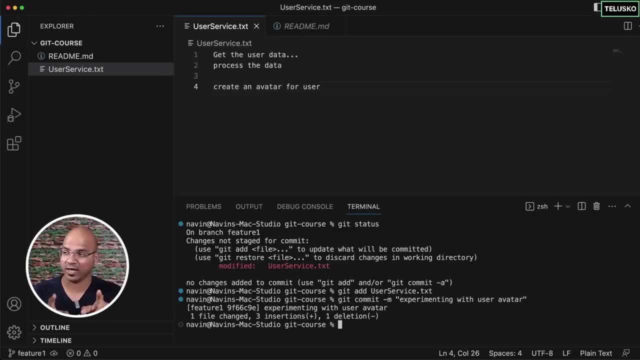 In which branch it is committed. It is committed in the feature one branch. Okay, Main branch has no idea what you're doing with feature one branch, So you can imagine this is your main. So this was your last commit right Before doing the branching. 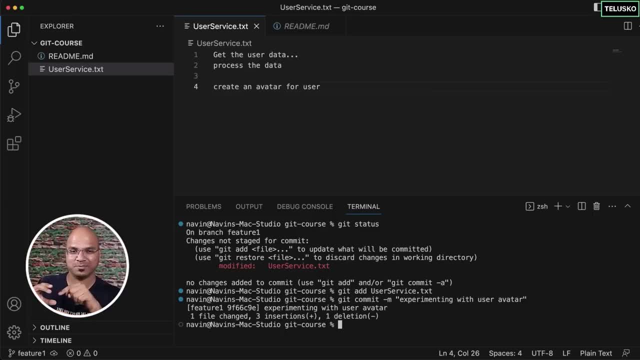 This was your last commit And main knows about this commit. Now what we did is we have updated some feature in a feature branch. Main has no idea That's a new commit And only feature knows it. Feature one branch knows it. 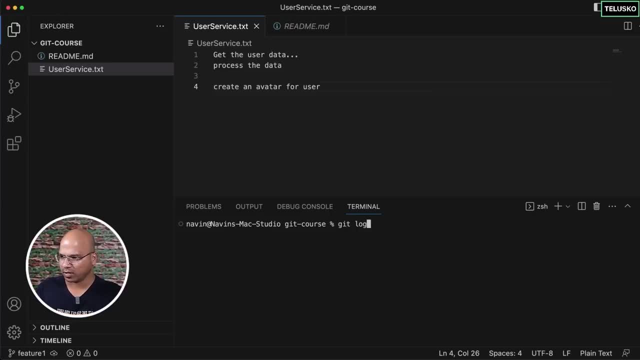 Okay, So this looks cool. right Now, if I say git log So you can see, it will give you all the commits. This is a recent one, You can see. this is a recent one. It says experimenting with user avatar. Just try to remember this. 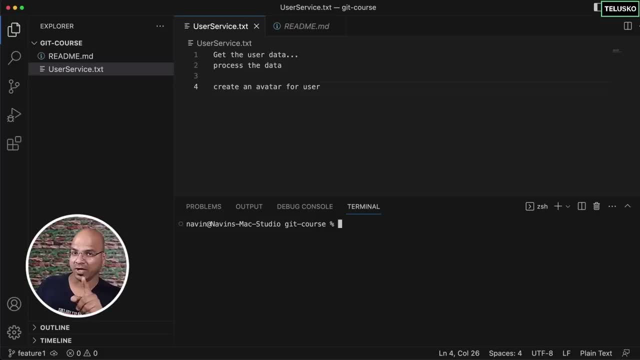 Now what I will do is I will just go back to the main branch And look at the code as well. So this is my working area, right? Look at this code. So the user service has one more line here, right? But if I move to main branch, how do I switch? 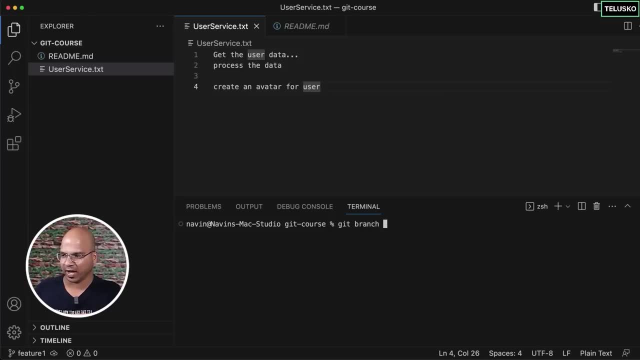 How do I switch between these two? So you can say git branch Or the git switch. So either you can use checkout or you can use switch. I'm using switch now You can also use checkout. That also works. I'm switching to main. 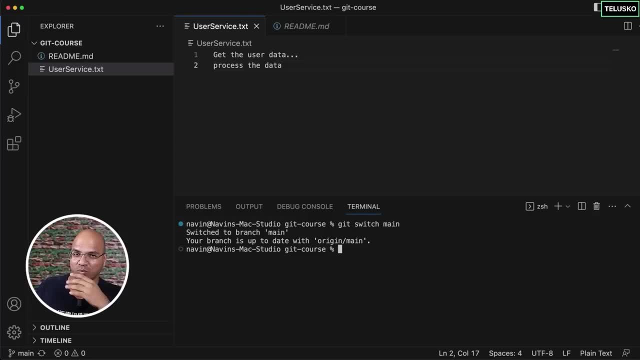 The moment I do that, look at the changes That line actually went. It's because main has no idea about that new line. But if I go back to feature once again, you got the new line. So this is a beauty between when you work with different branches, right? 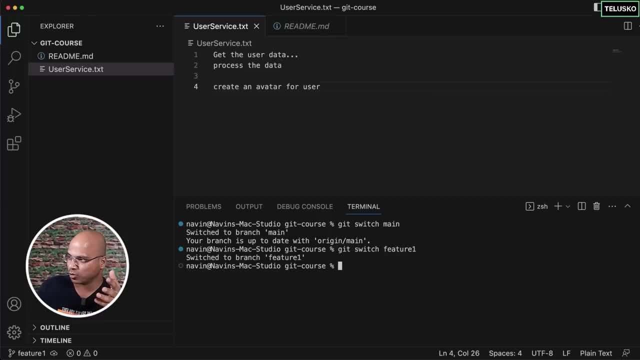 In fact, if you have more files in the feature one, it will also show those more files, And when you go back to main again, it will come back. So that's how, basically, you create a branch and you work on it. 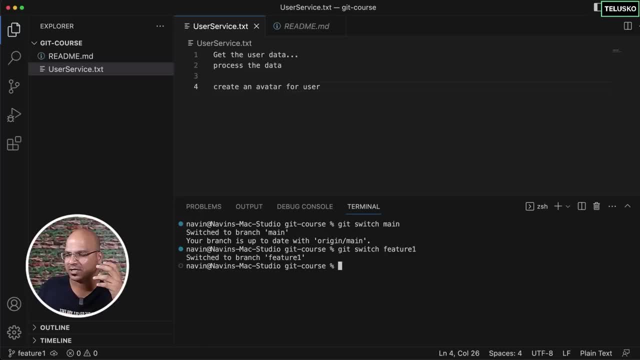 Of course you can create multiple branches. There is no limit. But what is the use of creating a new branch? right, Of course, if you can do something, you can do it on main branch And if you're doing something new on the feature one branch. 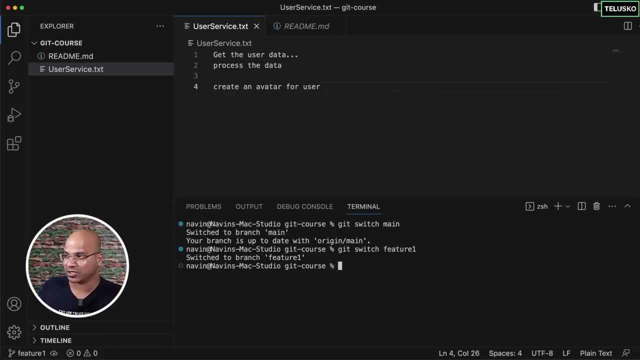 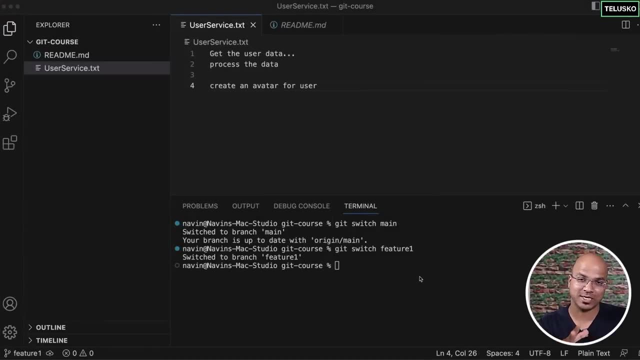 how will you get that data in the main branch? Again, that's a question we still need to answer, But we'll do that in the upcoming video. Now, in this video, let's try to create some more branches so that we can also see how do you delete a branch. 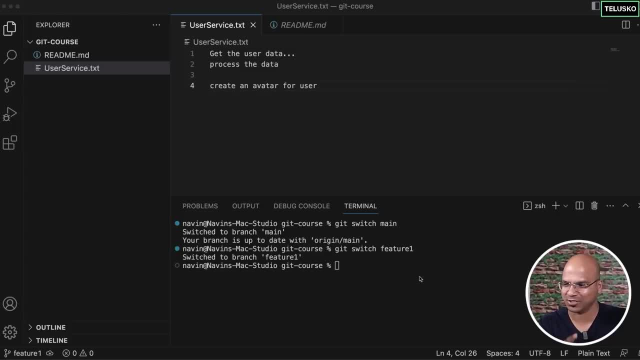 And also what's a shortcut to switch between branches? So let's try this first one. Let me create some more branches. So I will say: get, How do I create more branches? I can simply say switch. Of course, you can use checkout or you can use switch. 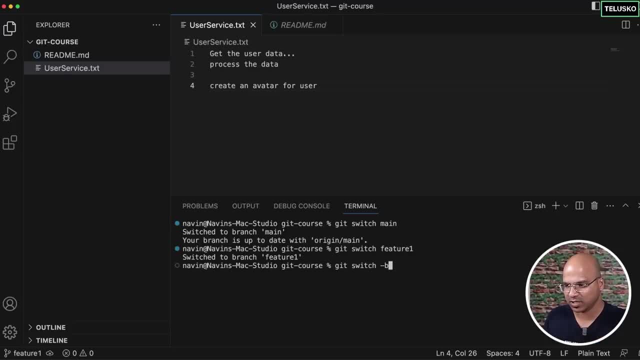 That's your choice. If you're using a checkout, you have to use hyphen b option, And if you're using switch, you have to use something called hyphen c. Now you can say hyphen c or you can say hyphen, hyphen create. 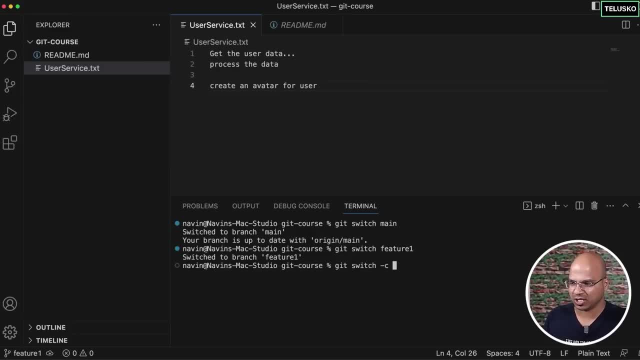 That's the option, And then you can mention the branch name. Let's say, I'm creating a feature, two branch, Okay, so I'm creating one more branch now. So in total, how many branches we have? We got three branches. 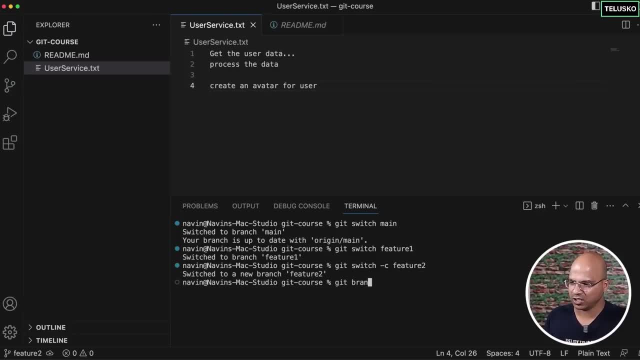 How do I verify? So either you can say get branch, Now, this will give you the list. So there's one option. Another option is hyphen, hyphen, all. Again, both does the same thing, But the difference is in this: get branch, you will see the local branches. 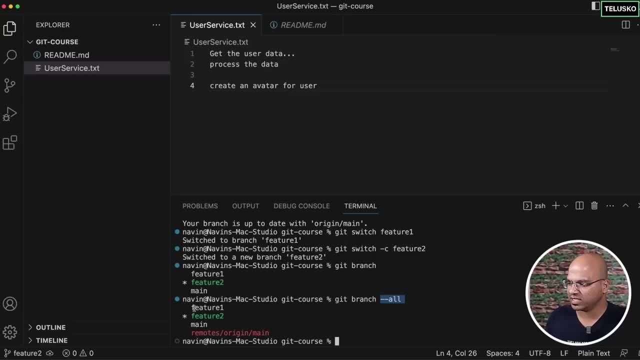 In get branch all you will see the local branches as well as the remote branch And if you can observe, in the remote, we only have one branch at this point. If you go back to your GitHub, we only got one branch, Okay. 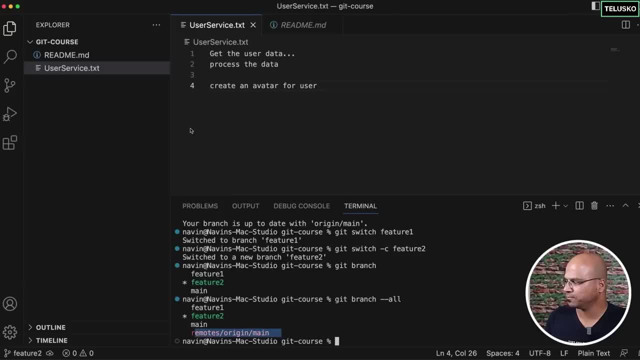 We don't have this feature branch yet, So we only have one branch, But we'll see. how do you push a branch to the GitHub? Now, at this point we can see we have only three branches, So we can check those things with the help of get branch. 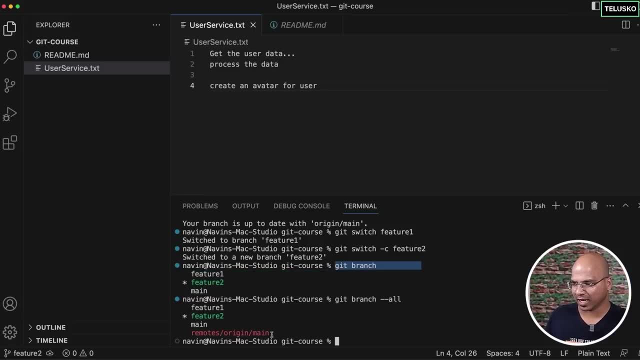 Or if you want to see the remote as well, you can say: get branch. all Now let's see Again. if I say get branch, we are into feature two right Now. what if you want to move back to the last branch? 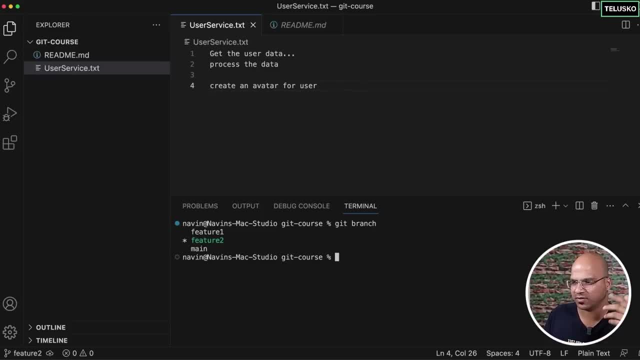 Now, since we say switch, it has created a new branch. But let's say, if I want to go back to the previous branch, I can simply say get switch hyphen. The moment you do that, now you can see it is switching back to feature one. 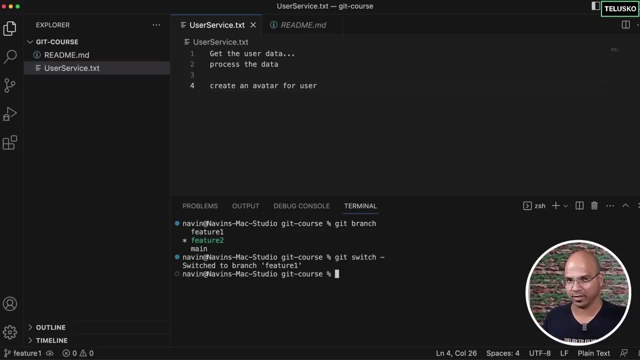 because we came to feature two from feature one. Okay, So if you want to do that shortcut of going back to the previous branch, you can say hyphen, That will be making it easy. Now, once we have seen this, let's also talk about deleting the branch. 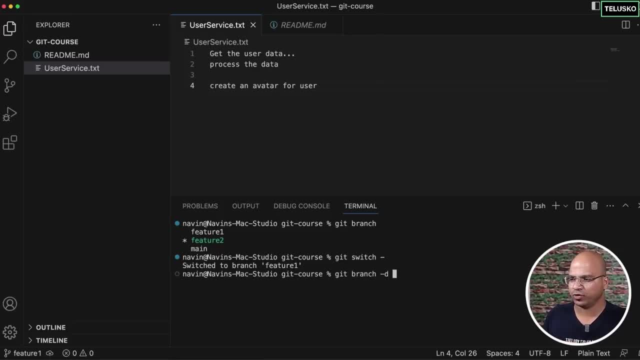 So you can say get branch And you have to use hyphen d. So if you want to delete a branch, you have to say hyphen d Or you can say hyphen, hyphen, delete, That's an option- And then mention the branch name, which is feature two. 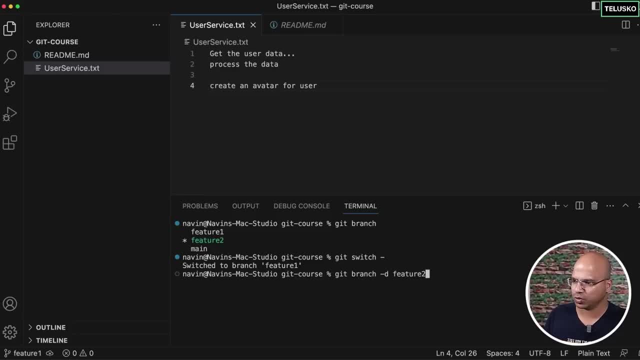 Let's say I don't want to work on feature two. So you can simply say feature two and then done, So you can see it has deleted the branch. And now if you check the branches, you've got only two. We've got feature one and we've got main. 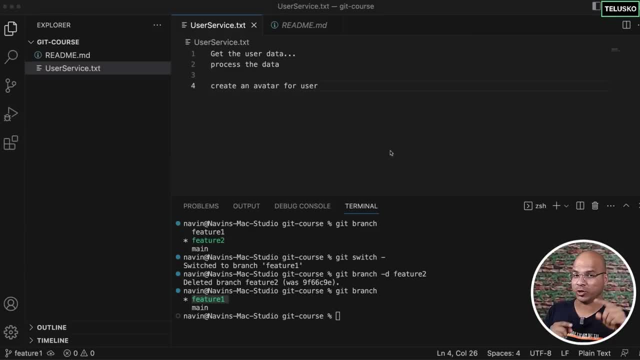 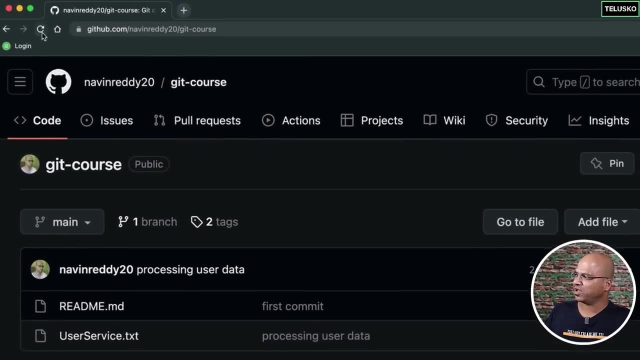 So now let's try to push the branch which is there in the local repository to the GitHub remote repository. So you can see we have a feature one branch. But if you go to GitHub you don't have it there. So even if I refresh so you can see in total we've got one branch. 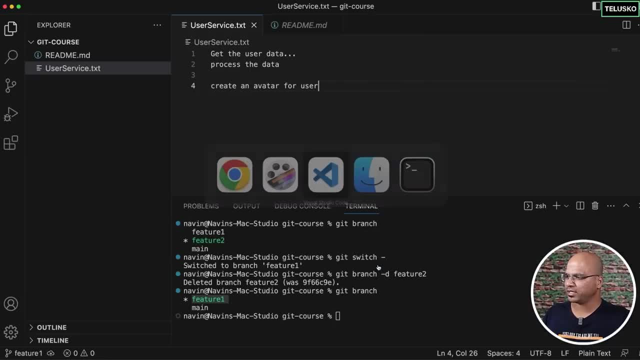 So let's create one. So what I will do is I will go back to my VS Code And this is where, okay, even before pushing it, I just want to make a few changes so that it will look good. So what I will do is, first of all, I have to check. 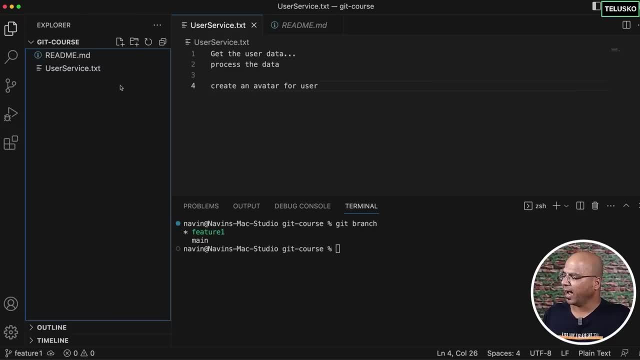 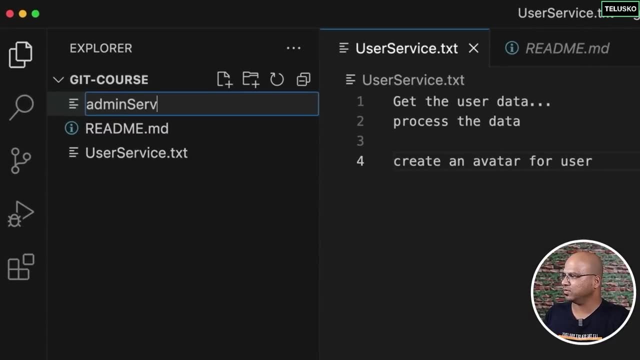 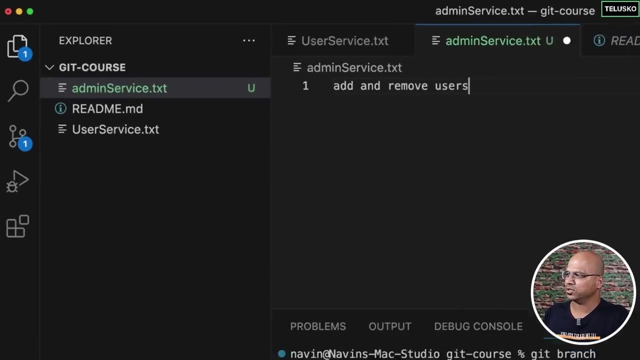 which branch I'm into. I'm into feature one branch And in feature one let me create one more file which is for the admin. So let's say this is adminServicetxt And what admin can do is add and remove users. 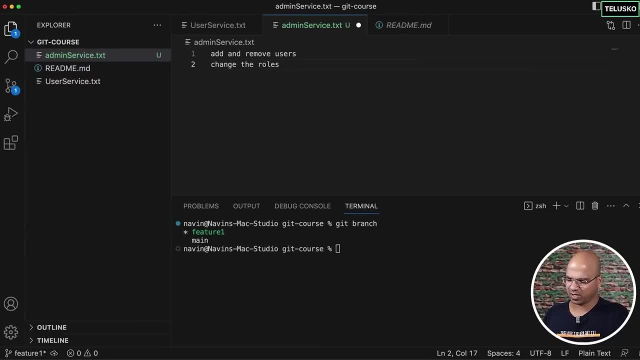 Change the rules, Okay, something like this. So again, assume I'm just writing one line of code, but behind the scene there are multiple lines of code, so that it will look good, Okay, So now what we're going to do is, first of all: 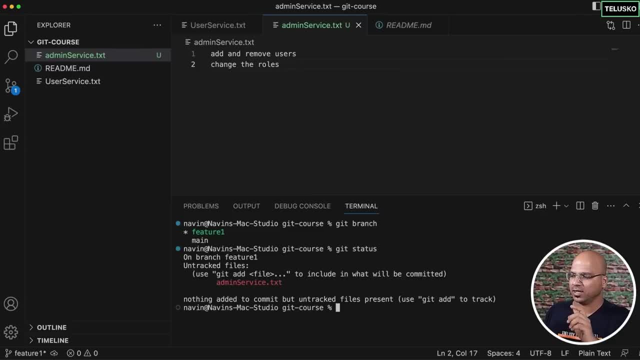 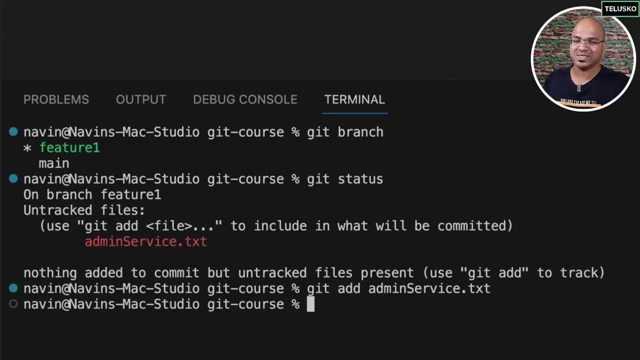 we are into feature branch, And in feature branch, if you say git status, there's one file which is untracked, So we need to basically add this file, which is the adminService. Now, once you have added it, it's time to commit. 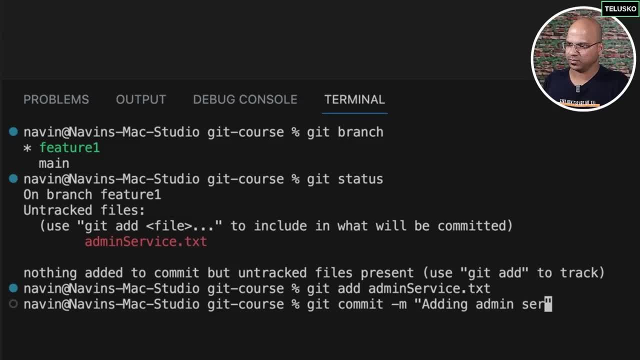 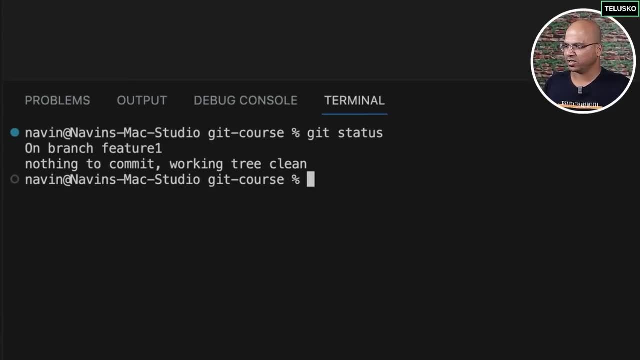 So I will say: adding adminService, Okay. So basically we have added one more service now. And if I say git status, everything looks good. But if you see, now we are into main branch, right. So if I see the branch, 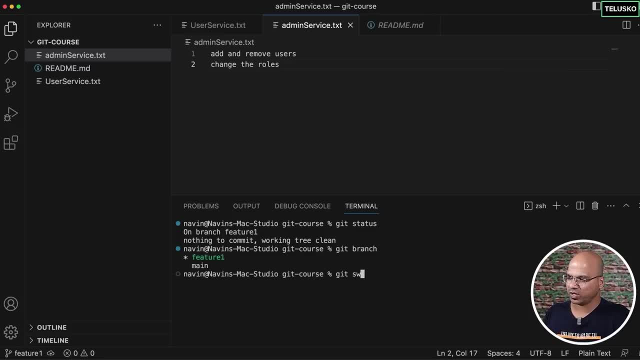 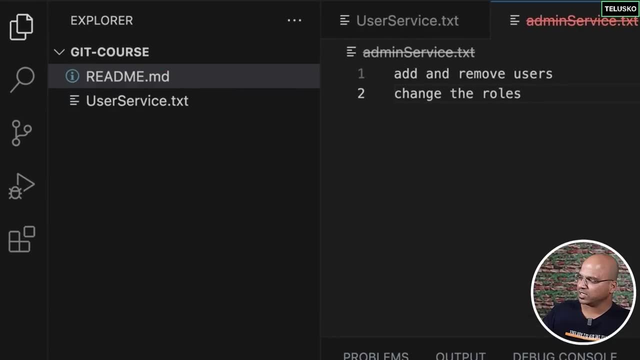 so if we are into feature one branch, and now if I switch to the main branch, just look. so the moment I say enter, see what will happen to the files. The moment I say enter, you can see there's one file which has been removed now. 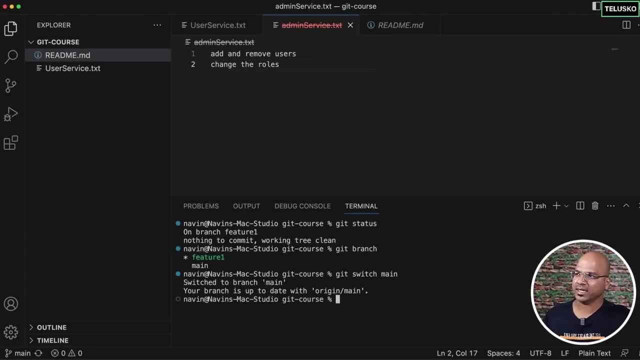 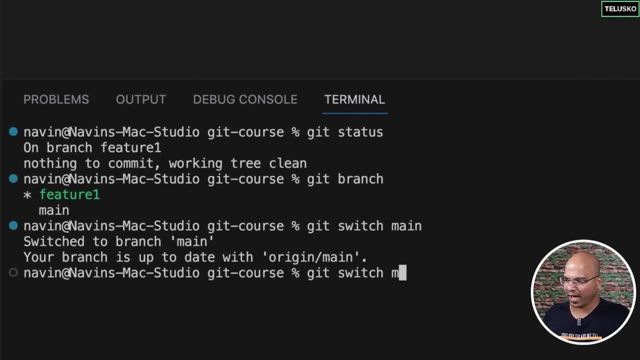 because the main branch has no idea about this file And that's why you can see there's also a cross here. But in main we only have two files. The moment I go back to the feature branch, now feature one, and if I say enter, 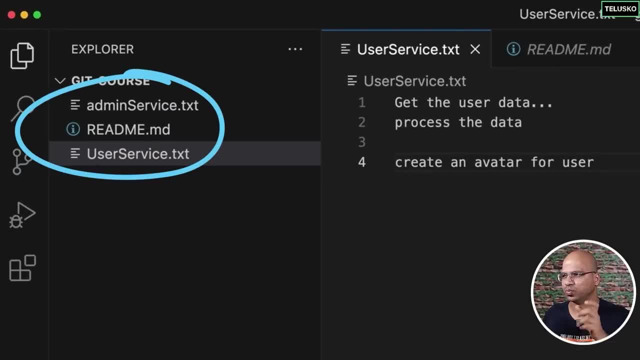 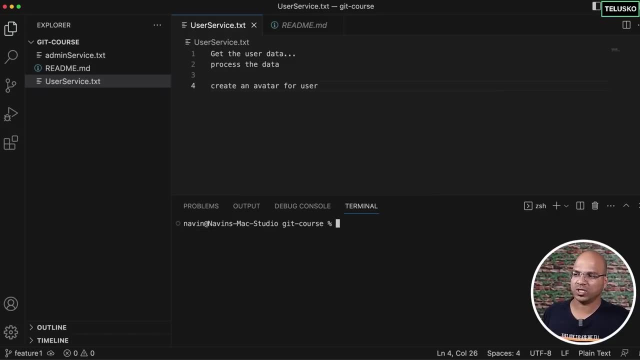 now you can see we got three files. So this is how, basically, when you work, you can actually work on those files. Okay, cool, But then I also want to push this to the GitHub remote repository, right, How do we do that? 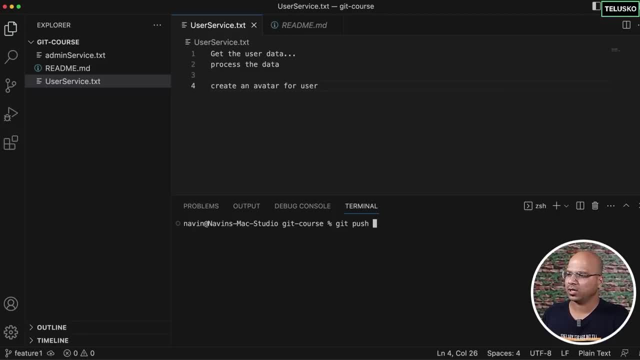 It's very simple now. So you can say: git, push origin, because that's the origin we have. And now we have to mention not main, because in the earlier case we used to say main, right, But this time we are pushing a different branch. 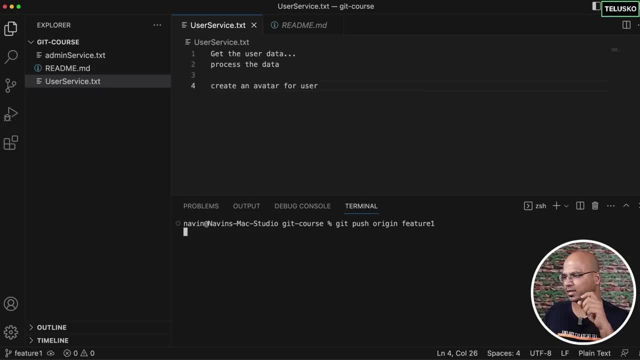 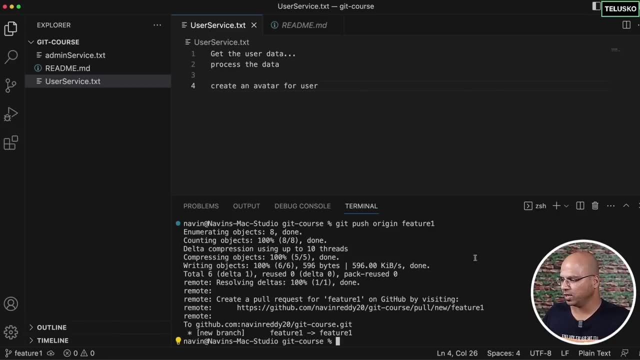 which is feature one, And when I say enter now, it is pushing this particular local repository to the GitHub repository. And it's done. You can see, there's no problem. It says on my remote repository, which is githubcom 1920,. 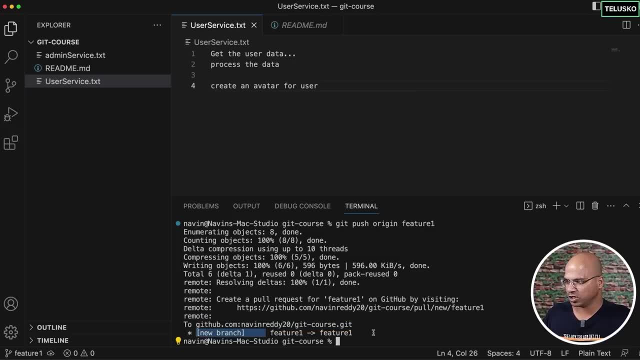 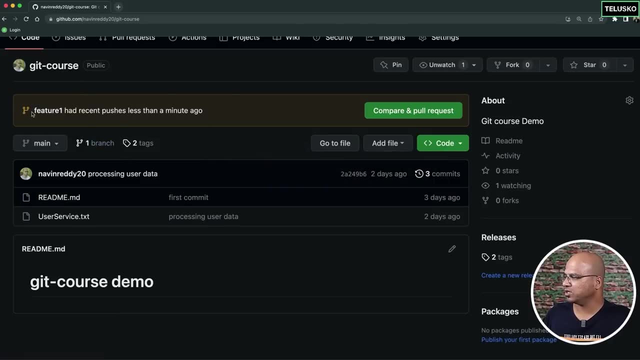 gitkosget. It has a new branch called feature. Let's verify, Let's go back here And you can see it still says one branch, But you can see there's a notification here. Feature one had a recent push less than a minute ago. 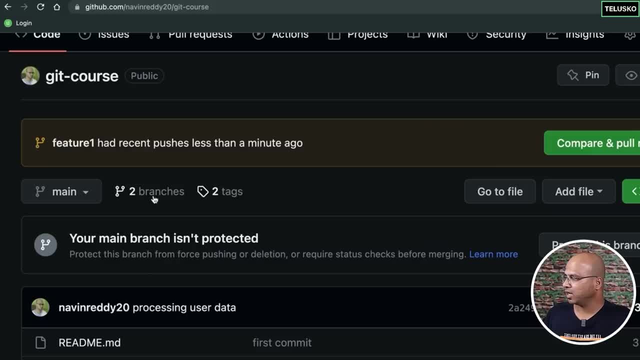 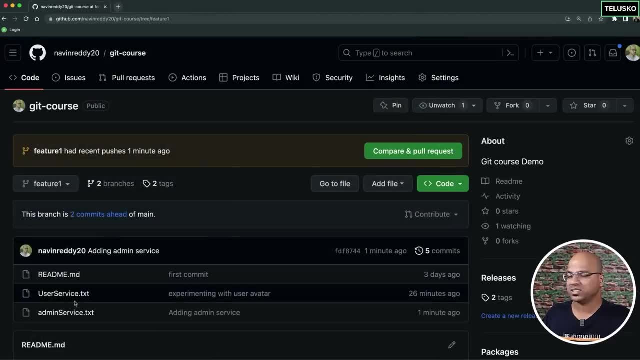 Okay, let me refresh to see two branches here And you can see now we have two branches. This is the main branch, But if you switch to the first branch, feature one branch- you can see you have three files. Okay, so this is the beauty of using branches, right? 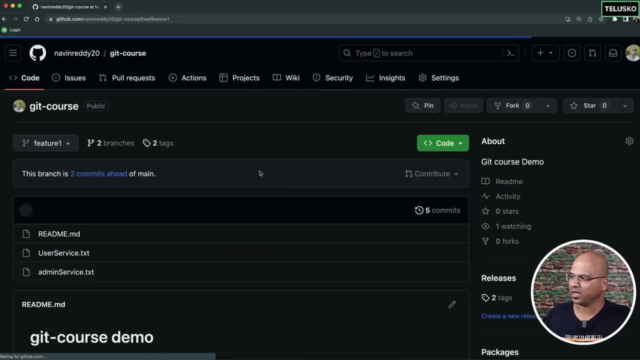 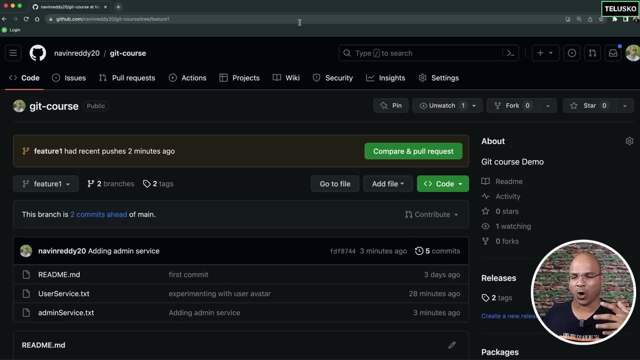 So you can also see that on the server. Okay, that's how, basically, you push the branch on the GitHub repository. So how exactly things are working here. So what happens when you create a new branch? Is it really copying the entire project and doing it? 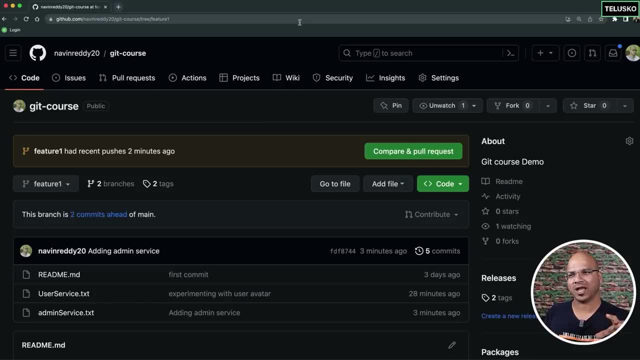 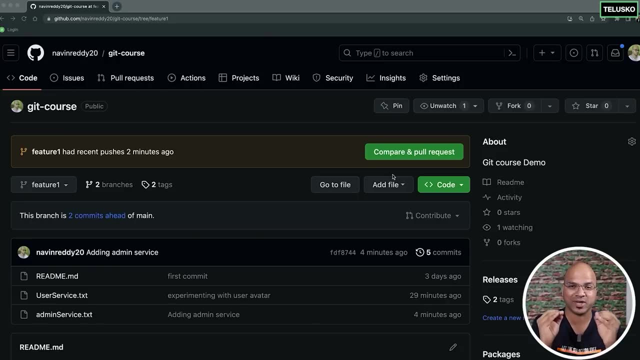 So let's try to understand that in the next video where we understand how branching basically works. So let's understand what happens when you create a branch. So let's say you have just done the git initialization on the working directory. Now at this point what happens is: 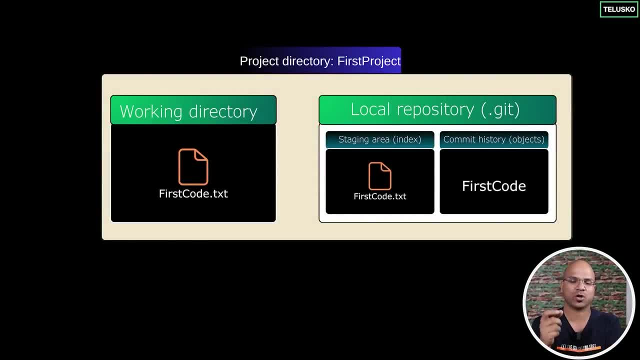 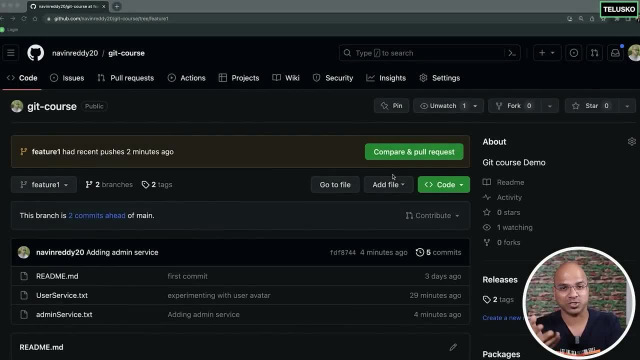 you get a different area inside your working directory which is called your git right git folder. Now, basically, whenever you do your commits, of course you have to do these commits in some branch right And by default when you say git init. 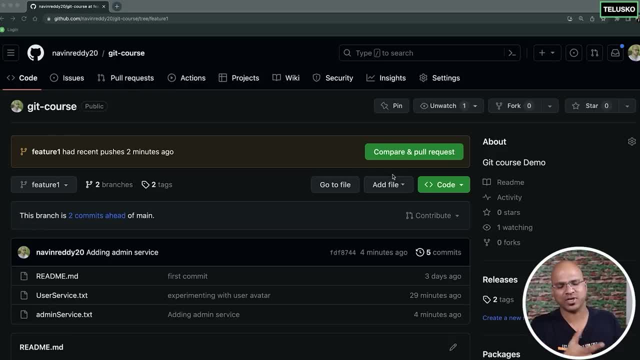 it creates a master branch. So let's say, in our case we are creating a main branch right. So default for us is main branch right Now. every time you basically do the commit, so let's say, when you do the first commit- 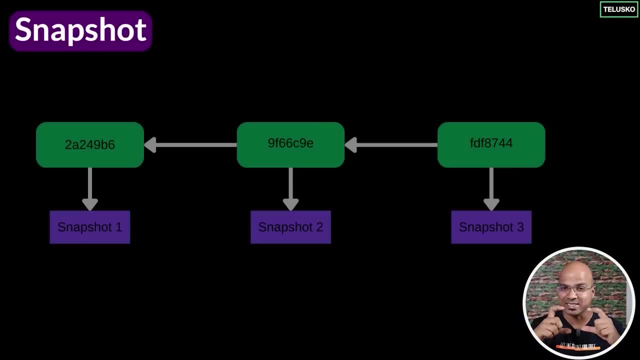 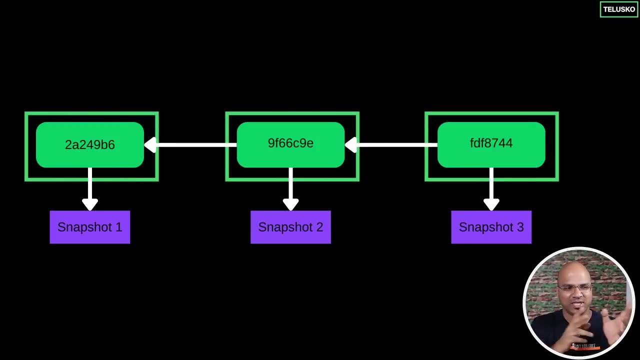 what git does is it creates something called a snapshot, So it will take a snapshot of your files, right, And then it will give it it's a commit number. That's your checksum. basically, We have seen the hexa code values, right. 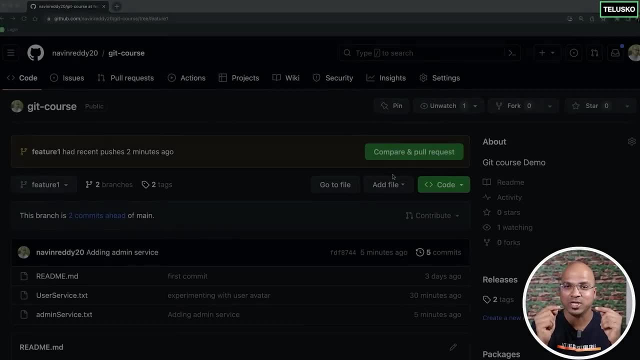 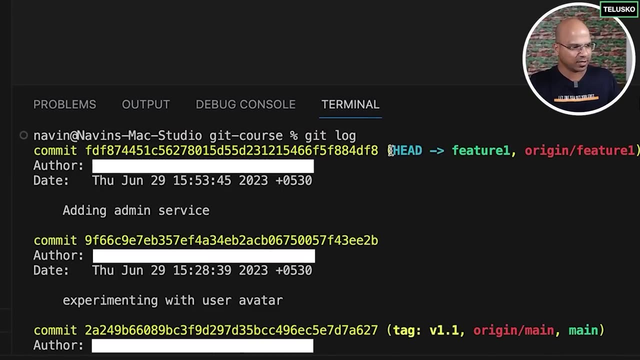 So that's your checksum. And then there's one more thing called pointer. Now how the pointer looks like, let me show you. So if you say git log, and when you say enter, remember this. we have seen this thing before. 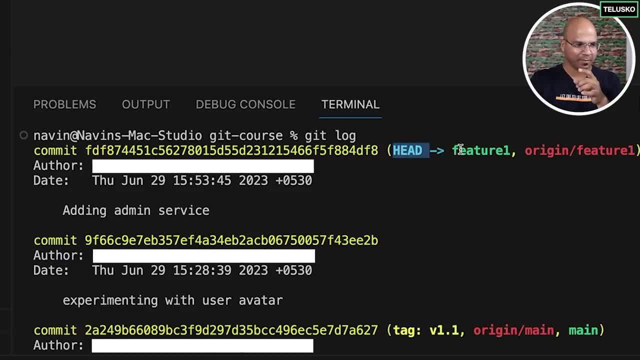 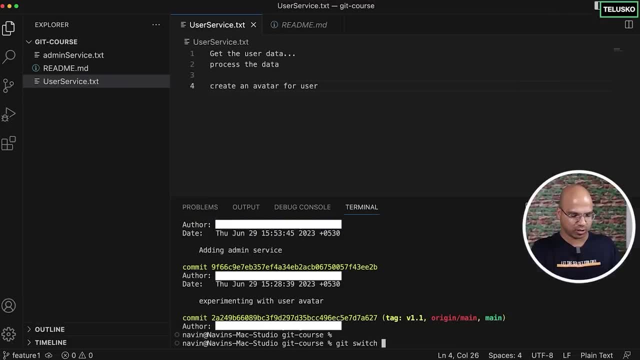 There's something called head, So at this point it is showing me a feature. because we are into feature branch, What I will do is let me just switch to. I will say git, switch main. And now, if I do, the same command again. 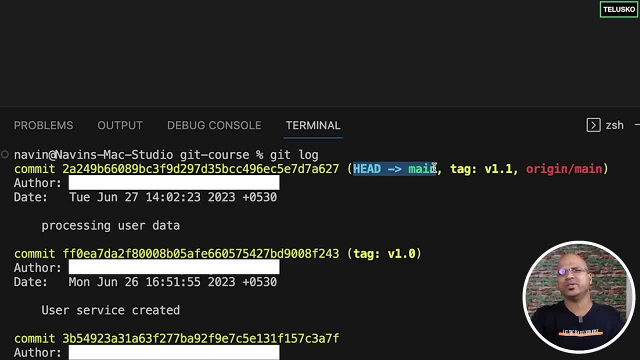 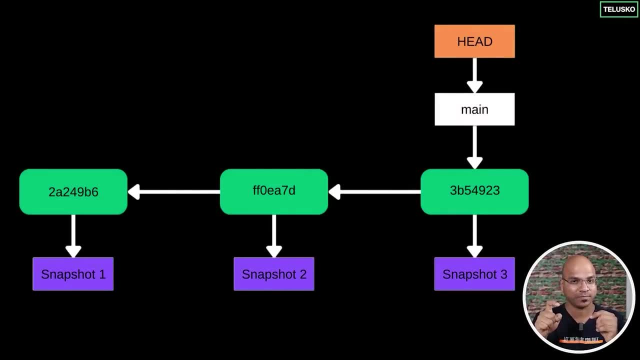 you can see it says head is towards main. Let's say we don't have a feature branch at this point. We only have main branch And then the head. so that's your main pointer. So it is pointing to the main branch, right? 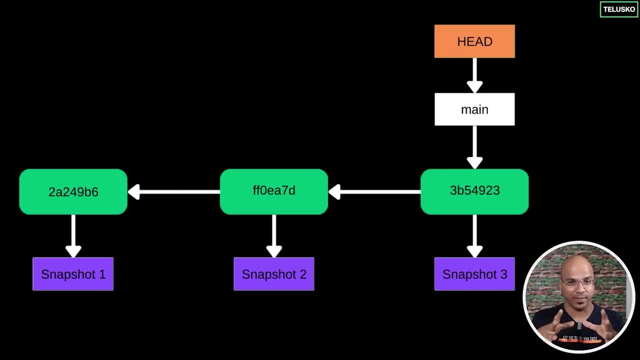 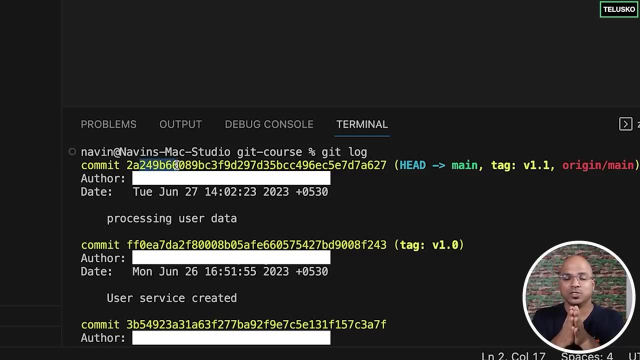 And main is basically pointing to your commit Now. the recent commit is this one, right Now, let's say, next time you are doing one more commit in the same branch, of course. So what it will do is it will take a snapshot. 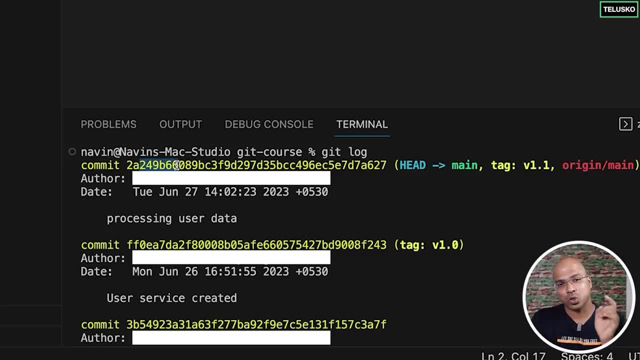 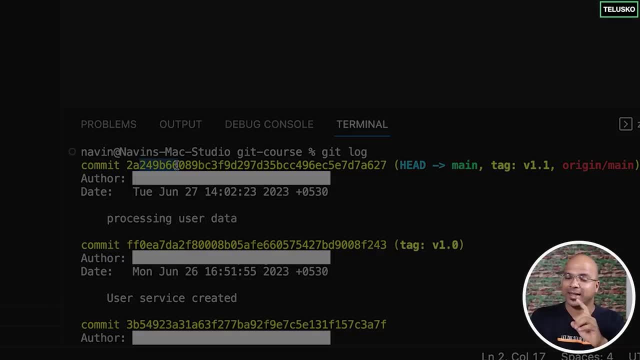 Now in this snapshot, basically you will have those files which have been changed. Okay, so it will not simply copy every file. It will copy those files which have been changed. Now, you have a previous commit, You have a recent commit with the new changes. 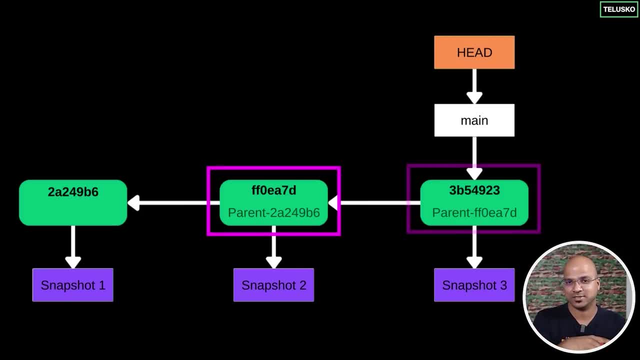 And then it will also have the parent commit. Why? Because if the files which have not changed is there in the previous commit, right. So basically it will have a pointer as well. So we will see that later how the parent looks like. 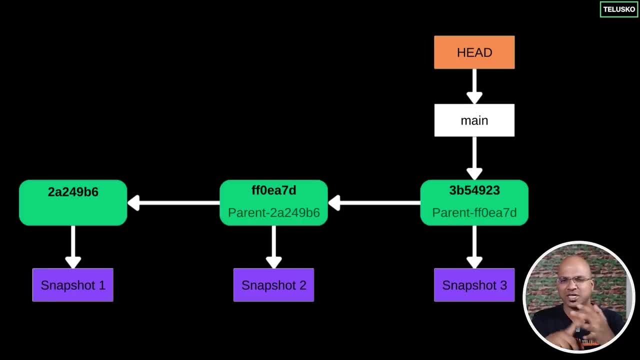 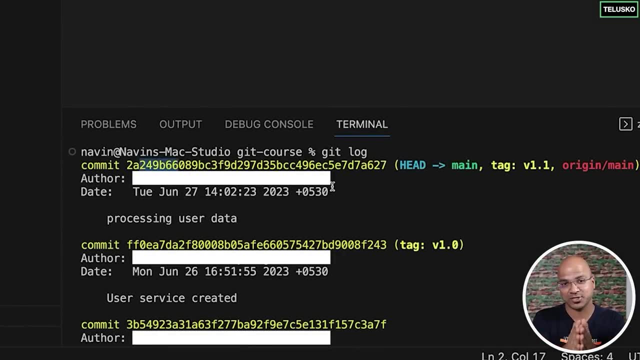 So it creates a parent, So it also has a parent. It has a checksum and multiple things. It also saves data in a tree format. But just to keep it simple, let's say we have checksum and the commit ID or the commit hash. 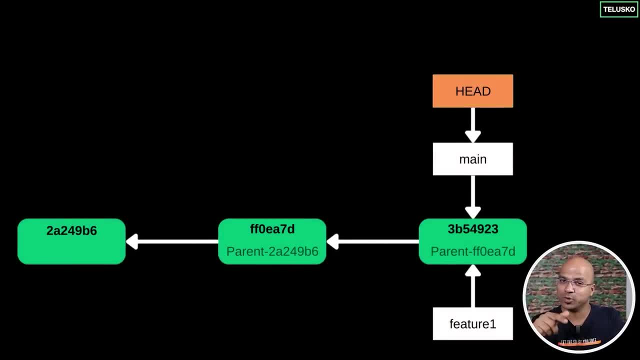 So the main is pointing to the new commit, The head is pointing to the new commit And now we are doing one more commit. So what will happen is, with the new commit, you will have a main pointing to the new commit and head is pointing to the new commit. 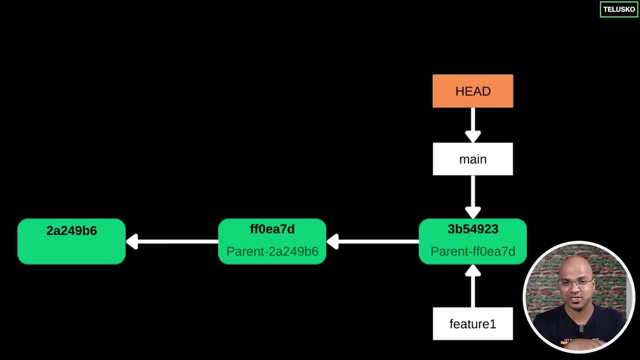 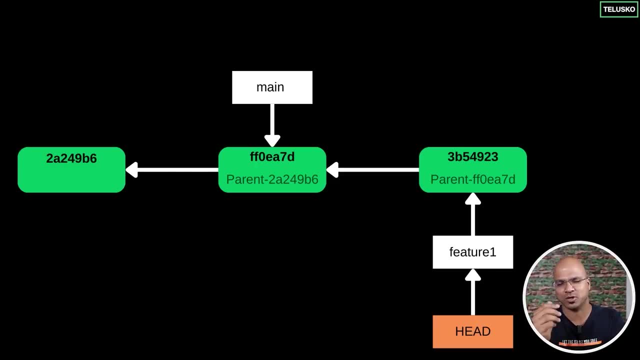 Yes, at any given point. if you want to go back to the previous commit, what you simply do is your pointer will move from the latest branch to the previous commit, whatever you mentioned, or latest commit to previous commit. It's that simple, right. 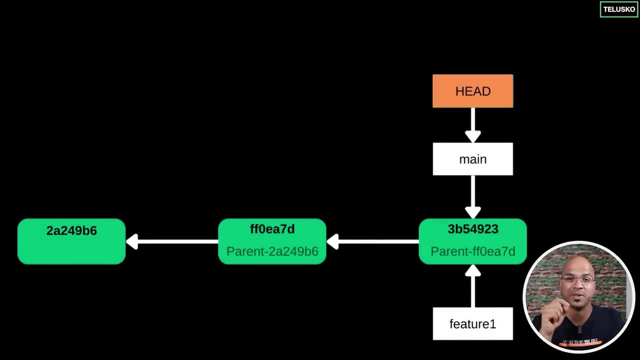 Now what happens is, at this point, when you create a branch, what is happening Now? basically, you have a main commit, right, The main branch. The moment you create a new branch, both the main branch and the new branch- 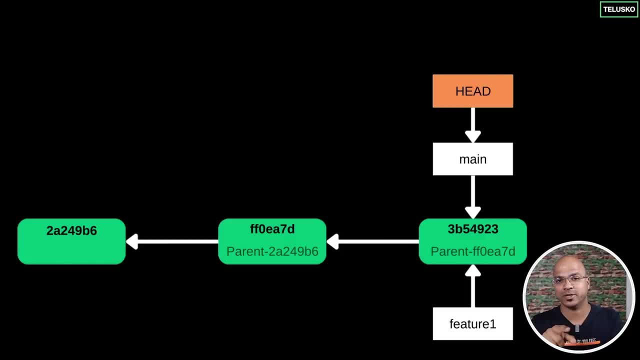 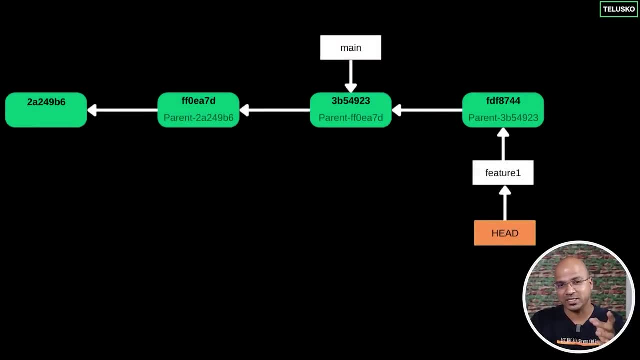 which is feature one in this case, is pointing to the same commit. Now let's say you decided to upgrade your features in the feature one branch. At this point it will create a new commit and your feature one is pointing to the new commit, right. 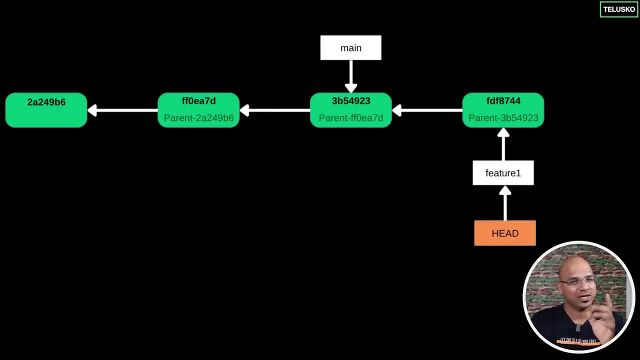 What about the main? Main is still with the old commit right. So that's how, basically, you create two different branches and you can work on them individually. If you want, you can also work on main. Maybe you want to do some more commits there. 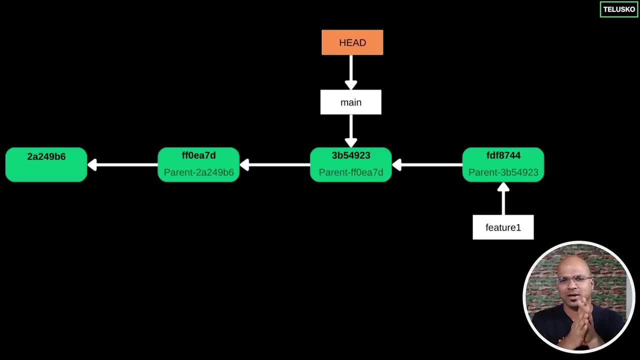 because maybe after the main commit you found some bugs. Of course you are working on feature branch, but let's say you found some bugs in the main. Now of course you will not directly work on feature one. What you will do is you will create a new commit from the main. 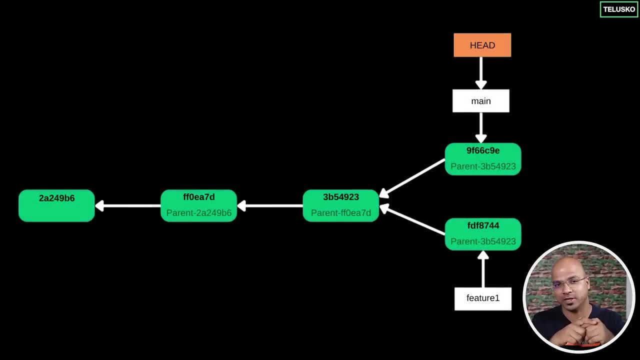 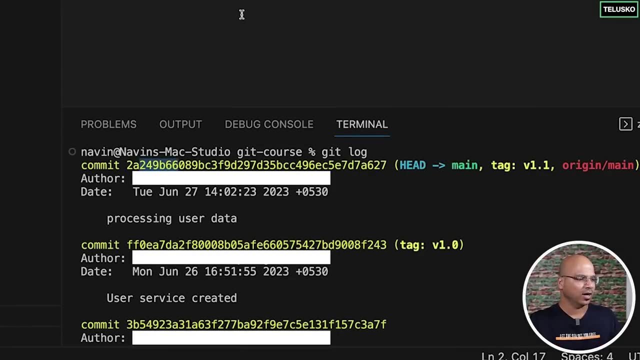 So the main will be pointing to the new commit now and the feature is pointing to the other commit. So that's how basically it creates the branch Now. if you want to visualize this, of course you can do git log. It will give you all the logs, right. 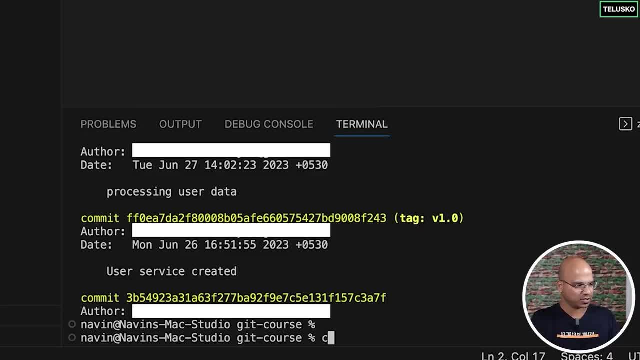 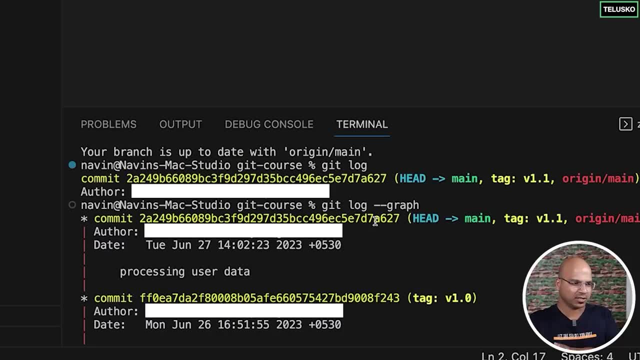 But there's one more command. You can say git. Let me just clear the screen. So there's something called git log and you can draw a graph here. Now, to this point we have not done any merging. That's why it is only showing to the main one. 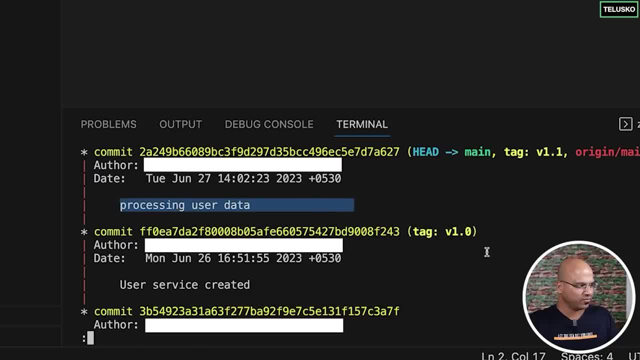 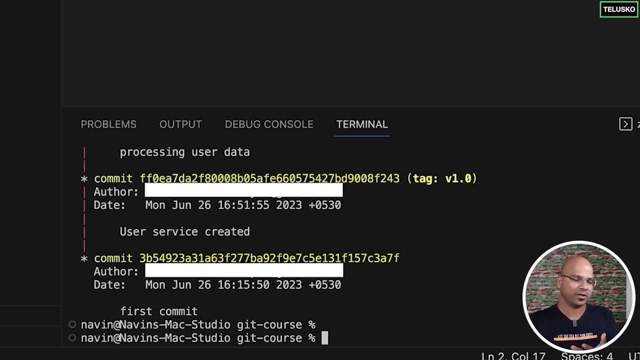 So it says: what are the commits? What was the message which you have done? So the commit and the message, And the commit and the message. if you say enter, you will see more. Now, if you want more visual representation, 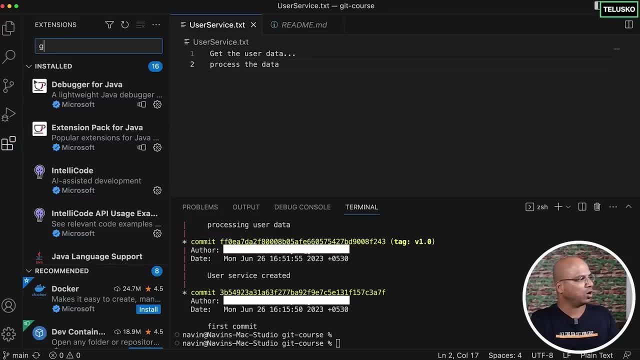 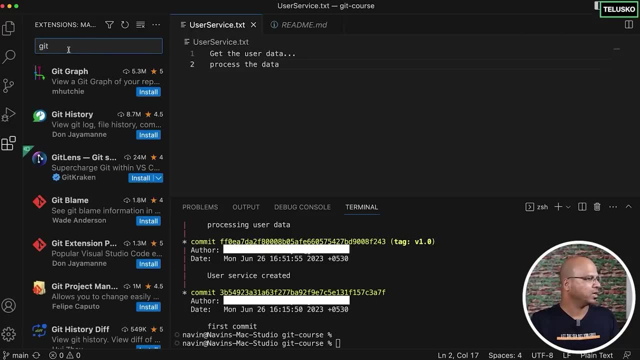 what you can do is you can install one extension, which is called git graph in VS Code And okay, it failed to fetch. Okay, So you can see there's something called git graph here. This is the logo, if you want to download. 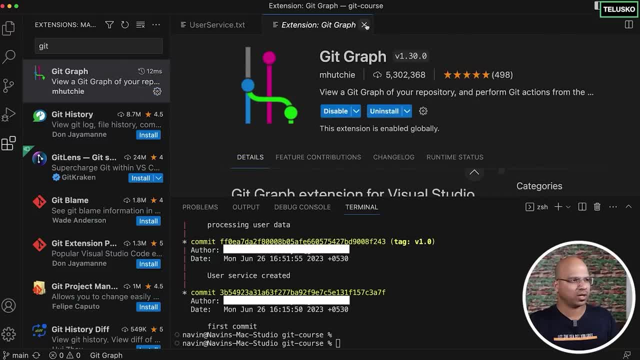 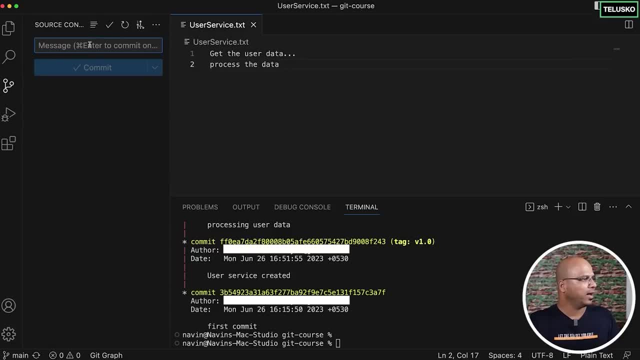 And when you say install, so it will take some time to install, I think it's done. And if you want to use it, you have to go to this particular icon here, which is for the git or source control, And there's an option here. 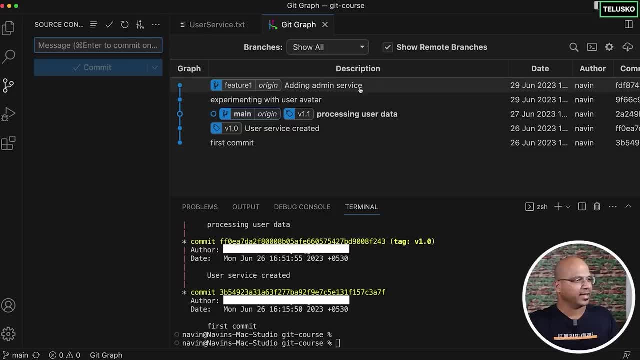 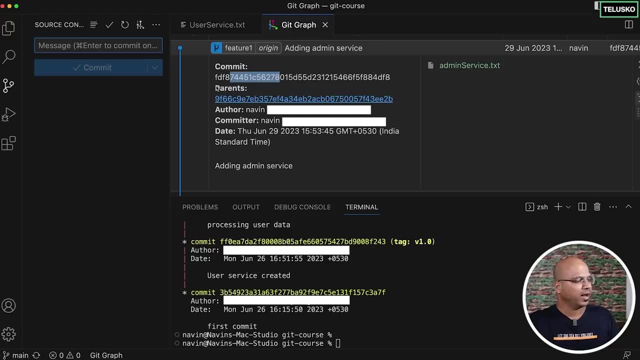 So, if you can see, this is a button which you have to click And now you can actually visualize everything. So, if you click on this, these are the things which happen with this particular commit And this is what I was talking about: the parent. 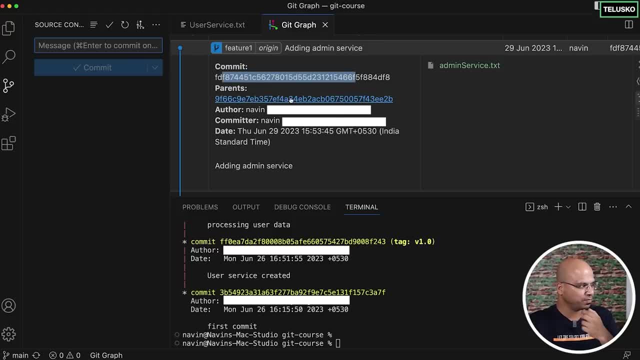 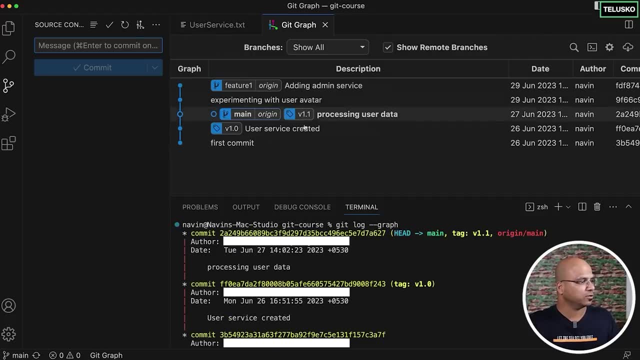 For this particular commit. this is a parent right. This was the previous commit, So if I want to show you in the console as well, we are into feature right. We should focus on the main, not feature, Because in this we are into main. 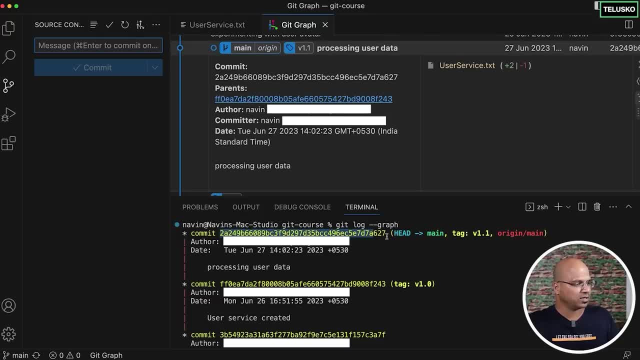 So I will just click here. So yeah, this is the commit right, The recent commit, And that's what we have here. And for this commit the parent is one commit before that. So you can see it says parent Now of course for one particular commit. 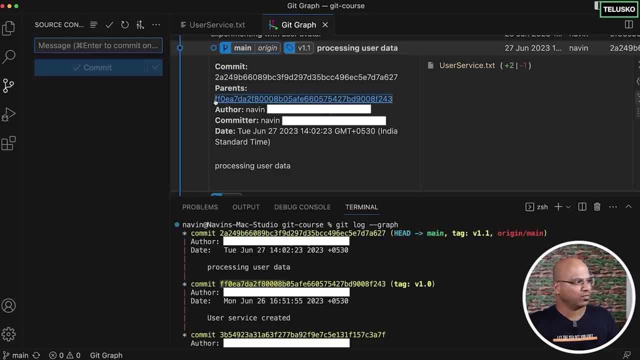 you can have multiple parents- We'll see that later- But at this point you can see we have only one And that's why I say there's a plural form right, Which is parents, And that's how, basically, you can see the things here. 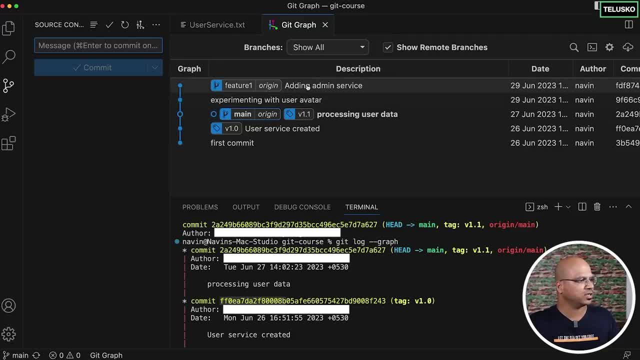 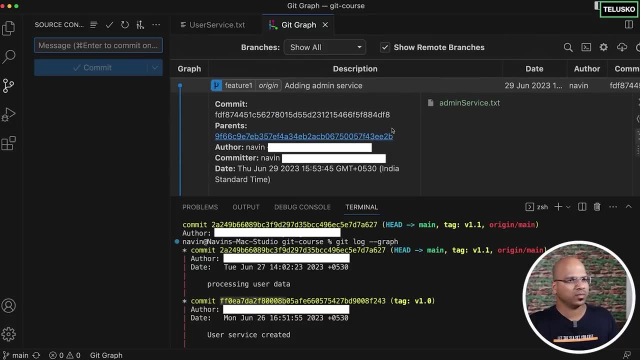 So, yeah, explore this And we'll try to understand this more. So you can see, at this point we have created a new branch which is a feature branch. Everything else is happening on the new branch. So, yeah, that's how branch basically works. 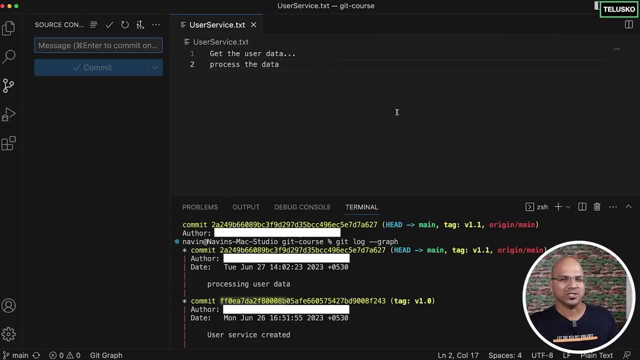 And now we also want to understand how do you merge two branches. That we'll see in the next video. So basically, now we have two branches, right? So if you want to see them again, what we can do is I can just clear the screen. 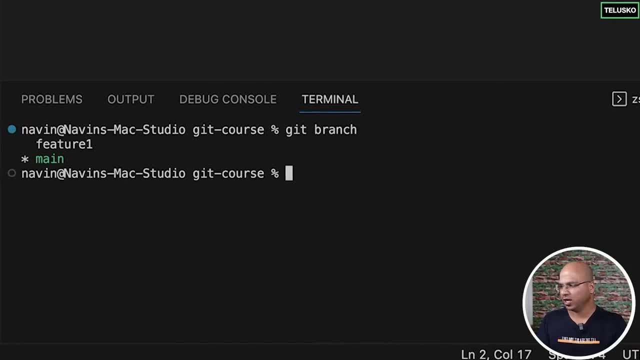 And I can say: get branch, And you can see we have two branches, right. And now what we want is we want to basically merge these two branches. We want to merge main and feature one. So of course we have done the work on feature one. 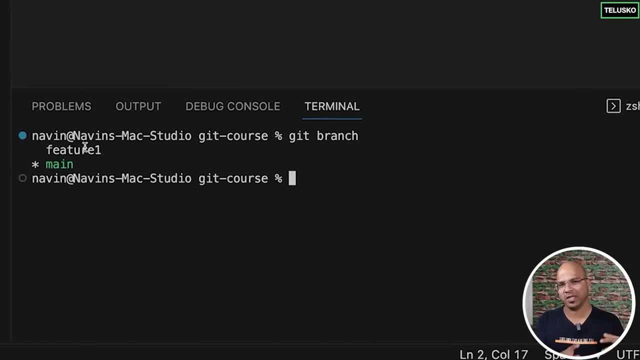 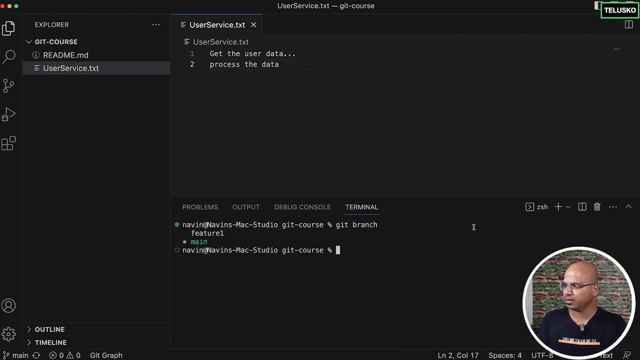 It looks good. I just want to merge it to the main branch. How will I do it? So the first thing is: first of all, let's explore the files. I am into my main Right And if I go back to git, switch. 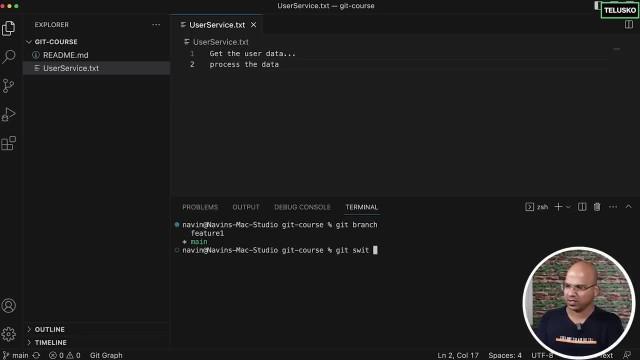 just check what are the difference we have here. So if I say git, switch to feature one, and you can see there is extra file here which is admin service, I just want to check if everything is good, that it's clean. I also want to verify if we have admin service on the GitHub. 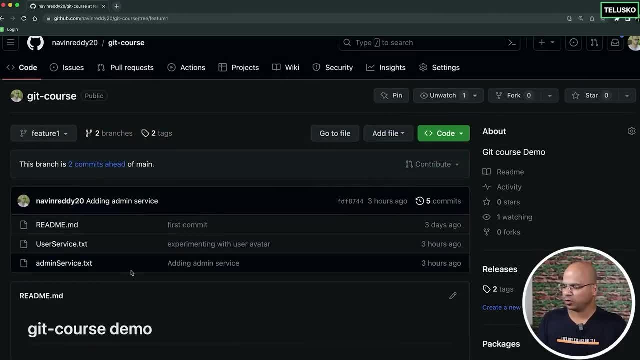 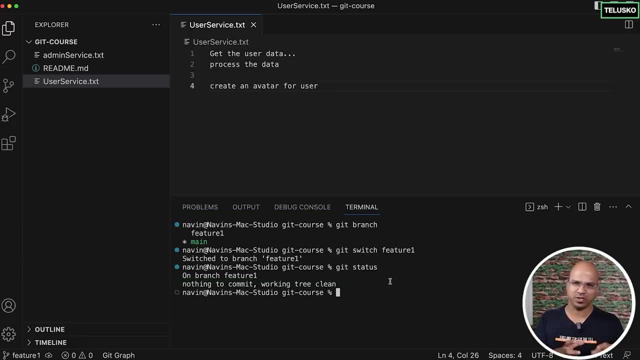 So if I go there, if I refresh, So yes, we also have admin service here. So that looks cool, right. So now what I will do is I want to merge the data or the features in feature branch to the main branch. 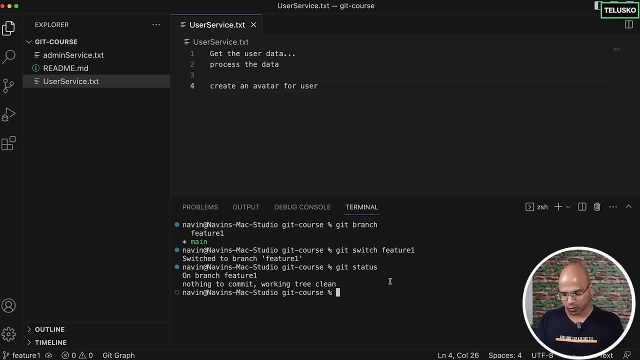 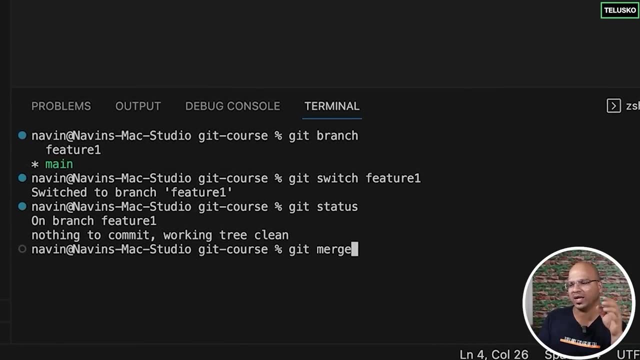 How will I do it? How do we merge? So, to do that, what we need to do is we need to use a very simple command called merge. Basically, there are two ways of doing it. One is merge, which we are doing now. 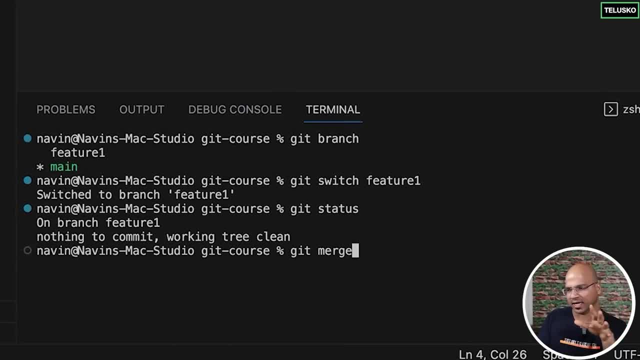 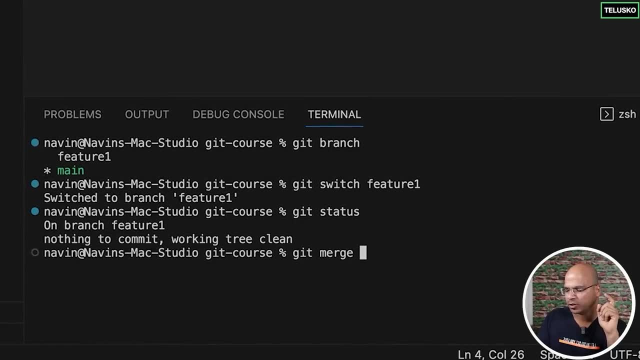 And the second one is rebase. We'll see later what rebase is, But at this point let's focus on merge. So we are saying git merge And then we just have to mention this, We have to mention the branch name. 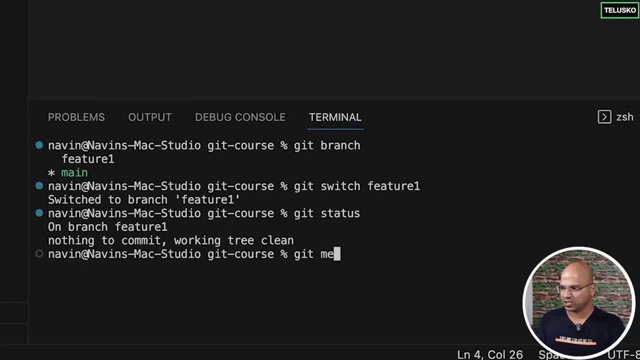 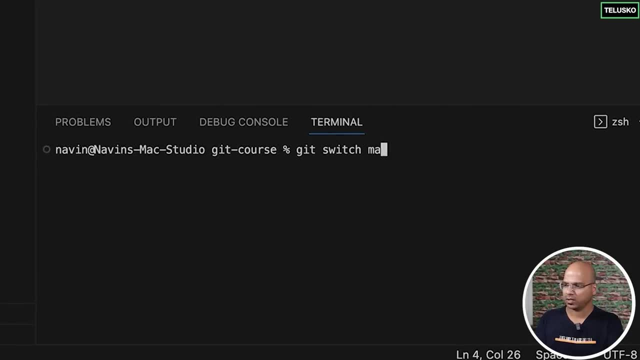 But to do that we have to make sure that we are in the main branch. So if you see, if you check which branch we are into, we are into feature branch, So we need to move. So we'll say: switch to the main branch. 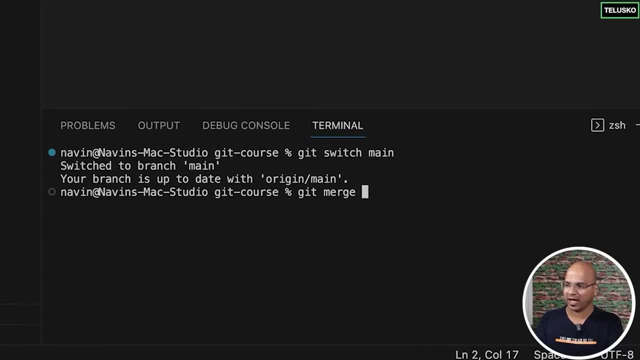 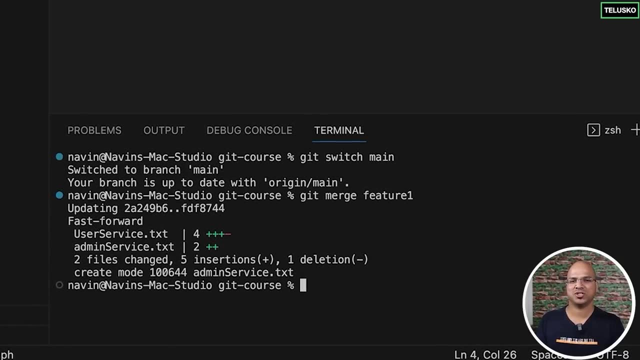 And now we can do git merge. So we just have to say git merge and the branch name, which is feature1. And when you say enter, okay, it worked, The merge is complete. There's no problem. Sometimes you do get problems. 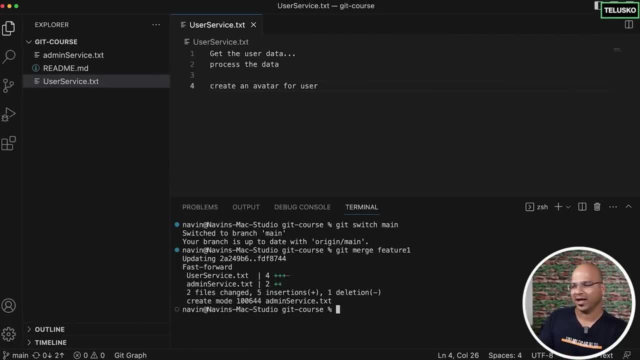 We'll call them as merge conflicts. We'll try to create merge conflicts later And we'll also see how do we resolve it, But at this point there's no issue And you can see we got git merge And it's working. 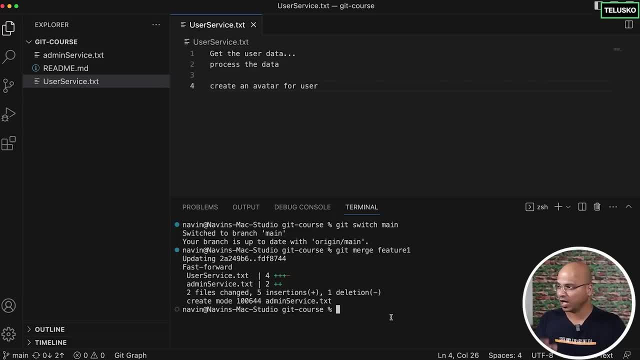 How do I verify this? If you go back to your main branch, of course we are in the main branch And in main branch you can see we have admin service. Okay, That looks cool. I just want to see if git status and everything looks good. 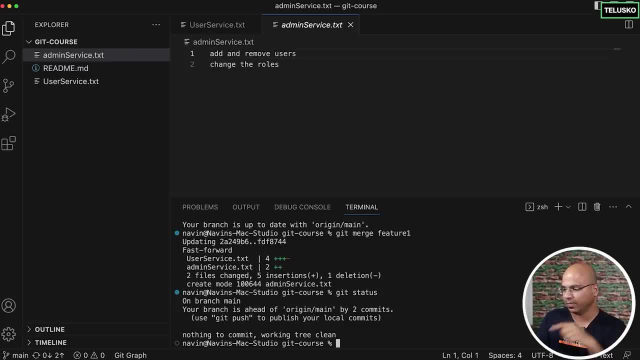 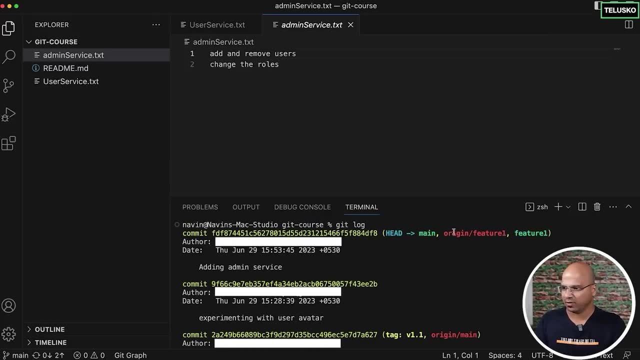 because the commits which happened in feature1 also came into the main. Okay, The way you can verify is by doing a log And you can see we were basically done this thing in the feature, But now it came into main And we can also verify that with the git graph. 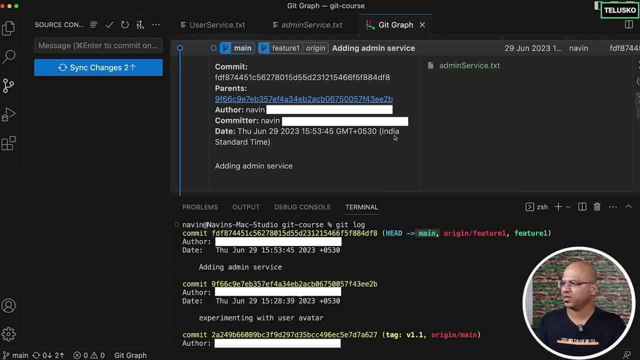 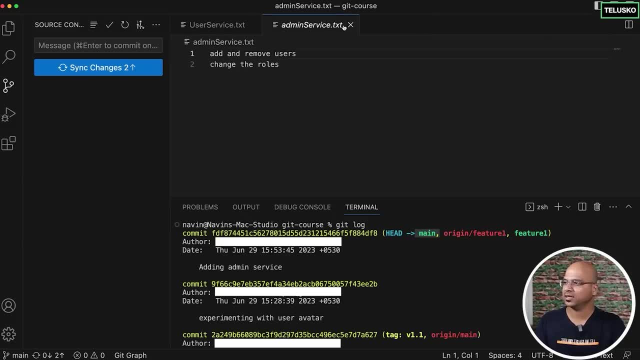 And if you see here, that's why we have done the merging right. So now it came into main branch from the feature branch. This is what it says. Okay, So merging is complete. If you go back to your GitHub and if you see here: 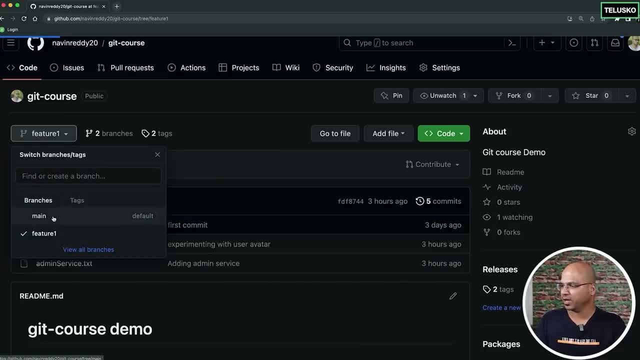 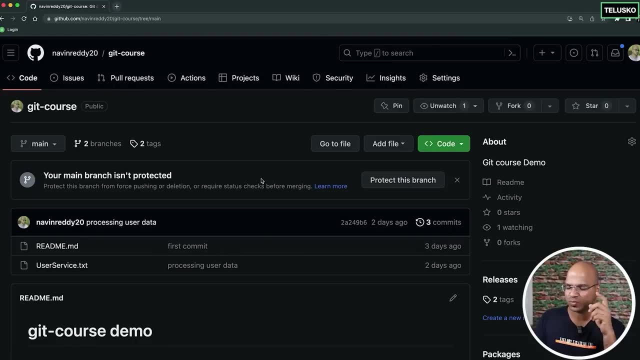 in feature1, we have three files, But if you look at your main branch, we only got two files because the update has not happened on the server. Okay, There's one thing which I missed. Normally whenever you do this merging and pushing on the remote repository, 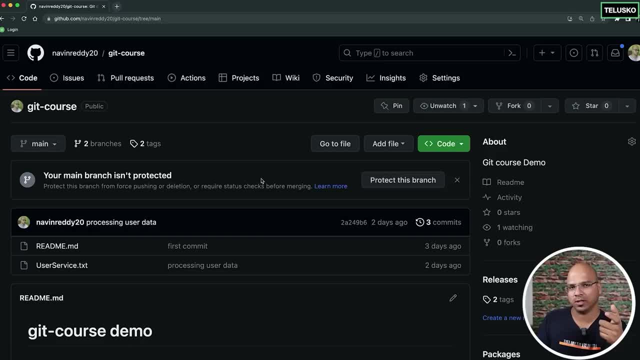 of course you have to push right. The first thing you do is you pull your remote repository. We have not done that because it was safe for me, because I'm not doing any. We don't have any collaborators, We're not working on main separately. 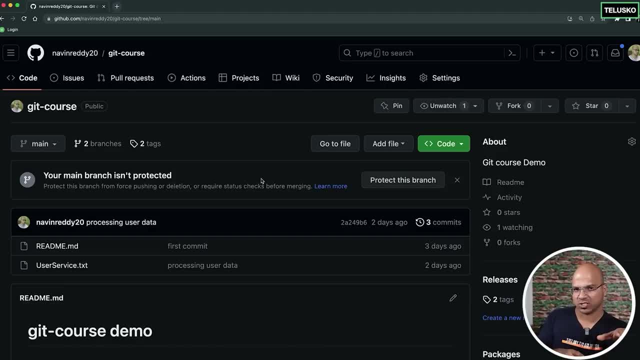 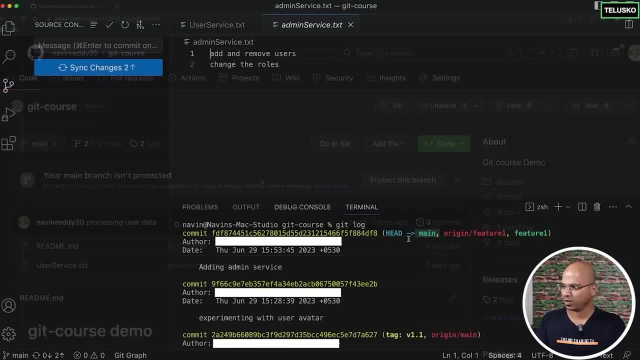 But that's a good idea. Always try to pull first. Okay, Because when you say pull so from the remote repository, you will get the updated code on your machine before merging, Okay, So how do you pull, basically, if you want to do that? 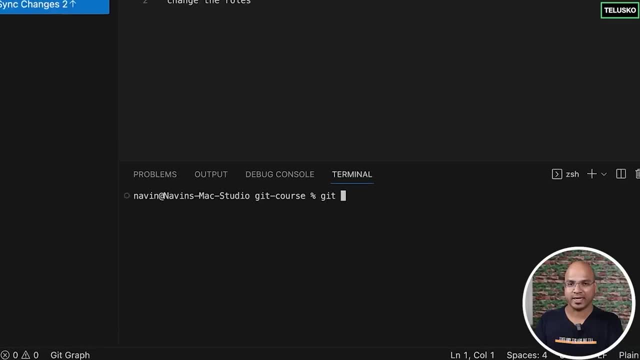 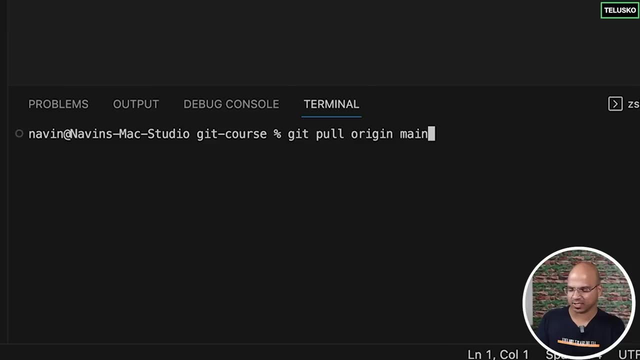 It's very simple, Let me just clear the screen. So you have to say git pull the same way you do push. So you have to say git pull origin And you have to mention the branch which you want to pull, which is main in this case. 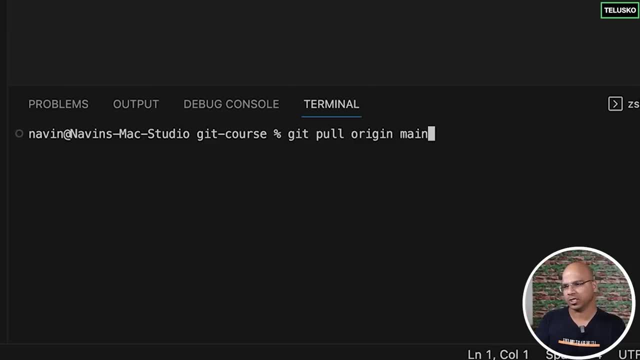 This is the step which you should have done before merging. Okay, But anyway, we have done the merge And now it's time for us to push it to the remote repository. So we'll say: git push origin and we have to push main. 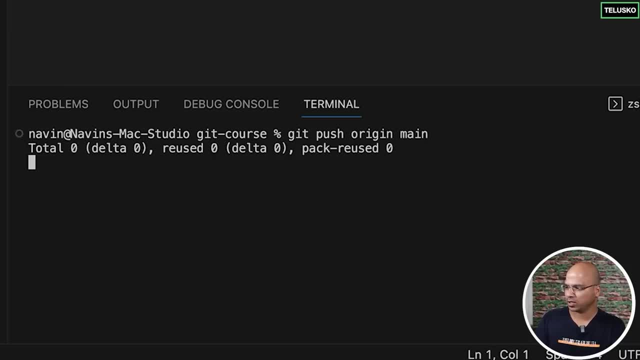 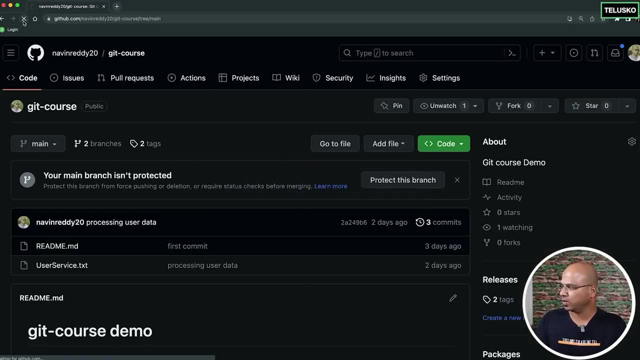 Let's do that. Things are looking good, There's no problem And done. You can see the pushing is done. Let's go back here And when you say refresh now in the main, you can see we have three files. 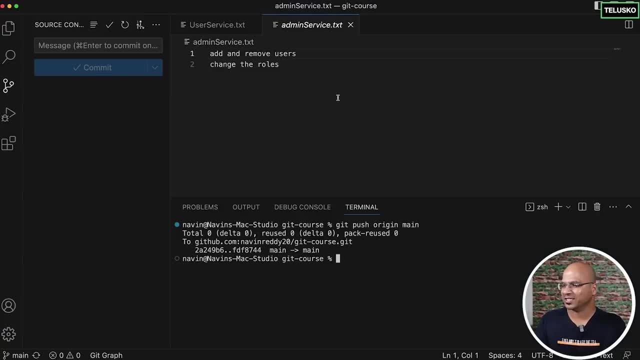 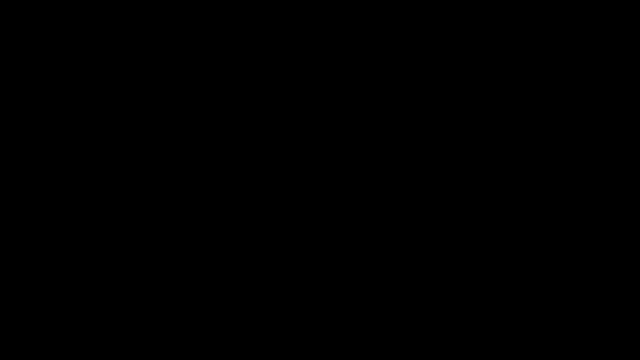 This is updated And we are good. Okay, So that's how, basically, you merge. Thank you so much for watching everybody. 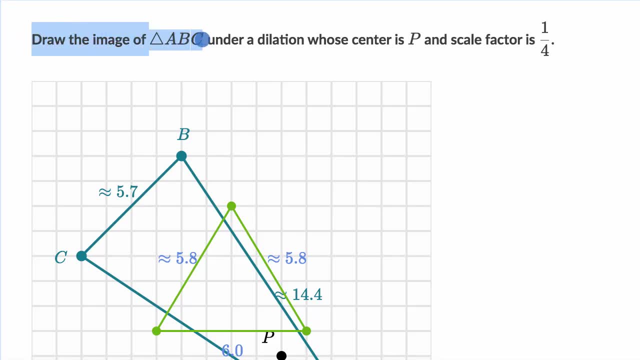 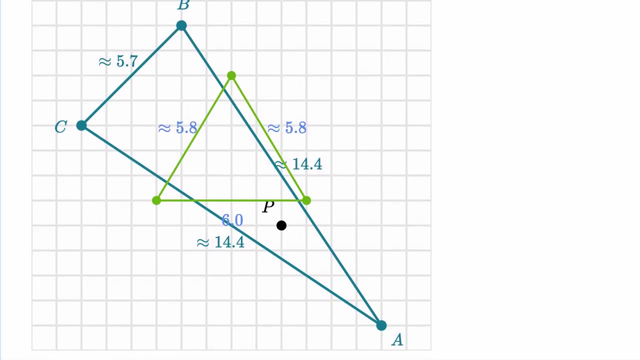 We're told, draw the image of triangle ABC under a dilation whose center is P and scale factor is 1- 4th, And what we see here is the widget on Khan Academy where we can do that. So we have this figure, this triangle ABC.